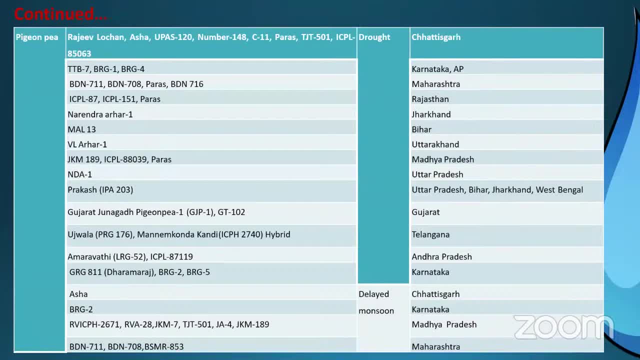 And ICPL 87. Narenahr, Etc have been developed that shows resistance to drought conditions and can be grown in different agricultural zones or areas of cultivation, while certain varieties such as Asha, BRG2,, etc. also shows 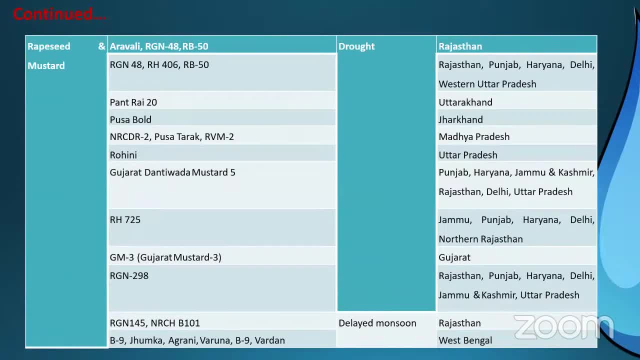 tolerance to delayed monsoon condition. Similarly in case of rapeseed and mustards also. this is also one of the most important crop that is grown in the rainfed area in India, and a number of different varieties which are resistant to drought conditions, which are tolerant to delayed monsoon. 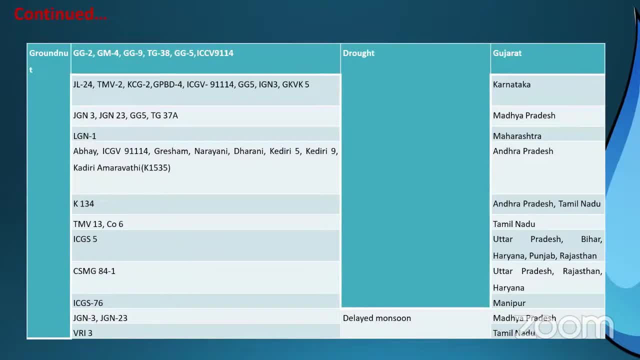 conditions have been developed in this as well. Groundnut, again, is another oilseed crop that is grown in the rainfed conditions in India, and certain varieties such as JGN3,, JGN23,, LGN1, K134 have been developed that shows resistant to drought condition, while resistant to delayed 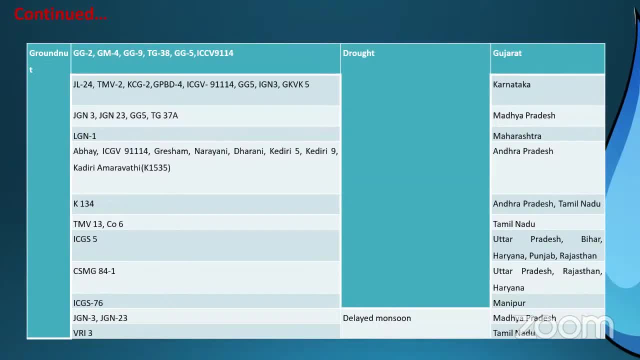 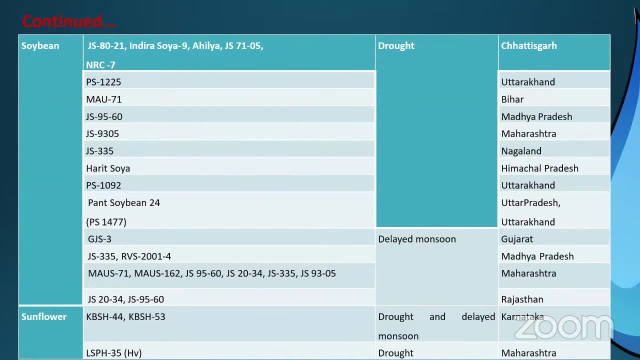 monsoon condition have been shown by varieties such as JGN3, JGN23,, etc. Then soya bean: again, a number of different varieties have been developed that are resistant to drought condition, tolerant to delayed monsoon condition in case of sunflower. 2,. 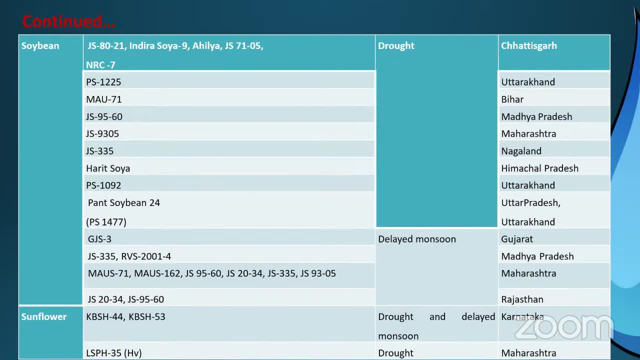 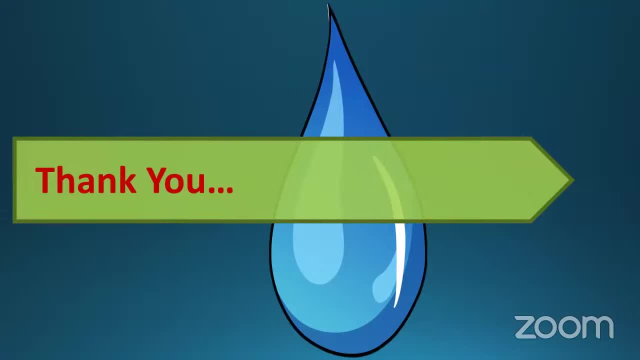 a number of different varieties have been developed that are resistant to drought condition, and a number of varieties have been identified which shows resistant to drought and delayed monsoon. So this shows that cultivation of the climatically resilient varieties provides the effective mitigation for climate change and therefore must be promoted, And also this is 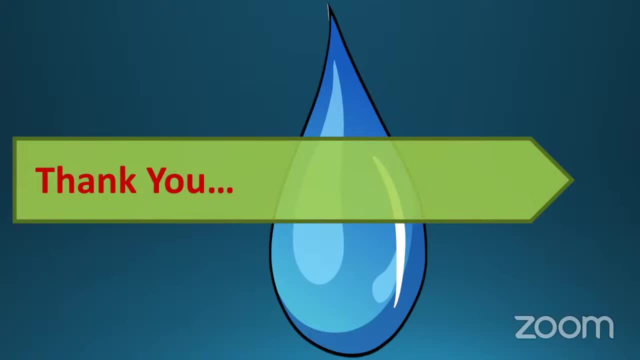 one of the most cost-effective measures that can be taken in order to mitigate the effect of climate change and reduce its effect on the crop yield. So, therefore, the cultivation of climatically resilient varieties must be done, So this is one of the most cost-effective measures that can be. 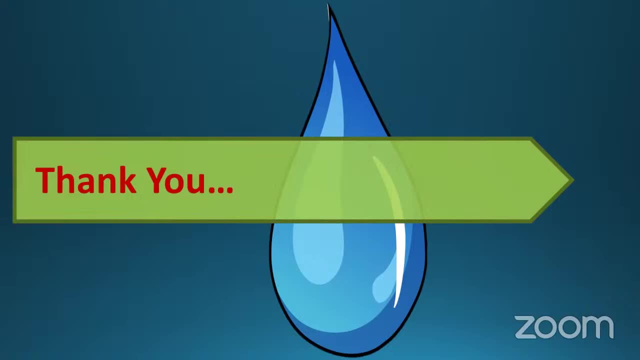 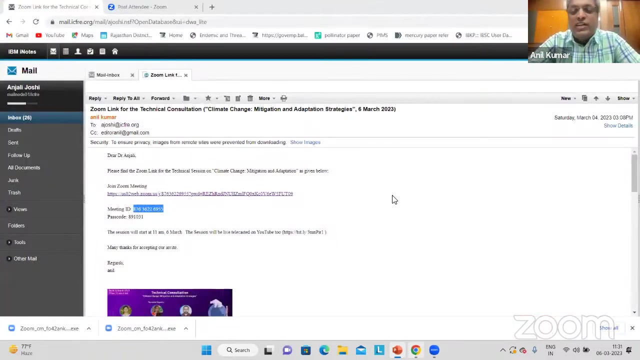 promoted, as well as interventions must be done in order to identify certain other varieties for certain other areas in which such sort of stress is like common. So that is all from my side. Thank you so much for your patience hearing. Many thanks, Dr Anjali. It has been a very detailed scientific analysis with the data. 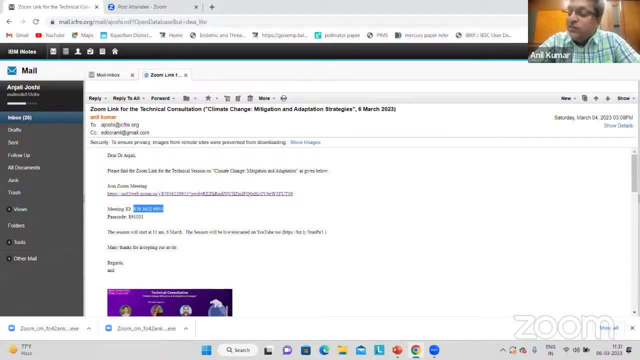 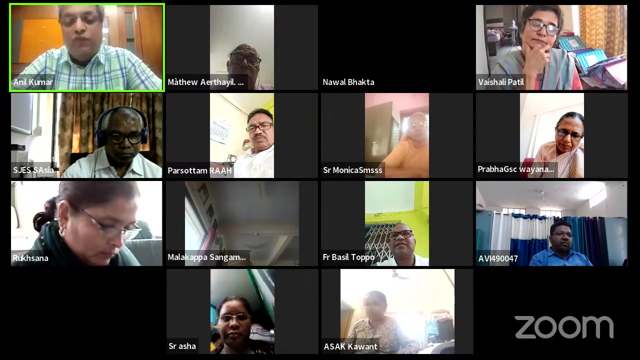 crunching on the impact of climate change, especially in the context of rainfall, how it impacts food production. You have shared a detailed list of climate resilient food crops which can be taken up, Friends. we will be sharing the presentation by Dr Anjali and we will also have a Q&A after presentation by all the thematic experts. 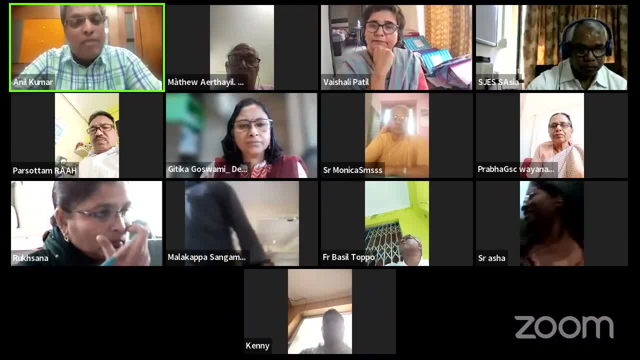 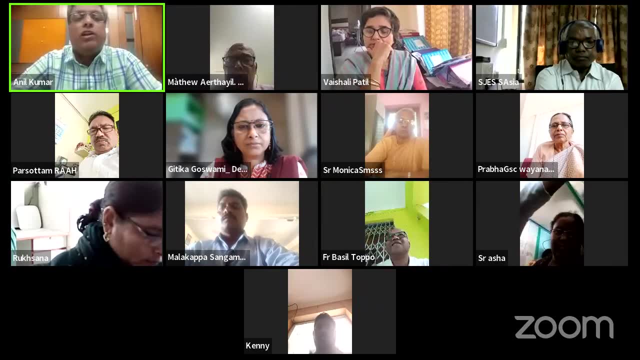 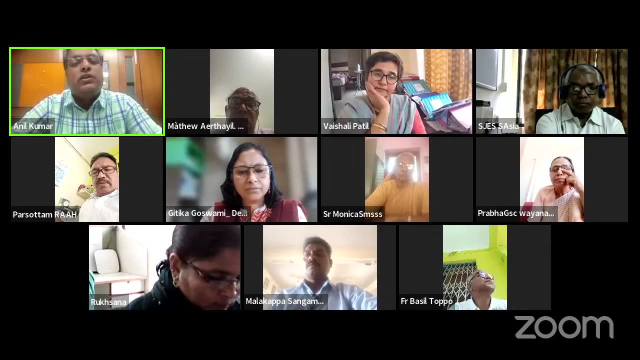 Now let me invite Gidhiga Goswami, who is the Associate Vice President and Lead Policy Research and Planning at the Development Alternatives New Delhi. With more than two decades in the environment and development sector, Gidhiga has been leading the policy and planning domain. 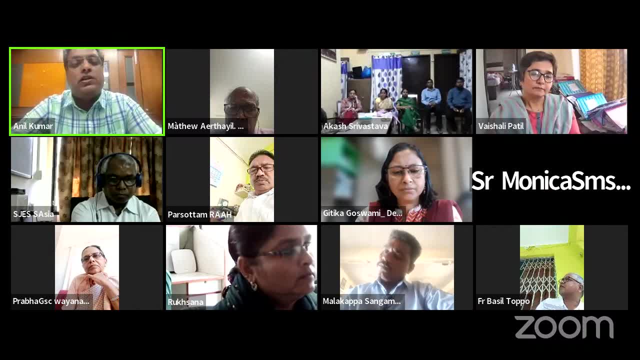 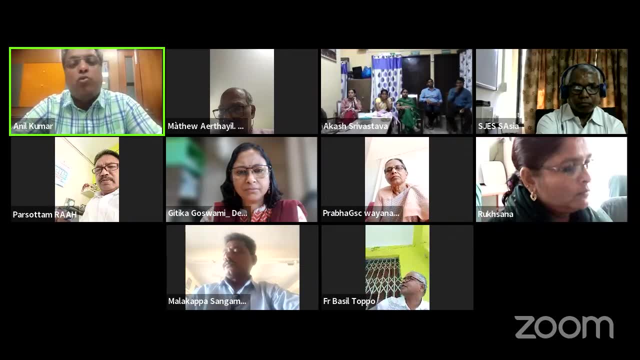 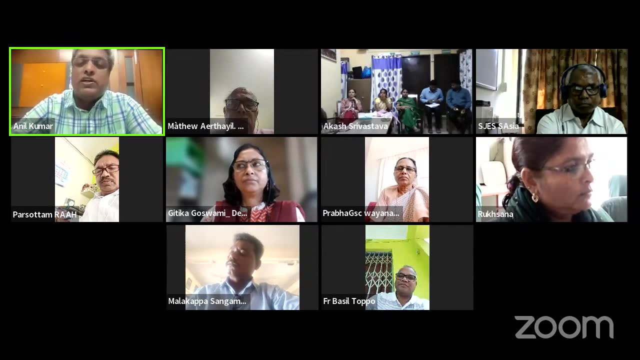 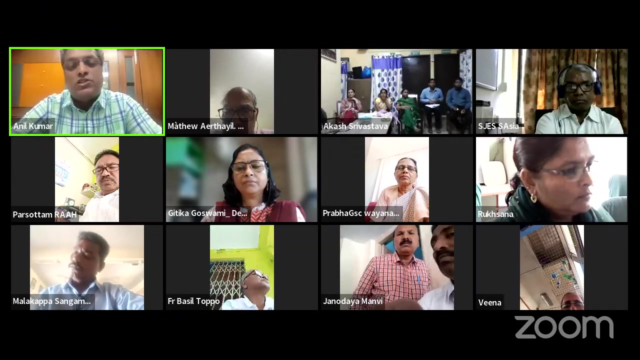 covering verticals like climate change resilience, inclusive development, sustainable consumption and mandate to influence and support public policy towards sustainable development. GIDGA has been associated with several national and international fora, including the various UN forums and processes: the COP process. 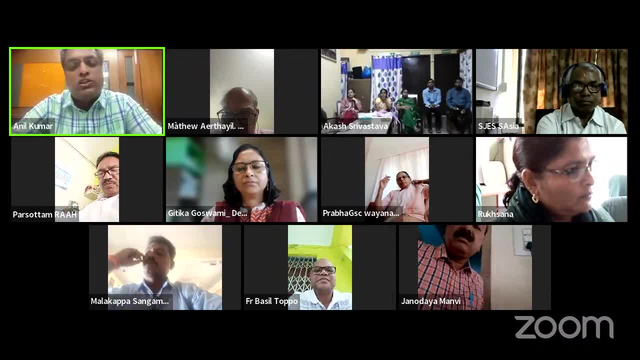 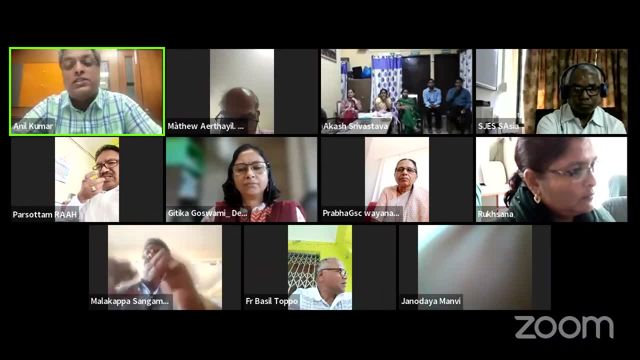 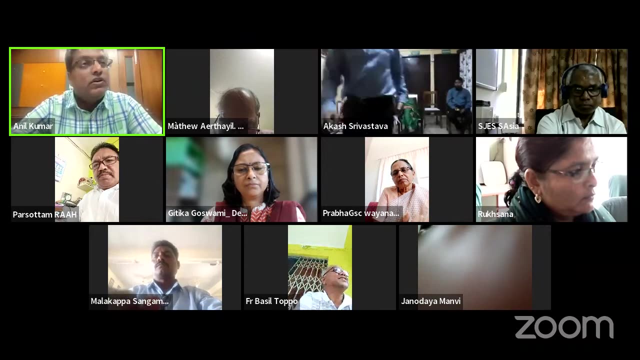 UN framework for climate change adaptation fund board, born natural capital working group under green growth knowledge platform at Washington and Paris, and many others. She has worked with the Ministry of Environment, Forestry and Climate Change, UNDP and many others. It is a great. 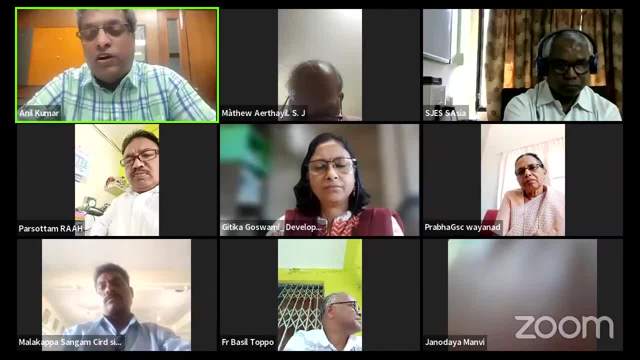 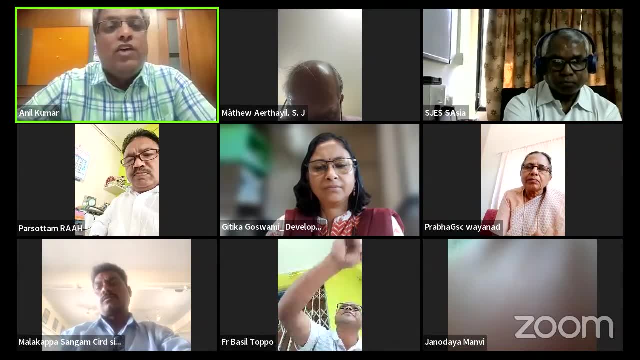 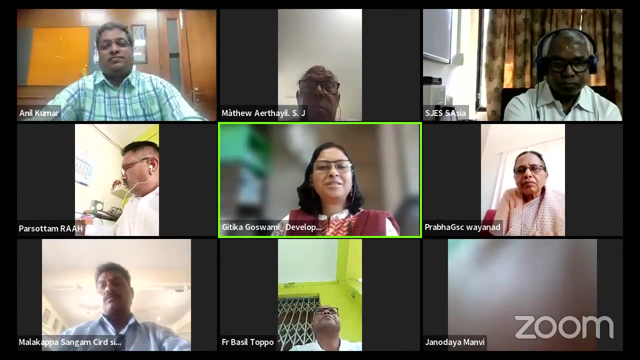 privilege to have GIDGA today and, for the information, GIDGA is also involved with the present G20 processes. also, Welcome GIDGA. the floor is yours, Thank you. Thank you, Mr Anil, and it's really a great privilege to be here. 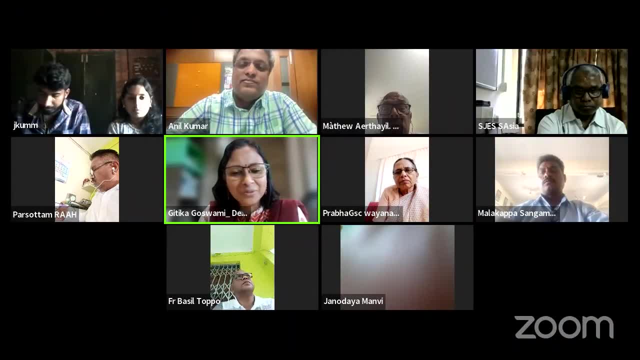 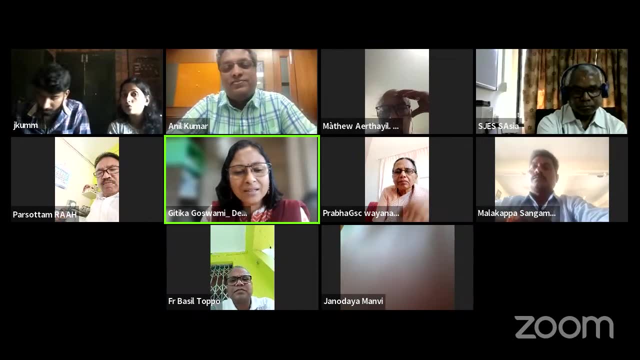 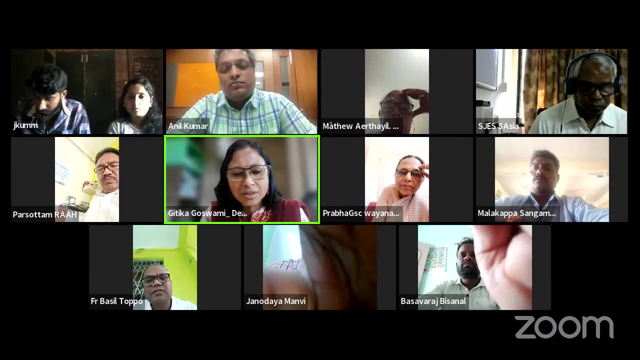 and present the work of Development Alternative in this fora, and I'm really happy to see there's 98 participants, and so from my presentation I will share Development Alternative's work in the adaptation and mitigation sector. Anil, I think there is- I get a. 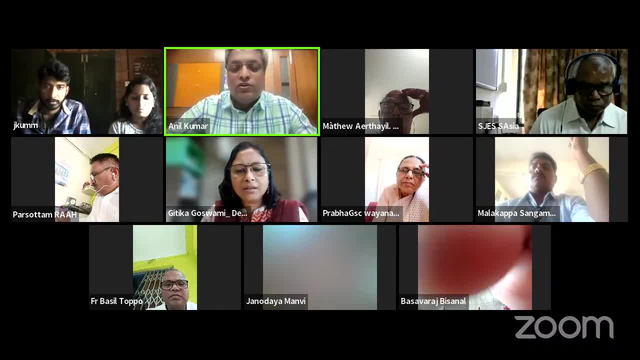 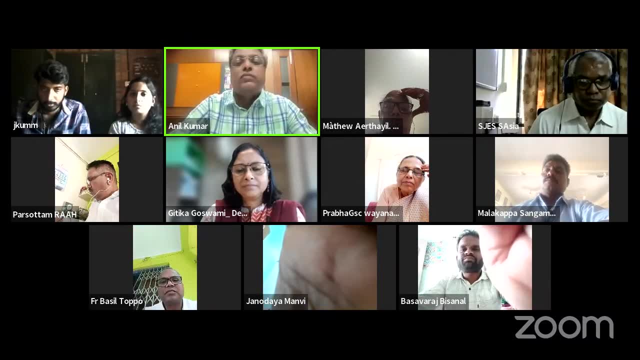 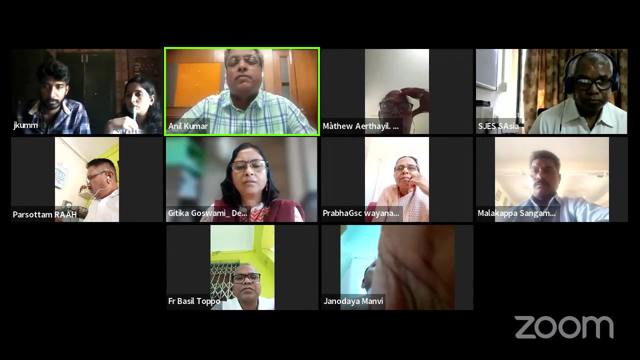 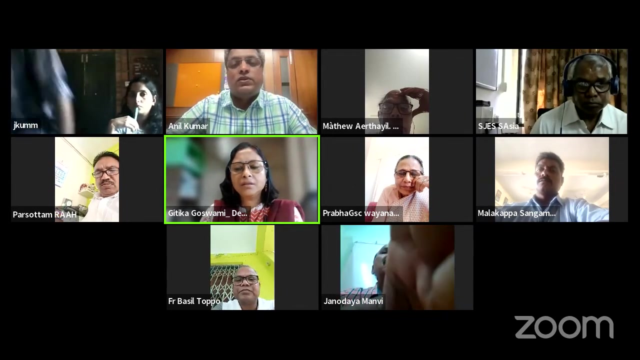 I cannot share. I think the other, Yes, can the other. You are the co-host? Yeah, You are the co-host, But here I can see one participant can share at a time. Is it that the other other presentations still on? 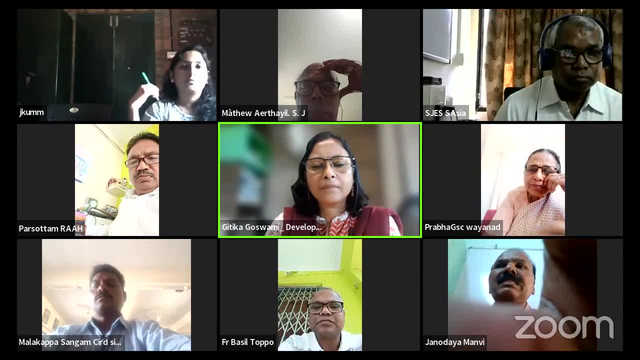 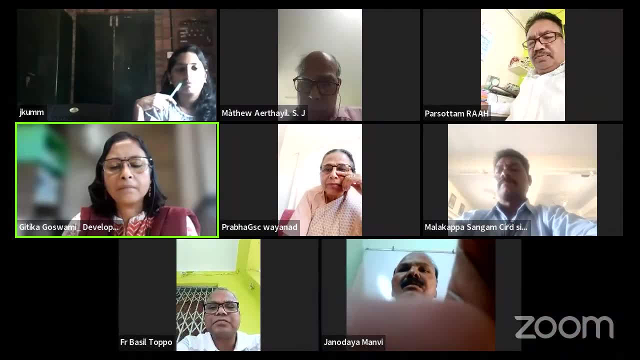 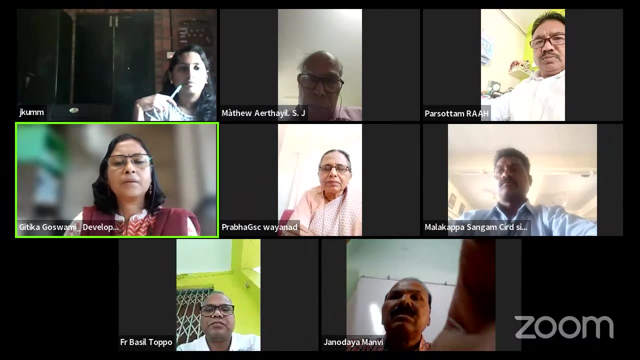 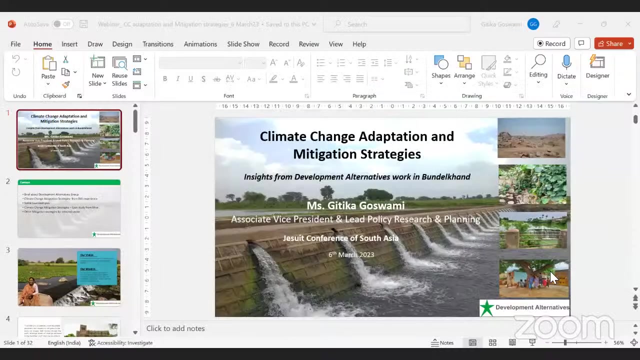 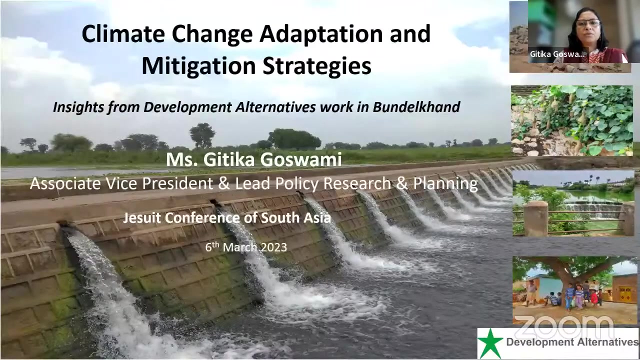 Can you see my screen? Yes, yes, it's visible. Okay, okay, great, Thank you, Thank you. Thank you, Yeah, Thank you, Yeah, So just a minute. So my presentation is all about the climate change adaptation. 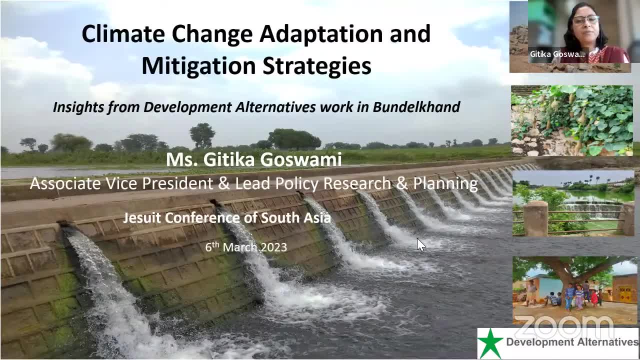 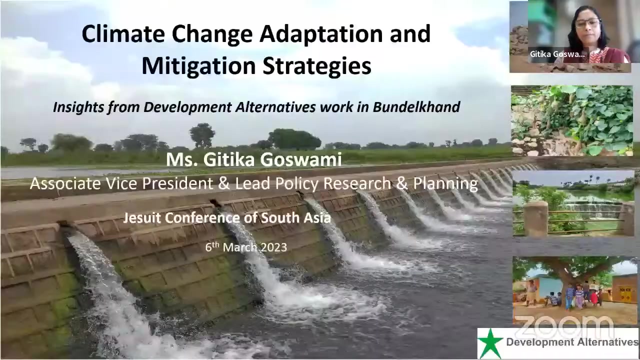 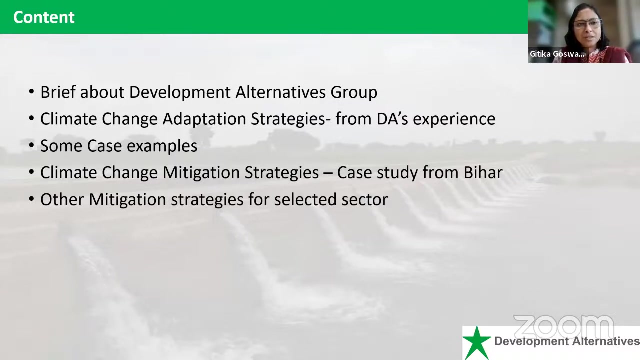 and mitigation strategies: insights from Development Alternative's work in Bundelkhand, especially for the adaptation part and mitigation. I will talk about the other work and other sectors where we are working. i don't know, it's not moving. yeah, yes, the content. yeah, as the so. this is the brief structure of this presentation. 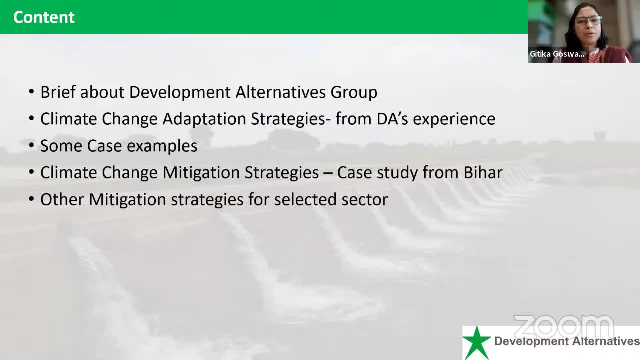 first, before i start on the adaptation part, let's just very briefly talk about develop, about the group development alternative group, then the climate change adaptation strategies from ds experience- some case examples. and then climate change mitigation strategies- case studies from uh, bihar and other states and mitigation strategies uh- some selected mitigation sectors. 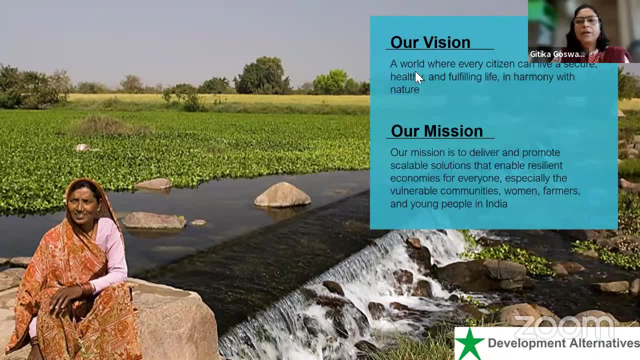 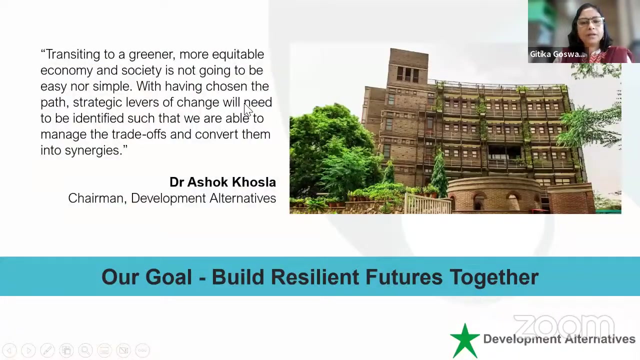 uh, so development alternative. our vision is a world where every citizen can leave a secure health and fulfilling life in harmony with nature. our mission is to deliver and promote scalable solutions that enable resilient economies for everyone, especially the vulnerable communities, women, farmers and youth. our goal is build resilient future together. this is the journey so far. 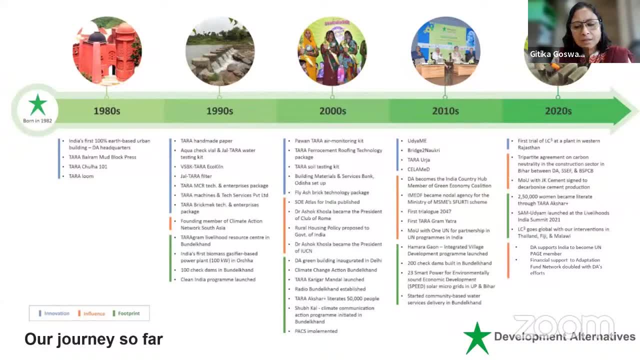 so we started at 1980. um, after that, in the year of 2020, we were good and we completed the month. uh 2022, we just completed 40th year. we just- uh, you know, celebrated our 40th anniversary. so this is the decade wise uh, mean uh outcome of. 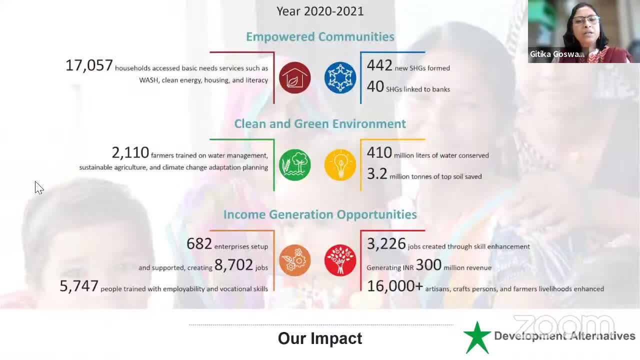 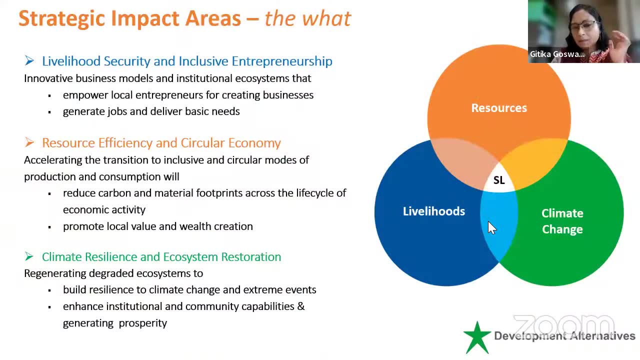 the work. i am not going in detail, but i will share the presentation. you can have a look. this is the impact area. so we work in a clean and green environment. we work in empowering communities. we work in income generation opportunities. so these are. these numbers are with me. 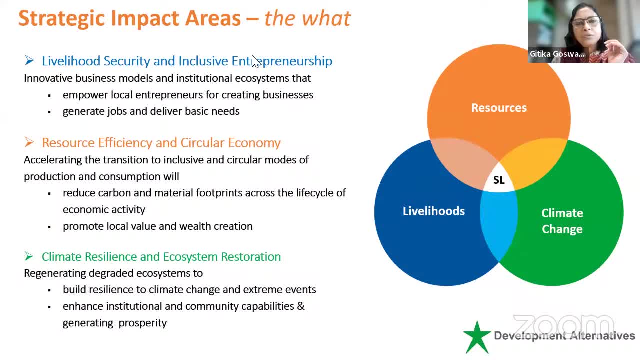 especially the impact numbers. now, coming to our what we do, you know- strategic impact areas. we, as everybody knows, you know- I think our previous speakers already mentioned- that currently we are going through a very, you know, challenging environment. we are having three main challenges that the humanity is facing. one is the lack of resources, lack of livelihoods. 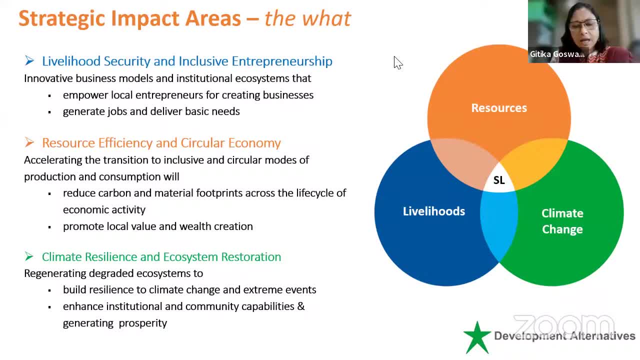 and climate change. these three to address all these three challenges. and to to develop a climate adaptive solutions for livelihoods. and to and to address the lack of resources. we work at length on the sustainable livelihood and on this level, livelihood basically falls under the the three impact areas. so the first challenges that 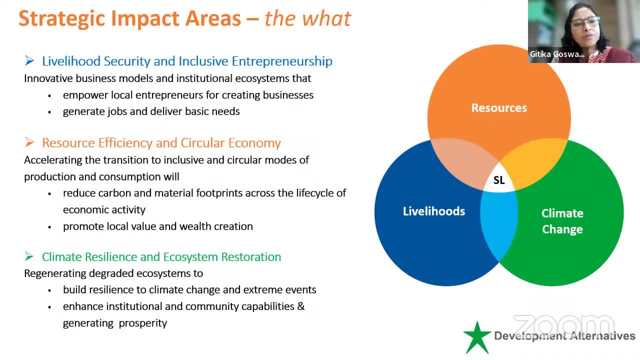 we we are addressing the livelihood challenges. that we are addressing through empowering local entrepreneurs for creating business, generating jobs and deliver basically. the second challenge is the resource challenge, the lack of resources. so how we are addressing here. we are working on resource efficiency and circular economy. we are accelerating the transition to inclusive and 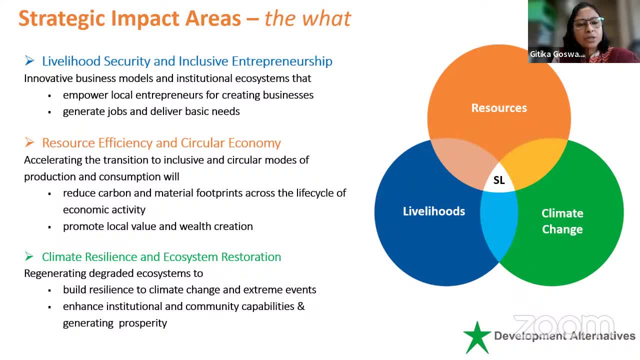 sustainable livelihoods. we are also working on the development of a model of production and consumption which can reduce carbon emission and material footprint across the life cycle, which can also promote local value and wealth creation. we are also the another most important parties that climate change, which is, as this is, the forum or discussing climate change we are 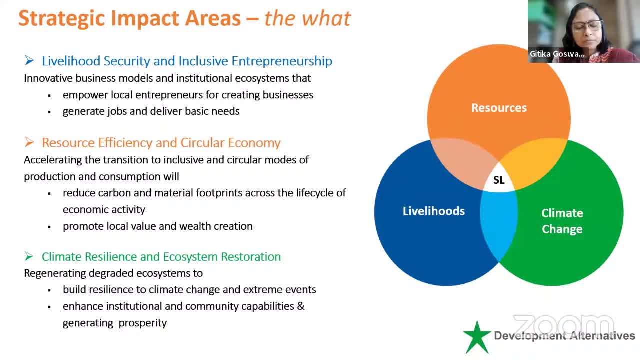 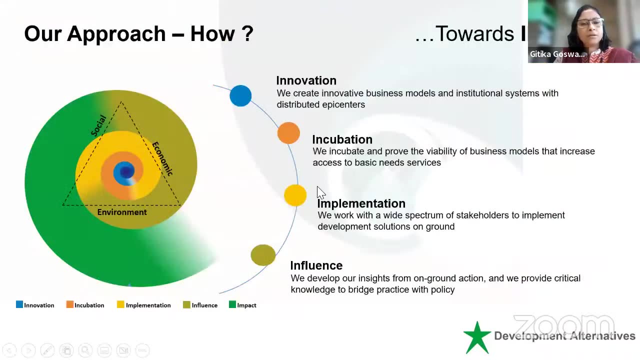 working on climate resilience and ecosystem restoration, where we are trying to generate degraded ecosystem, to build resilience to climate change and extreme events and enhance institutional and community capabilities and generating prosperity now. so this is, uh, the approach that we have taken so far. innovation at any innovation could be in a 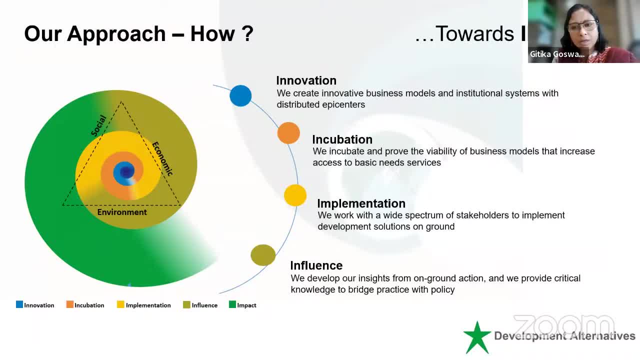 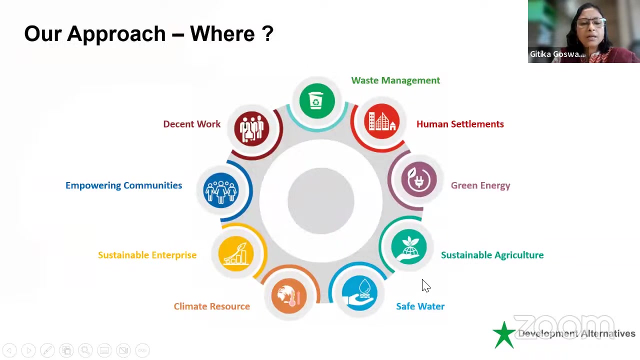 business model could be in the secondary resources. this type of innovation we are also. we are also working on incubation, implementation and influence, and influence through policy and advocacy. these are the settlement: green energy, sustainable agriculture, safe water, climate resources, sustainable enterprise, empowering communities and dissenting work. 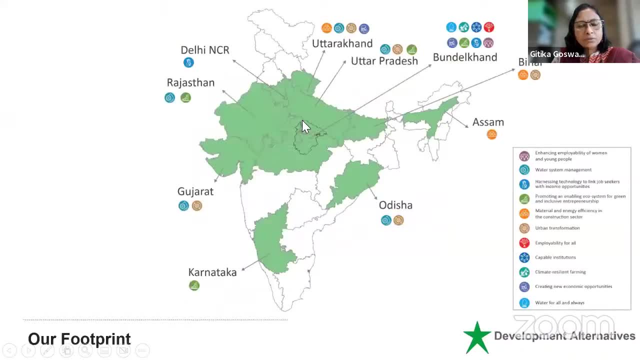 these are our footprint in india, so mainly the they'll create the infrastructure for the local. you can see, this is the area in the central part of India. It's called Budelkhand, 7 districts of MP. We started working in Budelkhand three decades before and we are working. 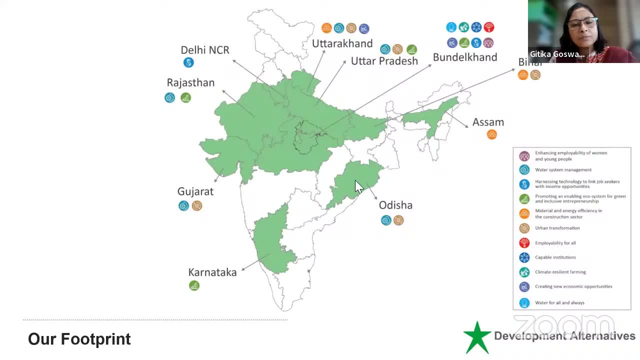 with the communities directly here, in other areas which you can see- the Orissa, Karnataka and Gujarat, Rajasthan, UP, Bihar- Our presence is there but we are working with the partners, So also a global footprint. We are mainly in the south of India. 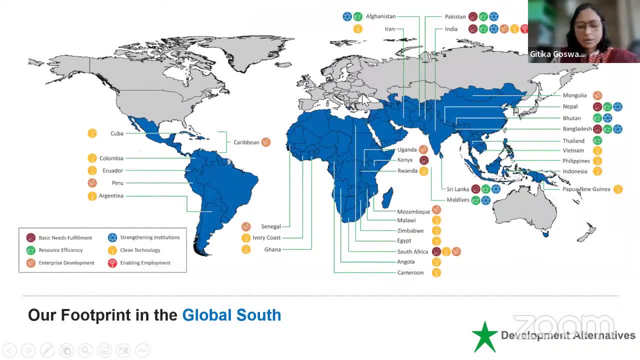 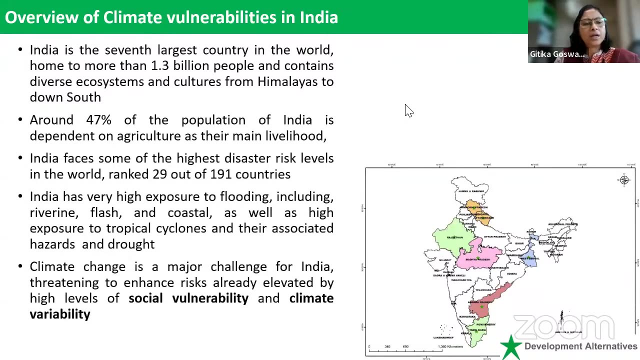 So now coming to the main part of India. So, as I think Anil has already mentioned about, what are the climate vulnerabilities in India? India is the 7th large country in the world, home to more than 1.3 billion people, and contains diverse ecosystem and culture, from Himalayas to down south. 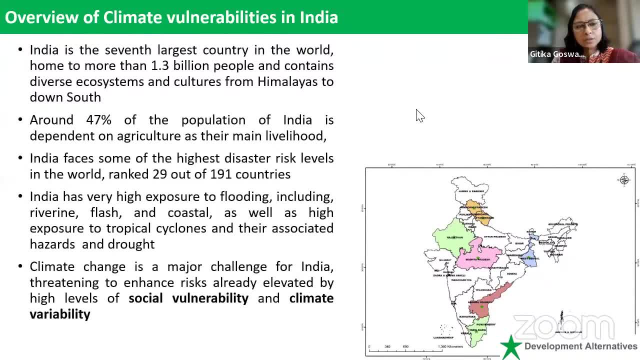 Around 47% of the population of India is dependent on agriculture as their main livelihood, And India faces some of the highest disaster risk levels in the world. India is a rancher. India has managed 29 out of 191 countries in terms of disaster. 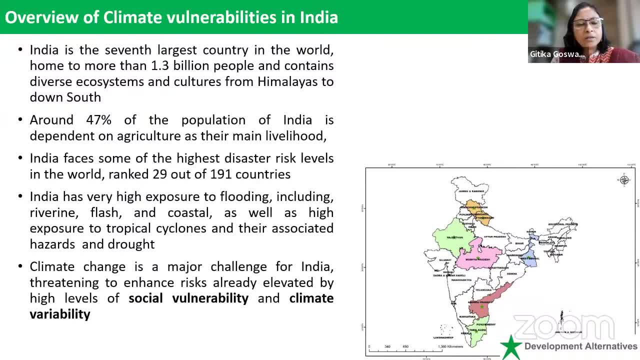 India has very high exposure to flooding, including riverine flood, flash flood and coastal flood, as well as high exposure to tropical cyclone and their associated hazards and drought. Climate change is a major challenge for India, threatening to enhance risk already alleviated by the high level of social vulnerability and climate vulnerability. 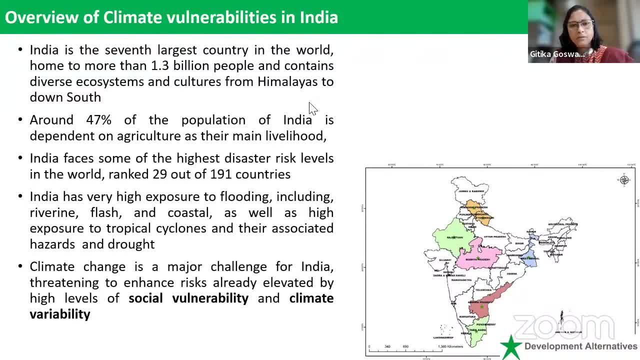 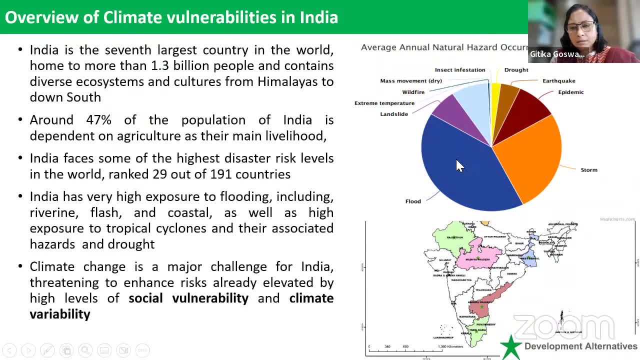 This is. This is, you can see in the pie chart, the maximum hazard and we face is a flood, almost 45%. Then this is strong And this storm is mainly because of this We have this huge, you know, maximum length of the coastal belt. 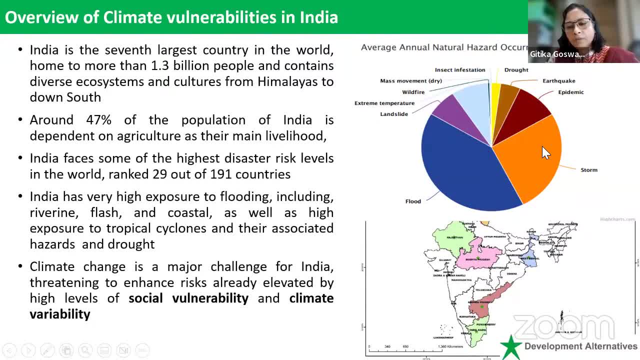 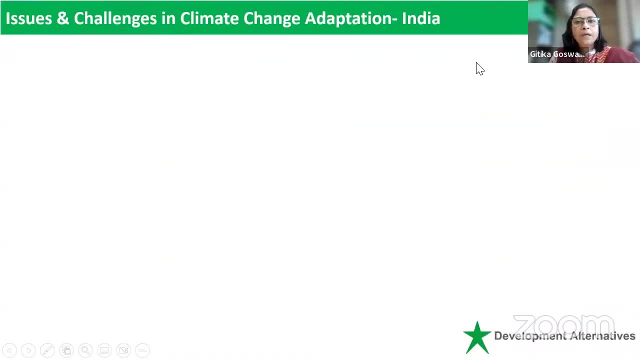 And we we have a lot of cyclone there And it's also around 35% And just you can see extreme temperature by life loss, drought, earthquake and epidemics. Now coming to the issues, you know issues and challenges that climate change adaptation challenges climate change adaptation in India. 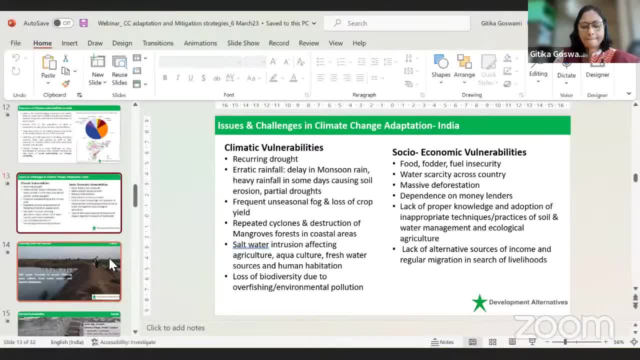 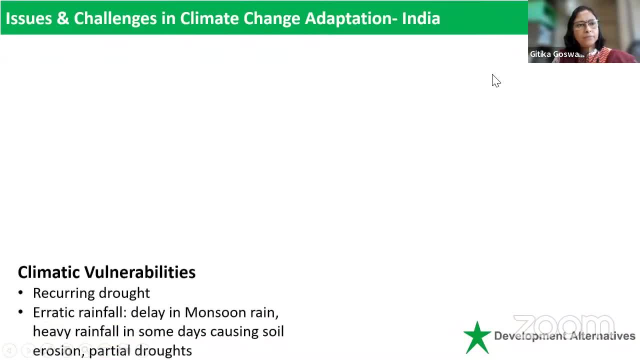 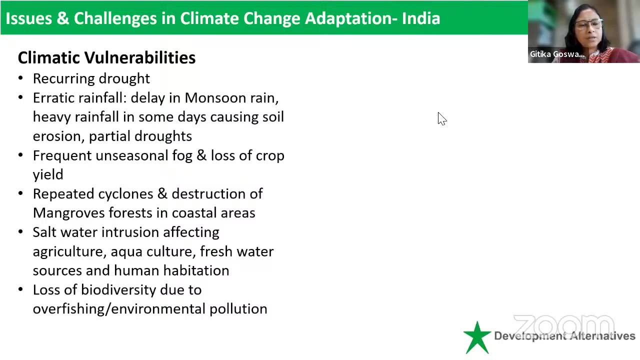 Sorry, Okay, Thank you. These are the different challenges of climate vulnerabilities: Basically the recurring drought, Recalling drought, Genetic rainfall, Delay in monsoon rain, Heavy rainfall in some days causing soil erosion and partial drought, Frequent unseasonal fog and loss of crop yield. 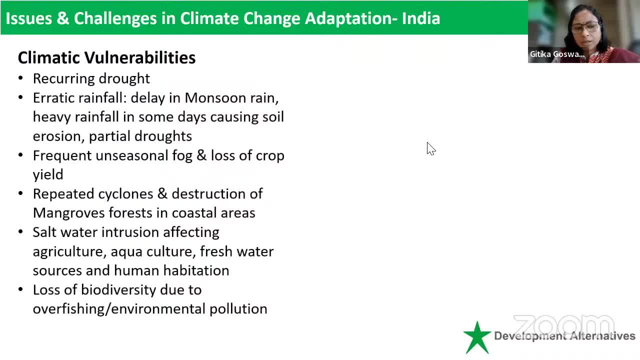 Repeated cyclone and destruction of mangroves in the coastal areas. Saltwater inundation and affecting the agriculture, aquaculture, freshwater resources and human habitation. Loss of biodiversity due to overfishing and or environmental pollutions. Socio-economic vulnerabilities. 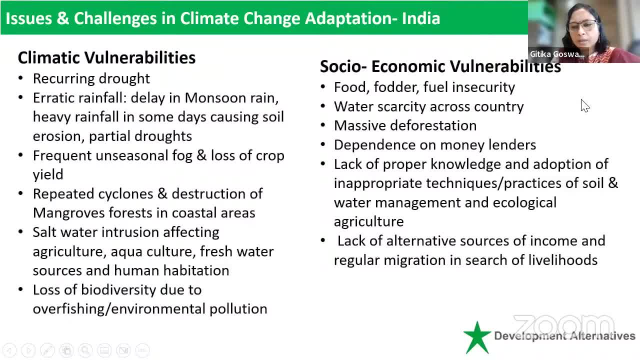 Due to these climatic vulnerabilities, there are huge socio-economic vulnerabilities that are very much visible here: Food fodder and fuel insecurity, water scarcity across countries, massive deforestation, dependency on the moneylender, a lot of migration, lack of proper knowledge and adoption of inappropriate 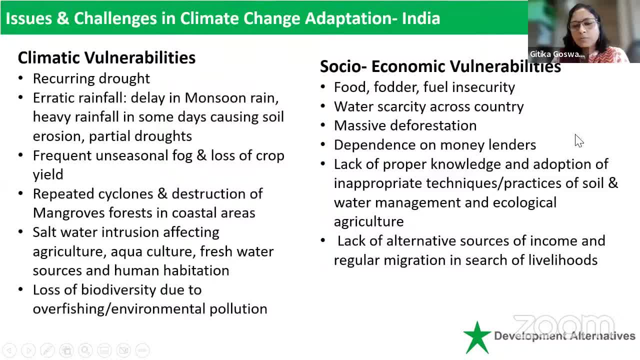 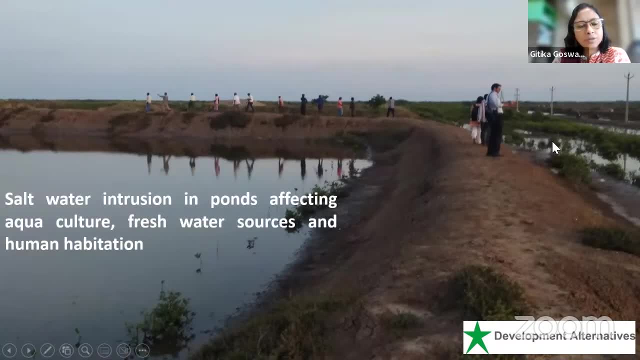 technologies and practices of soil and waste water management, ecological agriculture and lack of alternative sources of income. These are the socio-economic vulnerabilities. With this I am just saying. I will show some of these. What is the ground voice? This is in south, down south. there the main problem, the coastal areas- is the saltwater. 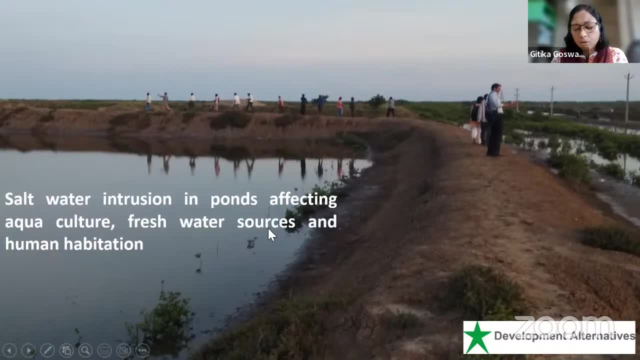 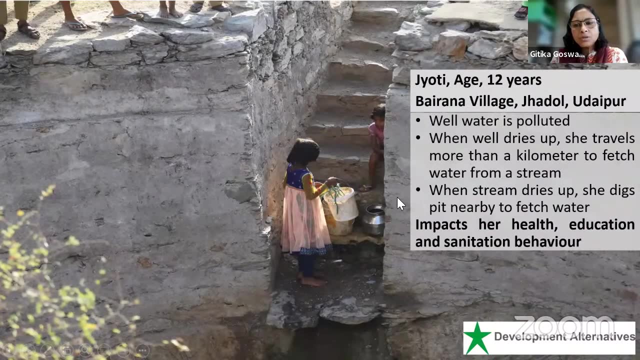 intrusion in the pond, affecting the aquaculture which is the main livelihood of these communities. Then this is from Rajasthan. this is a small girl, Jyoti. What she says, her testimonial, is that well, water is polluted when it dries up. she travels. 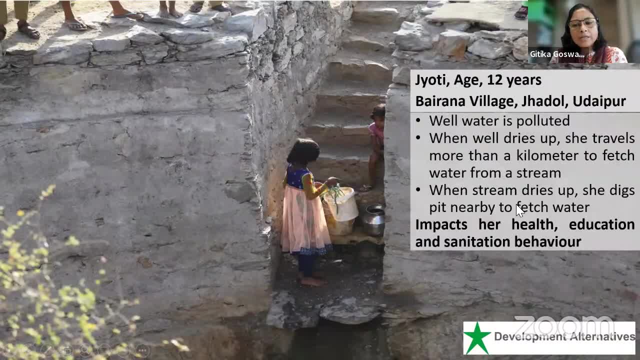 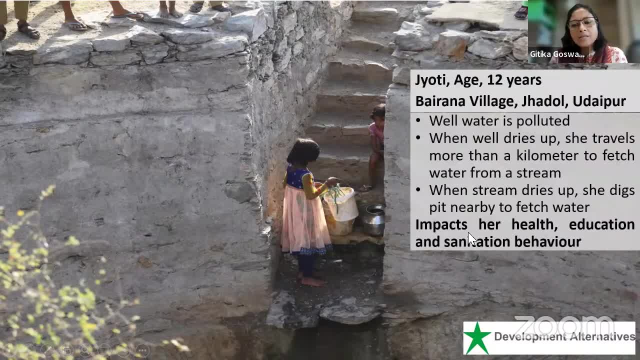 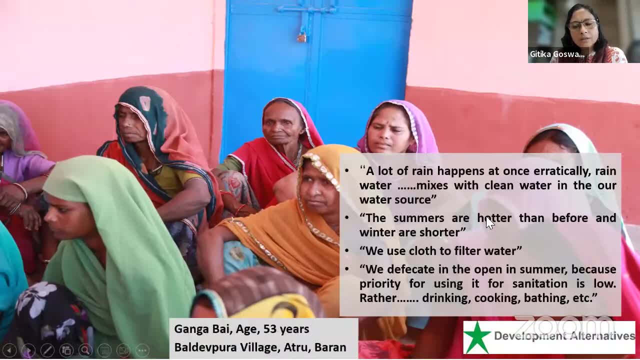 When the stream dries up, she digs pit nearby to fetch water, And that impacts our health, education and sanitation behavior. And when you know, as we all know, in India, when there is a scarcity of water and then 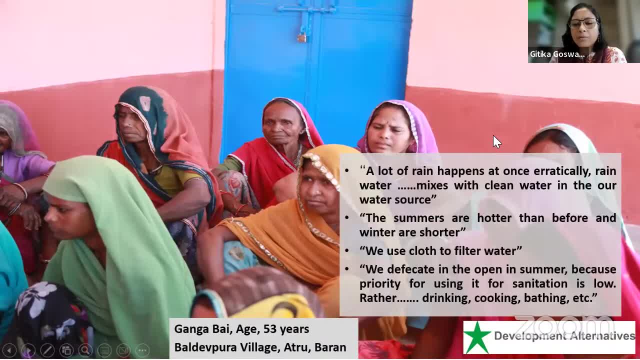 the girls and the women are mainly responsible for each of the families to fetch water and most of the cases it happens that the girls actually miss their schools. Here, these communities are women, members of these people, of the families, families in rajasthan. they are saying that the summer are hotter than before and winter are 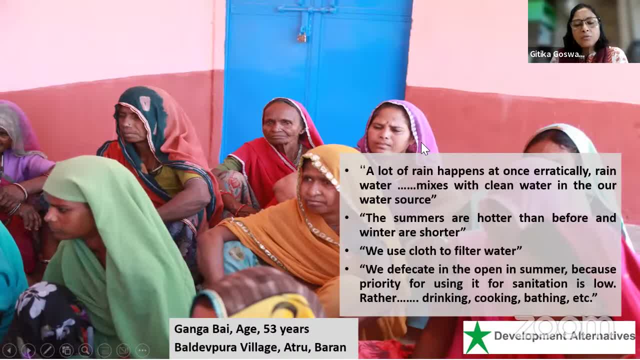 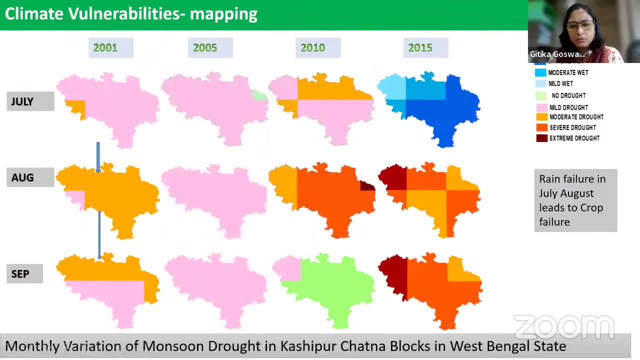 shorter. we use clothes to filter the water. a lot of the water is also polluted there and their- you know- sanitation problem, they are saying because they don't have a safe sanitation- then if we now just looking at these problems, if we do a kind of a mapping and of the monthly 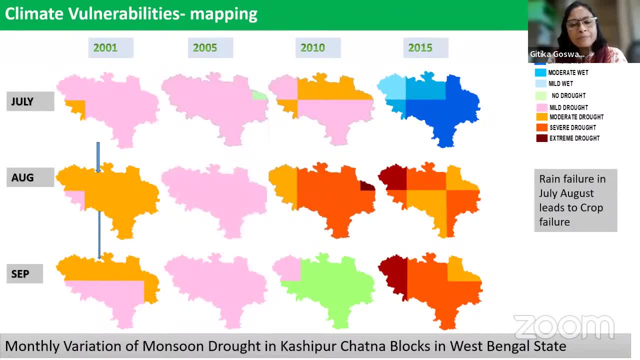 drought. i can give one example from the west ring or where you can see the same district. you can see in the month of july, august and september. you can see in the right side there is this legend where it even in july sometimes the rainfall is very huge, extreme wet. the southern 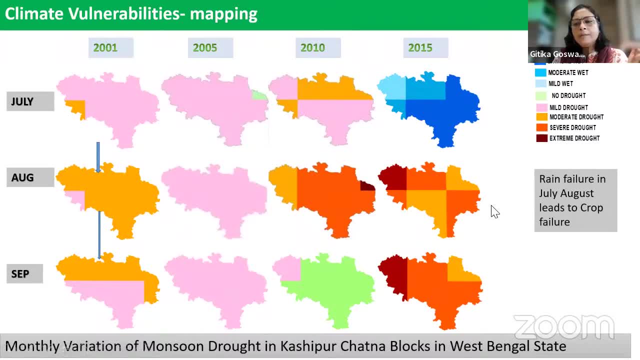 part of this district, but in august you could see that there is also a drought and in september the partial drought. in august and september this is a complete drought. and why this is happening? this is happening because when we have this rain, it's a very huge rain in. 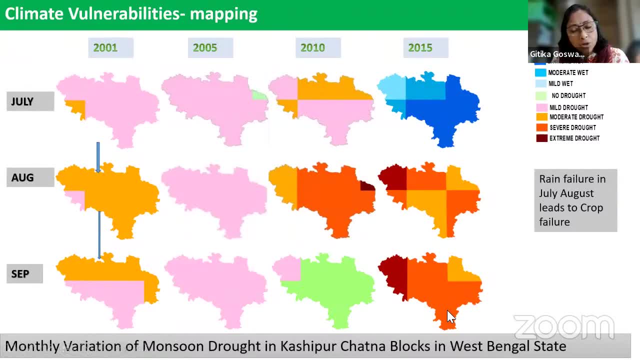 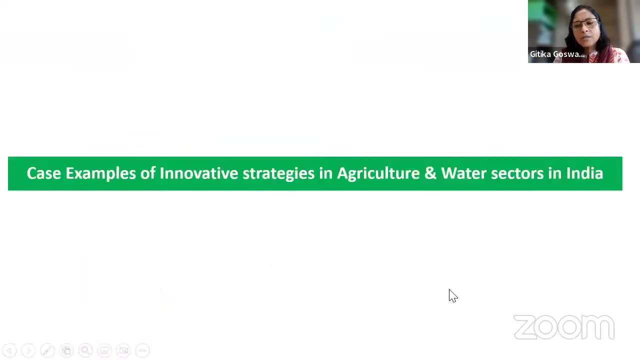 a very short period of time. there are a lot of uh soil, uh erosions happens and then in the two uh two, after two months of these uh rain, this area is completely became a drought brown areas. so this kind of hazards is actually very difficult to really. people have their. 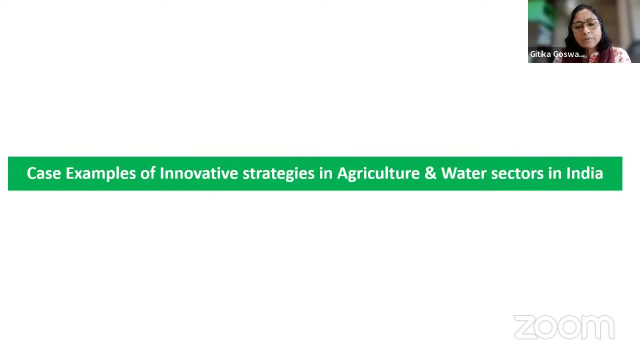 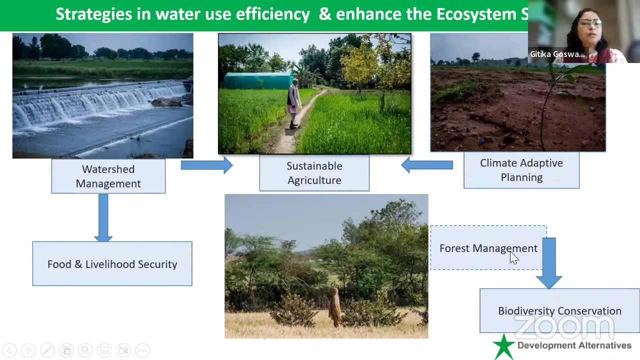 crops or in the field. and so i am here. uh will now come, coming to the areas: where and how, the what are the different strategies that we can take, which how? that's how we can really reduce that hazard and can also get our agriculture crops at the same time. here i uh. you can see, there are uh you know what. 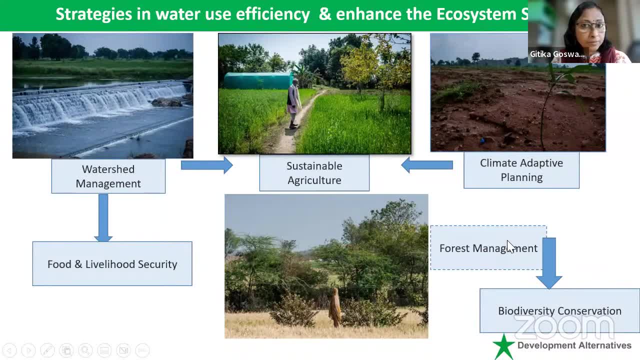 are the different strategies of the uh, of the climate change adaptation. the first thing is mainly in the drought brown areas, watershed management is uh traditionally being uh done and almost in all states we are working on the worst watershed management which can actually help to reduce the sorry. 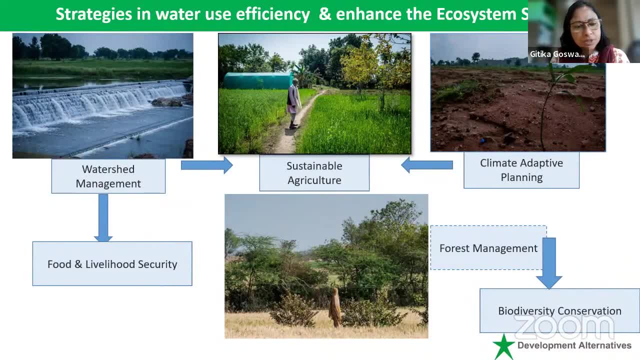 to reduce the rain washing away of the soil moisture and soil erosion, then we are working on, sorry so, under the watershed management also, there are several check dams that's being made, which can we became the water harvesting structures and which can uh benefit, to which uh the water, the groundwater features also happen and because of this soil, 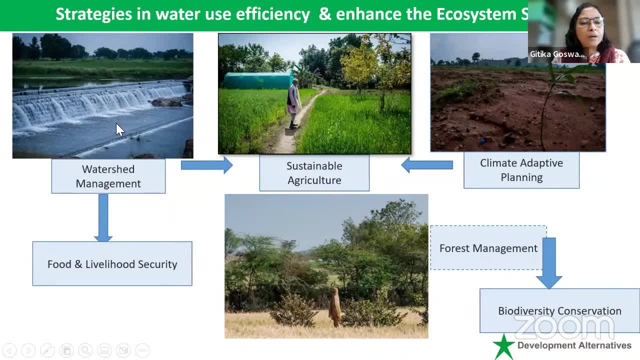 moisture also improves, which helps people to have their second crop. uh, where it is completely impossible, you know, without many of the cases that happen, uh, we can make it through to do this kind of surgicalness if people in this kind of uh water management or second crop uh such a rip off the soil because uh, the, we the or we have to think of a long haul of uh the water, you know, by the uh, the water storage of uh the soil. so we can't, so we can't, um, because of that, uh and uh and uh, uh, but uh, we can't, uh, you know we can't uh, so we can't. 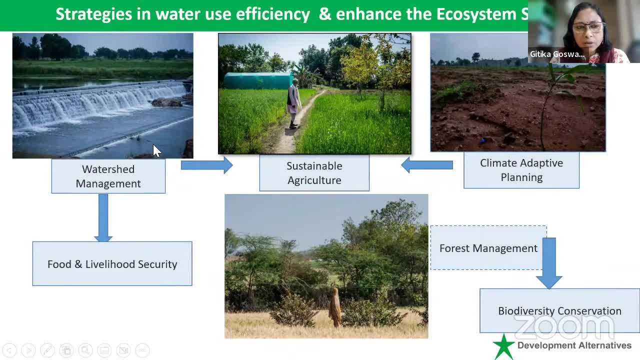 that in drought prone areas people can only take one crop during the monsoon or the curry season, but Ravi. generally they do not, do not get crops. but if you have this watershed management work and if you have your soil moisture till there in the winter season, you can very easily get a Ravi. 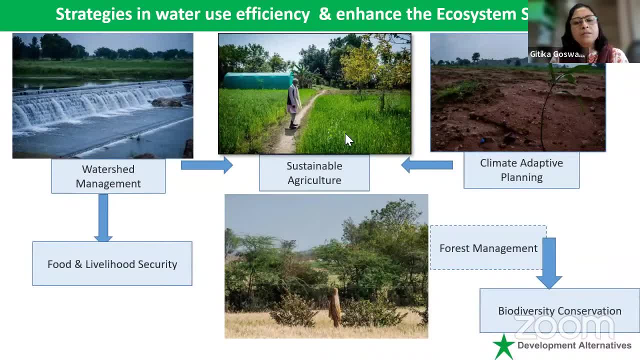 crop as well. This is sustainable agriculture, where we are actually looking at diversifying practices in the same area. we are having a crop as well as the horticulture species, so you can have double income. At the same time, in many places we can also have in the vegetable. 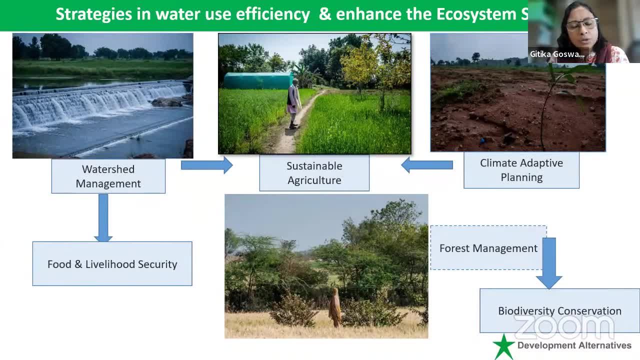 cultivation which can also enable people to not only have their nutrition, also they can sell the excess one- and which can actually give them a better livelihoods, all alternative livelihoods. These are some of these. So climate adaptive planning: that's most important when we have a very, you know, drought prone areas. 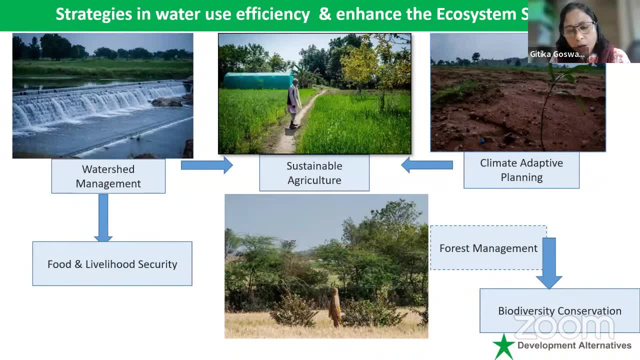 Climate adaptive planning also shows that you know you how you should plan, how much area you should take for a particular crop. which crop you can, you should choose. you know it should not be like water thirsty crop, so rice could be avoided, but we can have millets, we can have other water. 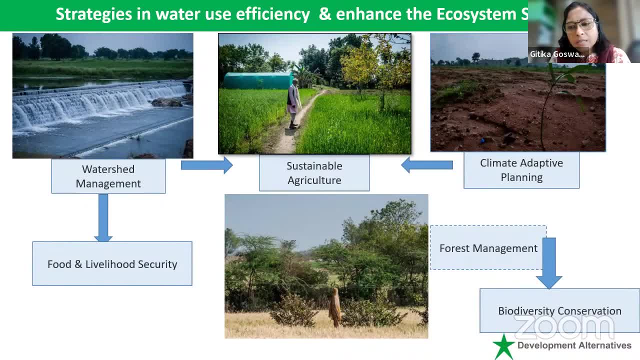 crops, Less water intensive crops as well. so that's the climate adaptive planning and it's it's actually helps a lot for people to have their livelihoods secured. then, at the same time, it's very important to have forest management, which can really result in the biodiversity conservation and when there is, 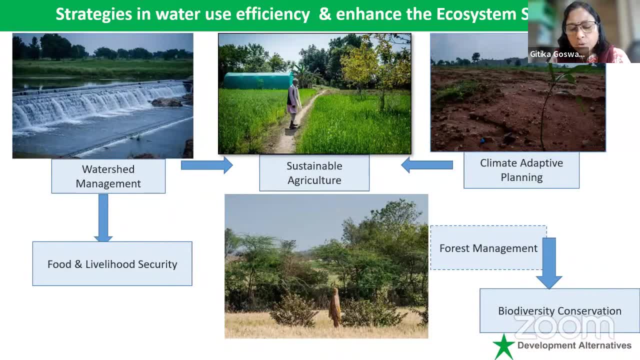 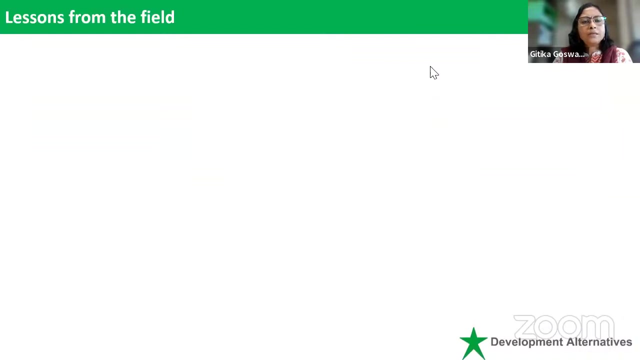 a forest. you know that forest can help you to to have their soil intact and can reduce us soil erosion, even if there is a heavy rainfall. when we have all these, you really should have the food and livelihood security. So now lessons from The field. so I will show some of these examples of how we can really reduce all these. 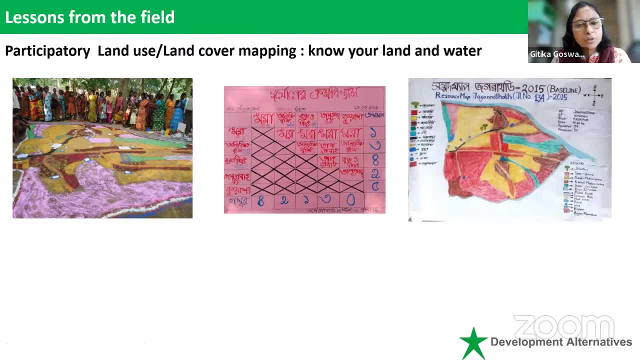 irregularities on. So there is also, along with all These agriculture planning and adaptive planning, we- this example- shows that how can really working with the communities and really, in a drought prone areas, having a maximum livelihood improvement. so this is one thing that we have done. we did. 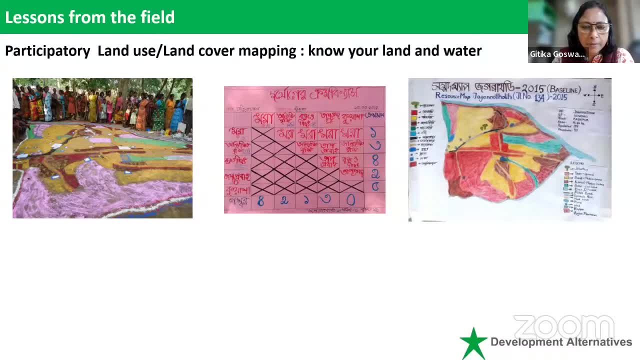 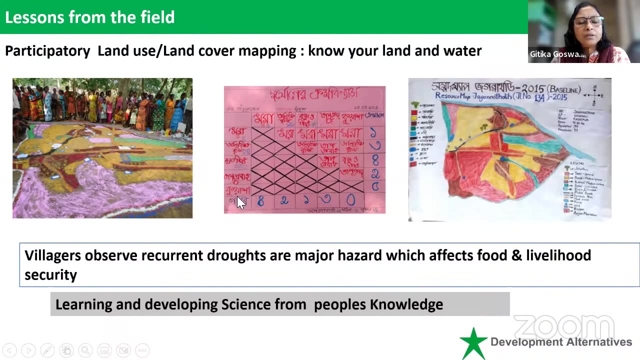 this through a participatory land use and land cover mapping. yeah, and we have helped us, the communities you know to, to map out their vulnerabilities. you know, here this is a local language, they have written it's in Bengali, so here they, in this mattress they have drawn, which is the most important. 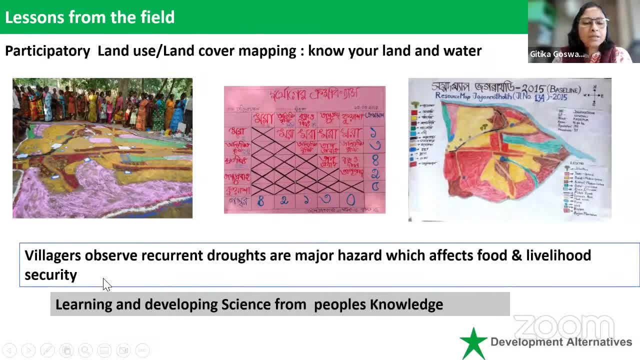 challenges that they faced and through this it has been observed that drought is a major hazard that they have faced and that is why the food and lab use security was a major hazard. so this, through these kind of mapping, we we can really come up with a what exactly the strategies that we should take up in. 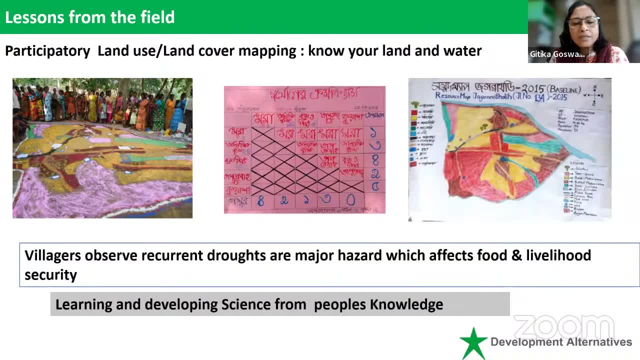 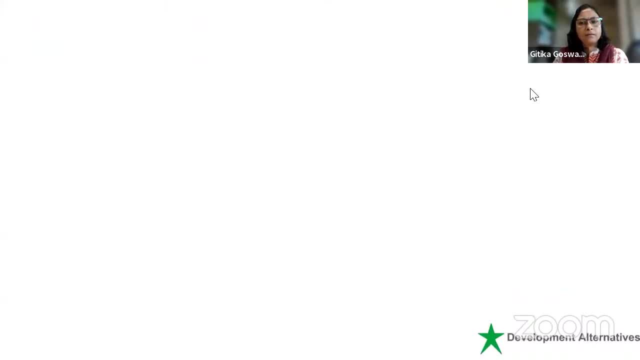 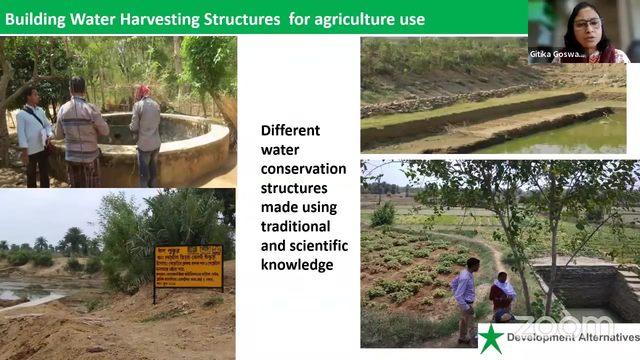 what condition this shows, the learning and developing science from people's knowledge. okay, any other questions? so these are some of the water harvesting structures成ime that was built to address those kind of droughtplessness challenges. so here you can see the well people in a newxa. 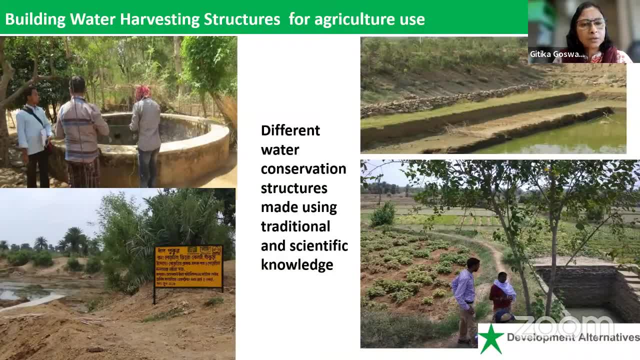 but this is the well with of the democrats blue worth scotland s-way through that particular data, or this is a project as it was sketched outside. the first one is the left side is a well, that's been made. then there is a pond. this is a stay. 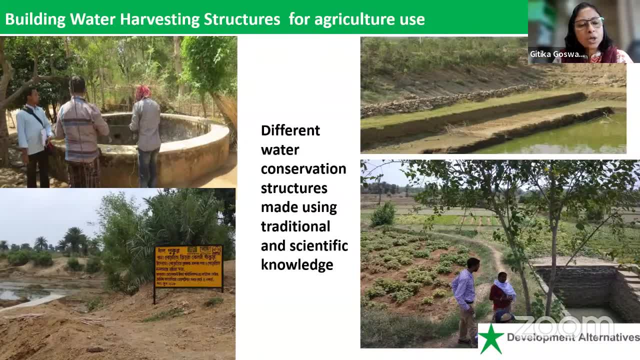 ponds. stay ponds actually helps people to have water whenever. i mean as much as possible. if you have a stay pond, the your area of exposure to the sunlight of the pond will reduce and then the also the transportation also reduced. so even if you know, in the hottest time still there is. 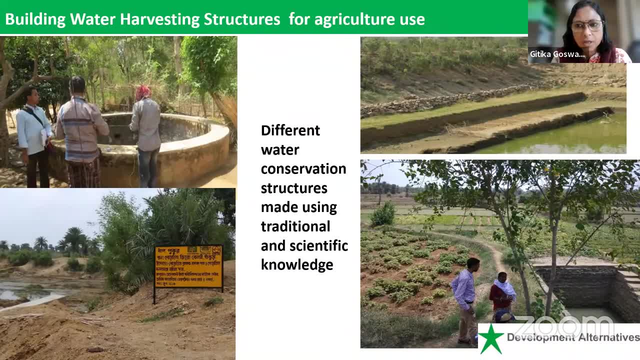 some water that's uh, that's available there in those spots. then you have here in the right hand corner, you can see, this is called hapa. this is also in the undulating areas like bakura purulia, and we have, uh, this, uh, it's called horizontal seepage and if you really uh. 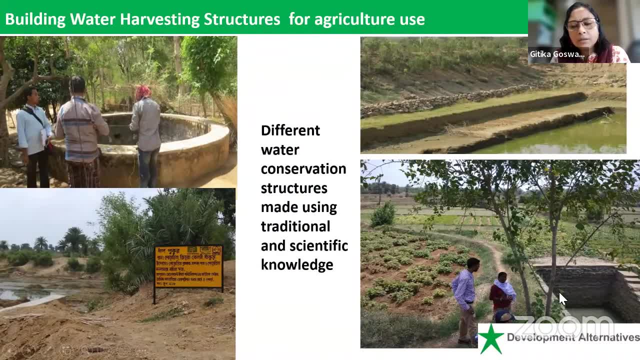 dug a small pitch. you can see that uh in the in the night, this sorry, so you can see uh that the water gets accumulated during the night time and then people can irrigate the water in the morning. and again this: if you completely pumped out this water from these small uh water harvesting structure, evening also, again it's filled up. 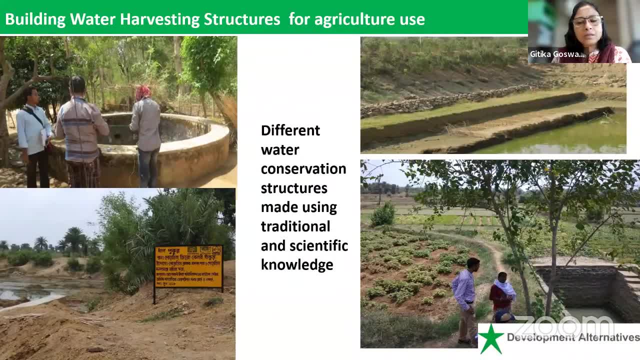 and you can have another irrigation in the evening. so it's something a very traditional knowledge, but it's a very traditional knowledge and it's a very traditional knowledge and it's- but we have made it a little scientific, make this uh peat little more, uh deeper, so that more. 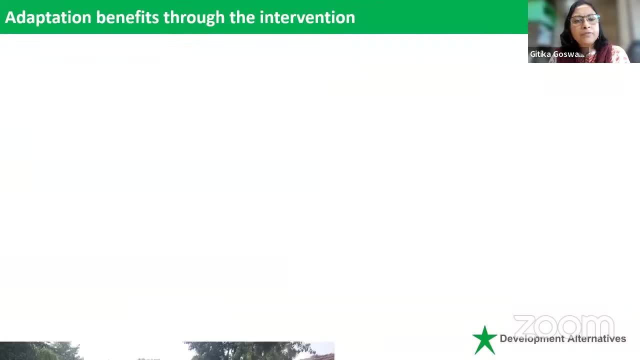 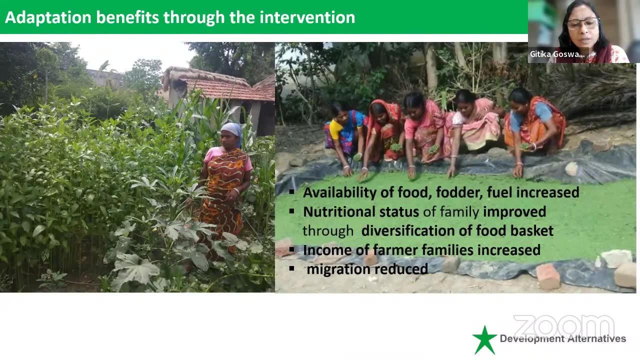 water can be accumulated. you have adaptation benefits through these interventions. these women- they're from their uh word. they have said that this- because of these auto harvesting structures they get. they get several types of the alternative cropping practices and that's why they're available to food fodder and fearless in the 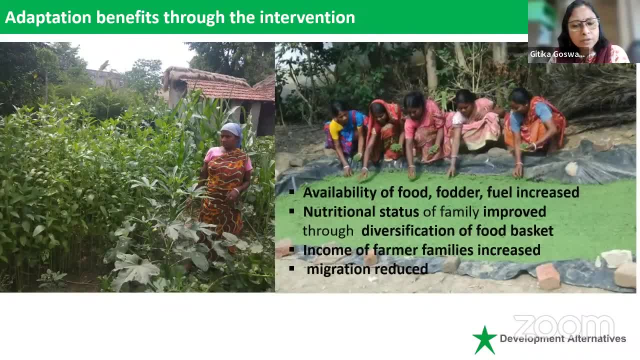 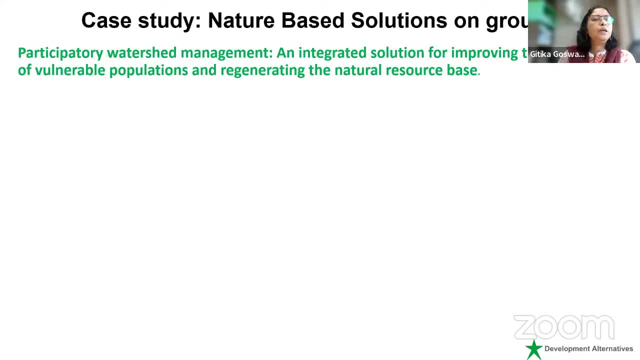 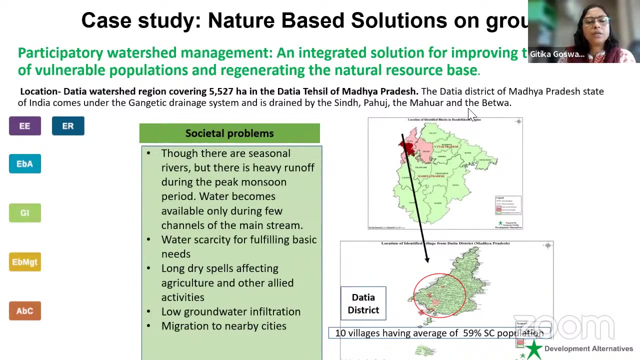 forest, and they also have a lot of other products, such as the uh. i am now uh coming to very briefly talking about in bundelkhand, one case study called nature-based solution. here also we have uh implemented a participatory watershed management and integrated solution for wind from the livelihood of the vulnerable communities. this is the universal. solution for the environment and it is also used in the environment and there is a lot of people who are interested in the environment and the environment is also used in the environment, in which the environment is used as the best way to Наikki, and the environment is used to 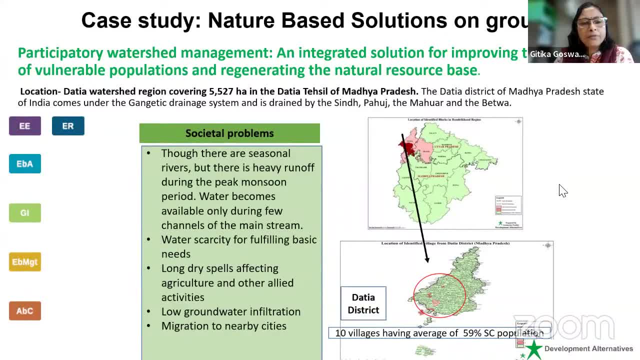 prevent the spread of the weather, so that you can see the area that is the most. a lot of people of the environment is used to create the environment. the environment that is the most unique and the most is a district. it's called Datia, where there was a same societal problem. 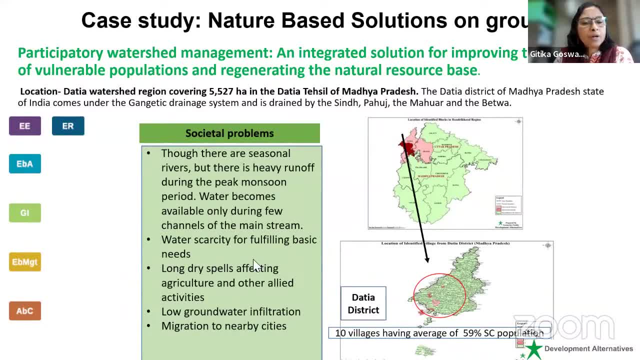 that there was seasonal river, very heavy runoff and the water scarcity and long dry spill and low groundwater infiltration and migration to nearby cities. Here you can see we have taken 10 villages where 59% of the AC population and taking the strategies of the nature-based solutions. 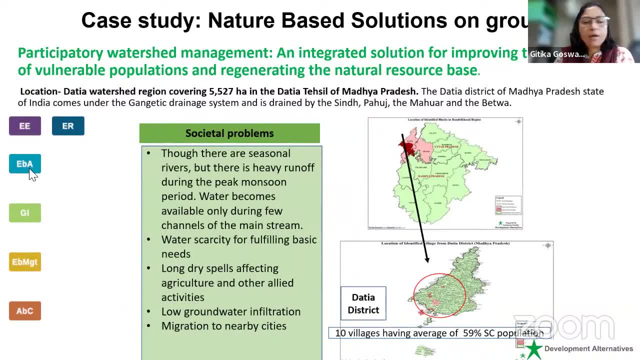 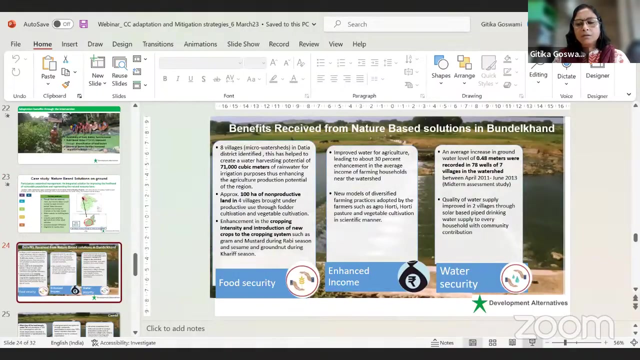 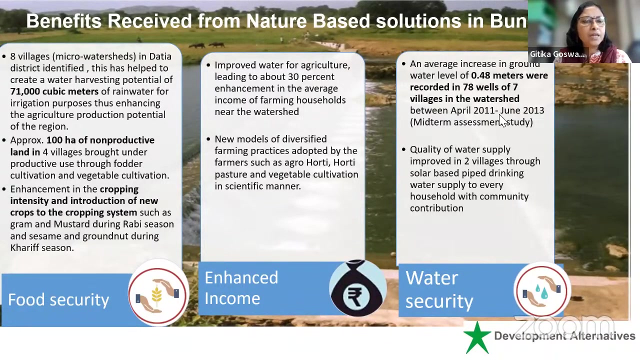 especially the environmental engineering, environment-based, ecosystem-based adaptation, green infrastructure, ecosystem-based management. We come up with this Now using these strategies we have seen. We have seen So benefits of these nature-based solution is that, out of these 10 villages, 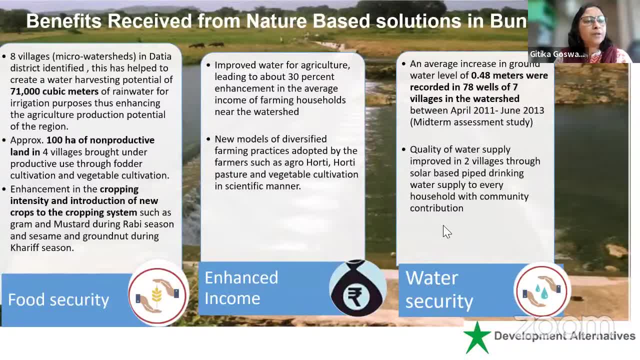 eight villages in Datia district identified this as helped 71,000 cubic meter of rainwater harvesting done. Approximately a hundred hectare of the non-productive land in four villages brought under the productive uses of cultivation of vegetables. enhancement of the cropping intensity. 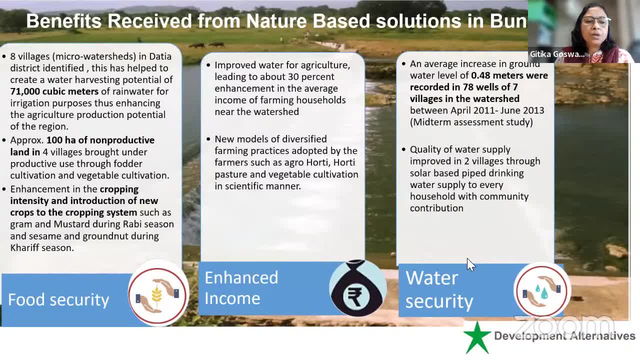 and induction of the new crop to the cropping system So that helps the food security. Then also that since the improved water for agriculture leading to about 30% enhancement of their average income of the farmer household, which also through these NBS new model. 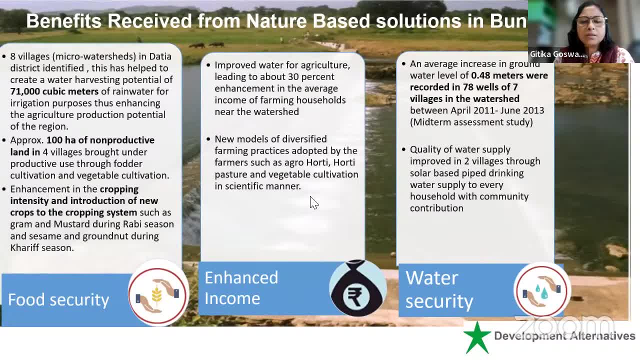 of diversified farming practices adopted by the farmers, such as agriculture, horticulture, horticulture, vegetable cultivation in a very scientific manner. It's also water security when built, because you have 0.48 meters where they got it, the rainfall. 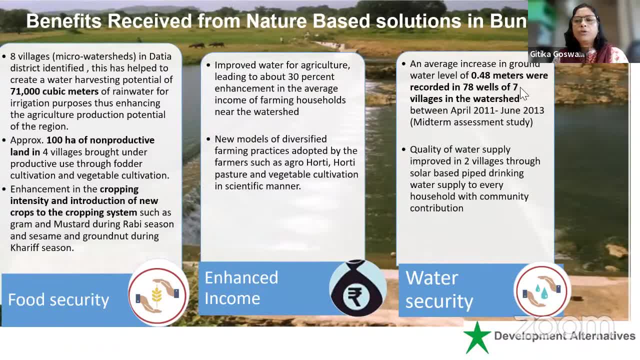 the groundwater. the groundwater level recorded 0.48 meters and 78 wells and seven villages in this watershed between this time, 2011 to 2013. and quality of the water supply, including two villages through solar-based pipe drinking water system, So that's enhanced the water security of that area. 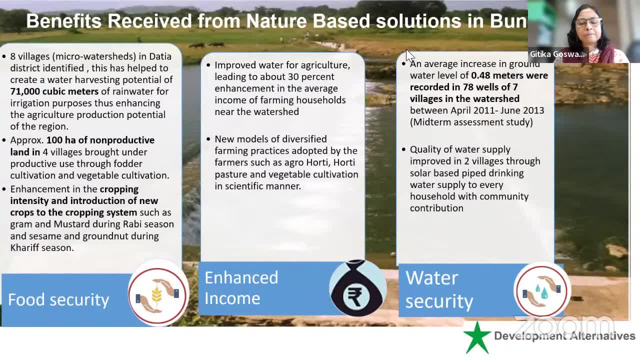 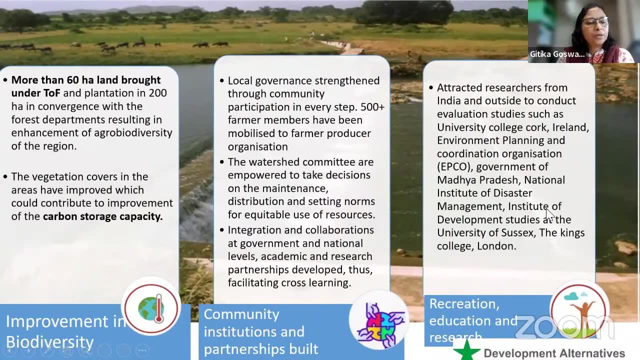 Then we have. There is also improvement in the biodiversity, because 60 hectare land brought under the tree outside forest and 200 hectare in convergence with the forest department, resulting in enhancement of the agribiodiversity of the region. The vegetation cover in the areas have improved. 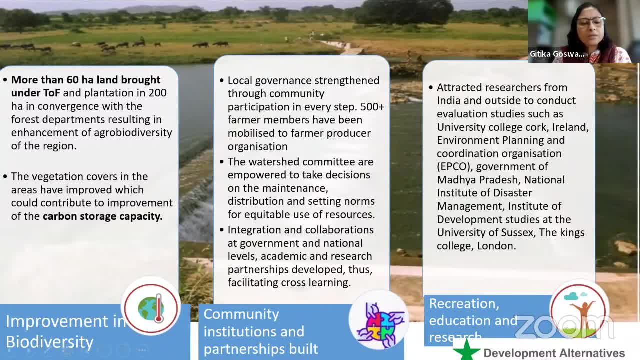 which could contribute to the improvement of the carbon storage. So that also shows that through NBS improved the biodiversity of that area. Then community institution partnership also built. Since you have the agriculture, you have good produce, you have good water condition, the local governments also stand then. 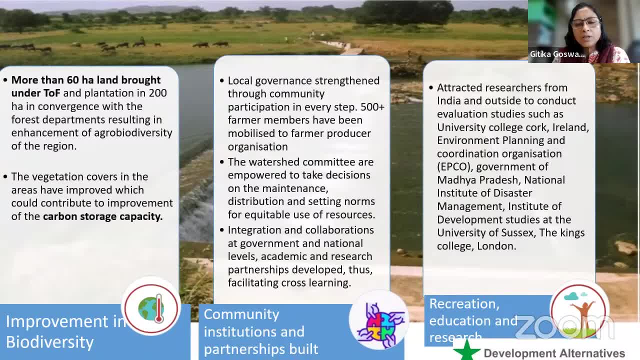 that the whole 500 plus farmers members have been mobilized to farmer producer organization. Water State Committee has been empowered to take decision on the maintenance, distribution and setting norms for equitable use of resources. Integration and collaboration at government and national level also happened, along with the academic. 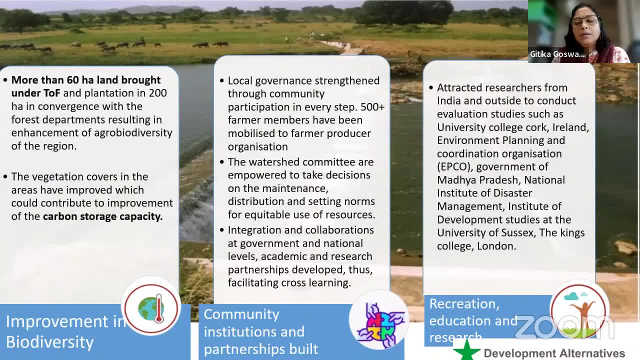 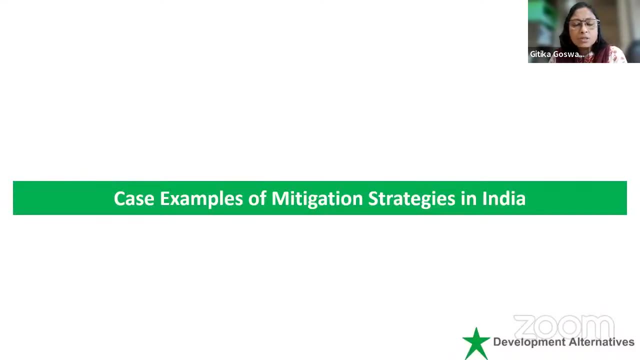 and research partnership. Along with that, there's also recreational and educational research also have increased. We could attract researcher from several places, from India and abroad, who came and did their research in that areas, also published paper Now coming to the mitigation. So this is all. 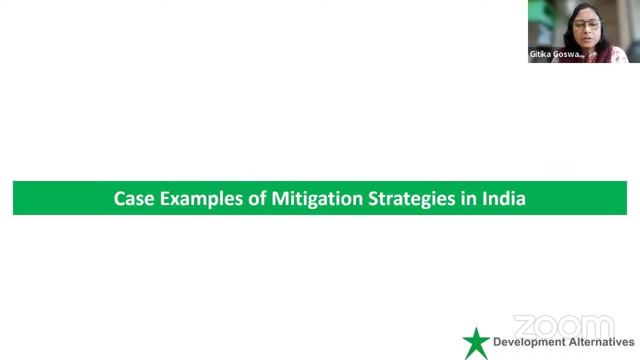 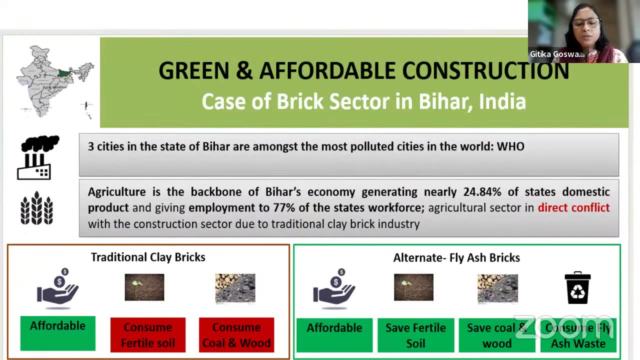 What I said till now was adaptation practices. Now I will talk about some of the mitigation strategies. in India, As you all know, there is in Bihar. we are working on a green brick sector- It's called. so what is a green brick? first of all, 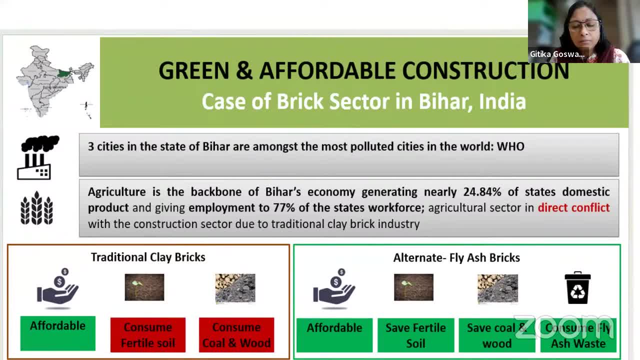 So, as you all know, the brick is a building block of the housing of our habitus, but then mainly in India we use, you know, earlier it used to be only red brick. Now it has been changed a bit, So red brick was all made up of soil. 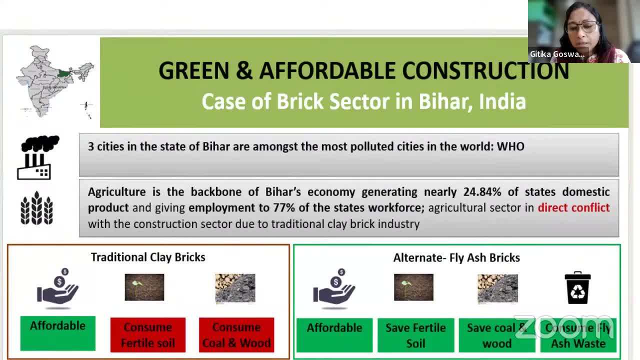 which is a topsoil and which is a very fertile soil. in case of like Bihar, because that's a gangetic flat plate And therefore there is also there are high chances of degrading the soil and, you know, losing the good agriculture soil. 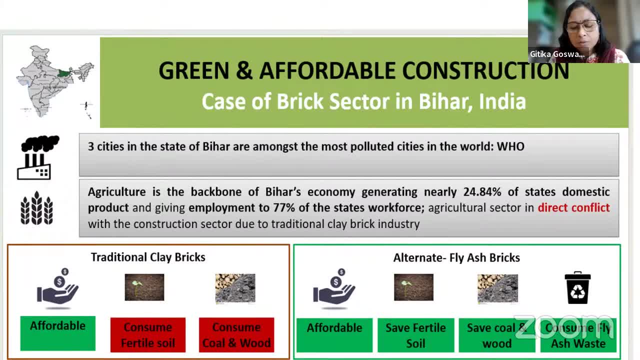 And therefore the agriculture. So what we did is we, and also Bihar, is having seven thermal power plants, And then also the by-product is ash And since it flies, it's called fly ash, And that fly ash used to be a pollutant a decade back. 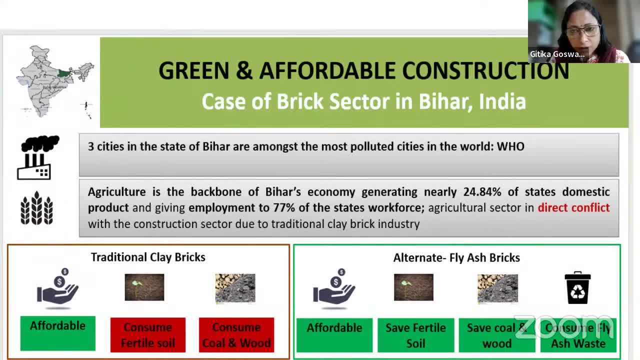 And we then started working with some of these technological institutes and come up with this. you know also, you know and come up with this. you know also also working with the NTPCs, the National Thermal Power Plant, And we have come up with one technology. 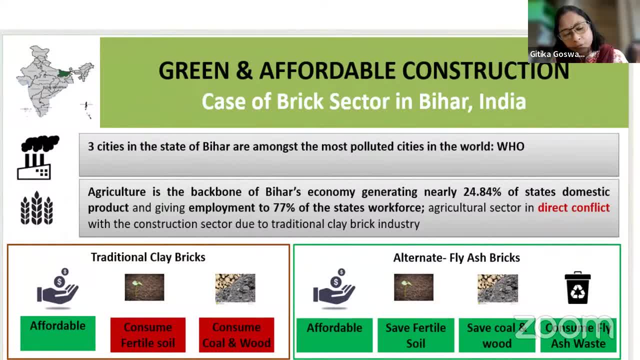 it's called fly ash brick. So how we can, when you know, in the plant itself we actually put a plant where it can condense all the fly, all the ashes in one place, And then we made the break out of that. 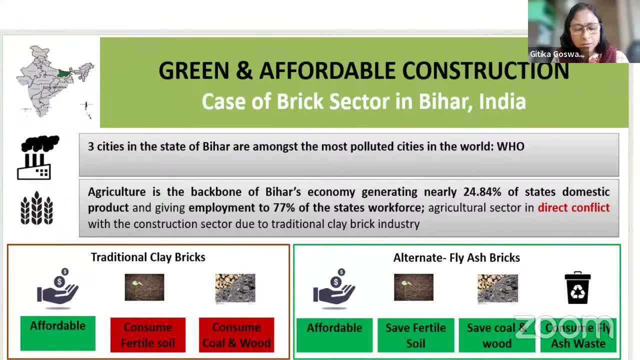 with some other component as well, with some cement and water And those different technologies that's available, And we made that brick. And that brick actually is a wonder product because it's not only taking soil, the top soil, So you are actually saving the top soil. 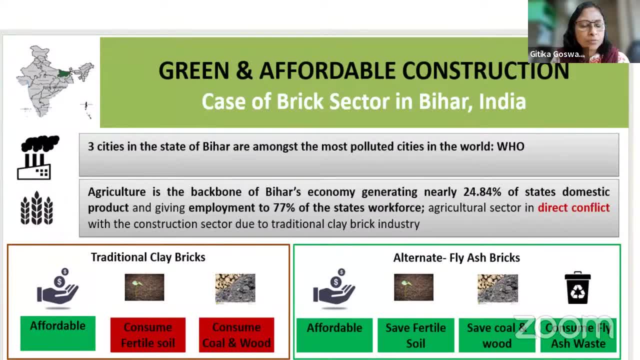 It's also not burned, because in the red brick it has to be burned And that lot of carbon emissions happens, but in fly ash bricks it has not been burned, So you can actually saving carbon emission And also it's a by-product and you are not. 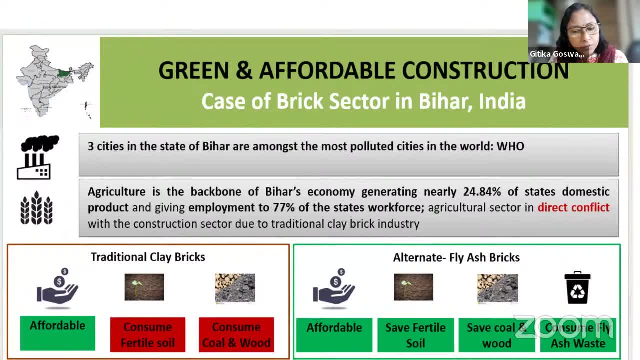 and also it's a product, It's a pollutant And so if you don't really do something out of it, it will pollute the environment. So these three things we have kind of worked together And we also at the same time 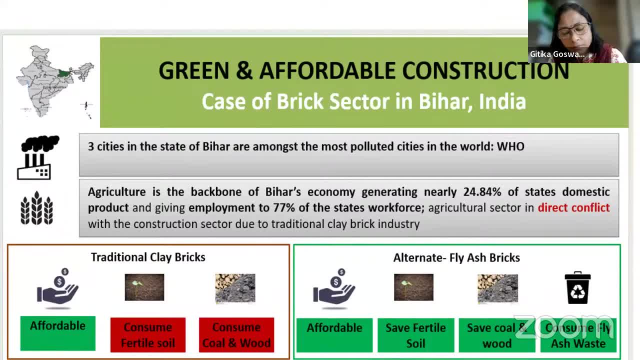 provided that this particular technology to many of the community people and they made their small enterprise out of this. So actually four types of benefits that we could get from the fly ash brick. So that's also kind of a mitigation, because agriculture is the backbone of Bihar's economy. 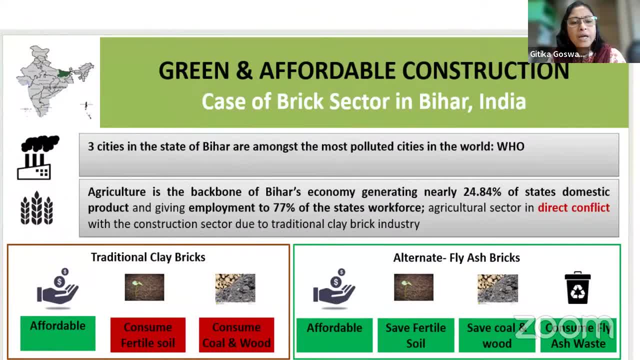 generating 24.84% of the state's domestic product and giving employment to 77% of the state's workforce, And so, therefore, if we could save the agriculture soil, we can actually not only contributing to the GDP, as well as reducing the carbon emission, and so on. 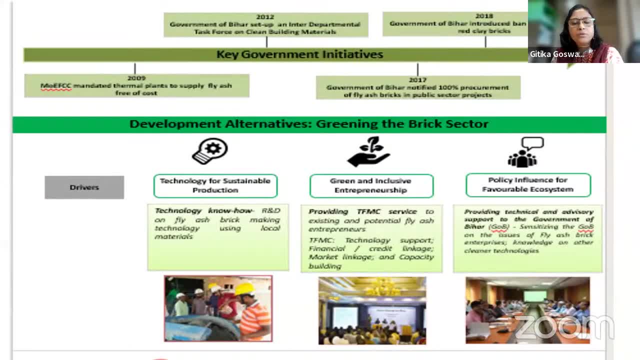 which I described just now, And we- so I already described. So with this we have also done a lot of policy advocacy. We also worked with the state government. They have then come up with the notification that all the government buildings will only be made. 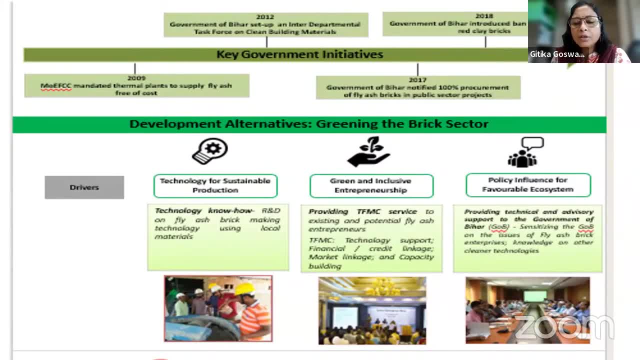 from the fly ash brick and there will be no use of the red brick. Now there are a lot of youngsters, young generation is now coming up. They come to us, they want to have their new, they want to start with enterprise and they want to start as a clean and green enterprise. 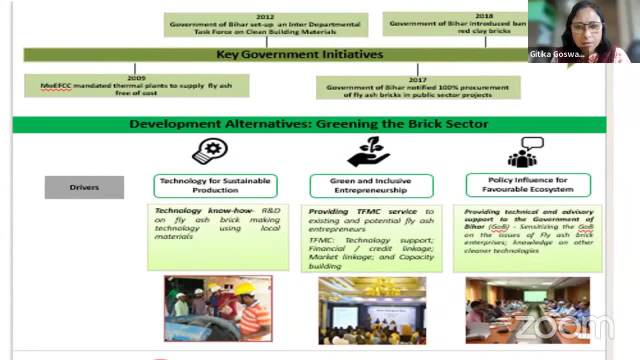 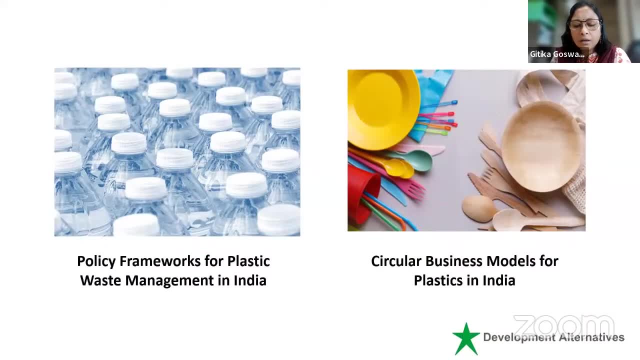 and fly ash is nothing like it, So this is that's why we call it green brick. We are also working a lot on the plastic sector, which is also a very harmful, as we all know, the plastic menace and the plastic era, and we are working. 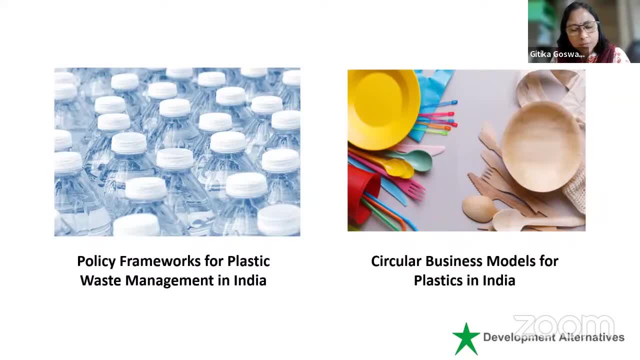 So therefore, we're working in four sectors to reduce the plastic waste and to make a circular economy business out of that. We are working with the policy maker for that extended producer responsibility, EPR. We are working for the circular business model which is already there in informal sector. 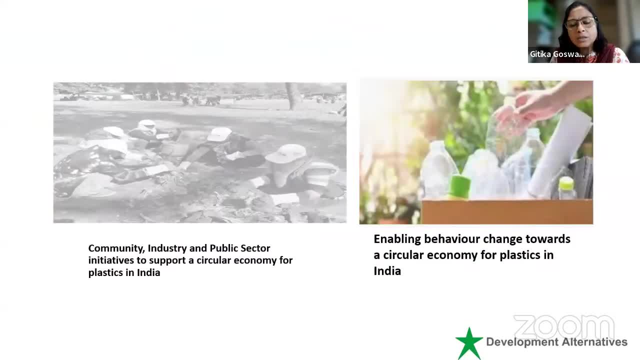 but we are trying to make it more formalized one to actually reduce the emission from a carbon emission as well as the pollution. We are working with the communities, and industry and public sector and small, small community enterprises are also coming up, Like in Assam there is a school, it's called Akshara school. 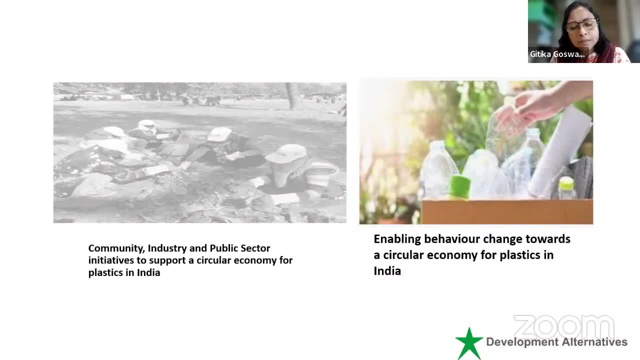 the school fees is only the plastic. You can give them the single use plastic bag. that will be your fees of that school. So it's a sounder, very extraordinarily innovative approaches. that is there all across India. We try to just try to accumulate all these together. 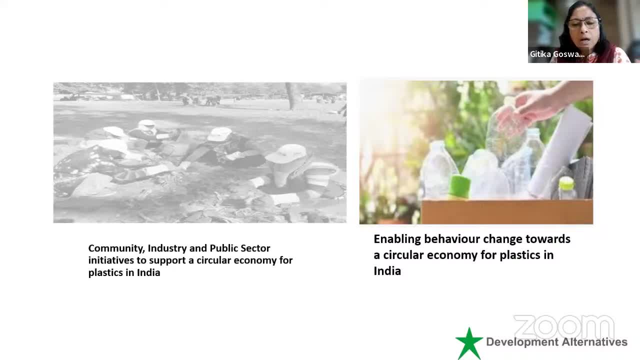 And we have come up with a strategy paper. and how does even the communities and how does even the communities, how does even the communities- communities can also make a difference in the society on this plan and make awareness of the plastic uh menace, then we are also working at the same time. the behavior change and this behavior. 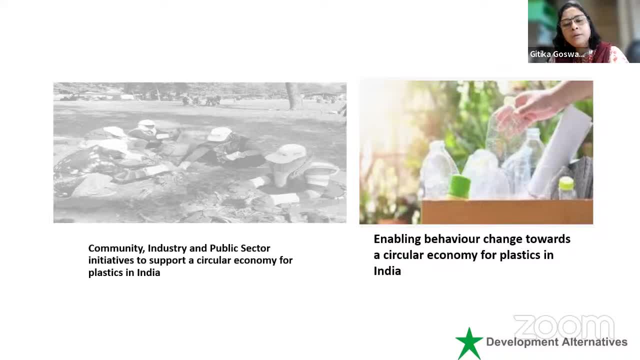 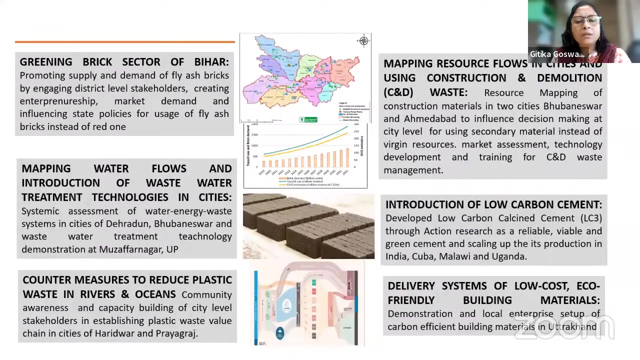 changes across from communities, from consumer to the, to the big corporates as well. so if we continuously, if we really avoid- you can avoid the multi-layer plastic like chips packet and so on- we can actually do great on reducing the plastic waste. then, other than plastic and fly ash, we are also working some of the other sectors to reduce the. 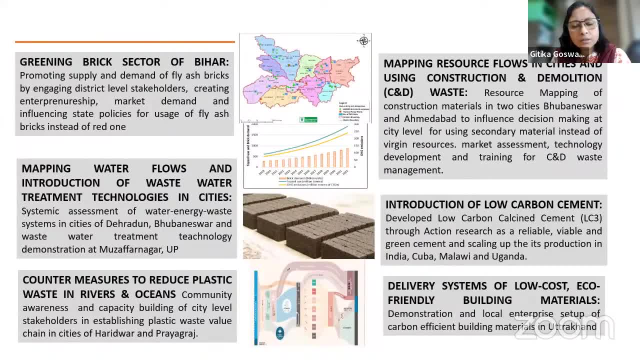 reduce the carbon emission and to make it a circular business economy. we are working with the wastewater sector as well. you can see. this is the, the photographs, that's a, the municipality, the water and the emission from the uh pipe water supply, you know, and the leakages. there are lots of. 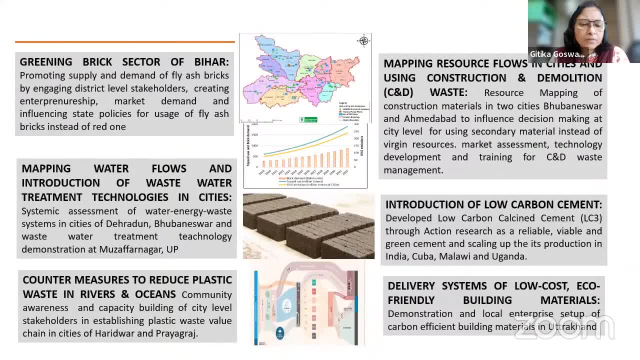 leakages that happens. we try to map out that. we are working with several municipalities on that water uh use efficiency as well as, um you know, reduce the uh emission from uh from the water supply. we are also working on another cement called lc3. it is also called a green cement. 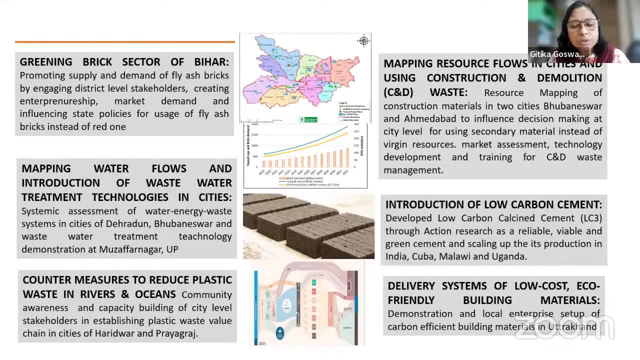 which is a kind of a kind of a new cement, but it is also known as a lime stone and you all know the cement is made up of limestone and limestone it requires, when we need to make cement, we have to do a lot of, you know, mining of the limestone, but this lc3 cement is coming up from from already. 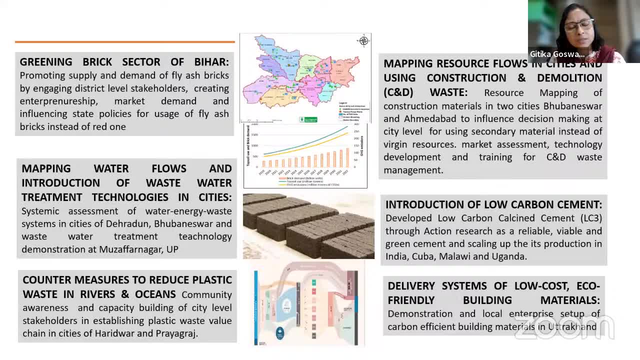 waste limestone. yeah, not no new mining is required, just using the waste limestone which is there as an over-warded around the mining areas. uh, we can. you can make this, uh, new cement, a lot of the cement working with us, like Holcim and others. and there's this, a great innovation in the cement sector, which 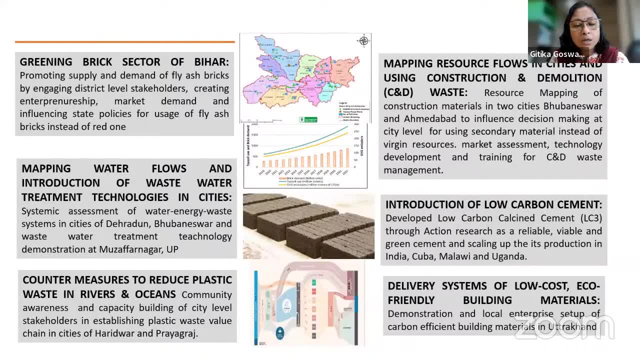 is the most pollutant in terms of the carbon emission, and so and there are also another is called construction and demolition pest, which is also another very important part of our city's life because, as you know, we India is really urbanizing in a very fast pace and a lot of new 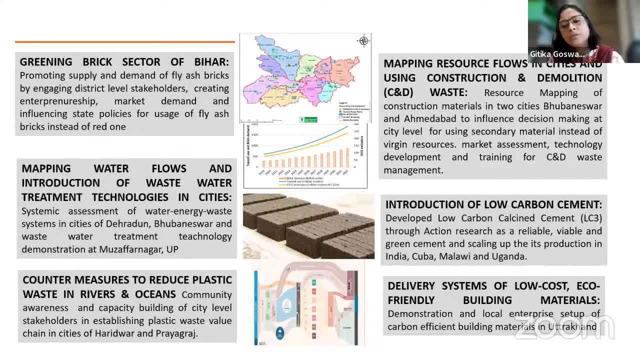 construction is coming up. along with that, the old construction is taking demolished and then this demolition material. you know it is important how we can really- and because of this demolition a lot of pollution also happens and our work is basically to work with the construction demolition vest and how to use this. 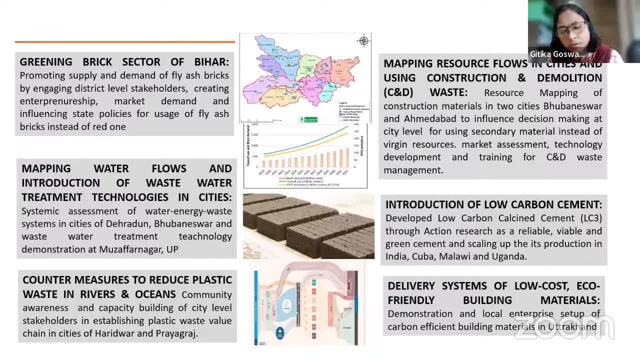 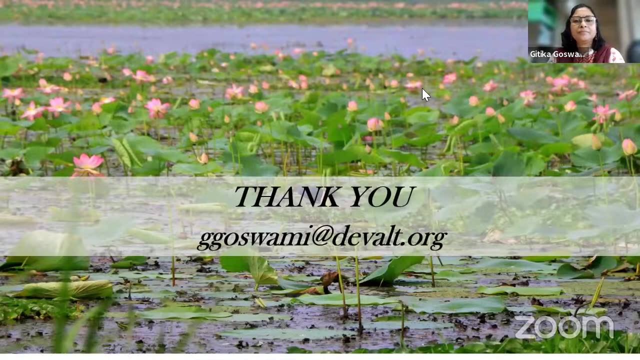 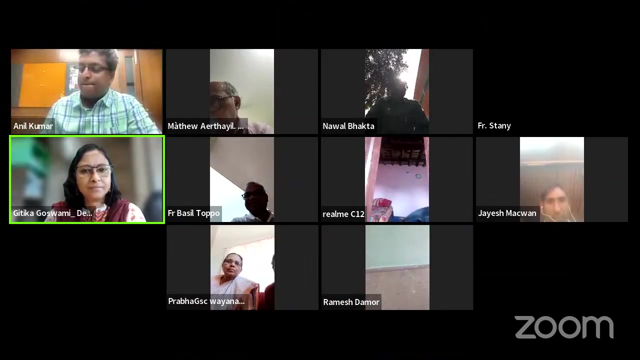 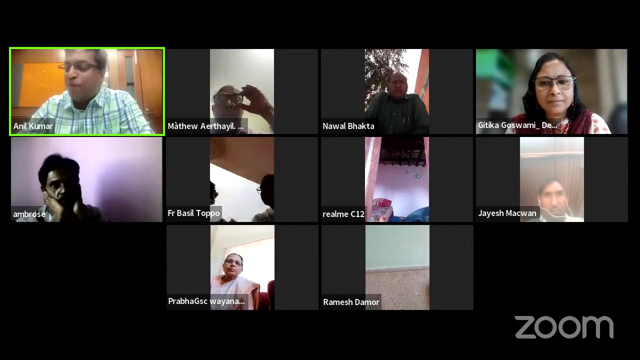 demolition vest into a, into a circular business, circular economic business, as well as providing, you know, livelihoods to the local community. so these are some of the mitigation areas that we are working and, yeah, thank you. thank you, many thanks, Githiga. you have provided a very comprehensive understanding of climate change. 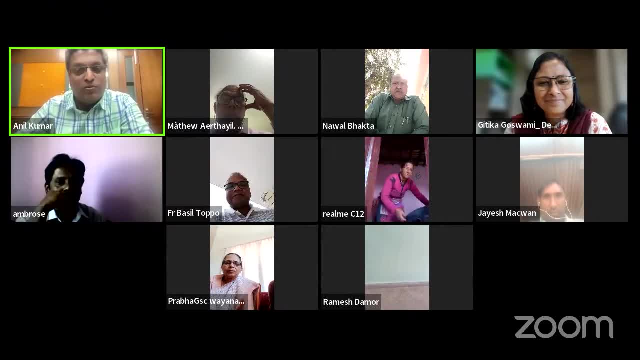 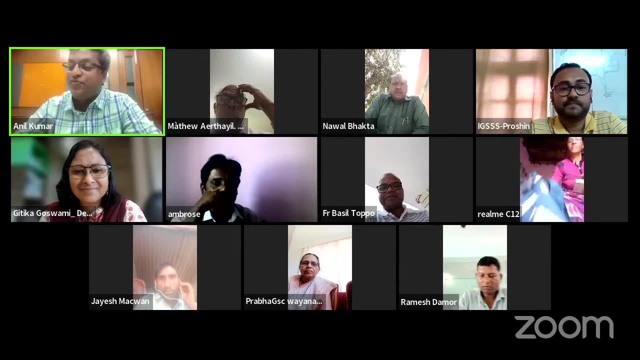 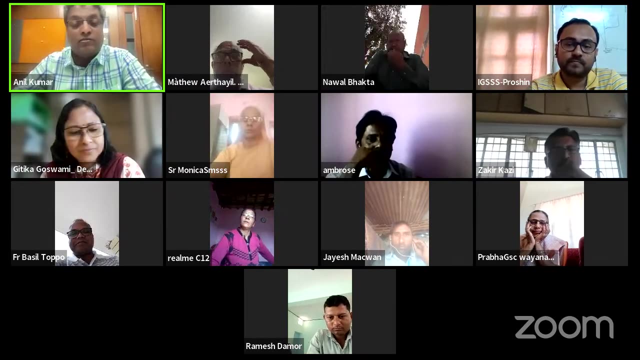 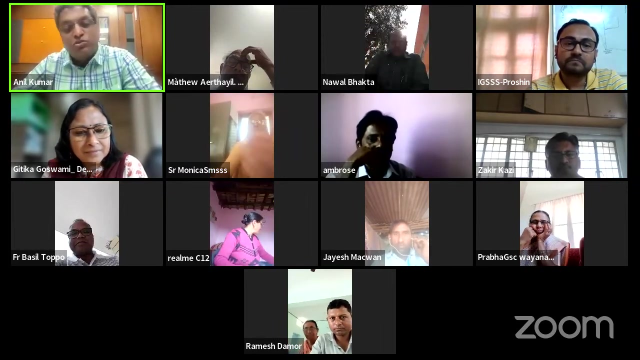 adaptation and mitigation issues, well grounded on development alternatives work across India. you have cited several examples, shared models and informed us how important it is to have a climate adaptive planning. Githiga also shared how climate change related vulnerabilities and adding to the existing vulnerabilities of women and kill especially girls, and thank you so much for joining us in. 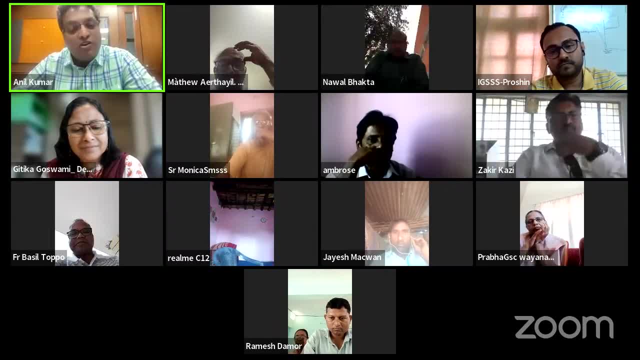 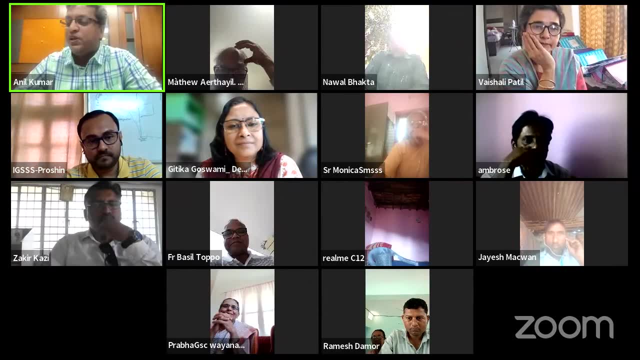 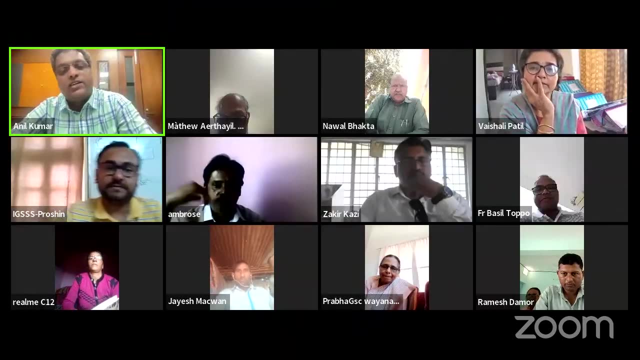 this important section today and we'll have a separate Q and A section after the presentation by Mr Proshin Ghosh. also now let me invite Mr Proshin Ghosh. Proshin is a scientist and research is the lead climate change adaptation program. 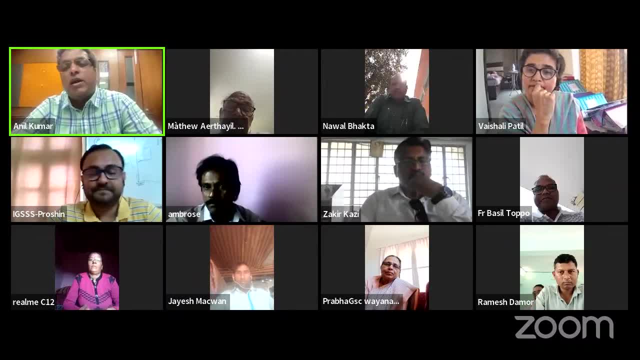 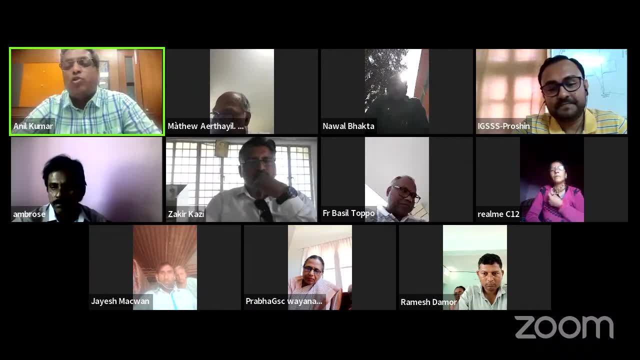 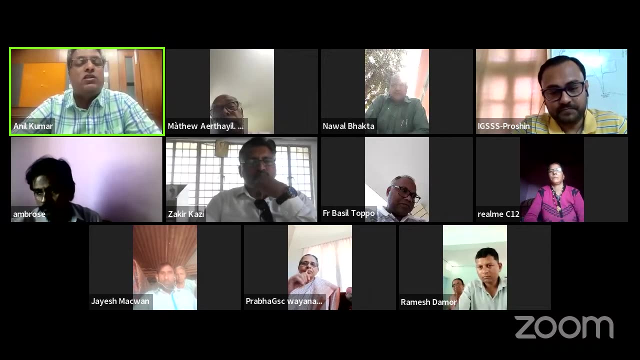 at Inter-Global Social Service Society Delhi. He's a community development practitioner addressing climate change crisis in vulnerable communities. Prashit has been engaged in identifying climate change risk and developing appropriate coping mechanisms for resilience. He is the innovator of urban disasters risk reduction model. 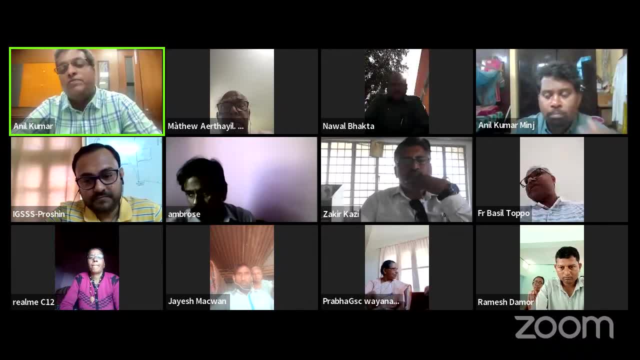 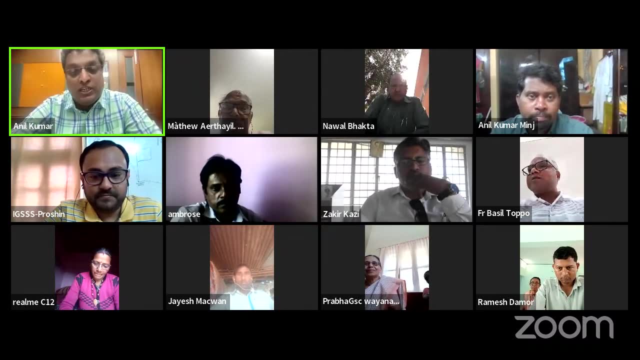 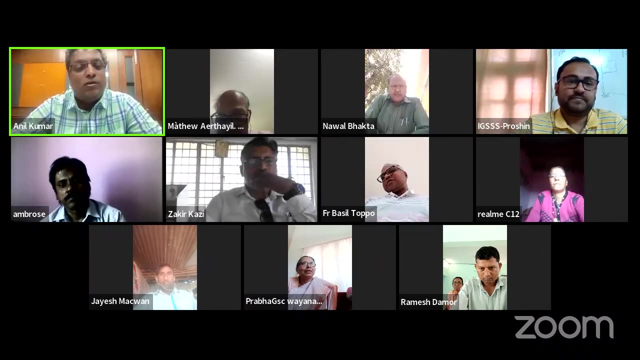 which is incubated in 13 project cities across India. Prashit will share about climate change metrics tool and participatory vulnerability mapping in today's technical consultation. Let me welcome Prashit Ghosh. the floor is yours. Hi, am I audible? Anil? 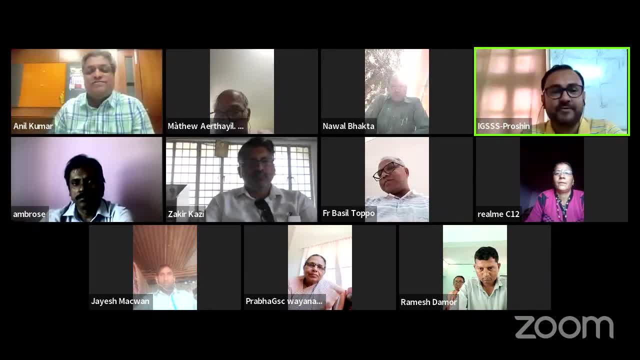 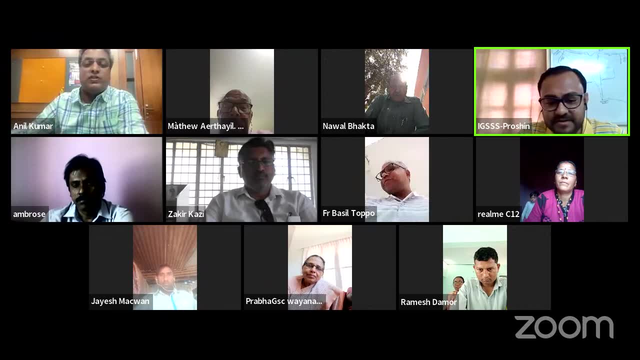 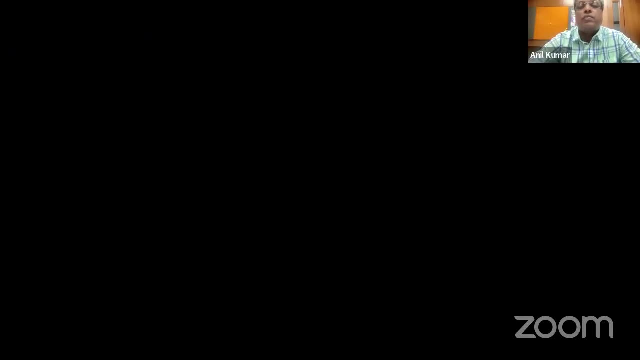 Yes, very much. Yeah, okay, thank you. So thank you everyone to be here Basically in today's my presentation. Anil, can I share the screen? Sure, yeah, Is it visible? Yes, yes, it's visible. 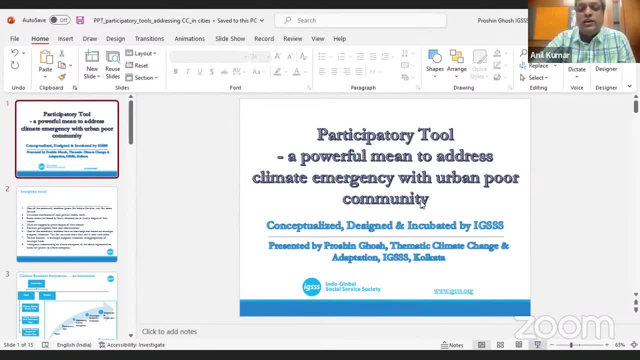 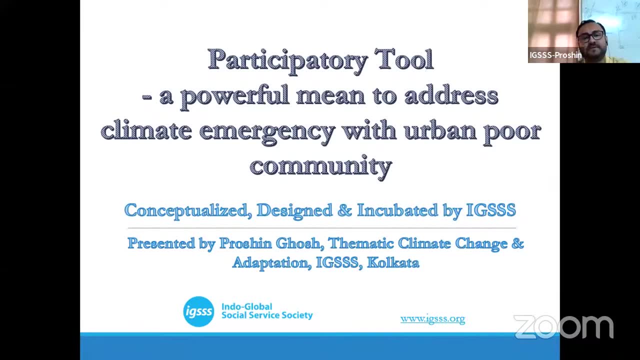 Okay, great, Keep it full screen, I think. Yeah, yeah, yeah, Yeah. well, thank you, Yeah. so basically, today I'll discuss about some participatory tools, as Anil said that we, Anil said that we, Anil said that we. 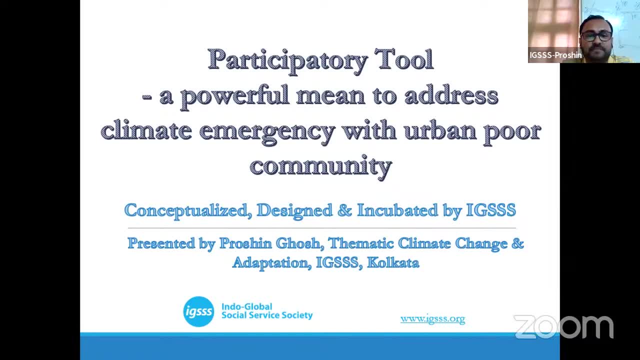 the IAS team had developed a lot of participatory tools, couple of the tools which are in time related to climate change emergency, to address these climate change emergency issues, especially with the urban code that is, in the slums. So basically, till now. 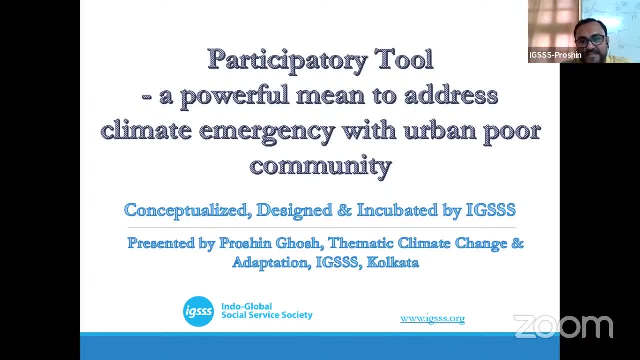 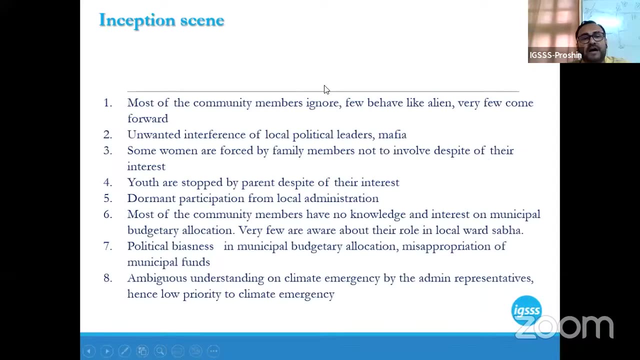 we have discussed about rural aspects. So now this is something different. that is totally urban aspect, and with the urban code community And with the urban code community. so next slide is: yeah, so basically, uh, when, uh, we are going to uh slump, uh, basically, we face such 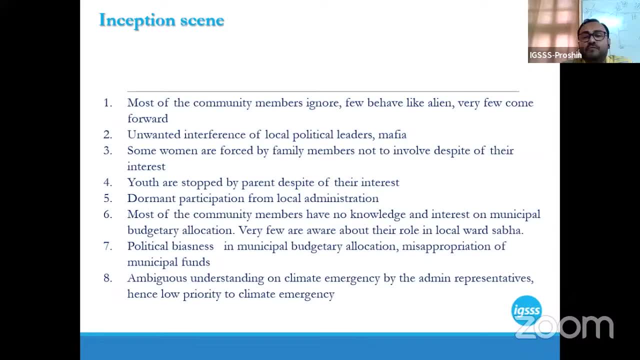 situation that is uh most of the community members see below. few behave like we are allies, uh. very few come forward unwanted interference of local political, local mafias. then some women are forced by family members uh not to avoid, uh not to involve with uh, with our team uh, despite of their 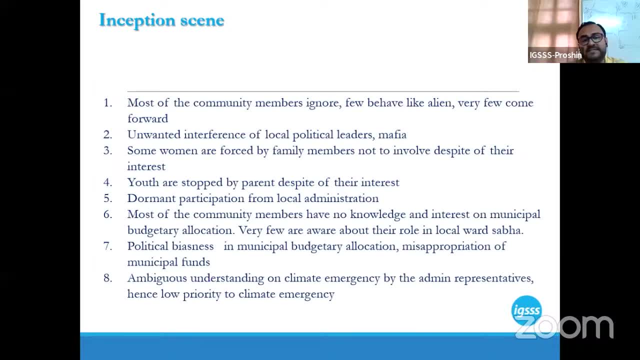 interest, basically, uh. and secondly, that everybody is very busy in the cities so youth are stopped by their parents, dormant participations of local administration. uh, then most of the committee members have no knowledge and interest on municipal budgetary allocation. uh, even few are ever about their. 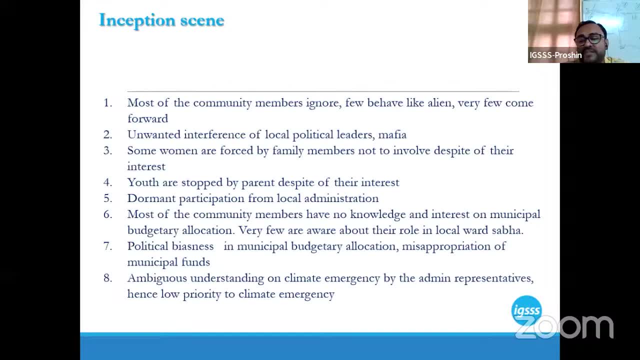 role and respond to the local wars. so this is the thing: uh we are uh far from the climate change emergency because our local- uh we will be, that is, the local urban bodies, are not very aware, or even even they are aware. uh, there are. these are the reasons uh they are not uh putting this climatic emergency in their 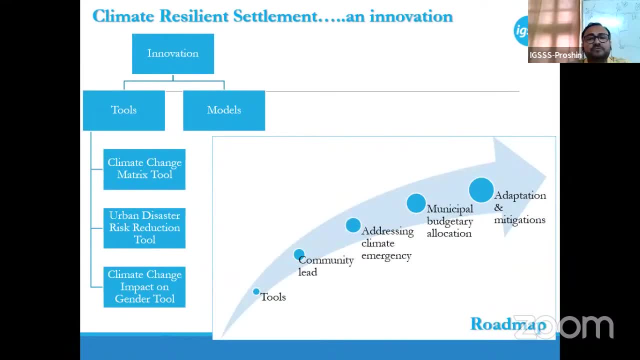 municipal budget allocations. so now the question is that, uh, okay, uh, just a minute. so, uh, actually the thing is that, uh, my uh heading is not sounding in this presentation. i'm not sure. probably there is a heading bar in this presentation. i'm not sure, probably there is a heading bar in this presentation. i can move this. 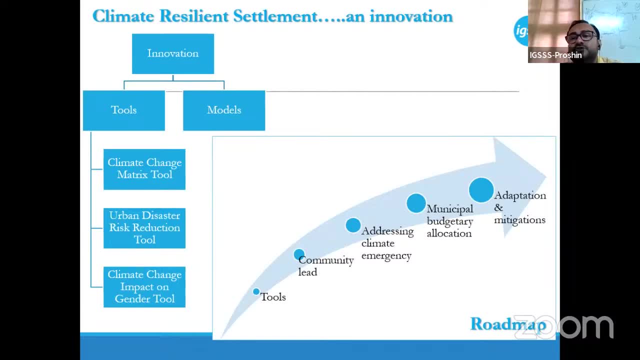 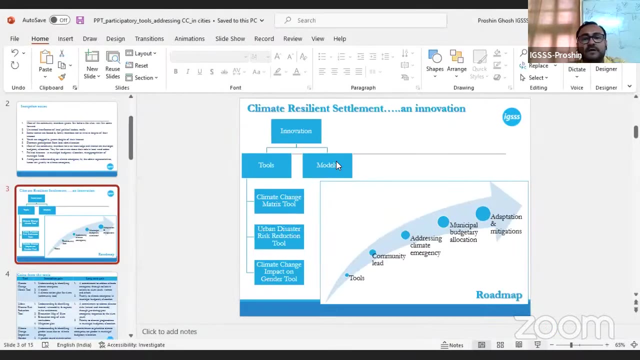 i can move this, uh, i'm not sure i cannot move this anyway, uh. so, basically, if we see that, uh, that any uh, so uh, if we see about any climate resilient settlement, so uh, uh, this is an innovation and basically, this is the this was a dream of, i guess. 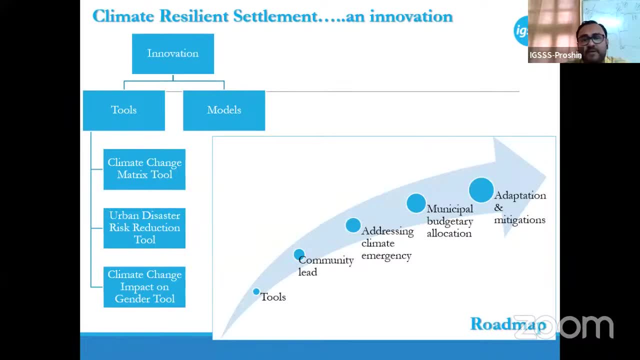 so, uh, this is an innovation and basically, this is the this was a dream of- i guess it is a couple of years ago- a climate resilient slump, and uh, if we think about the climate resilient slump, so there are some different types of innovations. uh, uh, we will uh play uh in the 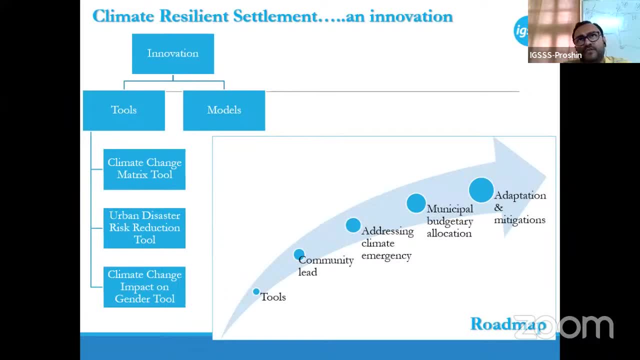 slump and uh, since uh, uh, three, four years, i guess, it is working in 13 cities, in 260 slums, uh, to make a climate resilient. uh, slump and it's been settlement. so, basically, uh, we are, uh, we are doing a lot of, we are applying a lot of tools, we are doing a lot of models. 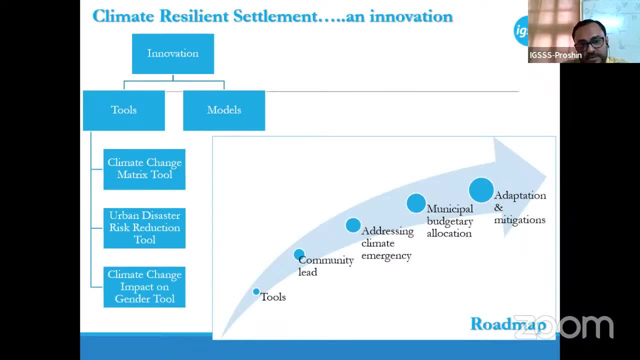 uh, which are in incubating, uh, basically in the slum. so, uh, i'm not saying about the models, because today is the topic is the tools, participating tools. so i'm just discussing about the tools. so, uh, within those tools, the three tools are very much correlated with climate emergence. 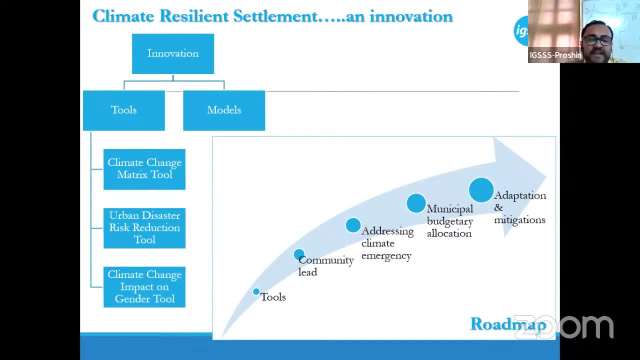 so the first one is climate matrix tool, uh. the second one is our disaster reduction tool and the third one is climate impact on gender tool. so, uh, these tools are basically uh, uh, when, when we discover and when we conceptualize and uh, prepare these tools. uh, the our main roadmap was the. it should be community-led, uh, and community. 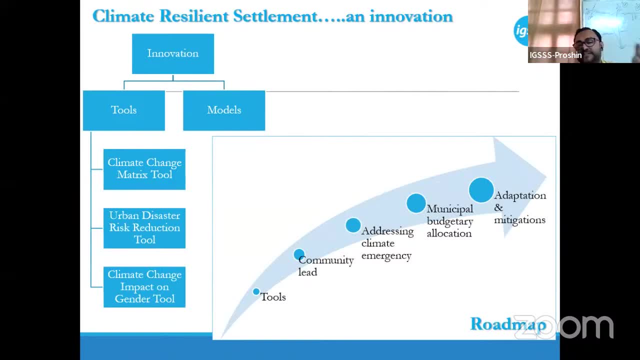 involvement is the mast here and the second is that basic climate emergency with these tools and third is uh how, how these tools can uh help uh community uh in maybe specifically budgetary allocations and ultimately, if the budgetary allocation done, then what are the adaptations and mitigations have done with the 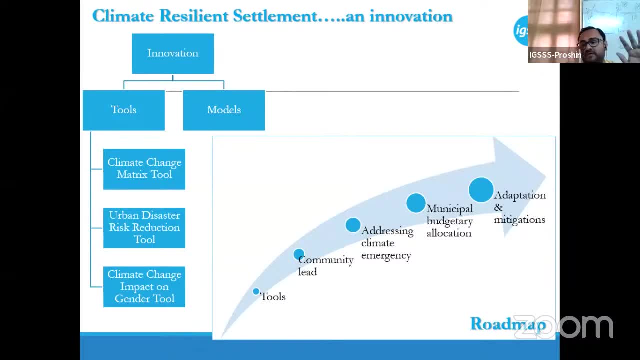 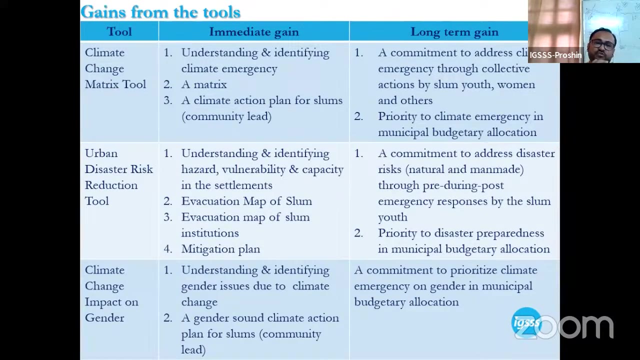 uh, urban core settlements. so these are the things, uh, these are the road maps uh, for uh, urban resilient uh settlement uh or other resilience slump. so what are the gains from the tools? basically, if we see these three tools, the climate change matrix tools, basically, uh, understanding, uh, the, the. if we see the short-term goal and a long-term, 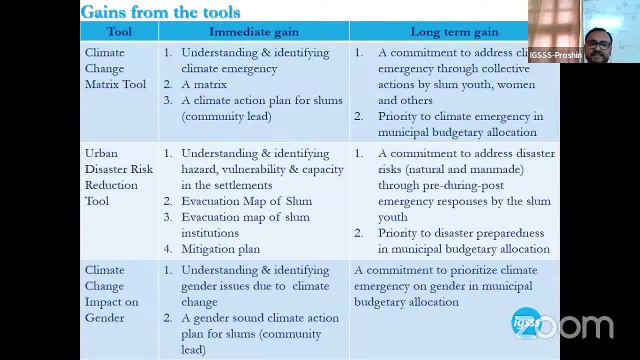 goal if we see the short-term goal: understanding an identified climate emergency. uh, student, what is the climate emergency? uh, the community members are not understanding what is the climate emergency. they can understand something: uh, that is too much hot here, too much cold, but uh, exactly what is? 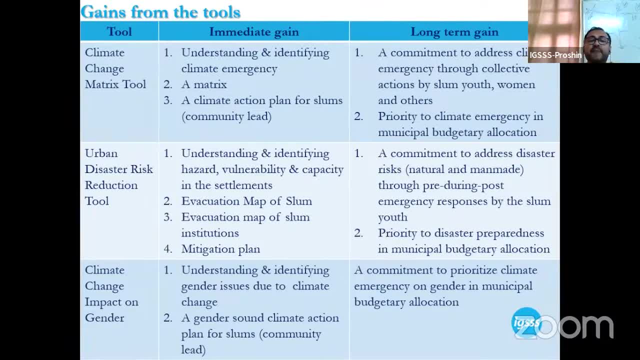 climate emergency- they are not uh very clear about this- then a matrix will come after the exercise and uh a climate action plan- uh totally committed- will come uh after this exercise and, in the long-term aspect, if we see a commitment to address climate emergency through collective actions by slum. 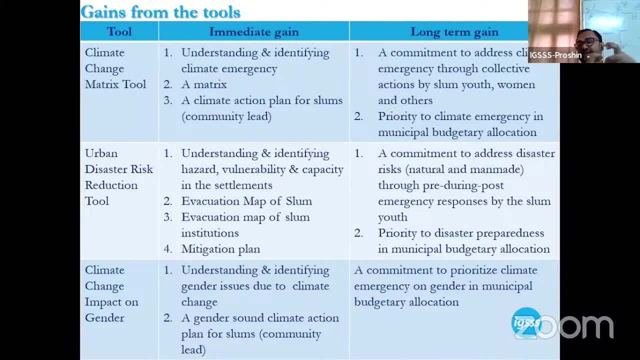 jobs, women and others- uh, i mean the york- have the commitment that we have to do something. uh, we have to address climate emergency through our and priority to climate emergency municipal budget and how we can prioritize a municipal emergency allocation in respect to climate change emergency. in case of second tool, that tarpon disaster is production tool, the uh immediate. 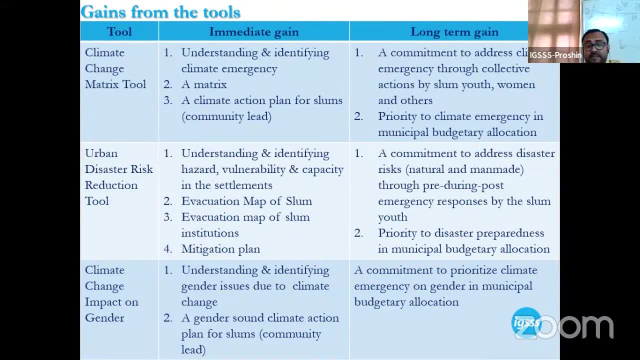 way is that understanding and identifying the hazard model in the capacity, in the settlement, uh, even then, even uh, the uh, the community members are not very much, ever, ever from the wasn't the vulnerability, but it's the capacity within the, within them, within the uh and then evacuation map. 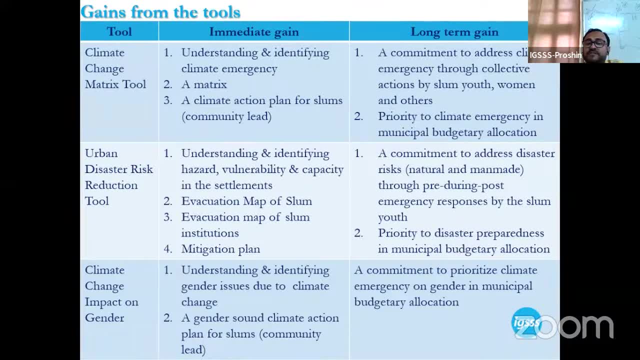 which will come after the exercise, and the evacuation map of the slum and the location, one of the institutions- and the mitigation plan, which will come up to exercise. if you see the long-term gain, then a commitment, uh, within the slum community that to address the disaster risk. 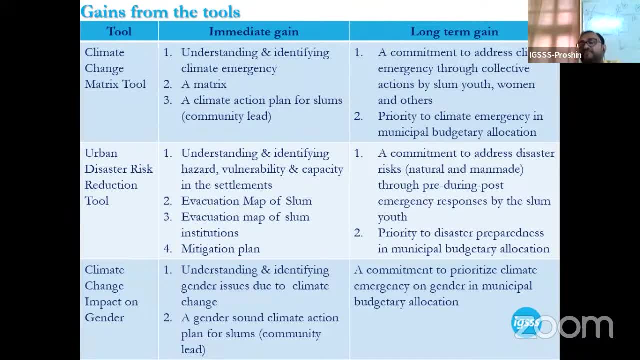 maybe natural, maybe man-made, uh, through pre-during and post-emergency responses by the slum, basically, and then priority disaster preparedness in municipal work. then the third tool on the climate change impact on gender. this is totally focused on gender. so, basically, if you see the short-term goal, uh, that understanding. 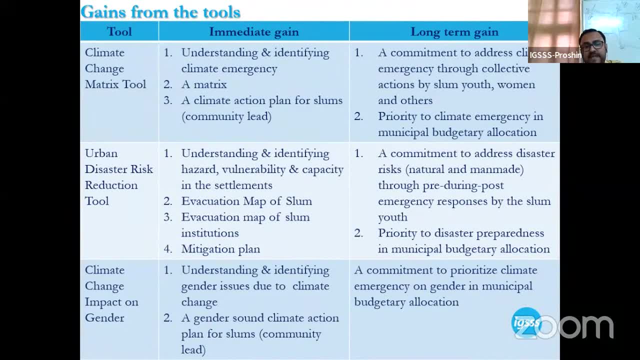 and identifying gender issues due to climate change and there are genders on climate action plan which will totally communicate, which will come after the exercise, and a commitment within the slum to prioritize climate emergency of gender in municipal budgetary allocation so that in the in this pre-tools, the main aim is how to mobilize municipal budgetary allocation. 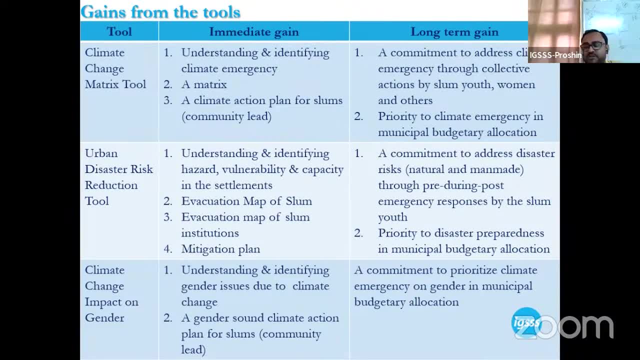 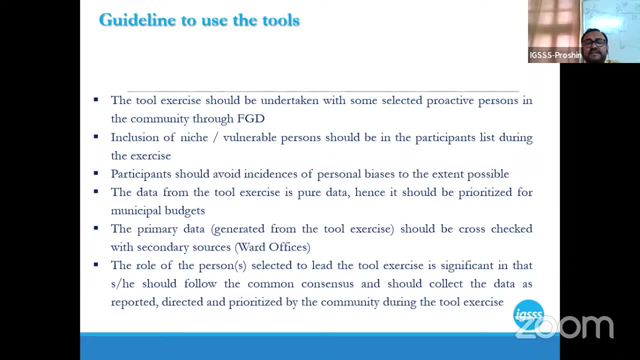 how to be managing the climate emergency and municipal budgetary allocation through the tools. then what is the guideline to apply these tools? first of the tool, exercise should be annotated with some selected proactive persons from the community to achieve, uh, a purposeful discussion of the recent vulnerable community. uh persons uh like uh, pregnant women like this uh. 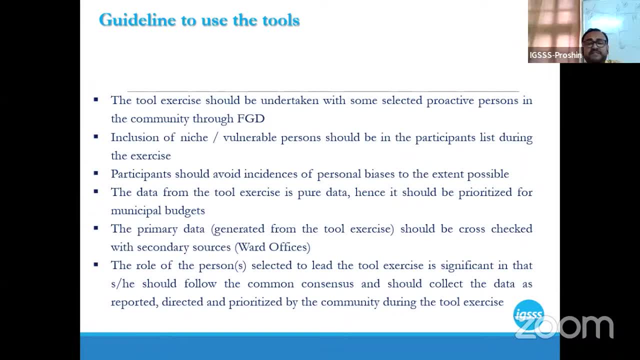 should be within the participant participants list during the exercise. participants should avoid incidences of personal biasness or to extend that as much as possible. the data from the tool exercise is very much pure. hence it should be prioritized for municipal budget budgets. uh, and then the primary data that's generated from the tool and 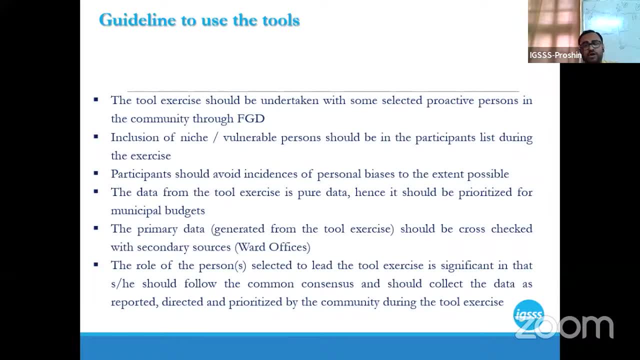 will be costed with the secondary data. the data which are in the uh ward offices mean with the officials and uh. the role and role of the person selected uh to lay the tool exercise is very much significant in that he or she should follow the common consensus and should collect the data as 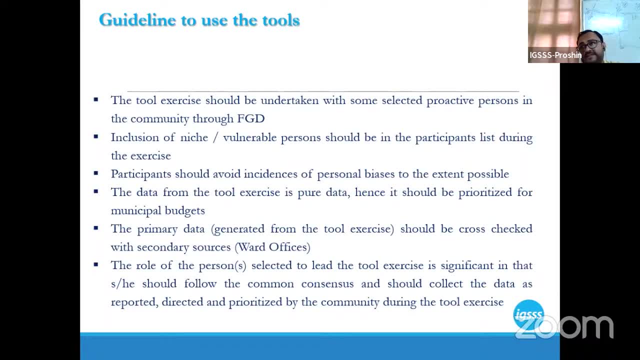 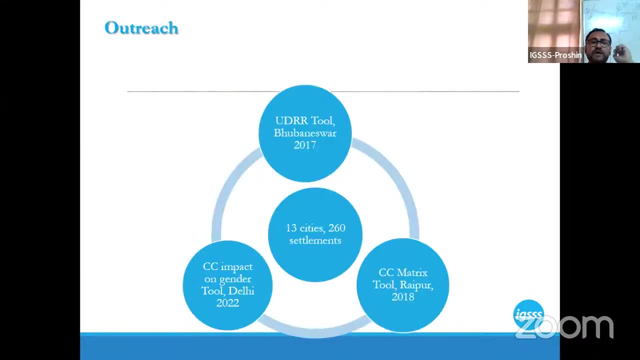 reported, directed or prioritized by the community with the tool exercise. we will- it should be- do that seller and we will be a good presenter with the maps. so, basically, when the tool uh started- which time so the risk of the outreach is- we started 2017. 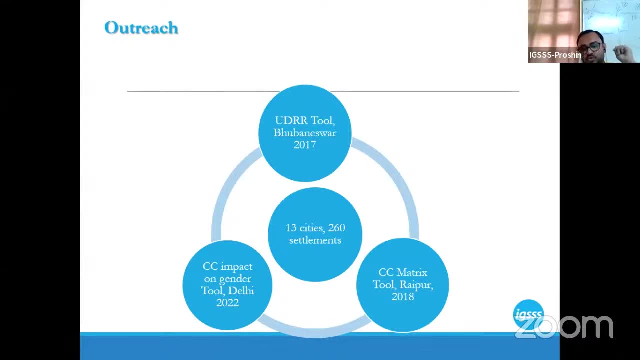 uh- we piloted this tool in rohanishwar- are the registered production tool. uh climate matrix tool was piloted in uh right in 2018 and climate change impact on data was piloted in delhi. and now all these tools are successfully implemented within 13 semesters to slah. 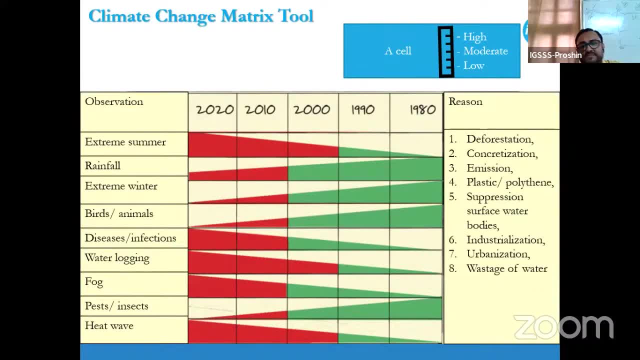 now i'm coming to climate, uh, matrix, climate in matrix 2. this is totally uh driven by community, uh, basically, especially the youth group and the will. so if we see a sale, because this is a matrix, so each map, the matrix is comprised of lot of cells. so if we see a cell, so the sale, uh, that is. 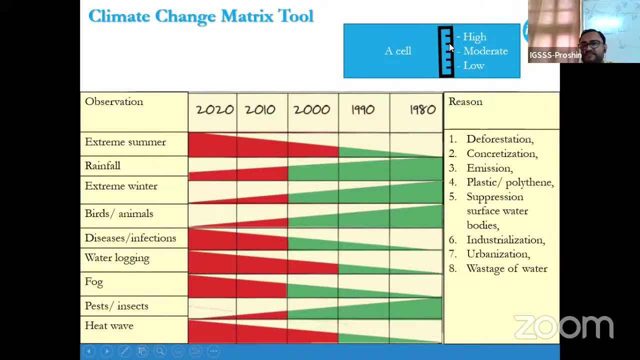 we, we have to, uh, we can divide this cells with a scale like this. so if it is more low, then the scale way and in the low or edge, and if it is a moderate, then the scale must be the middle edge, and if it is a high uh parameter, the scale must be in the uh upper edge. so this is totally our assumption. 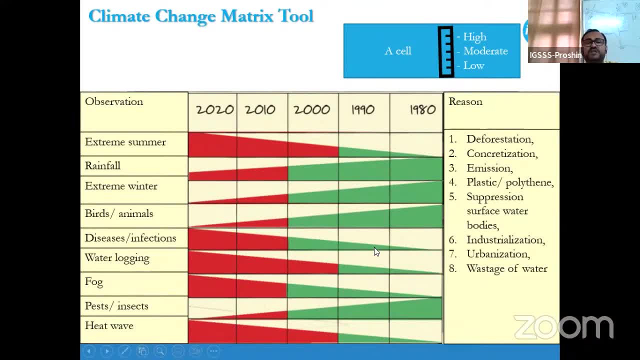 this is not very much scientific and very much database. this is totally the assumption to be the understanding of the community. not very much scientifically but it's totally community. so observation is that extreme summer. so we will ask community that what are the situations you are facing due to this extreme climate? 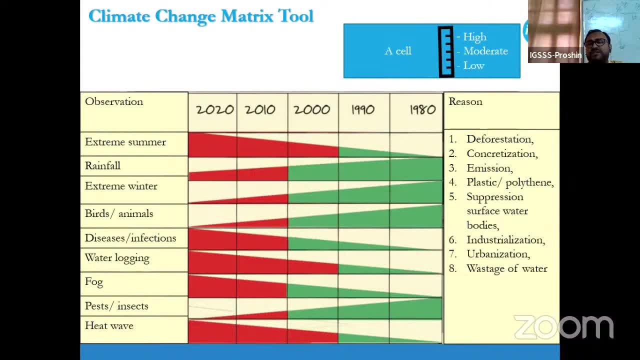 so then they will say that, uh, now we are facing extreme summer. so if it is extreme summer, then it means graph the water status in the last 50 years. so we have calculated the last 50 years situation, so it's 1980 to 1990, the 1990s thousand, 2010. 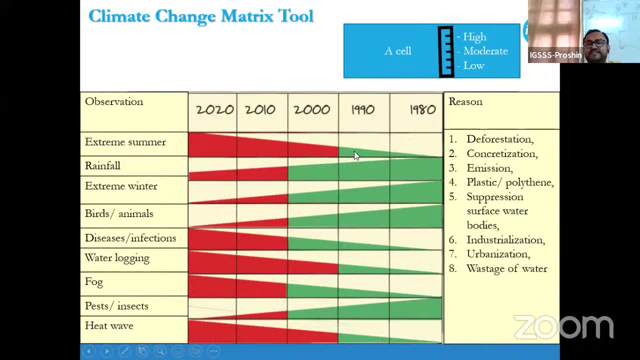 so they are saying that, uh, during the 1990s, but not very much high, but after this, 2000, uh, it's been very high. so this graph is like this: they created this graph and it's a very, uh, highly vulnerable situation from 2000 because there 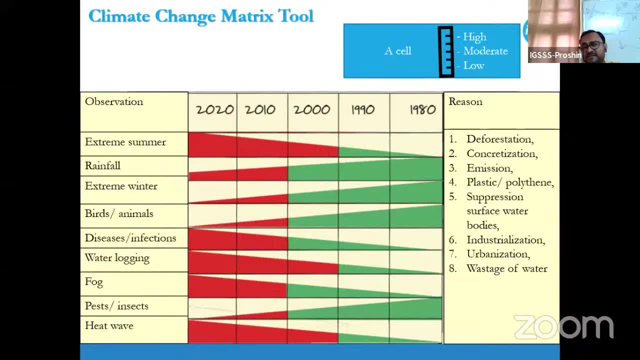 is: uh, the limit is there. the limit crossed, uh, crossed. uh, the extreme summer crossed the tolerable limit uh, of the people. so they give this is in high value and it's not. it's a moderate man. so this is the understanding of the family. so, in the same way they are preparing, 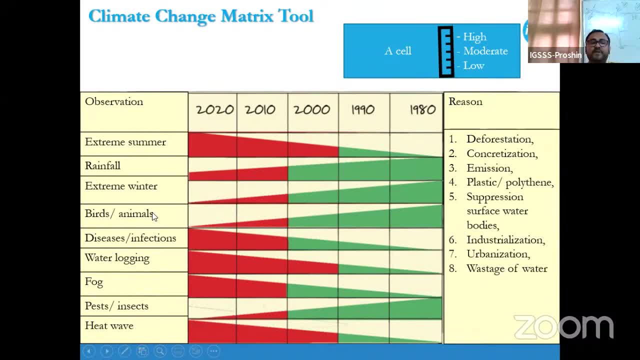 the graph of rainfall. they are preparing the drama, extreme winter. they are preparing the drama, extreme winter of what is the status of birds and animals in your local, local, local chief and degrees of diseases and infection. the water logging pops. these all the observations coming by from the committee, so we are not just facilitating the things we do. 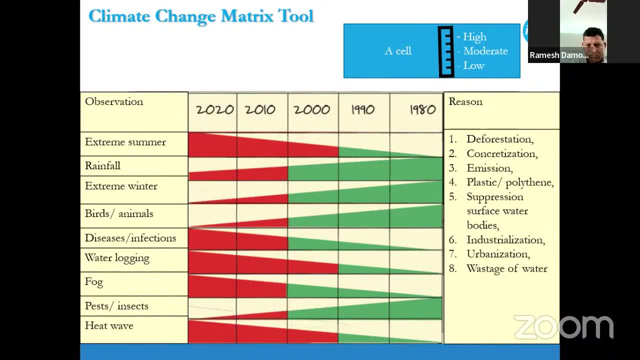 not force them that. what is the situation? tell me the water logging, the water logging. this is not good. this is not good. we don't ask them such things. this is not good. And they are preparing these drafts with their understanding that. what are the situation? like this, in the current situation. 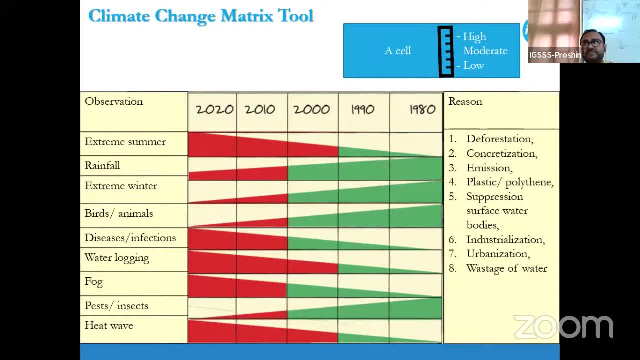 And, of course, the FGD will comprise of the youth group, leaded by youth group, but the FGD will be attended by young women, elderly people, Khaskarpe, 1980-ka, information, Chinese, The people who who are in the cities. they must be present in the FGD. 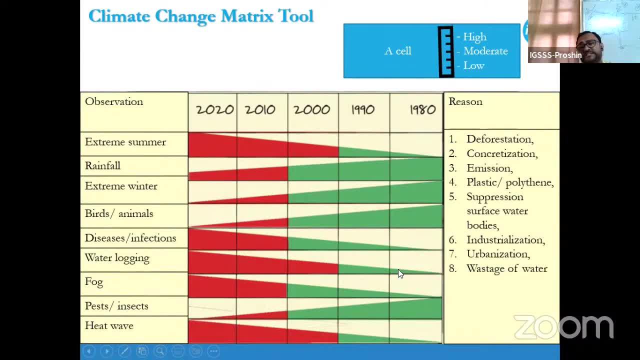 What is the reason? the people say that maybe deforestation, concretization of the city, because there was no such ground in the city. Everywhere there is it, either in roads, in the industry, then emissions are having to focus, And then medicine and politics. 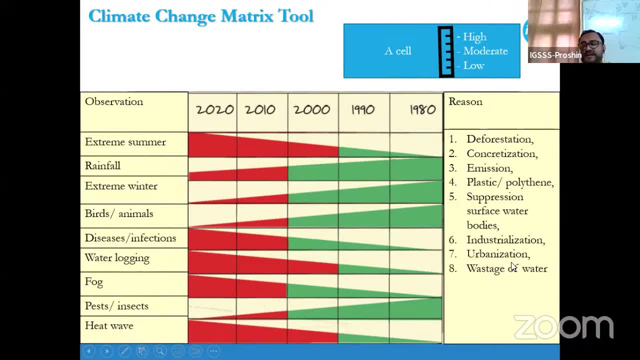 issues: operations of surface water bodies, industrialization, urbanization, waste or wastage of the water. so these are the things. this is totally comprehensive, very colorful things so that community can get interested and we can participate. this is a interior, very simple tool and just embrace the interest and just with the understanding to the community budgets. 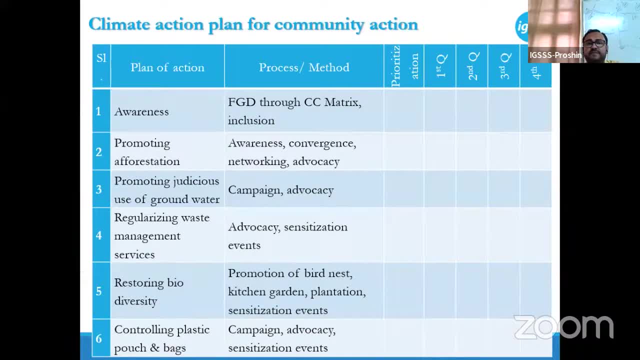 and after this tool, we, they will come to this climate action plan, uh, totally community. so they say that the plan of the awareness. so how they will raise the awareness like this way, that they will do this actually, uh, through this climate change matrix, uh, and inclusion, then maybe the 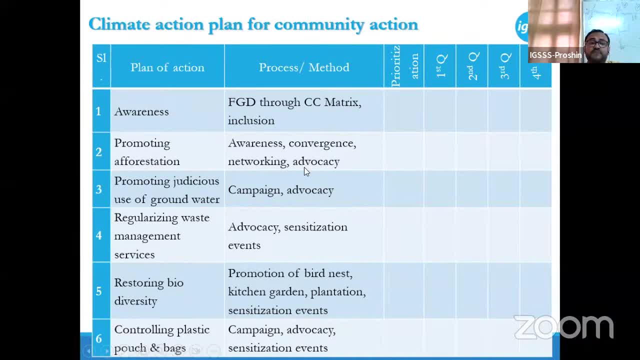 promoting our forestation with planting, awareness and convergence, developing for planting, uh, some trees within the cities, from the cities then, uh, promoting judicial children from one or two capital and advocacy regularizing waste management services, advocacy with the local municipality and sensitization events like this restoring biodiversity. 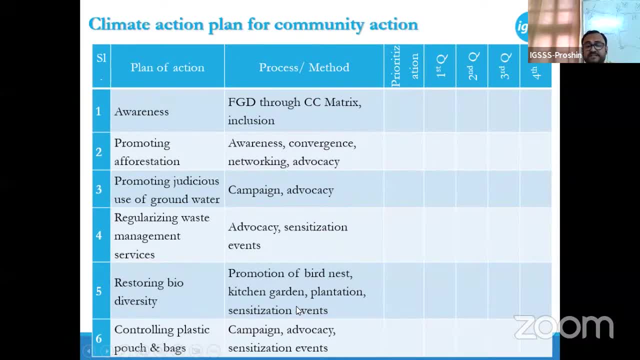 uh, maybe promotions about those kitchen garden plantations within their household premises like this, and contouring plastics and volume bags. so these are the things, these are the very important. maybe as they understood that if it's a department, so these things must be addressed and they planned. 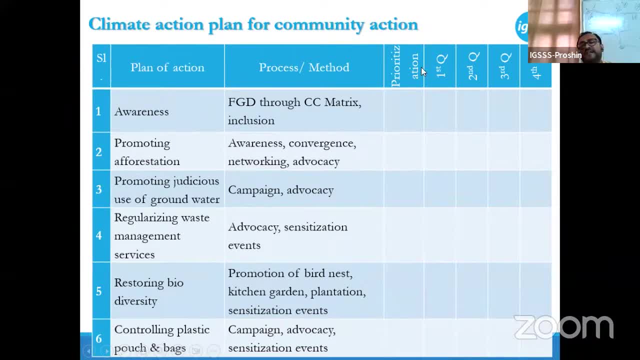 as per, uh the things, uh, this is the plan of actions and this is the prior. prioritization will be that which one we will do first and which one will be second into third. this is the prioritization column- and in the first quarter of the year, which one will make, and then the second quarter, the third one will focus on what things will. 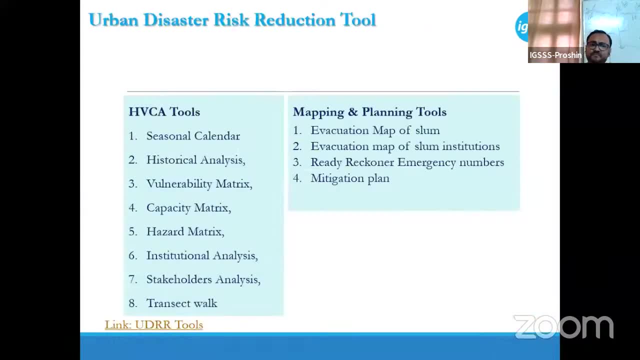 play. so this is the climate change matrix. now we are coming to the second tool, that is, urban disaster risk reduction tool. so the carbon resistance production tool is comprised of from hbca tools. we have a quality capacity tools. there are eight tools: seasonal calendar, uh, historical analysis, voluntary mapping, capacity matrix- capacity matrix- hazard matrix- institutional. 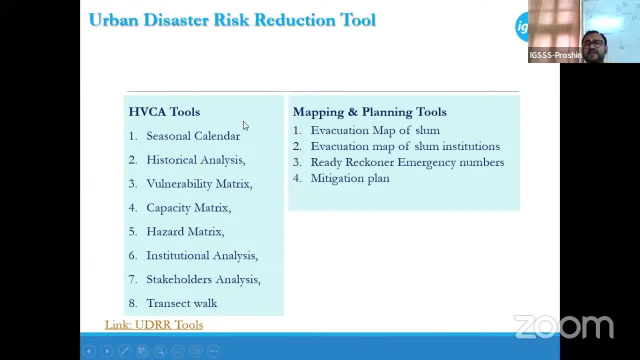 analysis and uh. these are all these tools very much in aspect to climate change and disaster. and then uh mapping and the planning through this evacuation map of the slums, evacuation map of slum institutions, uh ready recorder, emergency numbers and the mitigation plan. so if we see the links, so 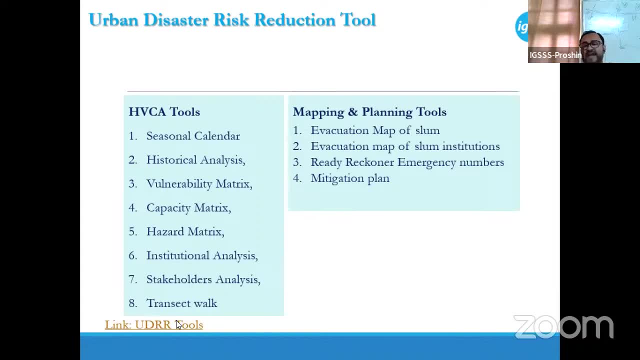 basically seasonal calendar. this is the signal calendar jam to december. and then what the hazards you are facing with that rain, flood water. these are the some hazards given here and some someone others. uh, that it will uh help the community to think, to uh understand what are the things and 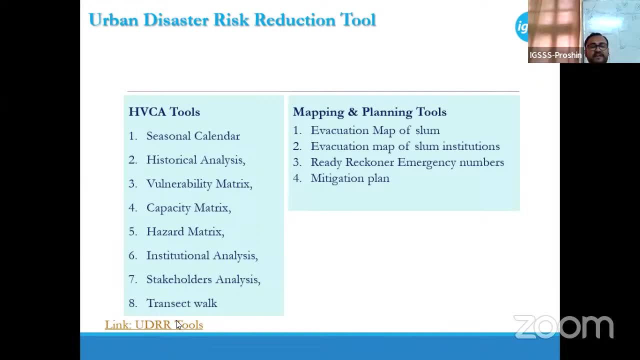 they will come back with their answers then. human diseases, malaria, diarrhea, someone others, occupation, migration, immigration like this and others, many food availability, uh related festivals, uh unemployment and alternative- i mean seasonal environment and alternative impacts will be dead like this. so this is the seasonal calendarian aspect to different disasters or climate change. 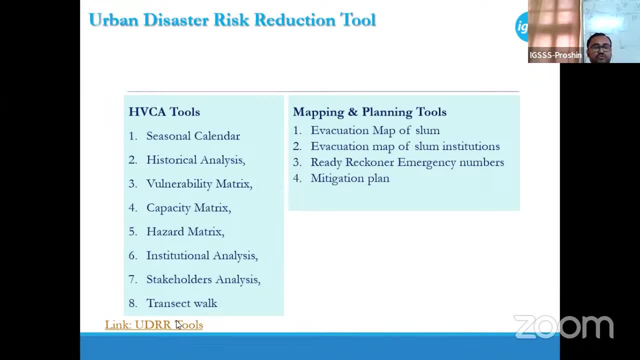 then uh historical analysis from 19th to 2018, so from january to december. which year, which month they are facing uh extreme climate events? this is the uh historical analysis. then vulnerability matrix: this is the matrix, that is. there are two different categories. one is population uh. 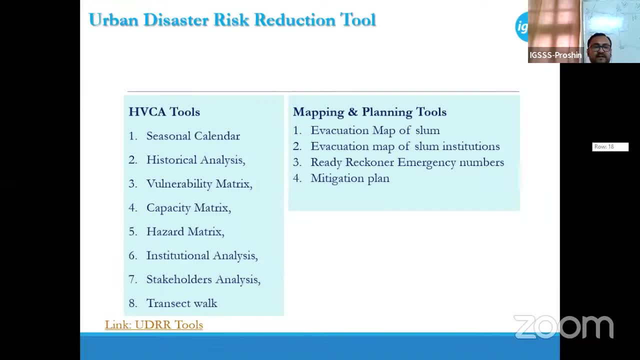 balancing population. the second is constructed. the third is: uh, yeah, these are the things then, uh, population. if you see the population basically, um, the vulnerable people are, together with these children up to six years, pregnant women like eating women, serious, uh, within the slum. so this is the population based vulnerability assessment and then infrastructure. 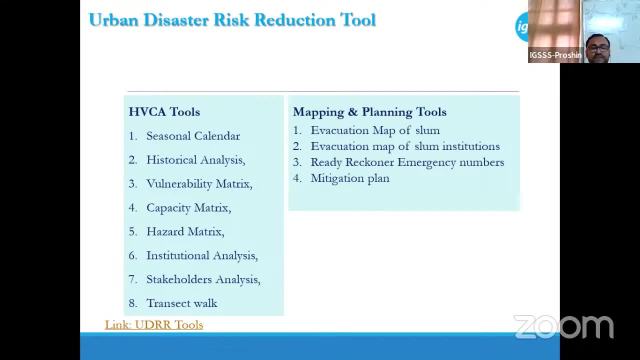 with vulnerability around in the house, although is suffering with portable, without portable water? how long suffering without sanitation algorithm? suffering without complexity? how long, uh, having tapping electricity algorithm ability to do what you need to do, what you need to do and how to perform the work of the people's? 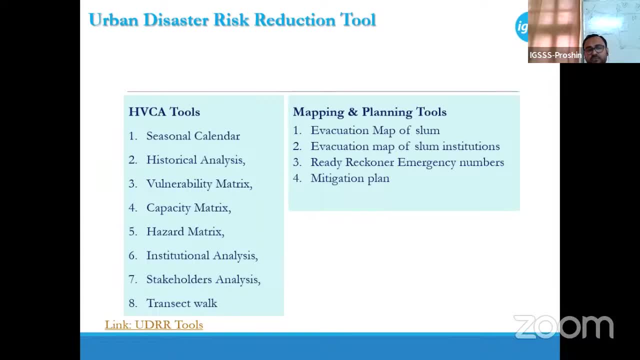 care as well, and all of these things are taking place within the slum, so its really important to waterlogged area. So these are the indicators which can access the vulnerability, the infrastructure vulnerability of the slum. So total household suffering. here we will, given this figure as a 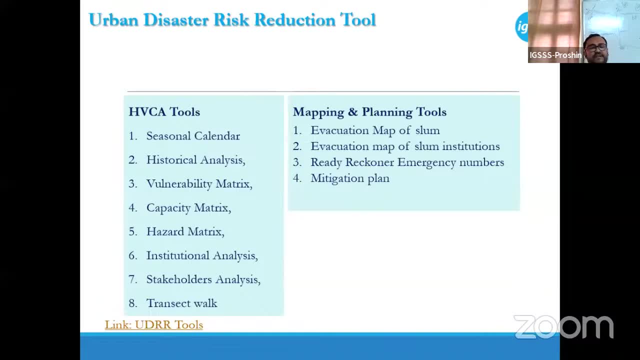 total number of households within the slum. The total percent is 34 percent. For example, the 34 percent of the families are totally infrastructure. they are vulnerable in aspect to their houses, Their household, suffering without potable water. 66 percent is suffering. 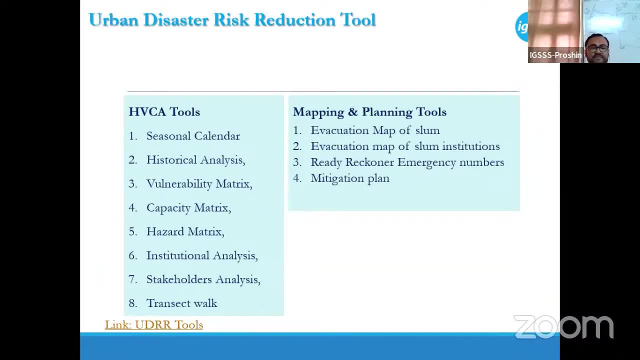 within this, Then capacity matrix. If you see the capacity matrix, so what are the capacities based on the population, That is, teenagers, and there are sports persons. are there medical persons? are there influential persons? are there government employees? are there construction: 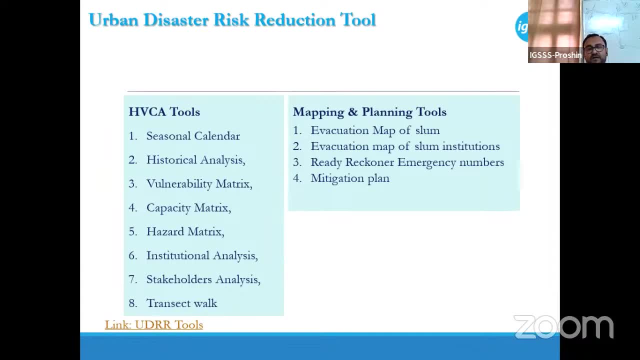 workers, neighbors are there. So these are the number of social families where these persons are belonging and then required number of the gap. what is the gap behind this? Basically, if suppose if we have 100, 15 families with sports person, but we need 120 families where sports persons are required. 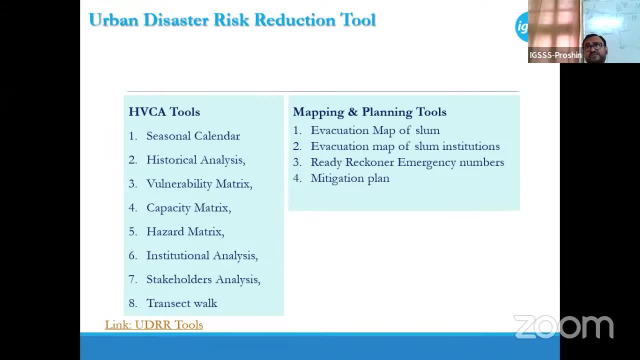 because sports persons are very much, very much active during this emergency responses. So the gap is only five. we need more five persons. So what are the? what are the plan to minimize this gap? maybe capacity building to other persons, or maybe within the slum, or maybe. 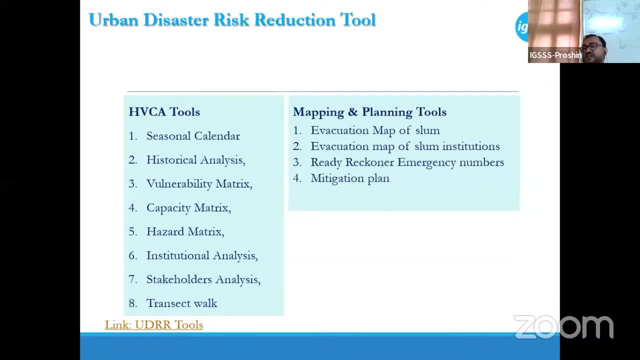 taking support from the neighboring slum. So these are the things which are coming from the coming in that what are the requirements basically as far in aspect to the population capacity of the competition, and what is the gaps and how we make up this gap. The infrastructure: 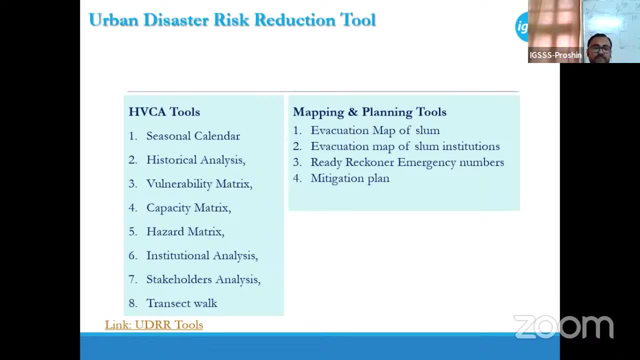 high-risk buildings: community toilet, deep well, temple, mosque, club, culverts like this. So these are the things, the same things as earlier, that what is the requirement and how many structures are required, and right now, how many structures are there and nogle structures are Fallen. we need at that level and some army departments we need right now. Can we have a lot of resources before we reach this? 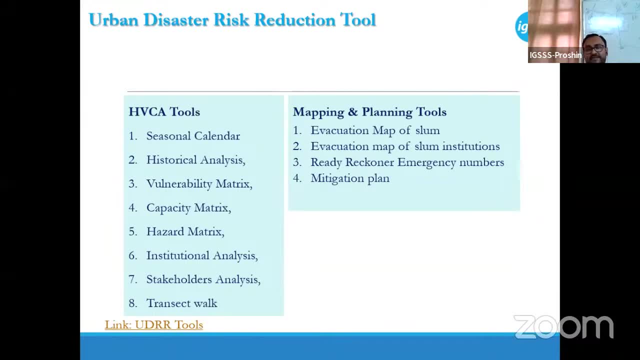 there and how we can minimize these gaps. then we come to the hazard factors. so, name of the hazards, responsible factors. we have to ask: what is the responsible factors? for example, if the hand is flat, then if we thinking about the damage, the destruction given the part situation, so mainly. 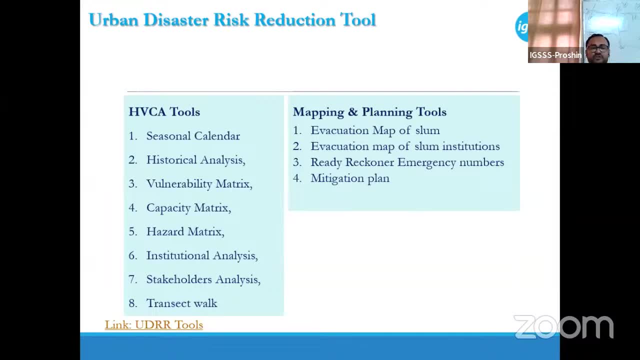 the capture houses, mainly no trains and this or distorted trains, no lying area, no rd1 system, no culvert or a distorted culvert, most music like this and prioritizations. then that is uh. within the hd, probably 60 percent says that touch houses is the main responsible factors for is the damage. 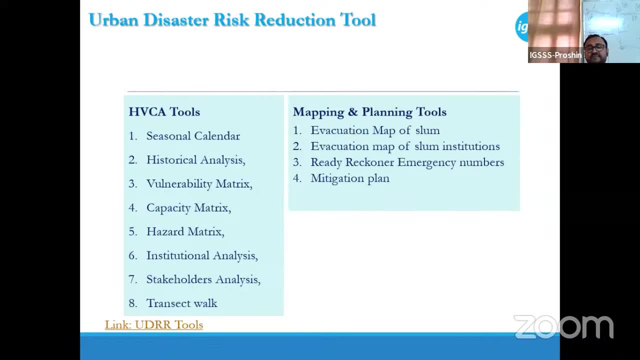 and distortion during the last situation. so this is the hazard matrix where you can understand that which one is the more important factor? uh, which which is responsible for the distortion of the slump, the we do the flux, then, uh, we are coming to the incident and analysis. this is: these are the institutions, uh, within the slums. so the number of the institutions. 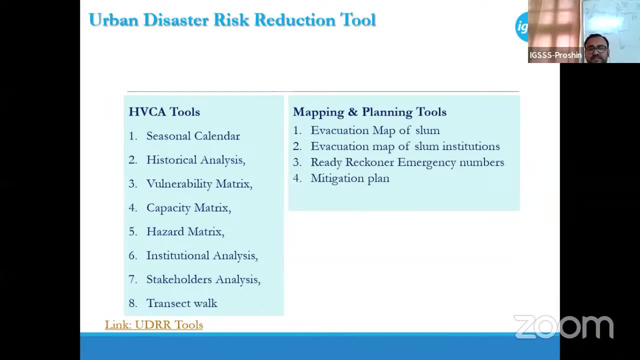 how many are here, what is the distance for the slump and the relationship is for with the slum members and the good of them? good or not good? then, participants, you know how many males are doing there, how many females are going there, how many transgenders are going there and a bit, uh, availability. 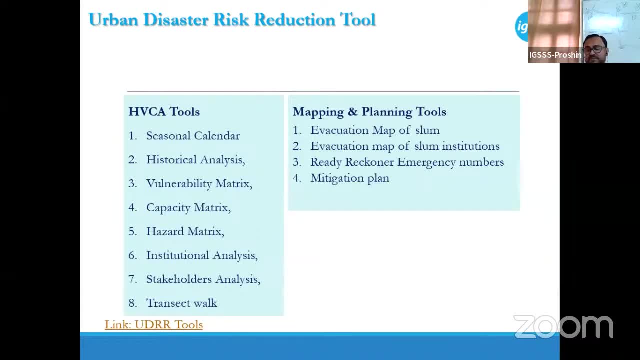 of the services during p general availability service, with that generally, and if it is an emergency situation. so what is the situation during emergency and post emergency and even immediately, uh, a couple of hours and a couple of days, pre-emergency, after the rd1. so these are the things, uh, of institutional analysis and then a transit. 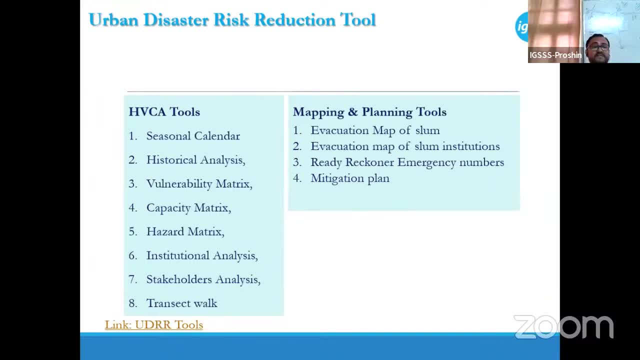 truck will walk the overall village. any aspect to our climate change. for example, the lack of back doors in most of the houses we observe and no windows in the back. why it is needed? because if we, uh, it got a slump fire, then, uh, we must evacuate, so we need a back door of winter. 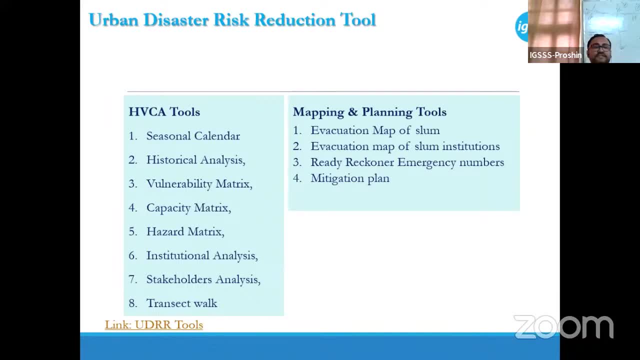 uh back building but nothing is there. the lack of staircase in outside of the building for emergency. so this is the thing that the secondary observation is: maybe some uh related to the departments, related to the local beauty dealers, for example. community members have not created a rapport with the school. 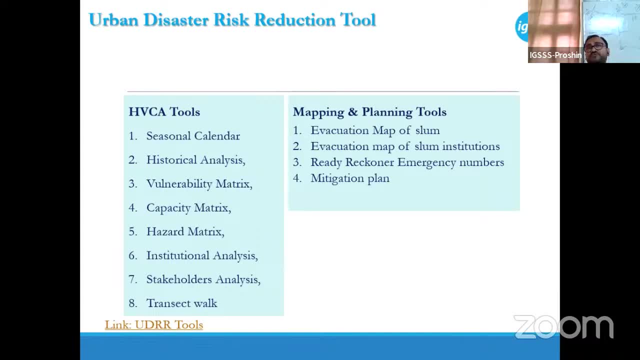 authorities. uh. so as they will not, they could not use the the uh school building here as emergency shelter during the margins and the stakeholder analysis. these are departments uh, at their prioritizations with departments is very highly prioritized to play a good role in the emergency. 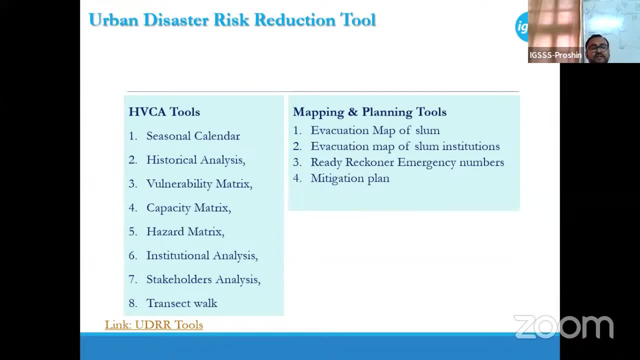 situation and the modern. these are the community loops. so the these are eight tools which we can understand, uh from this, uh from this quality mapping tools. now again, come to the presentation. now the mapping tools, now the code. now this is the. there are two, two different maps: evacuation. 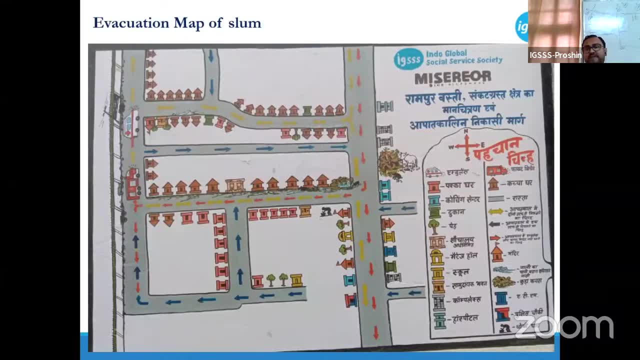 maps. what is evacuation map of the slum at the evacuation map of the slum institution? so this is the evacuation map of the slum, basically how to evacuate any emergency, for example, if any cyclone come, if any fire or slum fire happens, if any uh flood, uh water loving happens. these are the red. 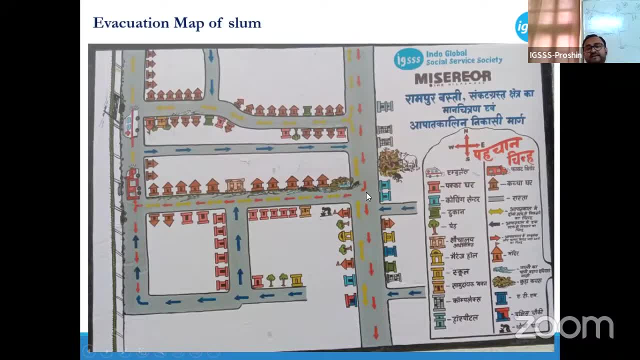 colors. these are the evacuation route and uh, these are the routes where from, uh, where from and uh fire truck, maybe an ambulance can enter with the slum. so these are, uh, the draw and wall painted uh, within the slums, which are every slum for the community itself. and these are the. 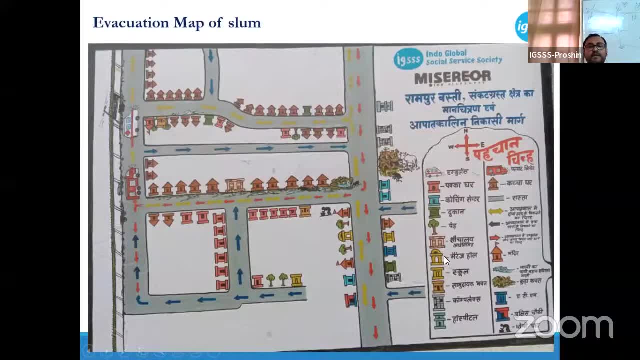 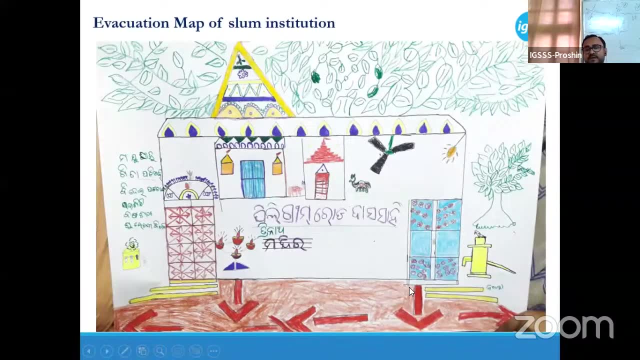 regions and regions. some of the things are presenting here. and then, if you saw the institutional evacuation of the mandi temple- so this is the main gate, so this is the way to evacuate- is the land, so they are coming, uh, to this level if a fire or if anything, uh, 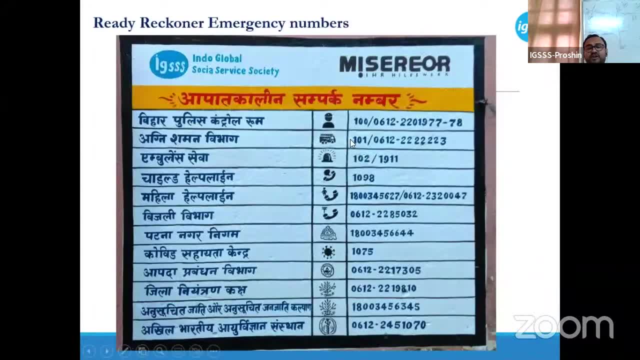 emergency happens, then this is the ready economic emergency context and this must be in all the uh slump walls, in this slump slumps in the walls so that emergency- because it's also the logo- is there, so that uh, uh immigrant person can understand the numbers, can know the numbers and they can drive. 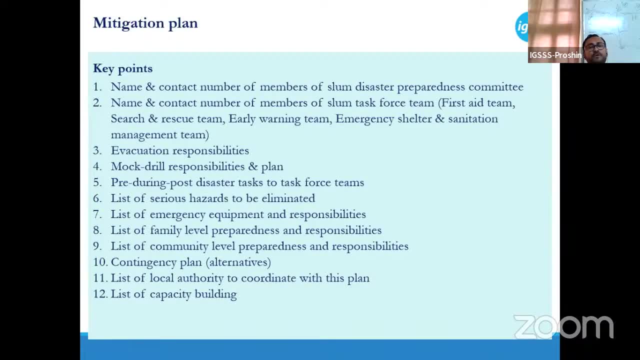 it to the emergency, then the key forms. so basically uh, mitigation plan is another very important for mitigation plan uh. but there are some key points uh which pass through the mitigation plan. name and contact number of the members of the slum uh disaster preparedness committee. name and contact. 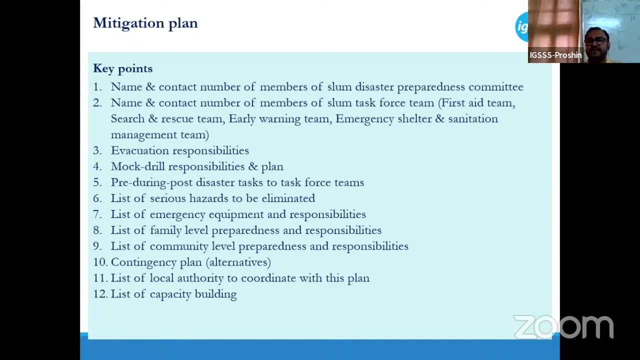 number of the slum: uh task force team. uh, there are. there are at least four task force team meeting in slum. maybe first aid team, search and rescue team, unvoluntary emergency intersection paramedics. then evacuation responsible to who take the responsibility during the evacuation to the emergency happens in the slum, then module responsibilities and a blockchain plan. 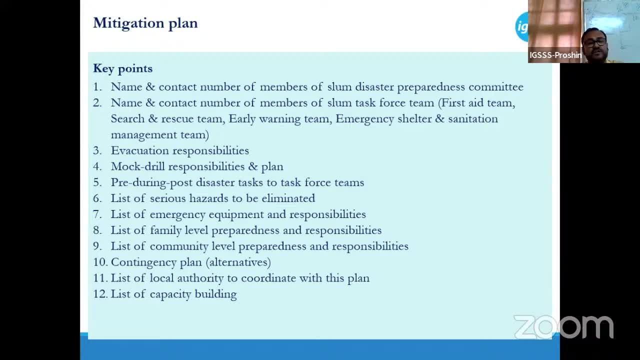 then, uh, pre, pre, during and post disaster tasks to the task force team. what are the domestic, during and post your tasks may clearly define, within the mitigation plan for the task force team at the release of two years, hazards to eliminate. what are the serious hazards? for example, there is a tilt on. it's a very serious hazard because he's not. uh, what with fire? so 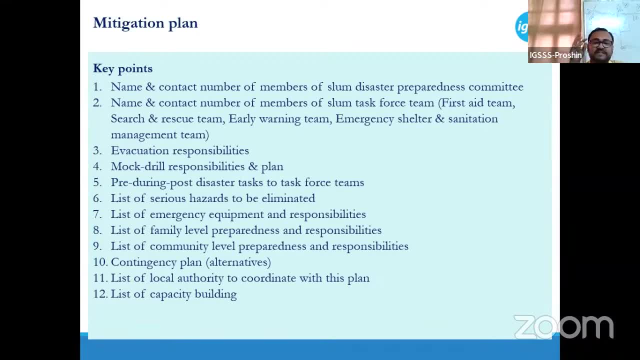 it can be positive: uh slump. so what are the serious hazards must be identified written in the mitigation plan: list of the emergency equipments, what the emergency equipments are there under, who takes the responsibility to use this emergency equipment for the emergency and the list of the family level preparedness and responsibilities. 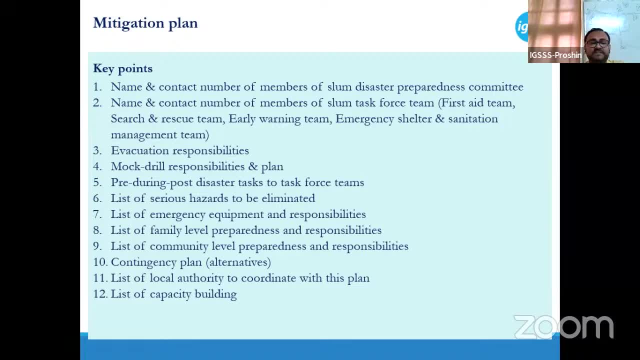 list of the community level preparedness. who takes the responsibilities then continues? plan alternatives gives a task posting. one of the task force team members, um, got injured during the evaluation of rehabilitation. so what is the responsibility for this case? uh, then, uh, list of the local authority to coordinate with this plan. 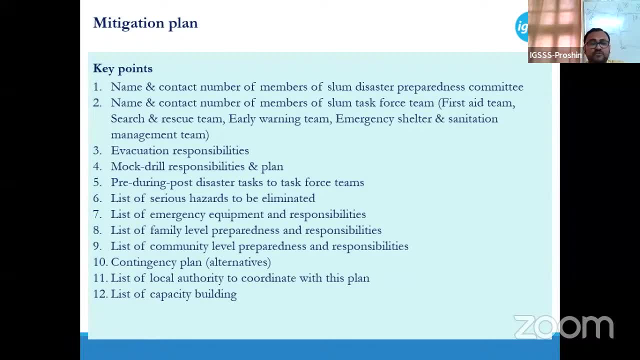 who are the local authorities, who will be from. from them will immediately support and the list of the capacity within trainings. what are the trainings required? so this must be integration plan. after preparation of this mitigation plan, this must be handed over to the local individual as 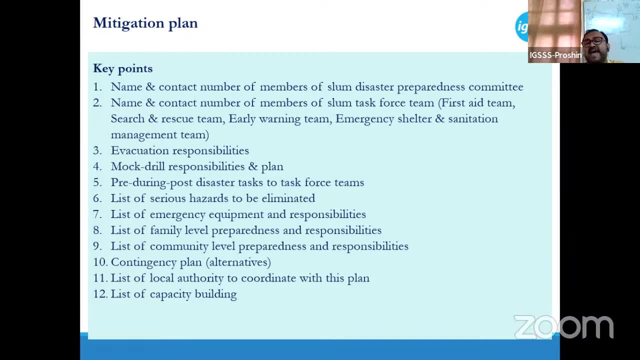 municipalities and the departments, uh, so that they can have an amount of the things and their roles, that this is the mitigation plan of aslam and we must engage with this because, in this sense, the Racism, rent and voter compute. that is the, uh, the role and responsibilities. 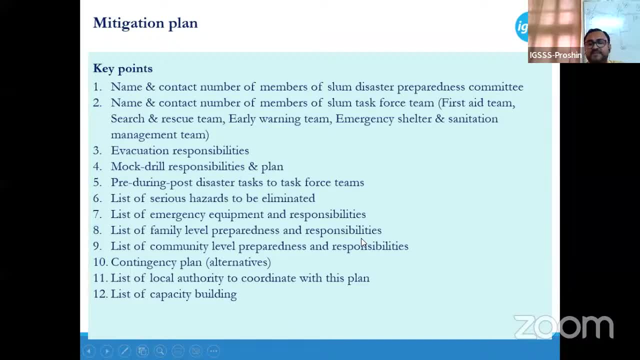 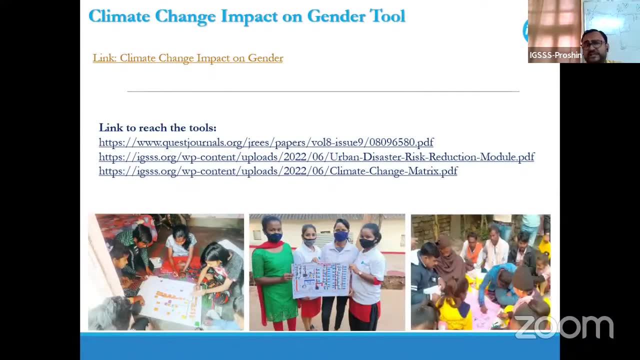 part their roles. also keep very much clear about that is that, uh, which departments will do what? the things we'll do, these are the things. so this is mitigation plan. now the third and the last two, that is, climate change impact assessment tool of gender. so if we see this tool properly, 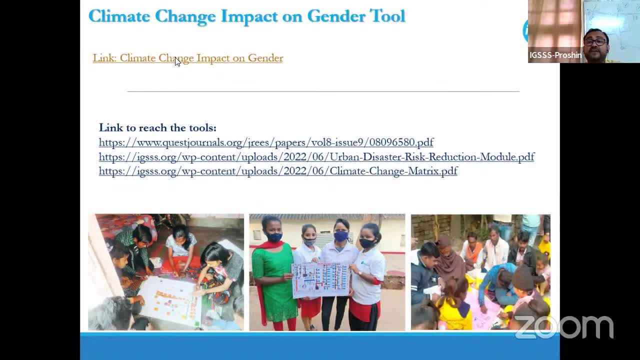 basically, this is basically a tool which can access the impact of gender only, the impact of into the climate change. So basically, we can do this. we apply this tool with five groups: One is for men, another is women, another is elderly, another is adolescent girl, another is adolescent. 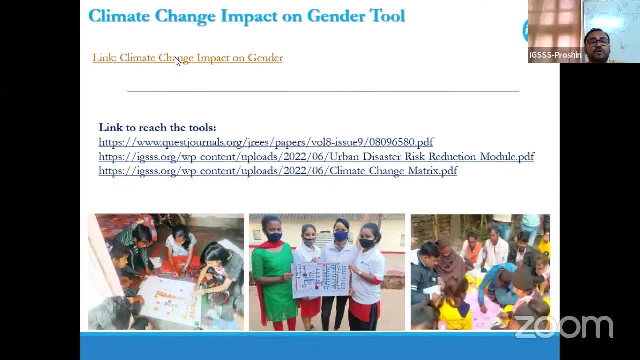 boys. There are five groups in each slum So we can add same as FGD, So we can take the 10 to 15 women speakers from the slums and then we will do this. Then there are different cells here. if you see the tool, that is climate situation in the year. So if it is extreme climate situation, 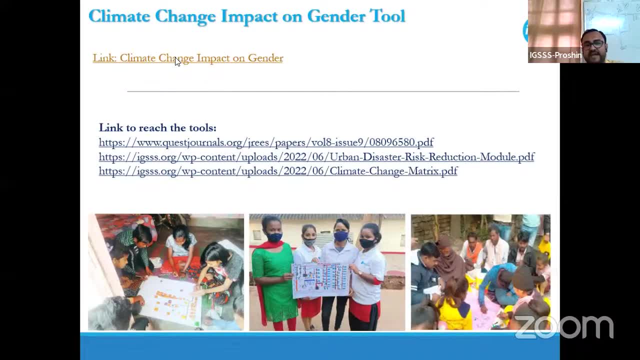 here, if you see this. So if there are two categories, we will assess: what is extreme climate situation, what are the things and what are the things for without extreme climate situation. That is normal situation, usual situation. So if we see the extreme climate, 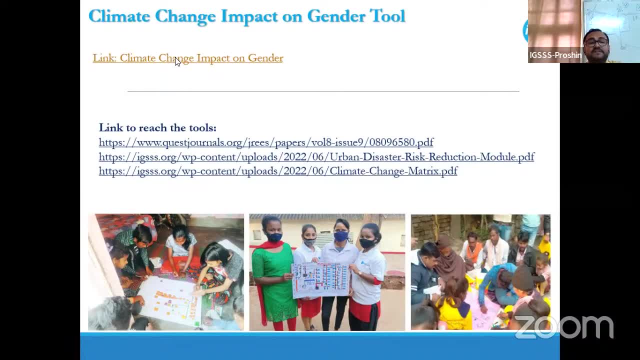 situation, the moms. we will ask them: what the moms? which months in a year you are suffering extreme climate crisis? Then what are the natural accessed by during this extreme climate? Is it a flat? Is it a cyclo? Is it like? what are the things? 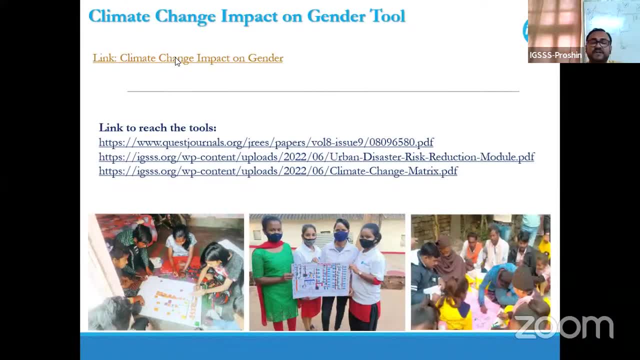 So we can understood this month's sale from the community with this questions And then we will come to the next part. next part that changes in the daylight. So the daylight is categorized in three different sections. One is: what is daily health? What are the challenges were surround? by these problems that are different each month, And the operational problems- they were almost the latest易 sloweding. Otherwise there have been more. So that means in the mostcontinent sensibility of this climate could be done, But in the last few months 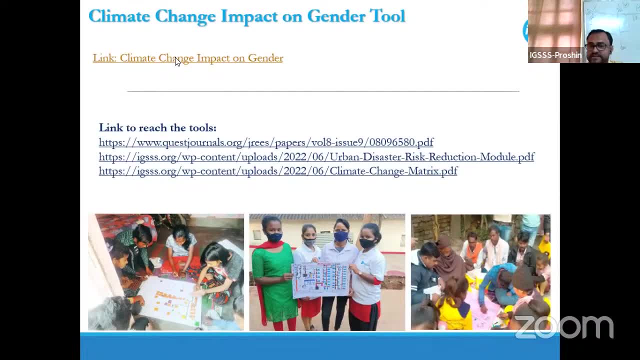 different the harm And these kind of issues. people have to be addressed. So, for example, they are facing in daily household chores what are the challenges they are facing in the livelihood and study during extreme climate situation and what are the challenges they are facing during daily self-management and other things during extreme climate situation. 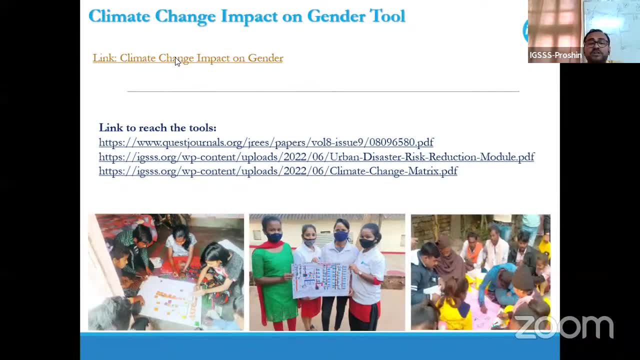 So if we say: ask them that, what are the tasks undertaken by you in daily household chores during extreme climate crisis, ie when there is flood, what household chores do you have to do, then they will express their feelings, express their figures, maybe tangible, maybe. 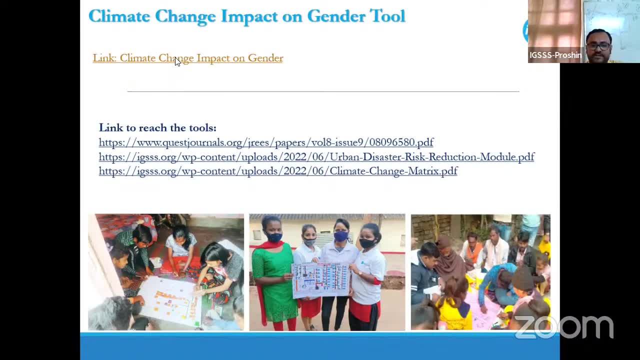 intangible whatever. So everything will be noted down and then after this, we will analyze that, if the tasks in household chores are clearly identified and noted, and analyze gender issues from this note and then how they are faced in daily household chores. Okay, Okay. 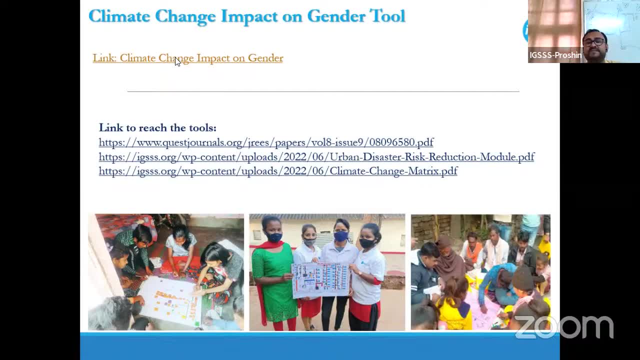 So this is the things, the same thing we will do for the livelihood and study, for the daily self activities and other things. For example, in Delhi, women applied this in one of the Delhi slums. then the women said that the water is a very difficult challenge, a very high challenge for them, because drinking 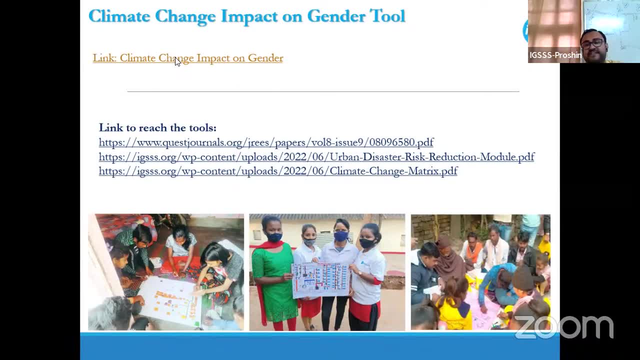 water is not adequate. they do not access the drinking water during the summer times, that is, the heat wave days, And so this is the challenge, This is their feelings, this is their understanding from this, and we will note it down every day. 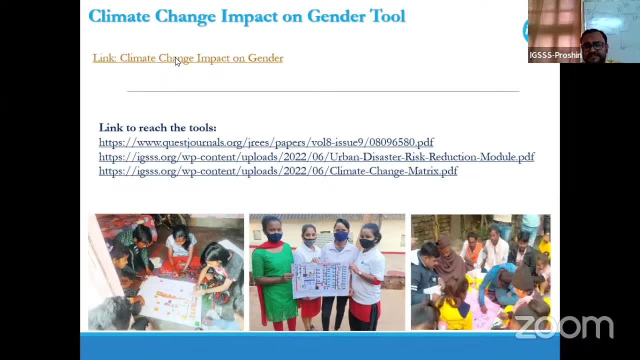 And if we say that, why you are facing this challenges, then they are saying that because water is our responsibility only, because our male members of the family do not want to take this responsibility. because if we are connected with the kitchens, because women are connected with the kitchen things, so water is totally entire responsibility of. 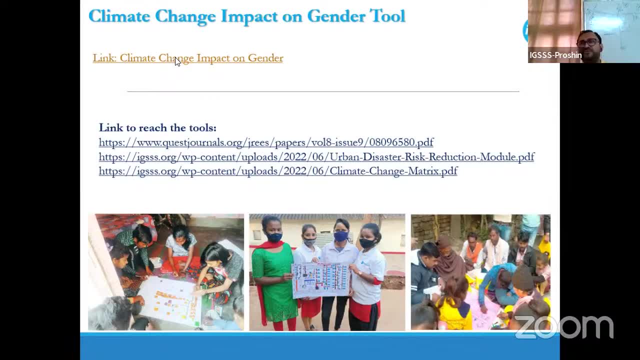 women. So this is the main gender bias thing. Why don't you Men are not participating in this, Why This is the only responsibility of women? So this is the gender bias thing We have to identify from their expressions, from their body language, from their statements. 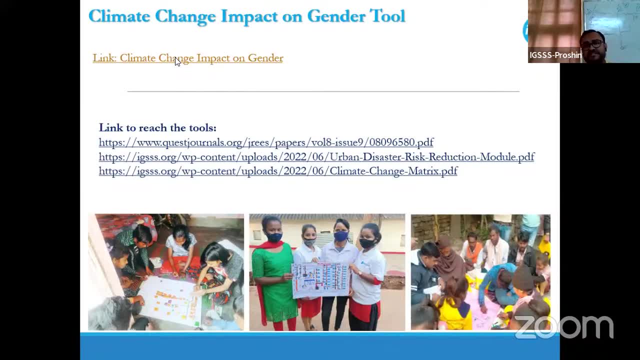 from their posture gesture. something like this: In one FGD, one women cried. this cry because they are saying when we are asking about their self activity, so they are asked that they are. this has been a lot of time using their words, their very big mainstream and health support because they have no sanitary pad. 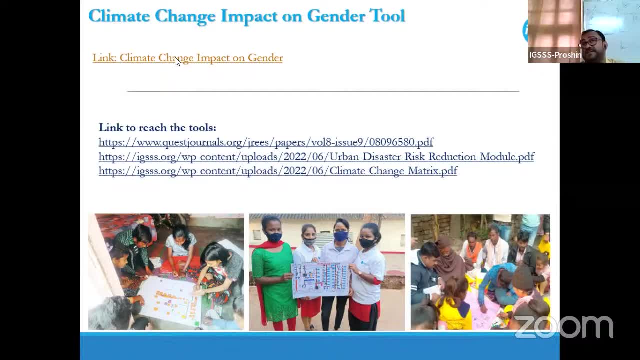 They are not using this act because they do. this Sanitary pad is not accessible for them And their husbands are, because they are not very much open to this kind of things. We can have one. This was analyzed. This was analyzed from a remote village of a bar street in the Grama Kutai land. 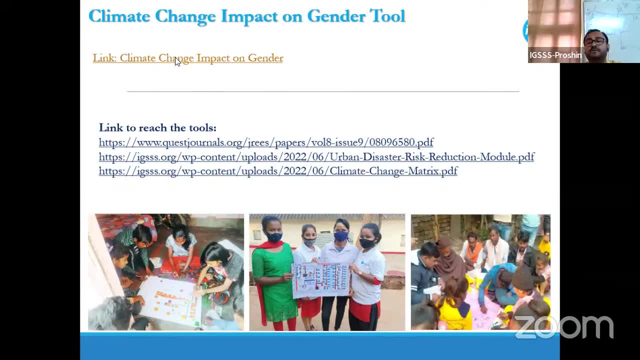 So this is the thing, This is very important, because this is a very important thing, So this is a very important thing, So this is a very important thing, very important things, very important information. we can connect from this. if we see their posture, gesture, their statement, their impressions, everything is very much important. you are. 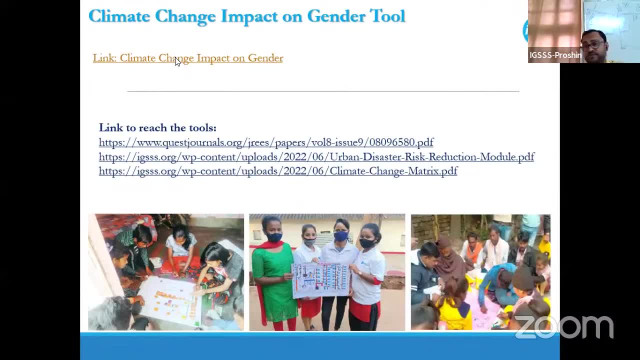 going to be searching, if we understand the gender issue, for this. so this is the thing that. apart from this, we will take some information if there is any traditional coping practices and if they back to this action, what are the things and how they must they help this? uh, these traditional 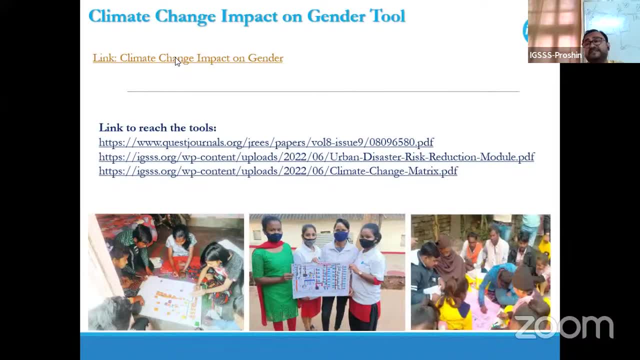 coping practices helps them. and what are the action points? what are the things? uh, what are the things? but the women think that one of the action points must be there to minimize the gender issues, to minimize the gender pains, uh, and to have a good gender sound action plans. 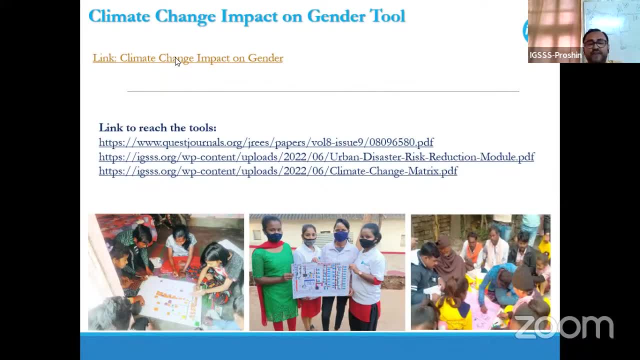 or the monetary additions. so this is the tool, very important thing which we can understand: the gender issues, the faculty gender situation, either in the slums or it can be used in the religious also the same thing within, uh. so if they're not, if the normal solution is against, no climate emergency. 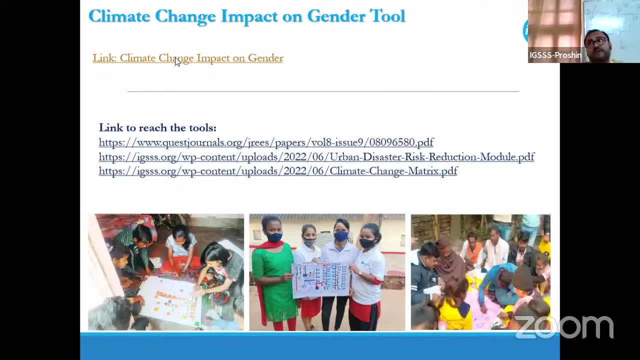 is there. so we can also get a lot of different issues when no climate emergency is there. so this is the tool which can accept the climatic impact on gender. so then come back to the uh presentation. so these are the tools which i am discussing here. so here the links are given here and 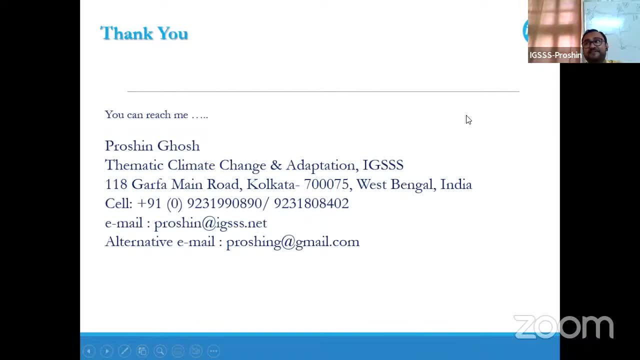 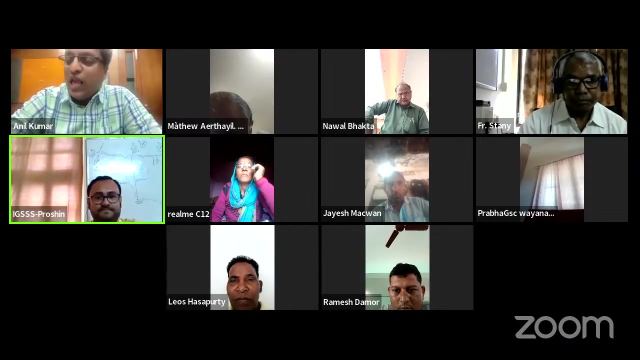 no more, because, uh, it's very heavy things, because you know that the tools is not very easy, i understand and, uh, in one session this tool's uh discussion opportunity is really heavy. so, thank you, i mean to give you this opportunity, uh. so yeah, thank you, prashan, it has really been a technical session with cogs. 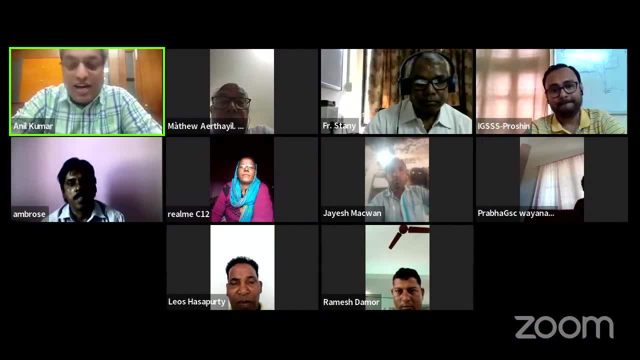 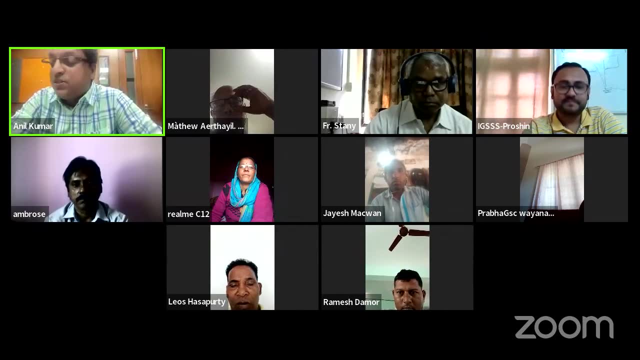 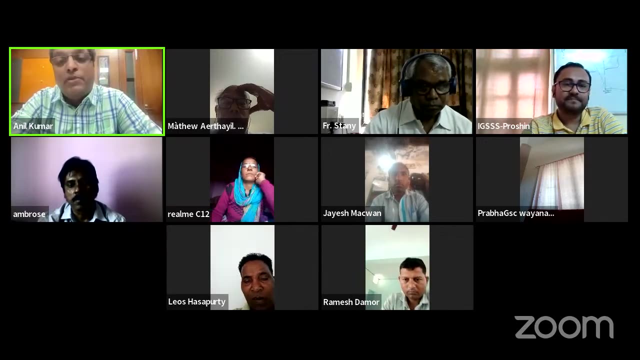 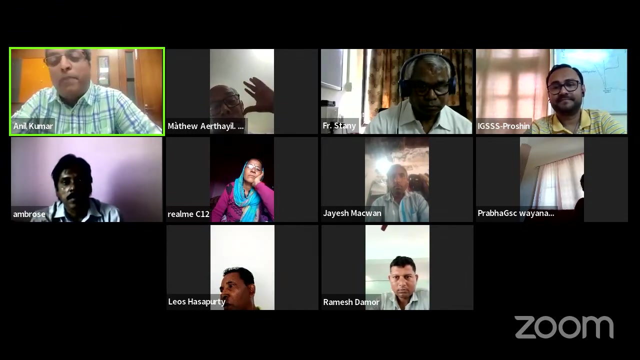 and it has been a bit heavy too. uh, you looked at climate change vulnerability in the climate emergency in the urban context, especially with regard to slums, because you have shared tools and guidelines which can be used at the community level for developing climate action plans, especially in the context of slums. friends, it has been a very power packed sections since morning. 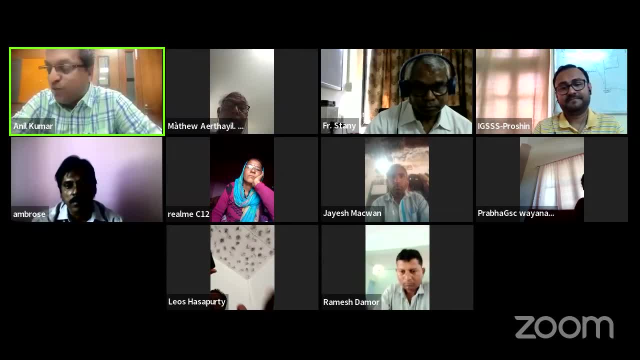 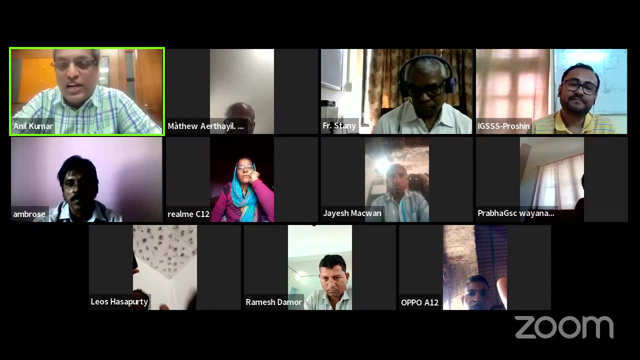 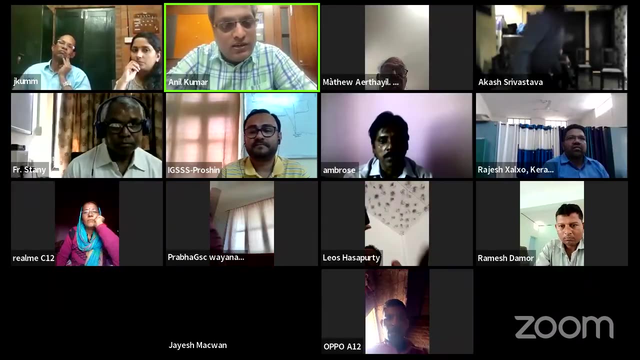 due to the positive of time we could know our presenters, who are technical experts, had to rush through their presentations. however, we will be sharing the inputs. they have shared the share also the presentations they have presented today. friends, now i will open the section for question and answers. 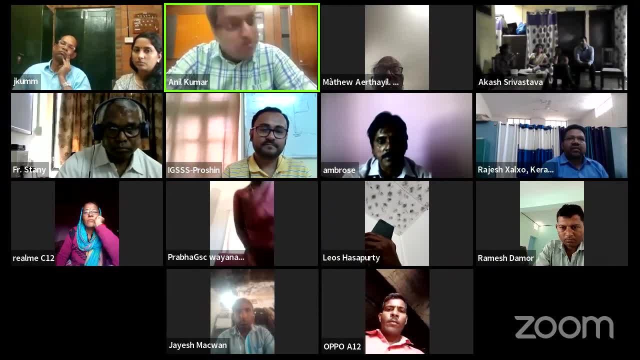 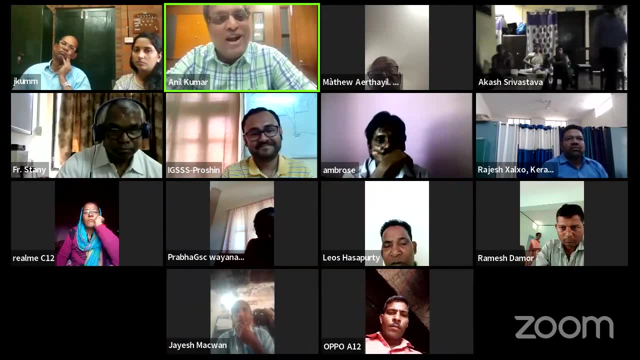 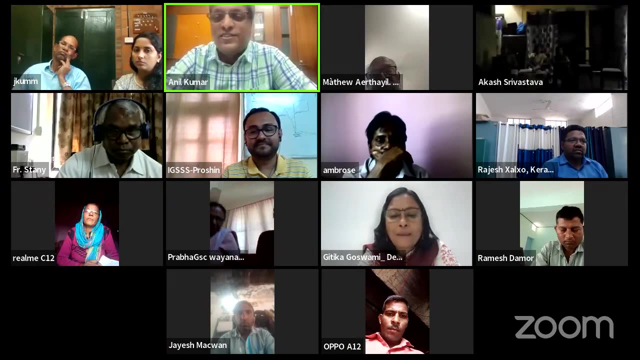 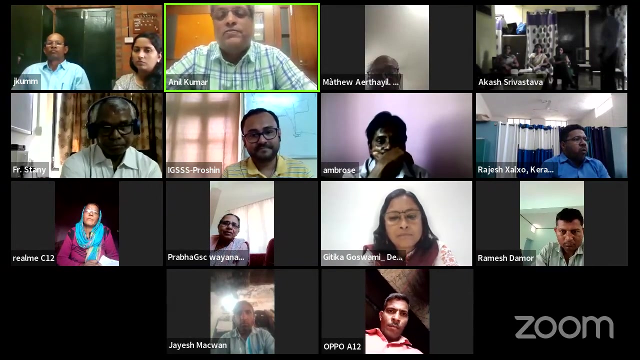 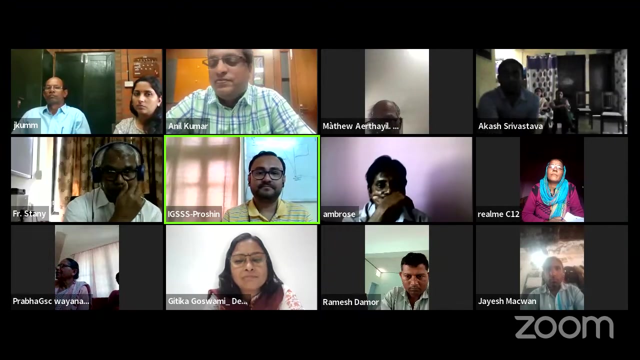 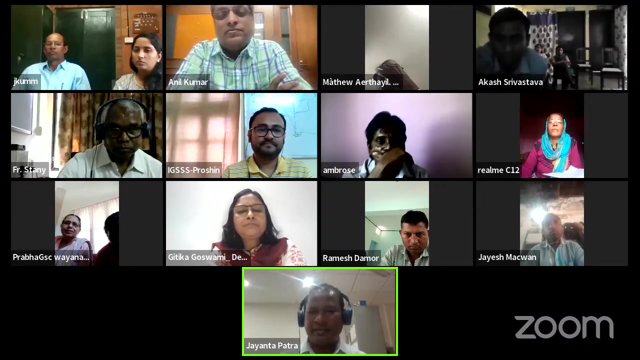 our speakers are comfortable, very much comfortable, in hindi. prashin and gidiga are good at bengali too, So you have wide choices with you. kindly ask questions and I will engage Jayanthak also to continue with the session further. Thank you so much, Anil ji. it's very, very enriching and let us invite the questions. 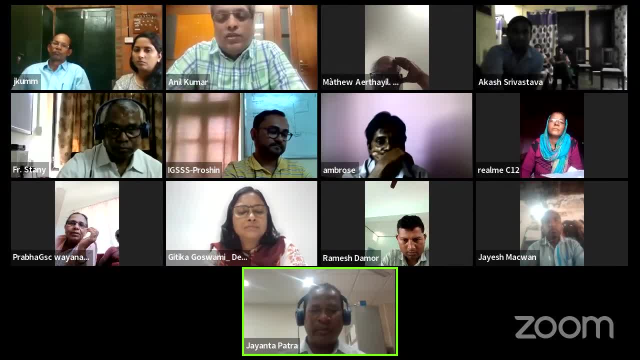 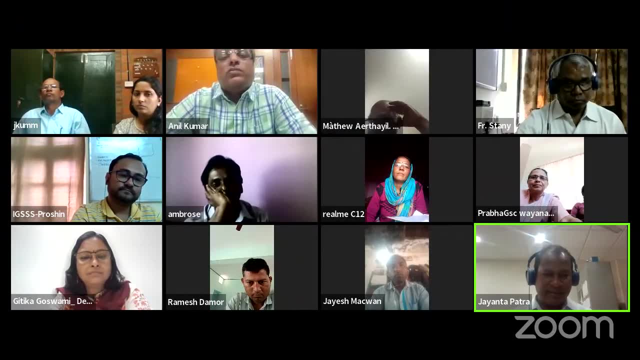 and also, if you are not able to ask also, you can write in the chat box. we will monitor your questions so that we can make it reach to the panelists. So is there anybody who can Ask the questions? any doubts? clarification. 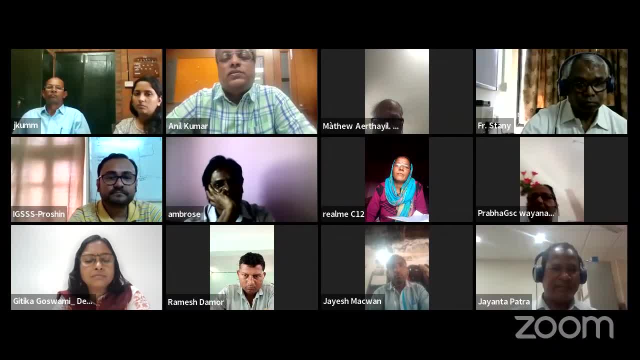 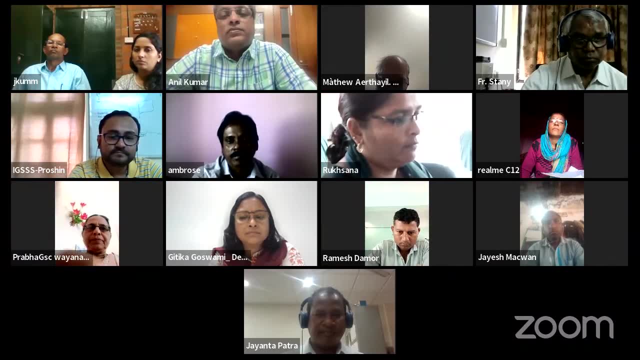 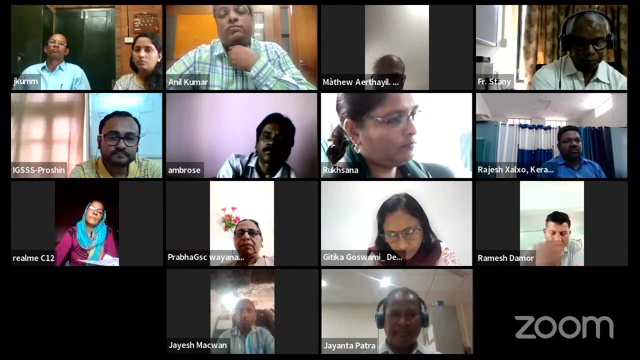 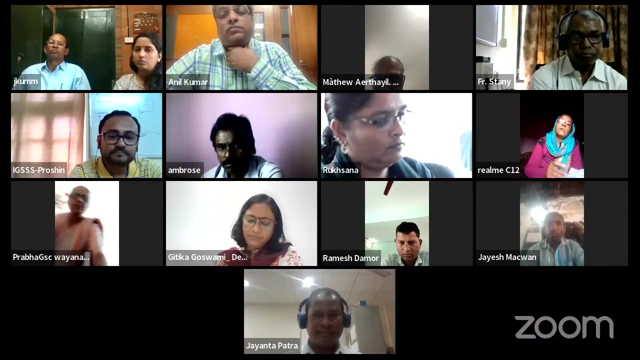 Jayanthak sir, this is Ajit from Bihar, Patna. My question is that Lokmanji is working here in seven districts in Bihar and mostly our interventions are with landless people. they are mainly residing in the near outside the village, near canals and all this. 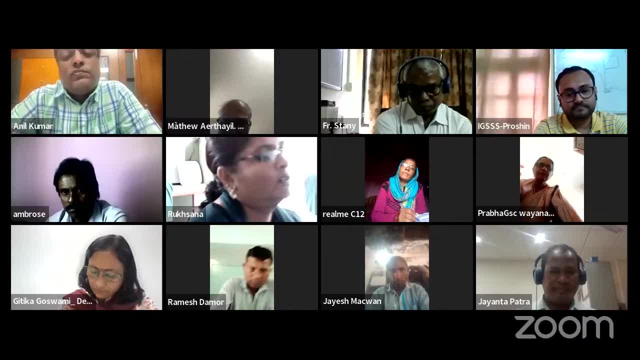 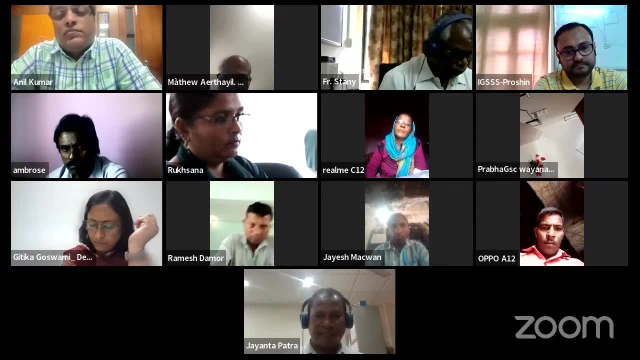 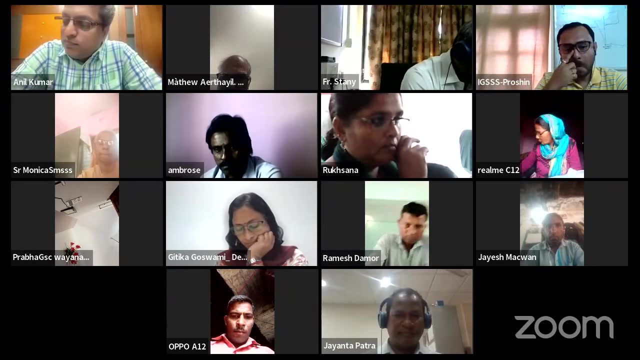 So, as we take this climate change as one of the major activities in our Bihar, Lokmanji Bihar- so we find very difficult to make them understand that they are the vulnerable ones. So what are the things we can do as a vulnerability mapping? 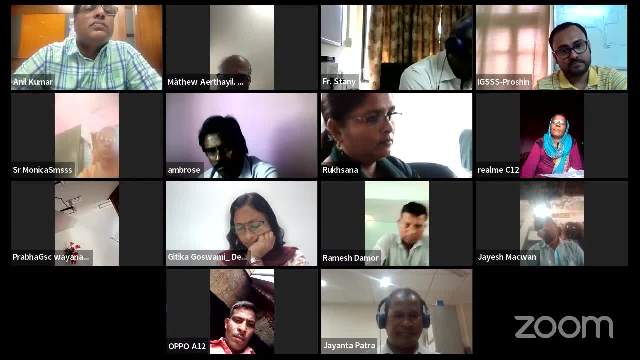 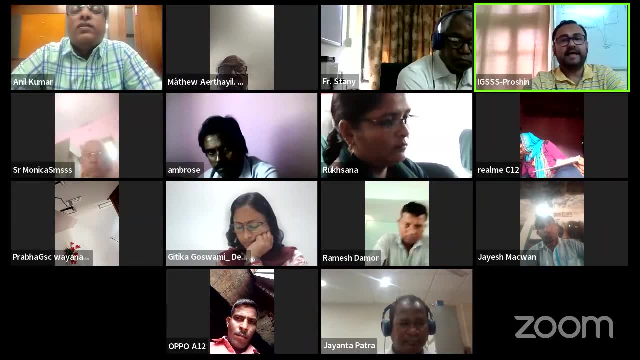 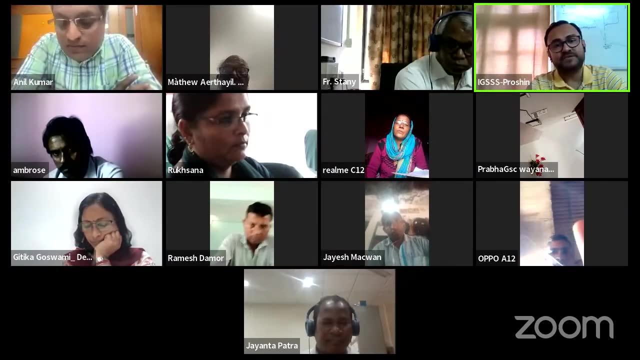 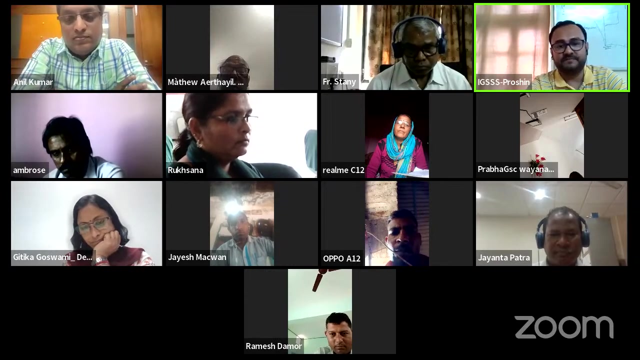 So maybe some of the process or some of the tools you can share, Prashant, would you like to come in? Yeah, yeah, yeah, Actually, before preparing the tool, there must be a rapid rural appraisal, rapid rural assessment like this, where we can go rapidly, just see the village and then we can talk. 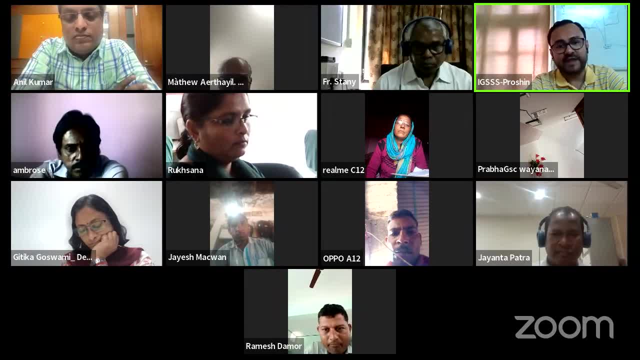 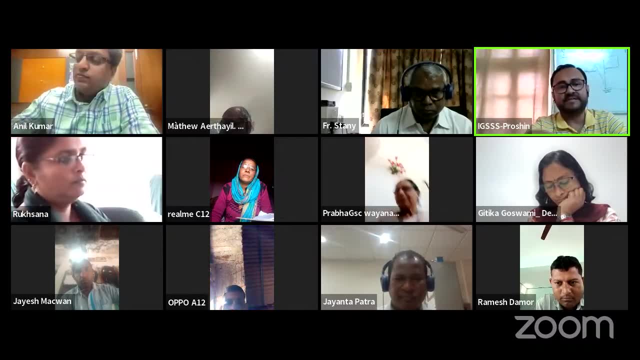 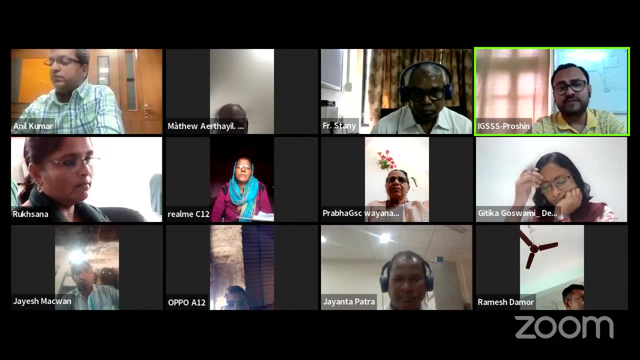 to the community, what are their requirements, what is their challenges, then we will prepare a tool to assess them. Okay, Thank you. So if we can assess the vulnerability matrix like what is very synchronized in the vulnerability matrix which I have shown in my presentations, and not only vulnerability matrix, also we 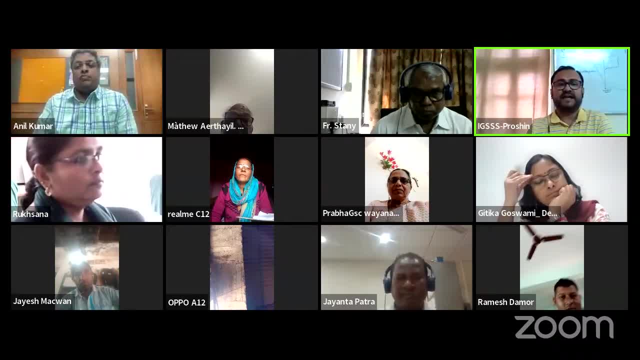 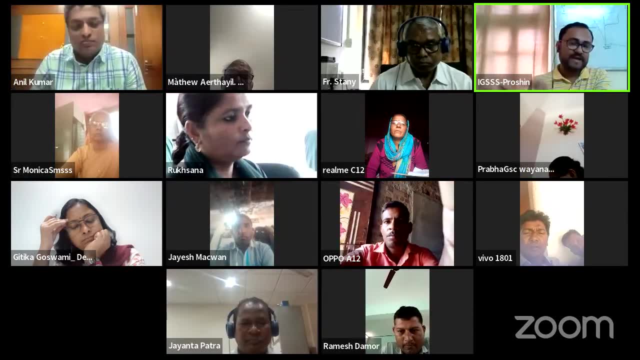 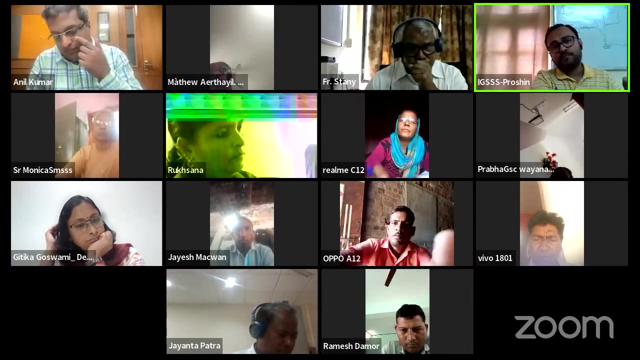 can do the capacity matrix simultaneously. otherwise we cannot assess the vulnerability, because not only vulnerability is the main part, the main part is also capacity. So if I have capacity and if I have five capacity and I have 10 vulnerability, so how we can enhance our capacity to cope with 10 vulnerabilities? 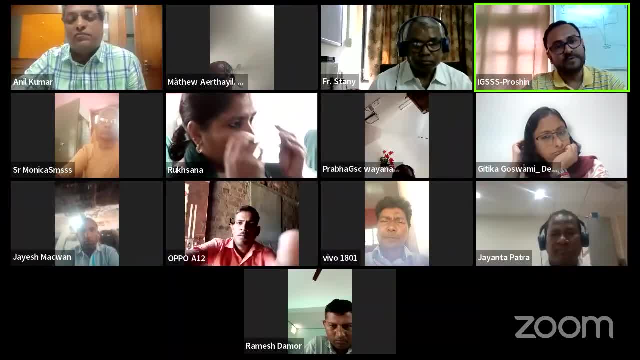 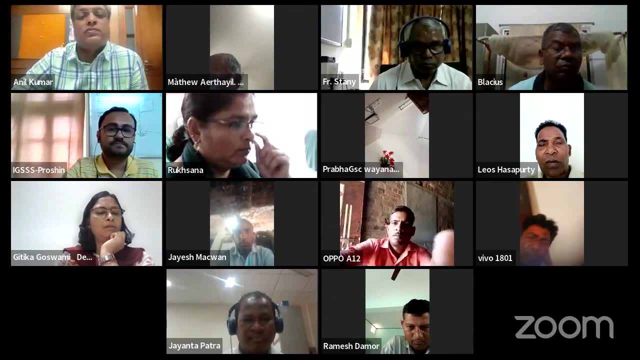 So this is the things we have to do. These are the homework we have to do before we go with the tool within the term. Okay, Thank you. I just want to add here, Anil, if I can: Yes, sure. 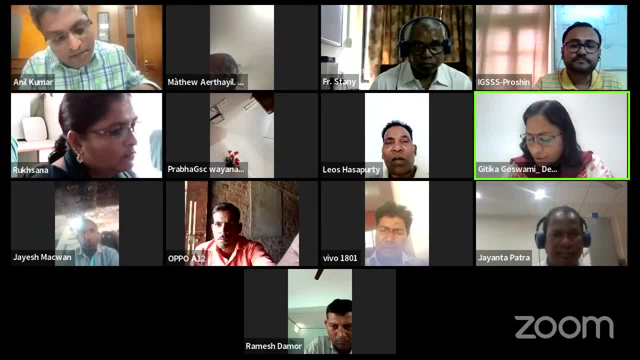 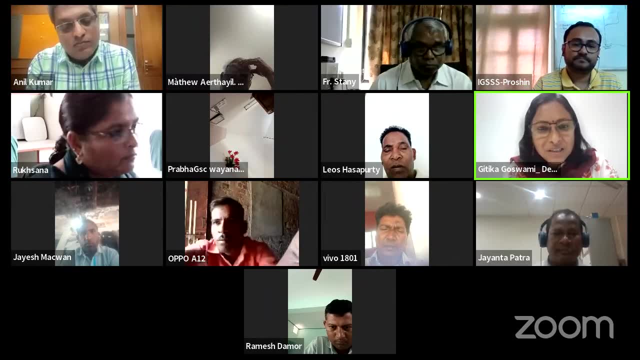 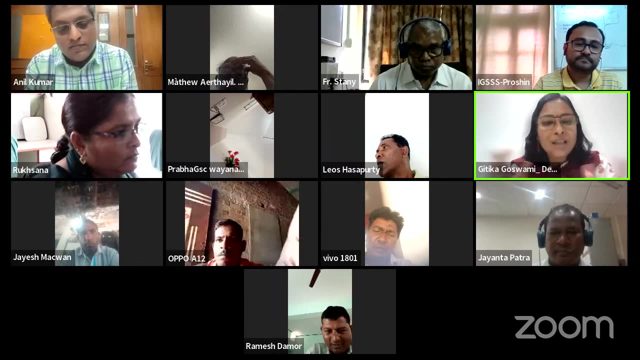 Yes, So thank you for this question. I think very relevant, First of all, that community doesn't understand the climate change and they don't know they are most vulnerable. So I think it's very important. I think the first thing, if we really talk them in this language, this is difficult for. 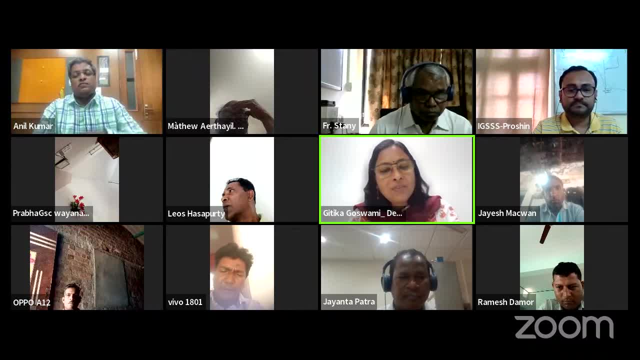 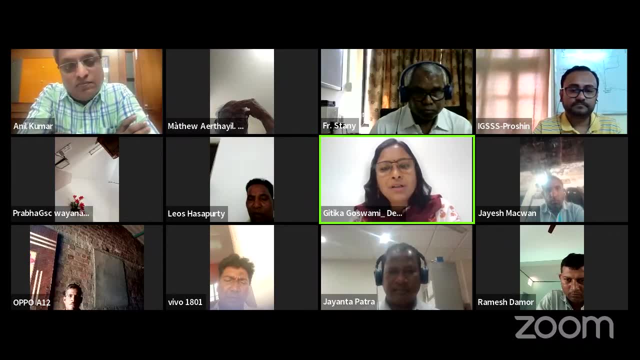 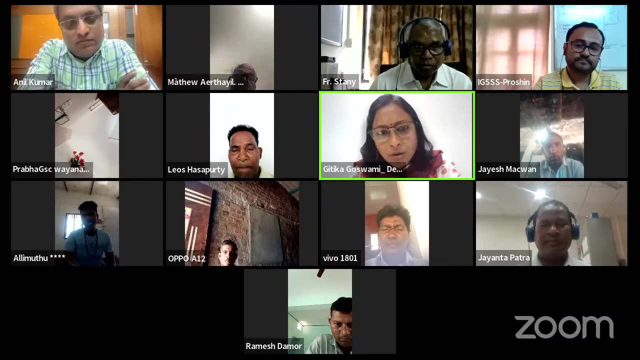 them. but if we talk them, talk with them in their language, I think they, in my experience, I see they know much more than what we do. I mean, our experience comes from their experience. So the first thing I think we need to, what we need to see about, you know, asking them. 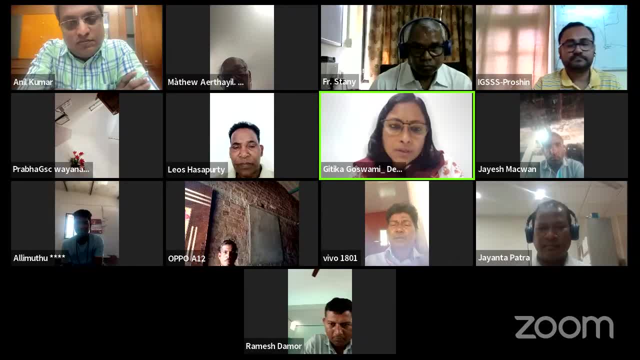 their problem and asking them what was their like 30 years of experience. I think that's a very important thing To think about. okay, you know these people who have been in the area for 30 years or 40 years back in that area and what they're missing. 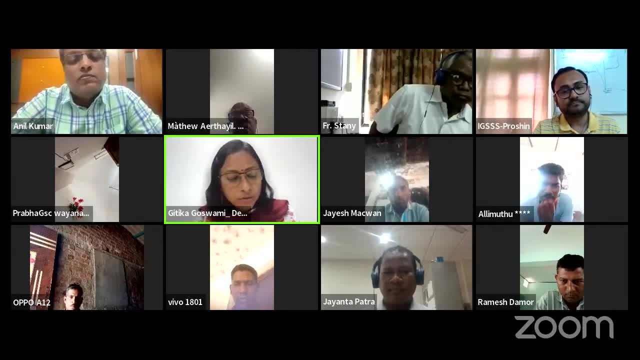 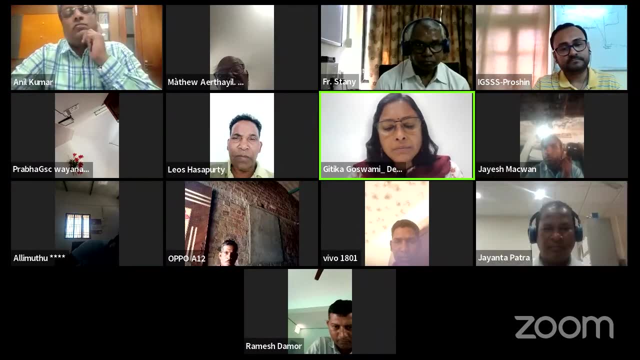 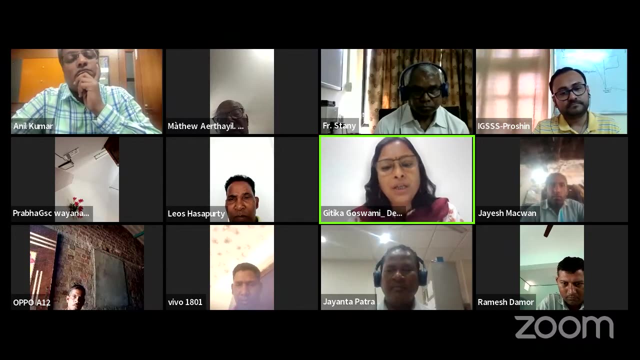 So many cases in West Bengal I have seen, and also in Bundelkhand I have seen, the housewives. even they said not the climate change word, but they said the soil is dry. They said the first thing we need to do, we need to get rid of this heat. 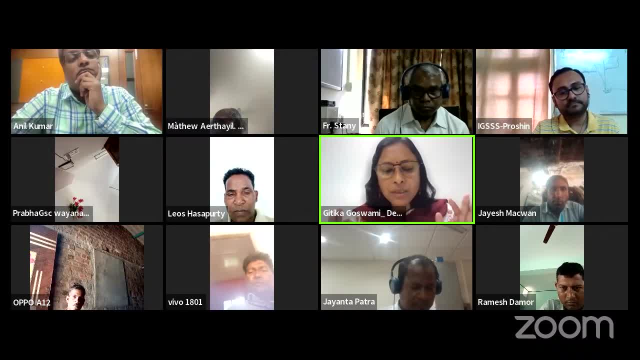 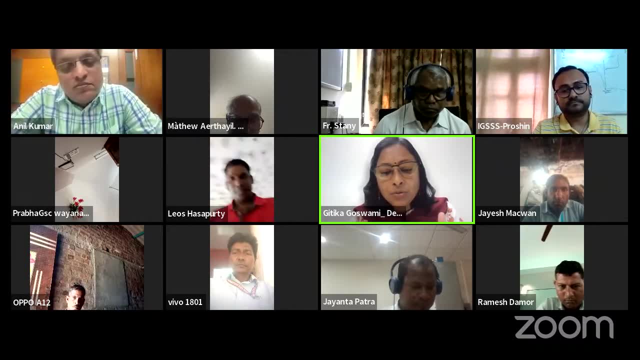 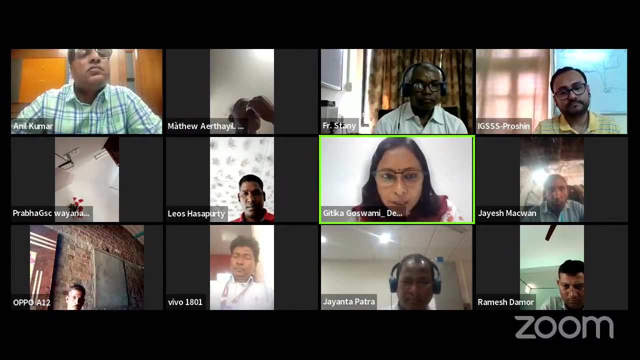 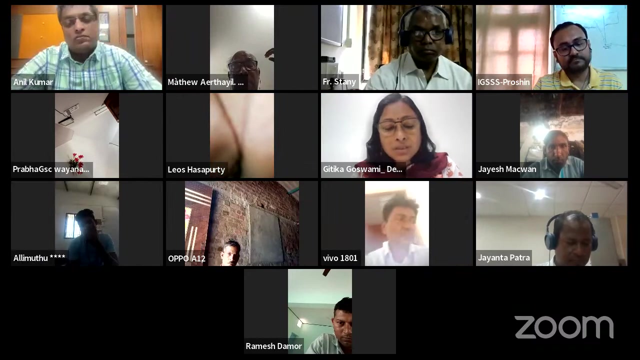 We need to get rid of this drought, We have to get rid of the drought, We have to get rid of the drought, We have to get rid of this drought. then they say, which is basically soil moisture dried up, which is temperature increased, which is sometimes. they say: 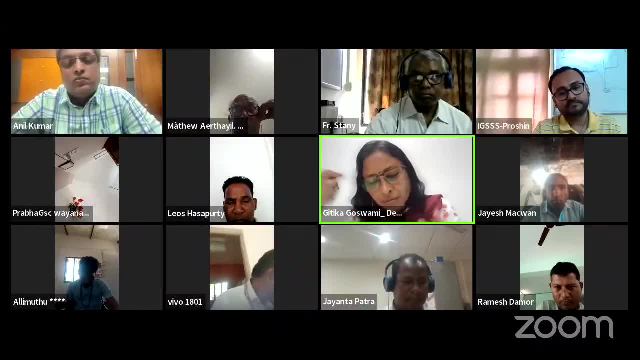 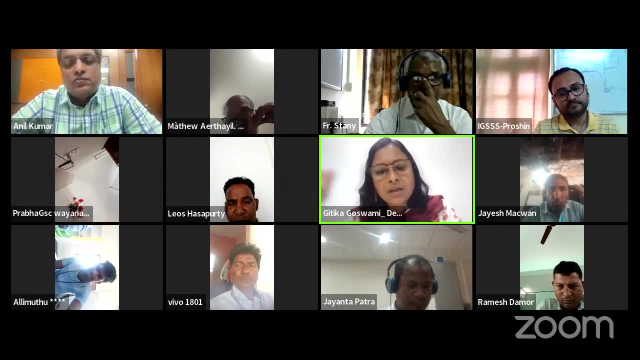 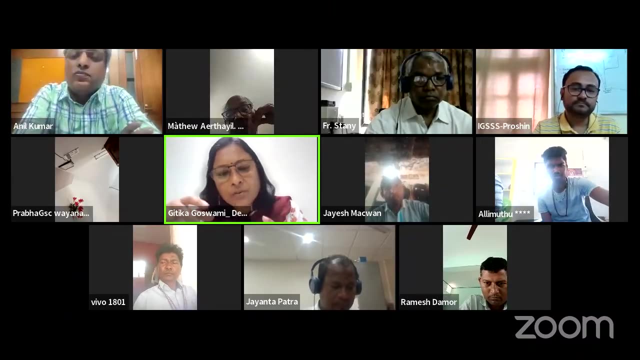 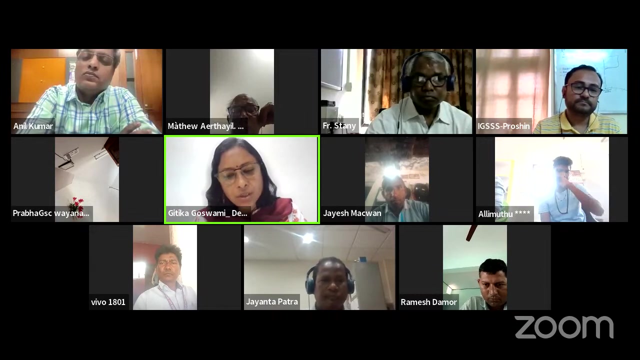 so this is all showing that heat increased and that's basically climate change. due to this, this happens. so one is that you need to talk to the local language and ask them: what is the problem that they are facing and what was the problem? what was there in those areas? 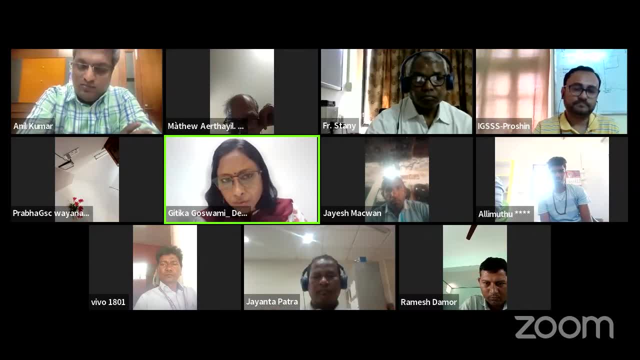 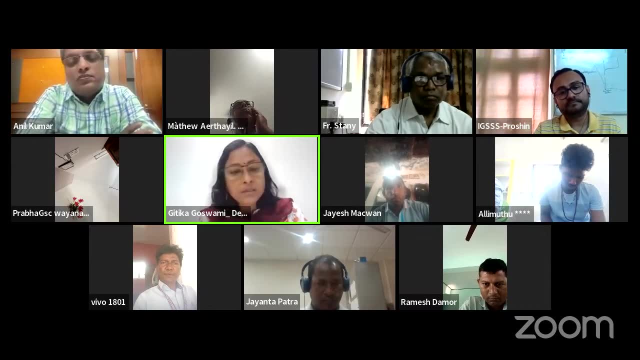 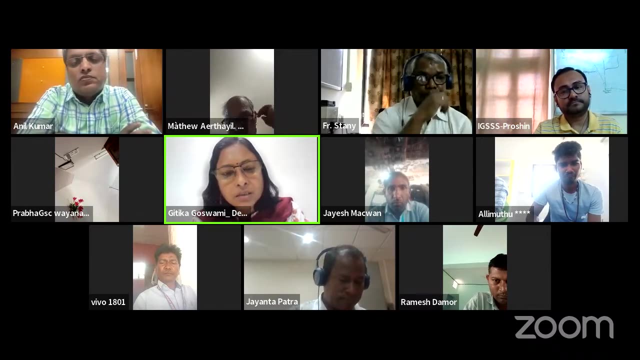 30 years back, 40 years back, 50 years back something, and that is why they are saying they will understand what changes have come second, if you talk about landless people. so I would like to really know what exactly you are working, which of the sector? 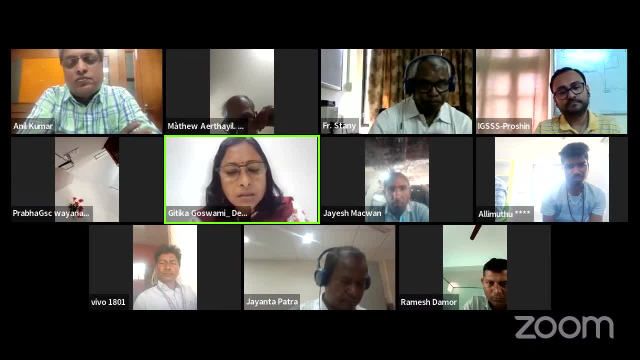 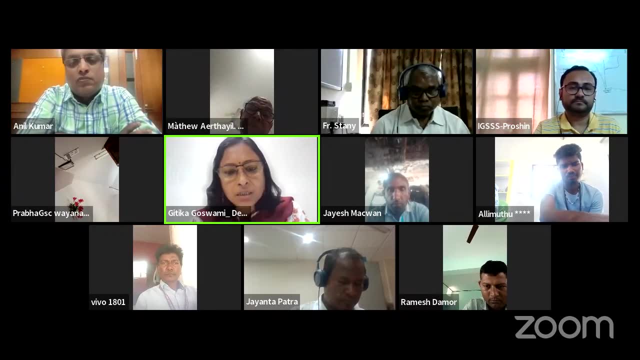 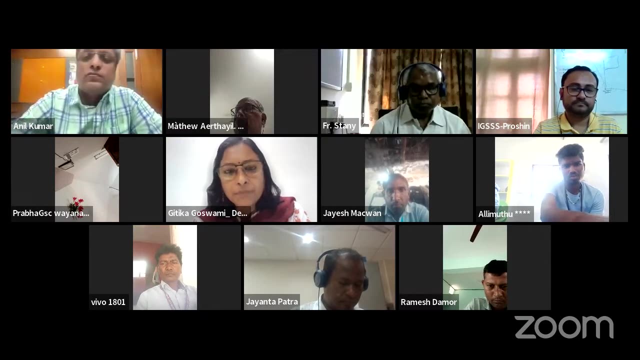 that you are working with them because they are landless, so I feel like they don't do agriculture, or maybe they are agriculture labourers not having their own agriculture land. if I understand that clearly, maybe then I can say that we can really work with them, what type of work you can do. 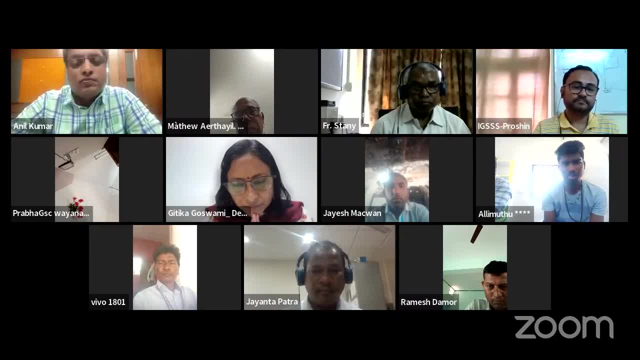 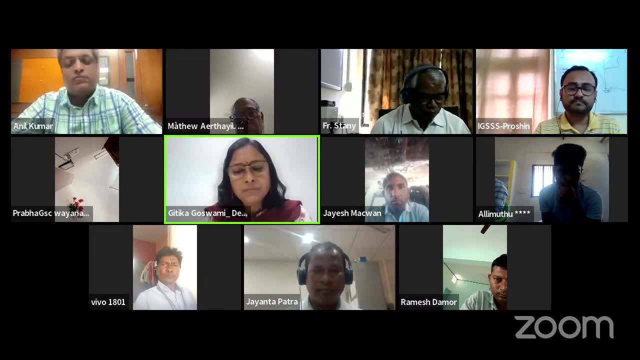 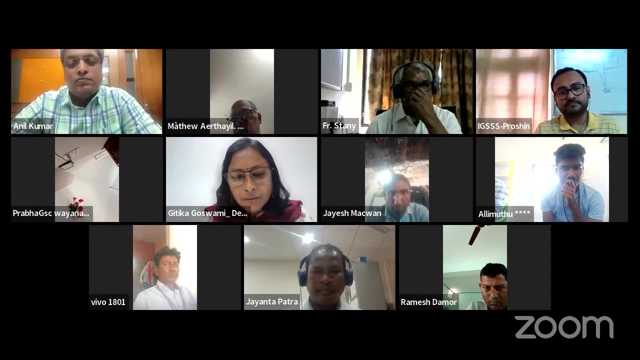 yeah, ma'am, they are actually the landless workers. they don't have any land, so they go in others land to work. okay then, yeah, so I think then in that case, the agriculture, they are basically then labourers and they are getting their wages. you know, it might happen for them. 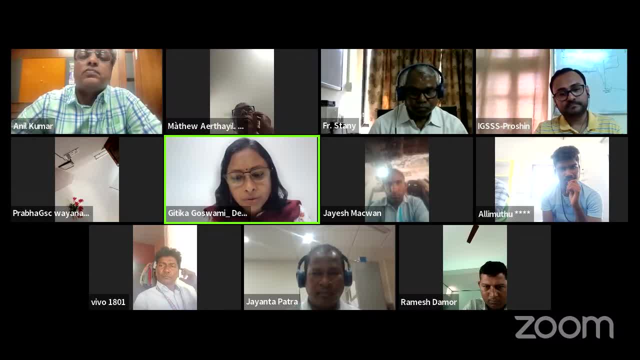 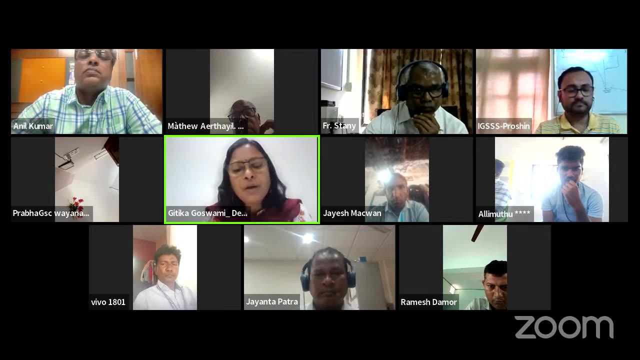 that they are not getting enough number of working days in the village and that's why they are. they are moving out and, you know, migrating. maybe that that is one issue and that's an issue of climate change and they, they become climate refugees. so I mean we can talk much. 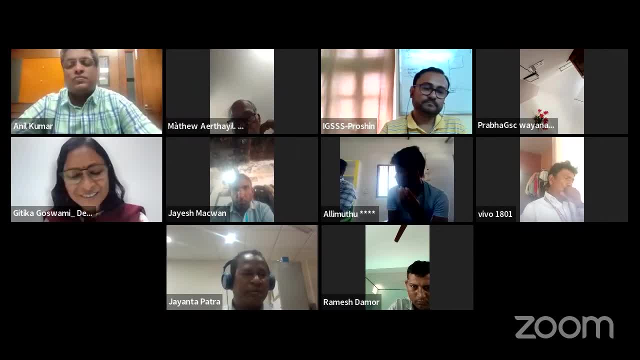 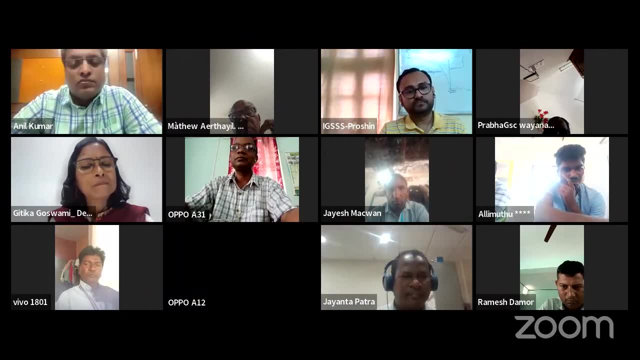 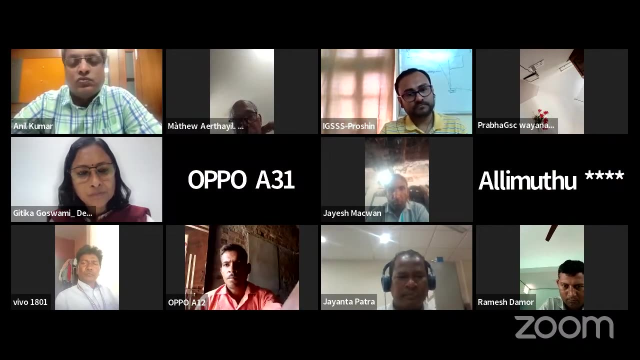 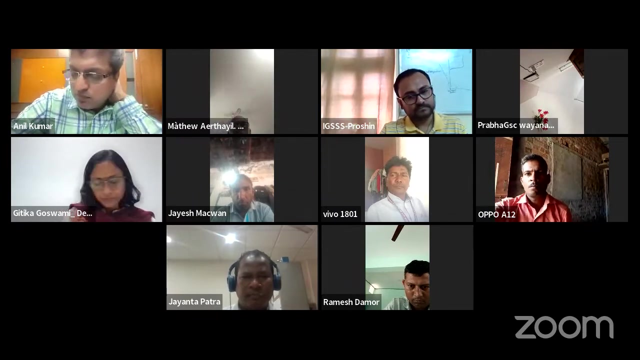 on this and yeah, thank you then, sister Marcy. yeah, sister Marcy, yes, yes, yes. So our problem is like: we are working with the fishing community here in Trivandrum and the fishing community is facing faced with natural calamities and man-made calamities. 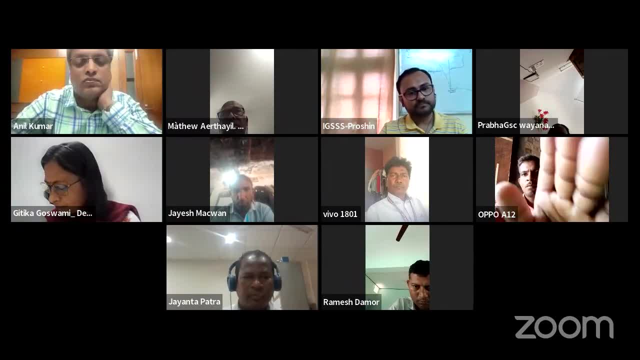 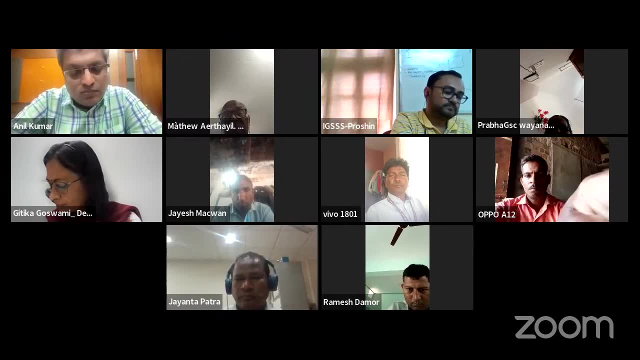 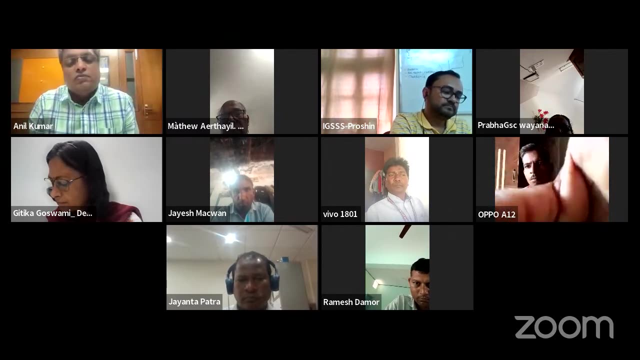 so natural calamities, now the recurring cyclones, one after another, it is coming, and also sea is very rough and the sea level, water level has increased and there is sea erosion and houses are demolished because it washed away with the rising water and added to that, the construction. 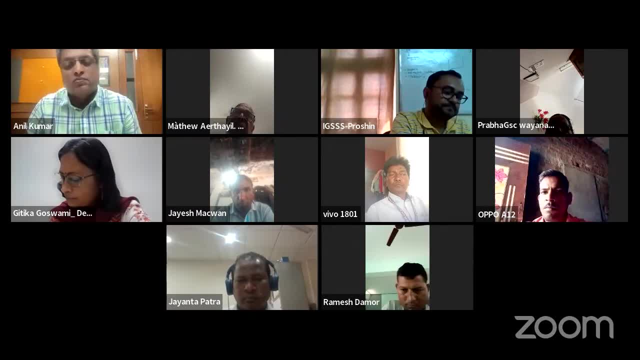 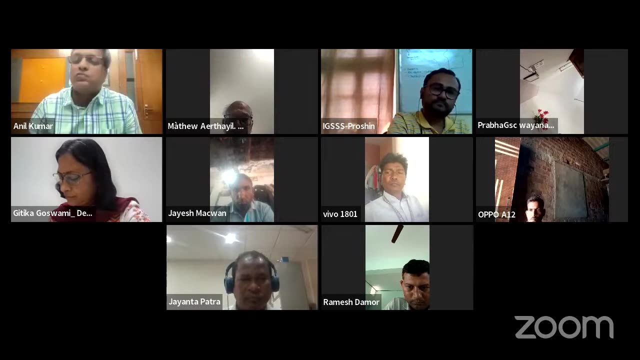 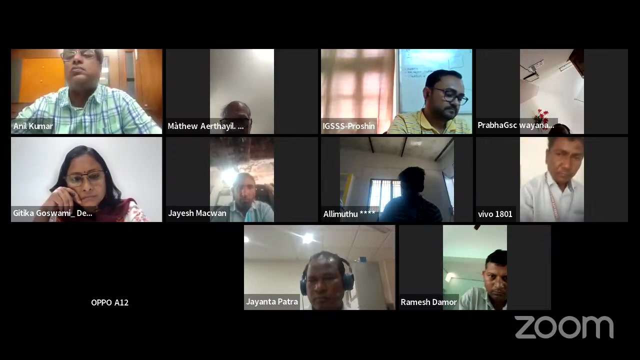 constructions, illegal constructions are happening in the seashore also, mining is happening and sand mining, all this is are. these are all happening and India is a signatory in the in the in the coastal areas. but then how far we can work into situation in the coastal areas? 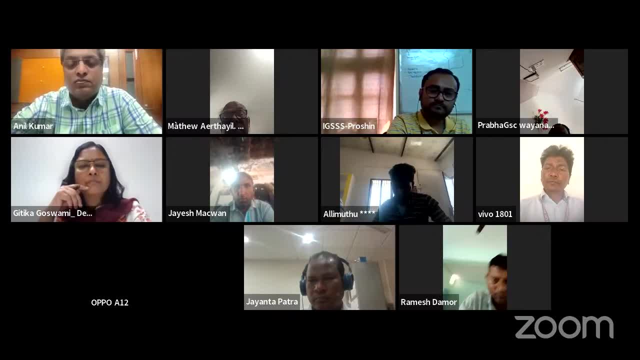 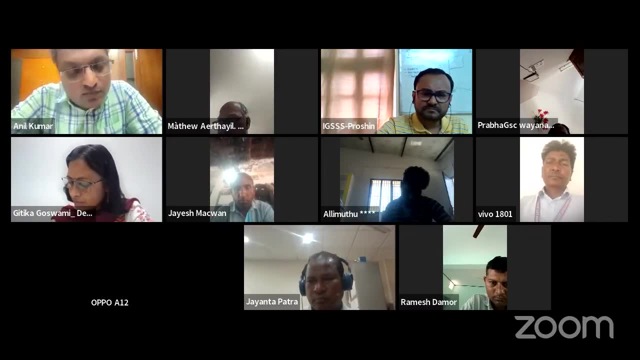 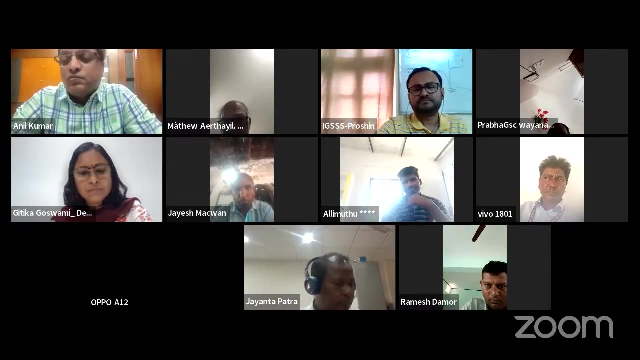 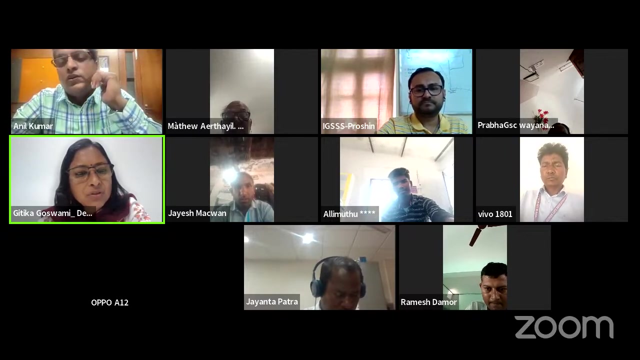 that's my question. people lose their livelihood and they are not able to get into the sea at times. another thing is, the fish also is reduced, so these are all affecting the lives of the people and a lot of people are losing their lives. Anil, can you please ask everyone to mute? who is not talking? I think there is a lot. 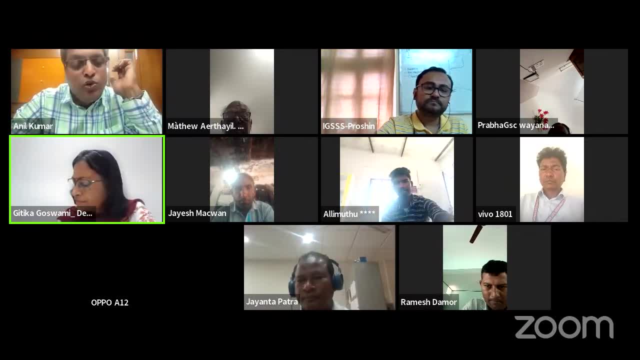 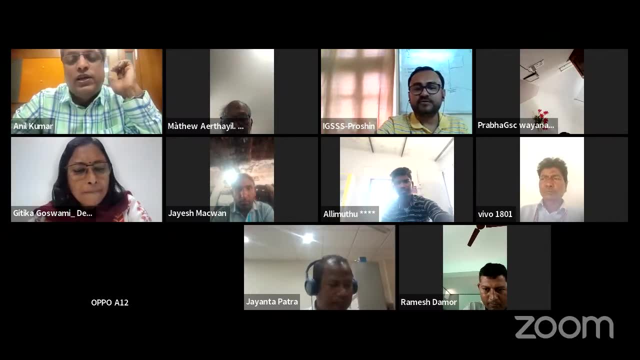 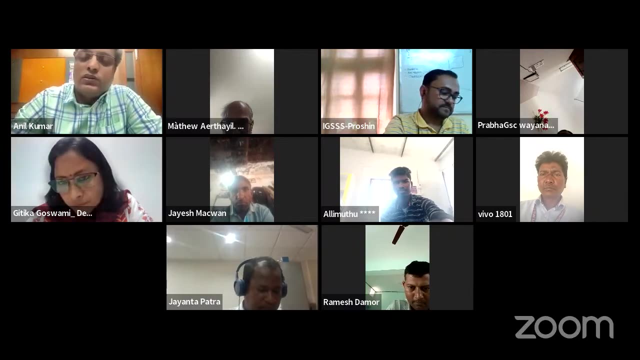 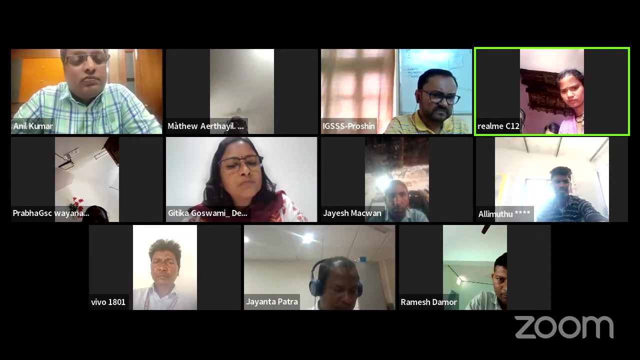 of…. Yeah, some is coming in. Yeah, yeah, Please mute your mics. Could you get ma'am Sister? can you please repeat the question again? because, yeah, this is, our problem is like this: we are working with the fishing community and we don't have a solution before. 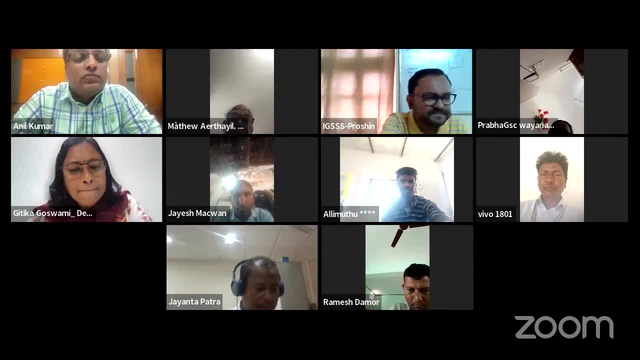 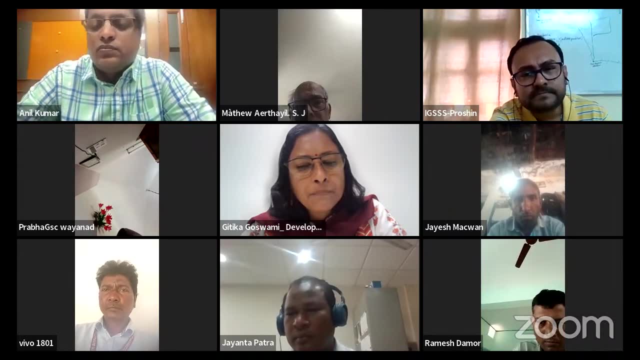 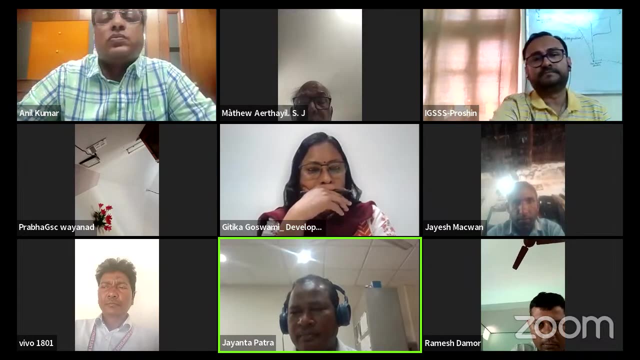 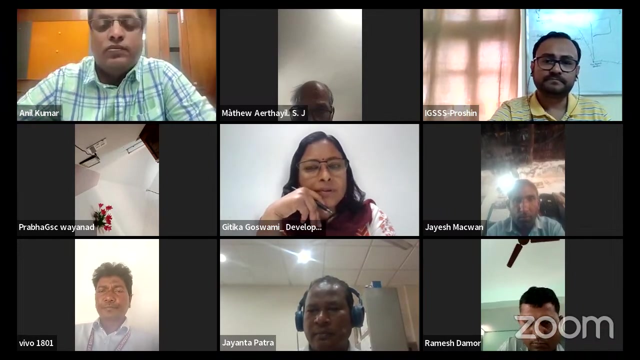 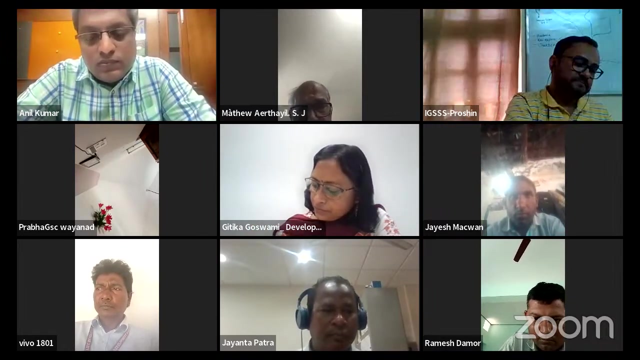 them, because the government is… The government also is adding to their difficulties. Who is real? Just I put it. yeah, Please mute it. Yeah, I did it. So every year, the seawater level is rising and there is recurring cyclones. it's all. 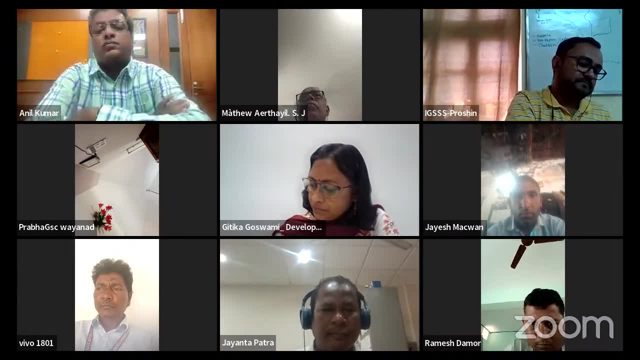 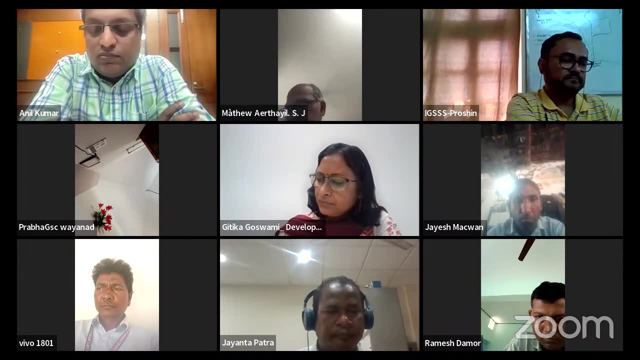 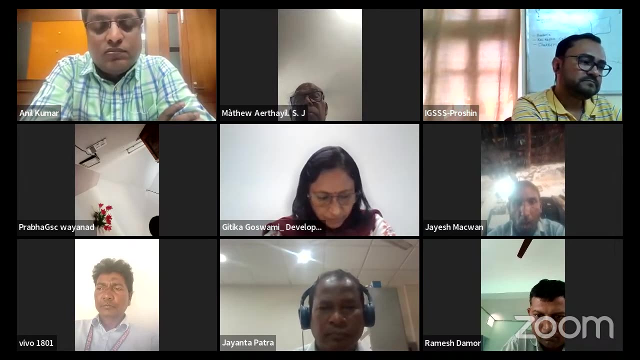 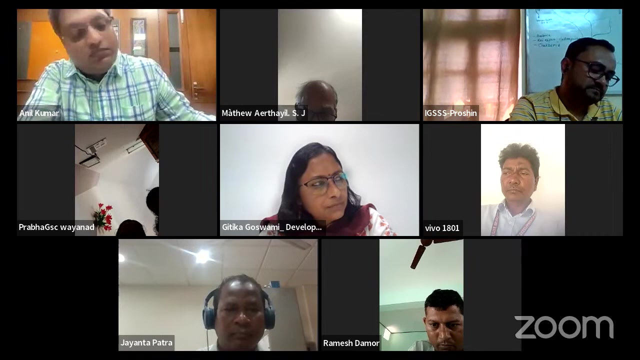 we can attribute to the climate change, but people are not aware of it. however, we say also they will go to the sea and they are depending on the sea for their livelihood. So now, recently, what is happening is like illegal constructions And big ports are on the seashore, plus mining- sand mining- is happening, so it is an added 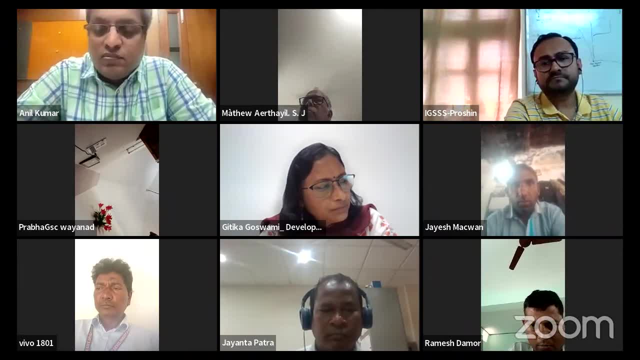 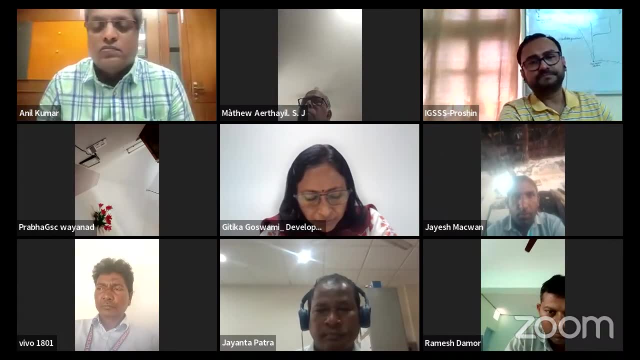 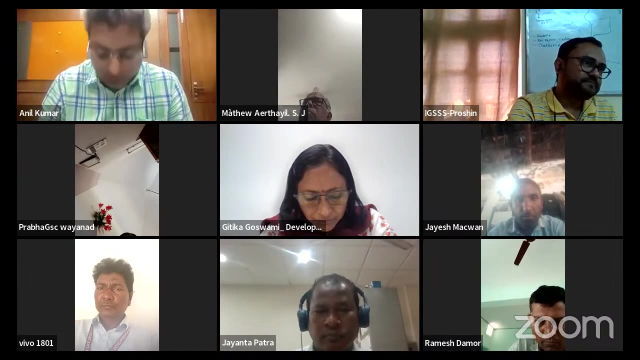 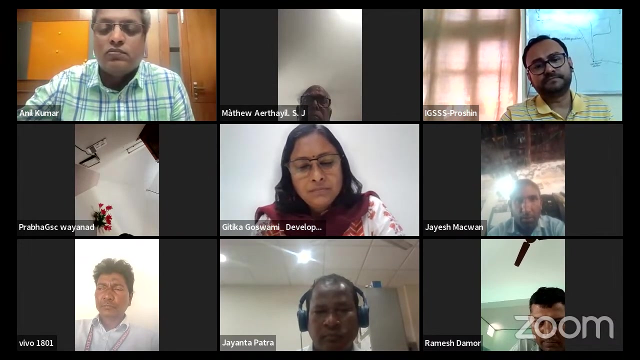 destruction of the nature and causing problem to the traditional fish workers. They are losing their job, they are losing their houses, they are losing their identity. So this is the condition where we are working Right, Right. So our problem is how, as a lock bench partners together, we can make an effective our presence. 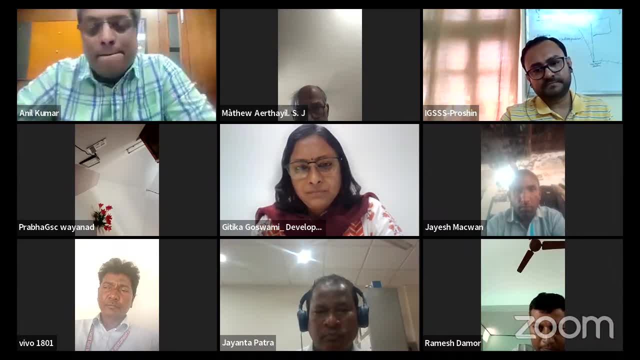 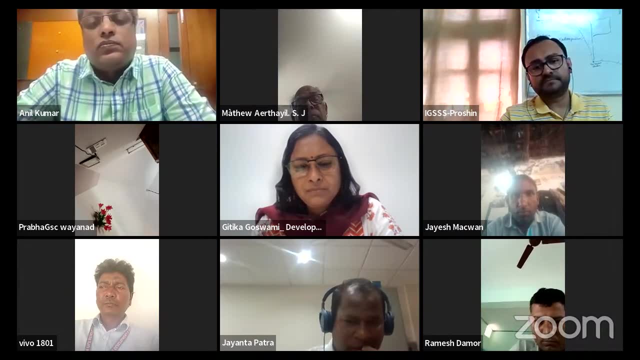 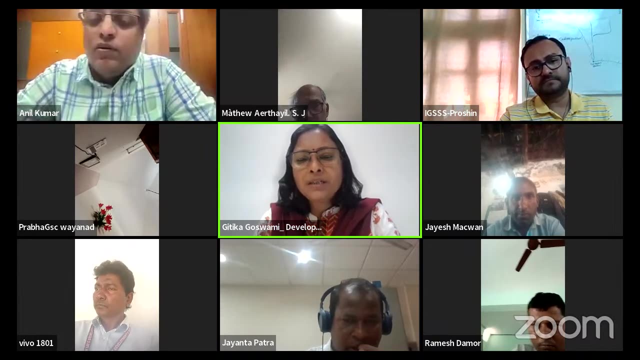 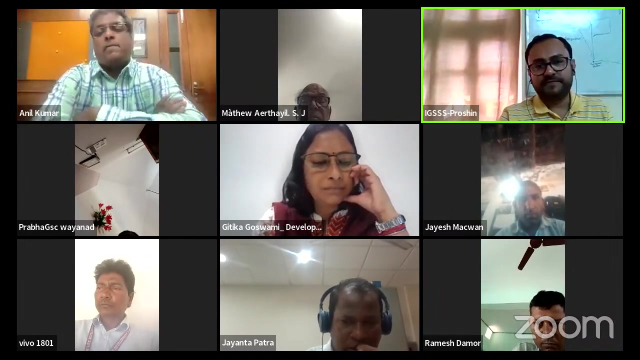 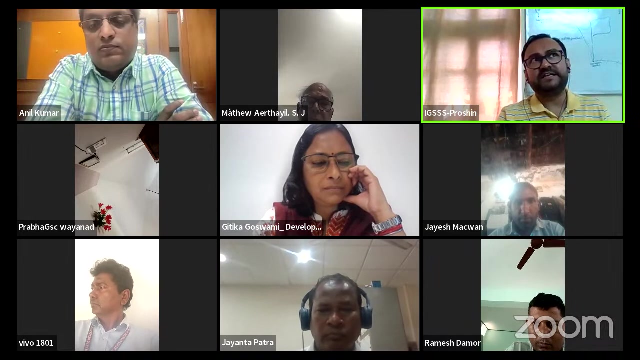 effective among the people to resist this natural like global warming, and to take precautions? Rashuni, you will take that question or maybe I can…. Yeah, Yeah, Actually. first, our situation analyzing is very important in this. what is the current situation and what is their understanding? that is the problem. you have said the problem. 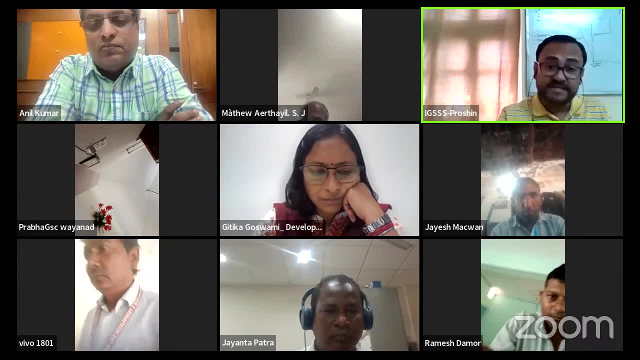 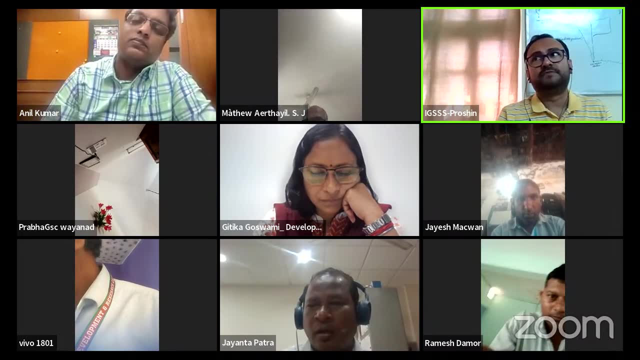 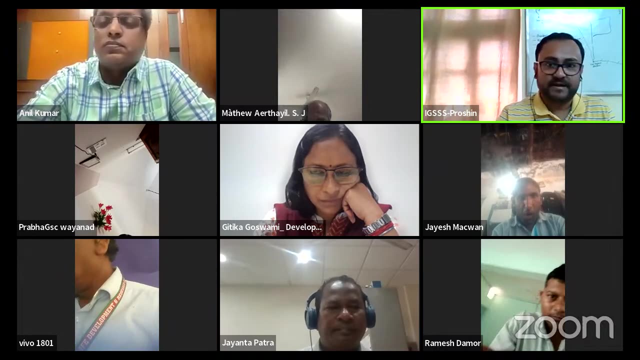 statement. but what is the solution the community is expecting from us? that is very important because we, for example, if we say that fishermen must use some alternative language, So this is what the solution is. Okay, so this is not the solution. because their bread and butter is fishy, so some people will. 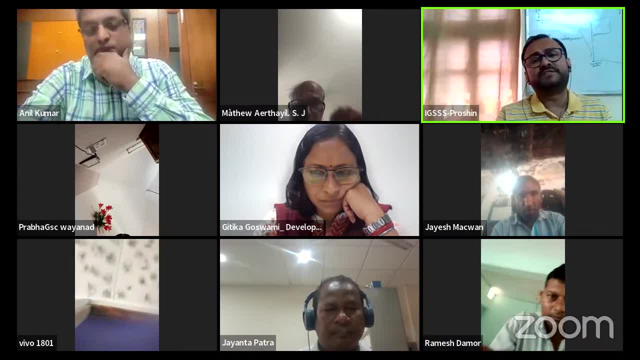 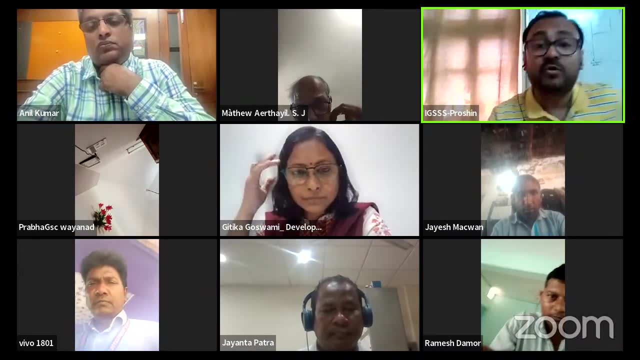 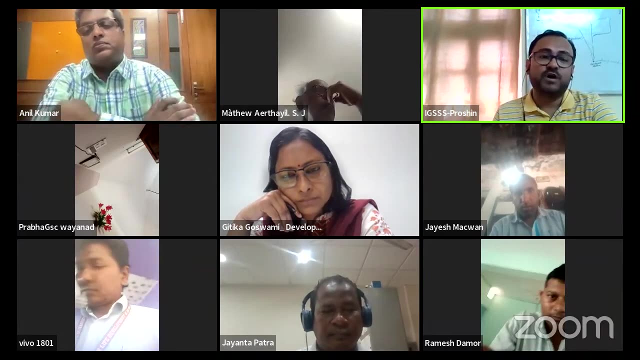 some people do not want to do something other, some doing something other which is different than fishing. so what is the solution? what are, what are they thinking that how they can address these challenges? so first we need a very important discussion with them and then with the local beauty. 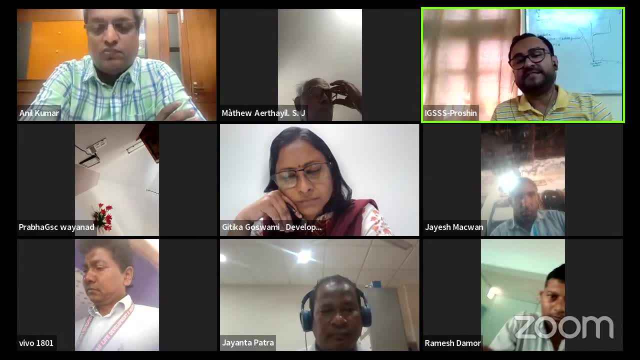 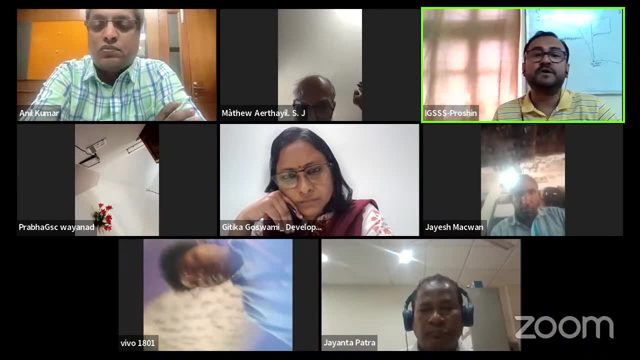 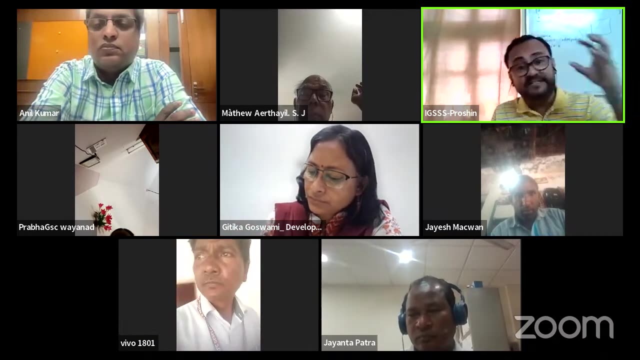 wearers, local uh departments, line departments, customer and then a discussion with them. if we can hear that made us some joint joint workshop and uh simultaneously. if we say some a good network, we can produce some good network, good alliance with this issue. highlighting this issue because there are a lot of ngos, there are a lot of co2 working with fishermen community in the same area. 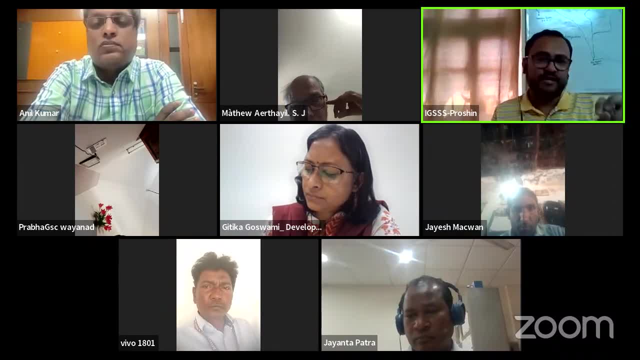 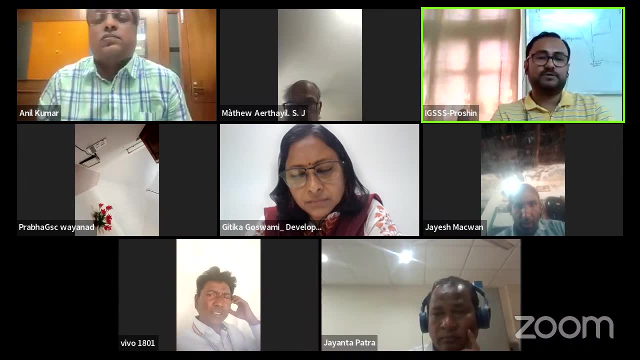 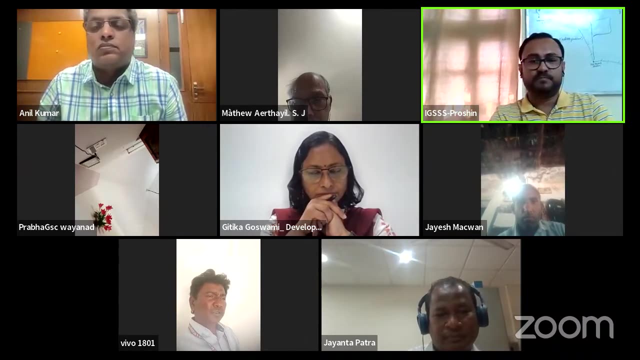 so if you can come to the same platform and with a good networking interview, and then we can together in a group we can go to the duty bearers, for example, any departments, maybe in a local admin representative or maybe any uh good resource person, so so that they can understand. 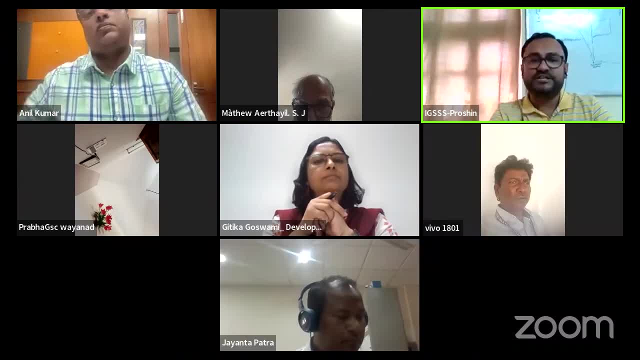 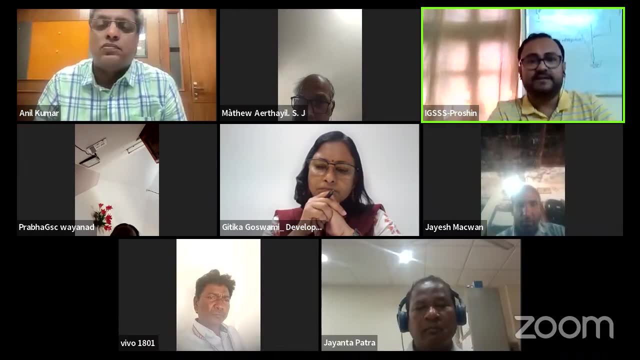 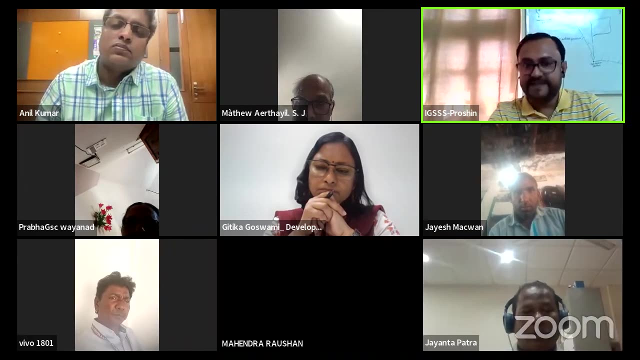 understand their masters of solution, uh, with this negotiation with them. this is the thing, and, apart from this, i am not sure about the book, but this is just my only uh thinking that, uh, how much is mangrove sustainable in this area? because, uh, you know that, uh, after this pop 28, there is a big alliance, uh, regarding this pop, sorry pop. 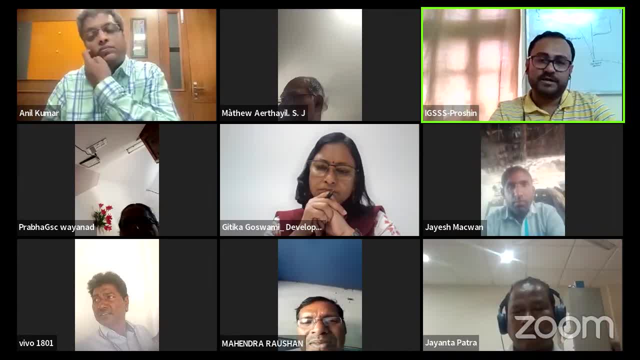 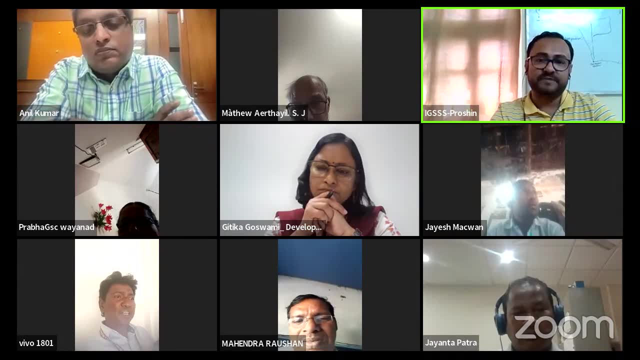 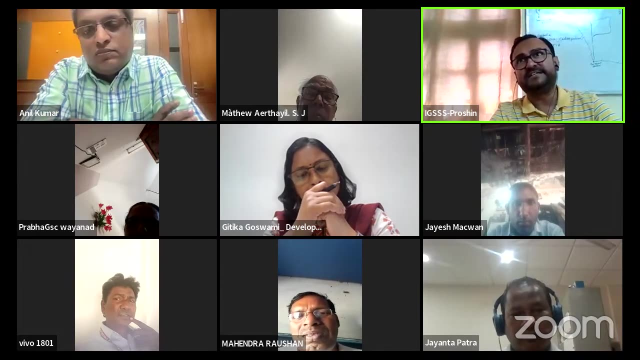 uh 27, there is a big alliance regarding the mangrove, uh sensitivity, uh so, and even our central ministry is also very much interested in this. so if the area is suitable for mangrove plantation, at least if we see that 50 years, 60 years or maybe 100 years before there was a 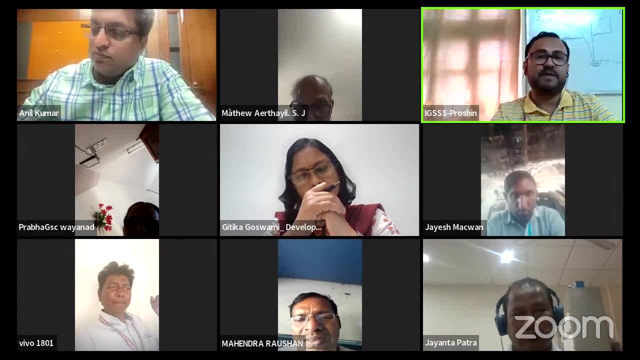 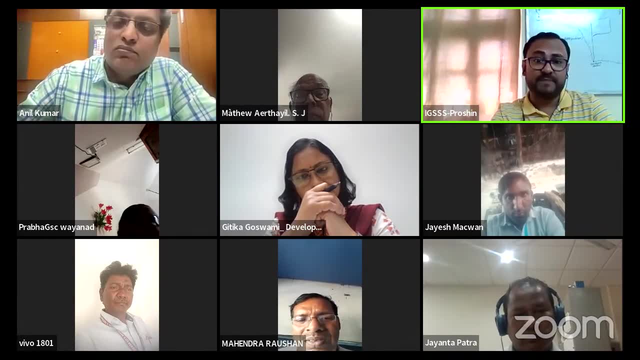 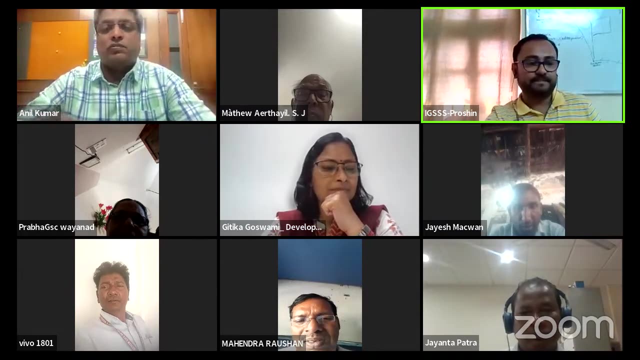 mangrove plantation area and i would patch. then we can regenerate this mangrove and replenishment, this macro plan so that the uh- the erosion problem and the uh- the embankment bridge problem is compound. so this is the uh input from my over to people. yeah, hello, thank you, thank you, yeah, i think uh, yeah, you have actually. 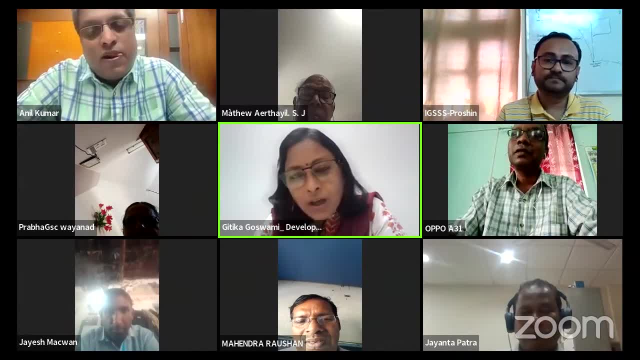 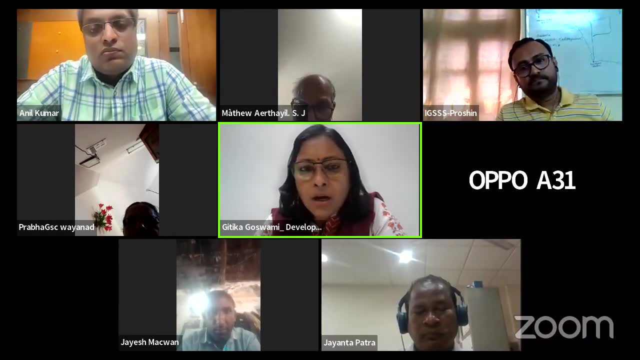 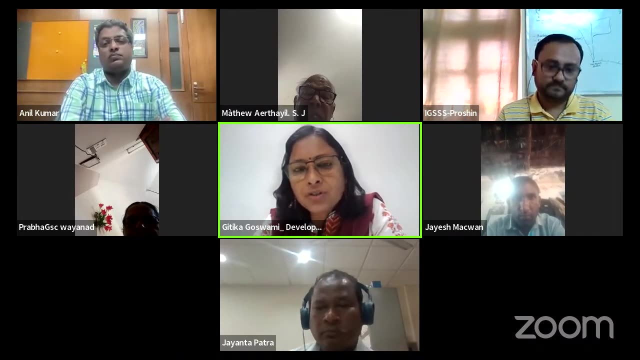 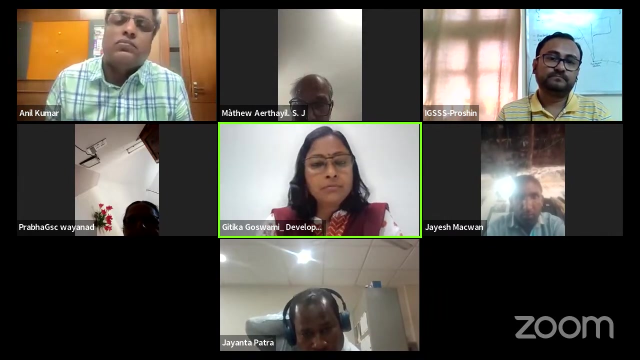 uh, touched all of these points. so, uh, first of all, i i would also just emphasis on uh, this, uh, you know rapid cyclone. uh, now, the nba is the nature-based solution, is a mangrove plantation or reforestation, or regeneration of macro. i think that's, uh, that doesn't really require a lot of infrastructure. 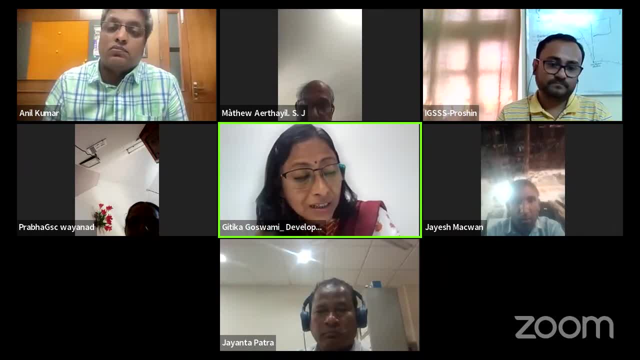 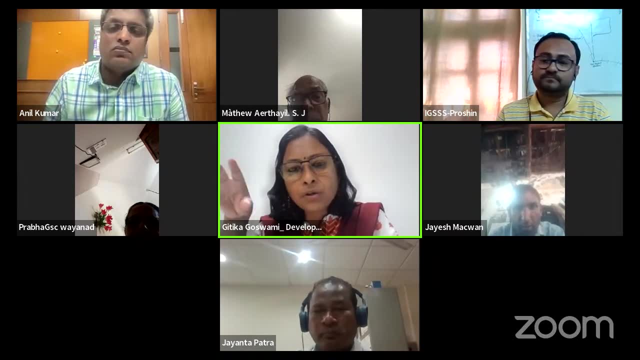 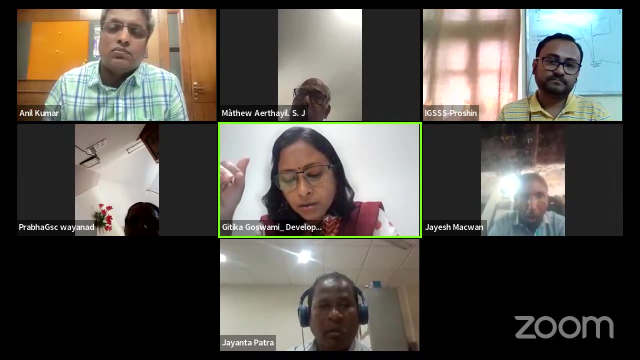 but it's just required communities to also communities can get some kind of livelihood for that, you know, for the mangrove regeneration, and i i think that's one of the best case examples: several places along the river, along the coast, uh in uh, in orissa, in sundarban. 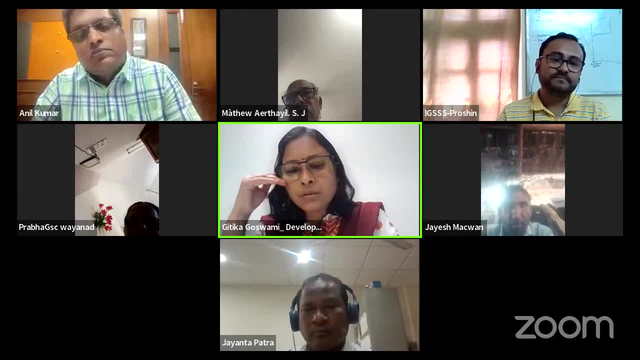 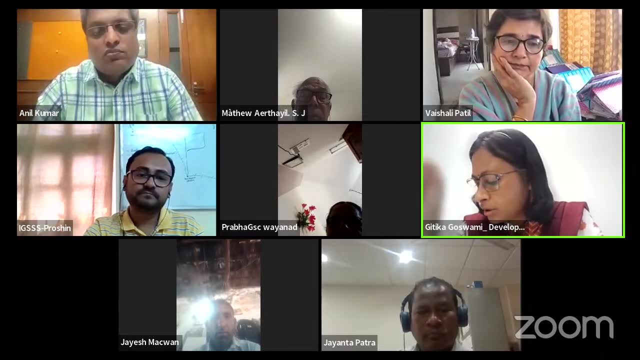 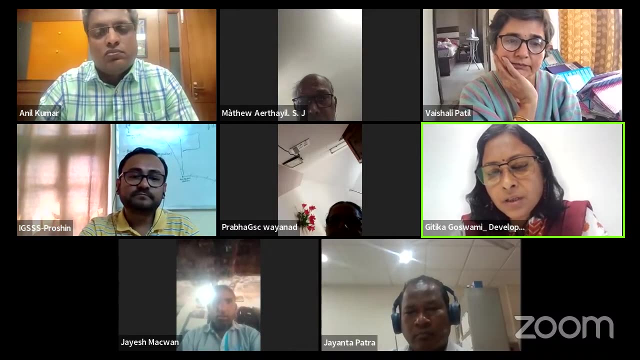 and other areas that's been happening. so which is uh best, uh uh, proven technology for, uh, the the coastal cyclone and erosions? the other thing is, i think, as person also mentioned about the diversifying livelihoods. i think, uh, that's very much important. a lot of the. 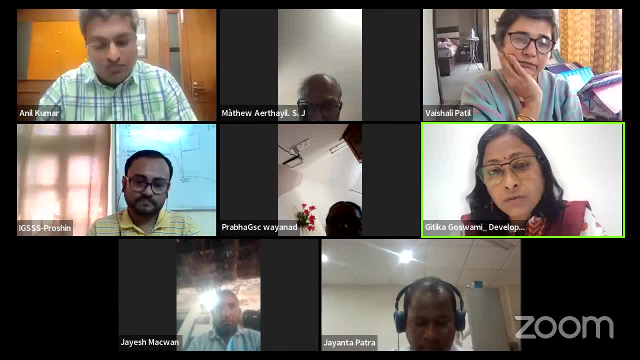 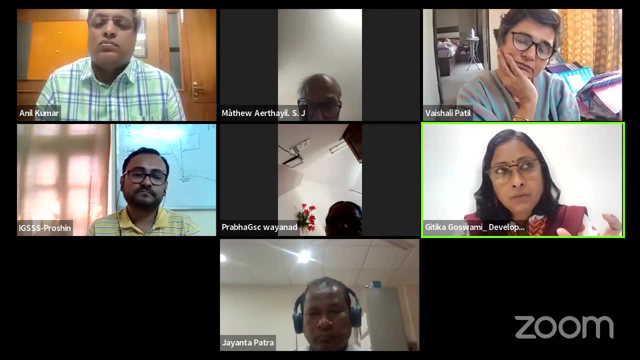 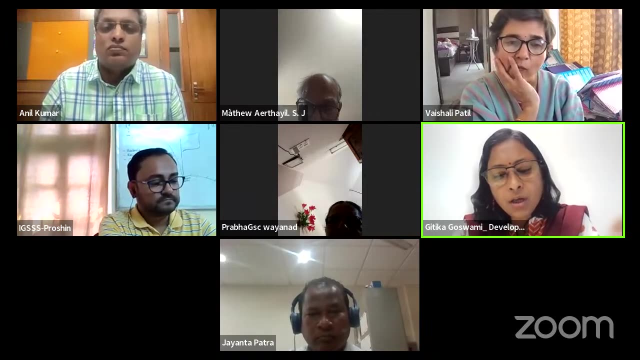 different institutes, uh, agriculture and fisheries institute. they are working on, uh, different varieties of salt water, varieties of fish seedlings. that's the come up. calcutta is one. they are working in sundarban a lot uh the agriculture and fisheries institute, so maybe that's an we can have. 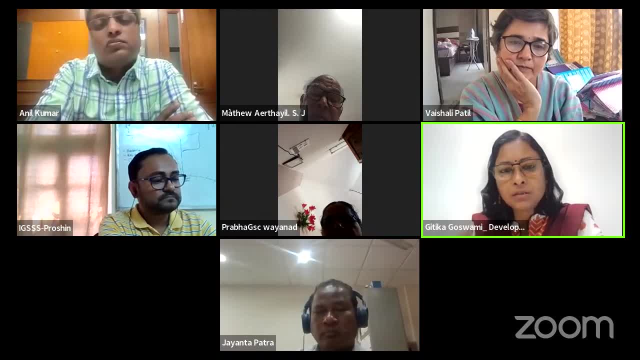 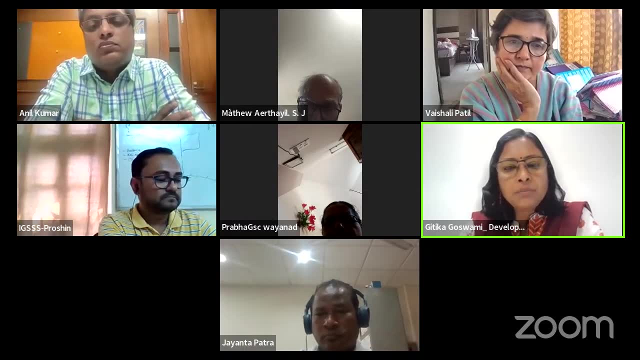 a kind of a network where economic missions and the local government, NGOs and the communities can come together discuss about the problem. and there are several- uh uh, you know, pilot very successful pilots has been there across the country. just that we cannot connect that. so these are kind of a forum where we can actually connect. 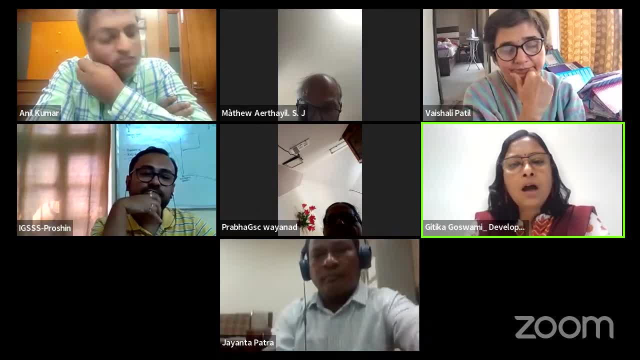 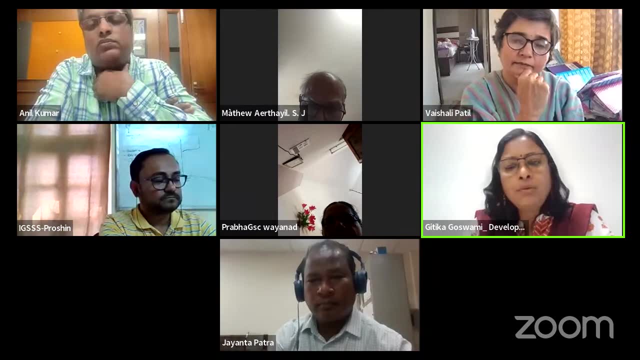 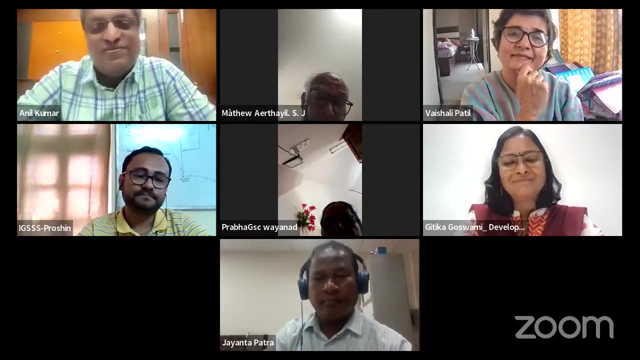 them and where a very good example is there and how can we learn from one another? so i think that's how, Sister, we can solve a bit of those issues. issues of the local community, that is true, we are also. we are also in that, in that process. 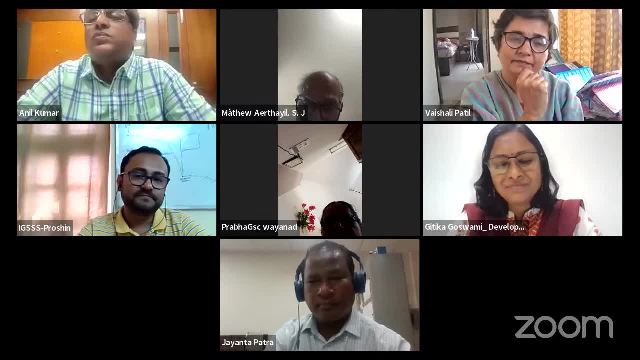 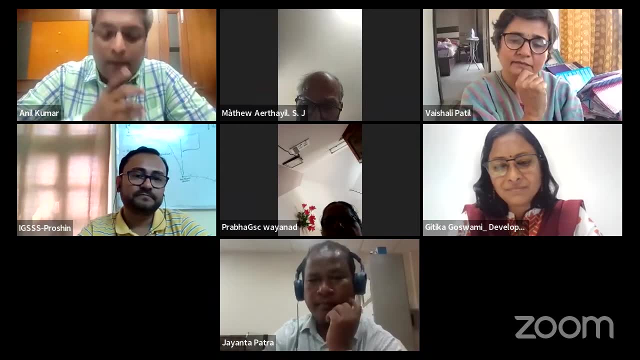 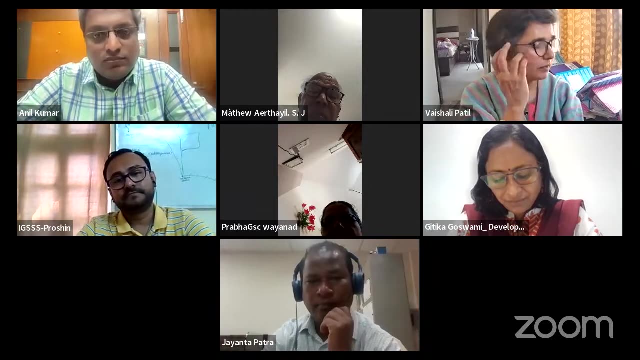 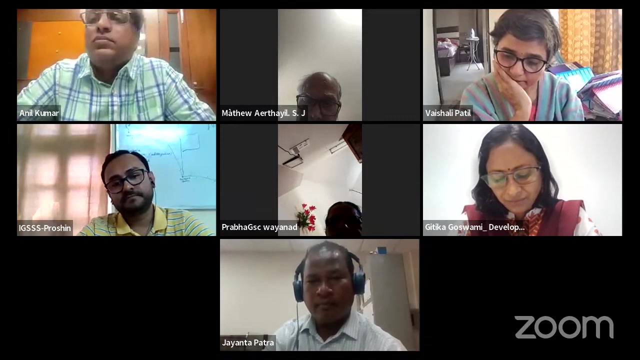 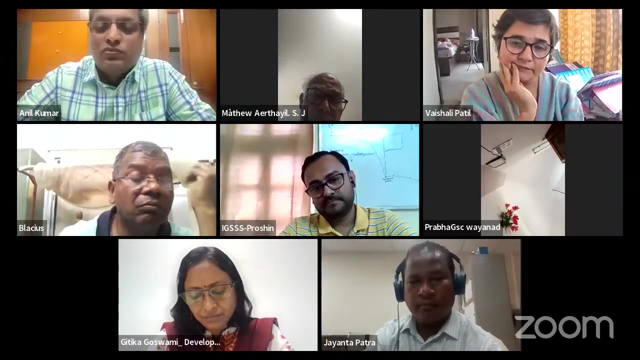 now it has to be wide enough to resist the plans of the government to support the multinationals and like corporates, corporates to start building the illegal constructions, and that causes more difficulties on people, adding to the natural, like global warming. so that is what, surely, that networking and putting our effort together can help us. thank you. 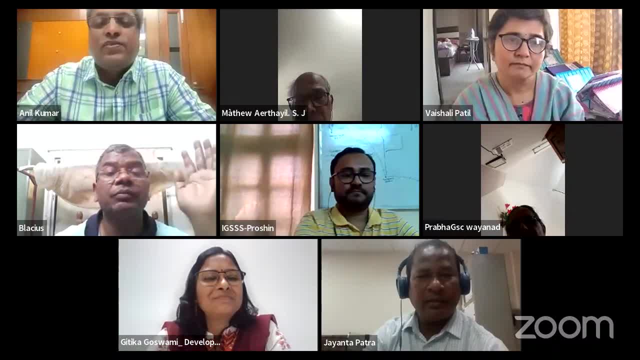 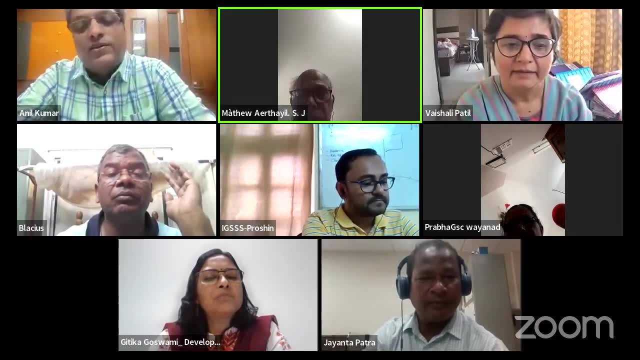 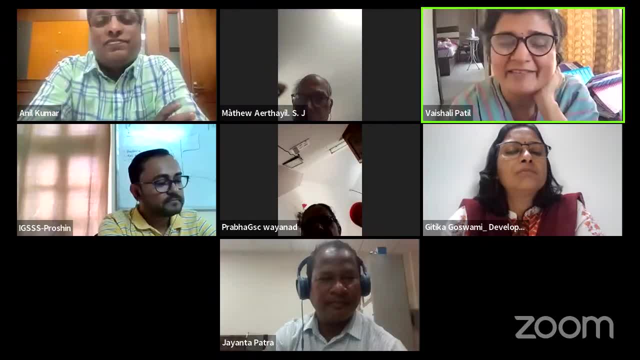 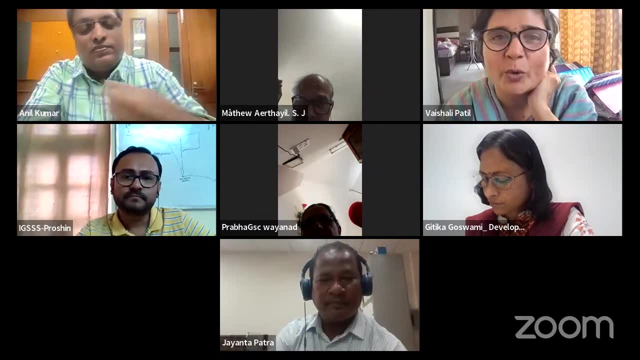 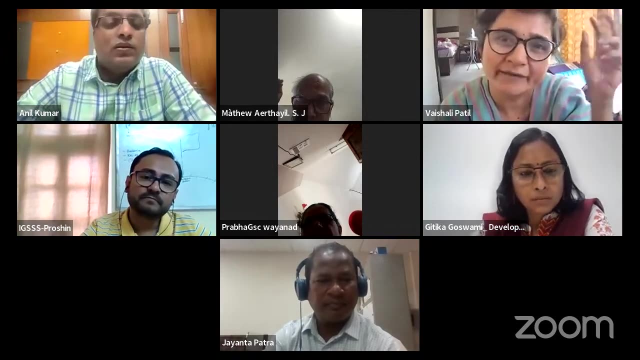 in raigat district, maharashtra, we have a twelve percent of the tribal population and among them is percent are the pvt. some challenges with them. pvt g's used to do the zoom cultivation previously and those that all zoom cultivation used to be on. 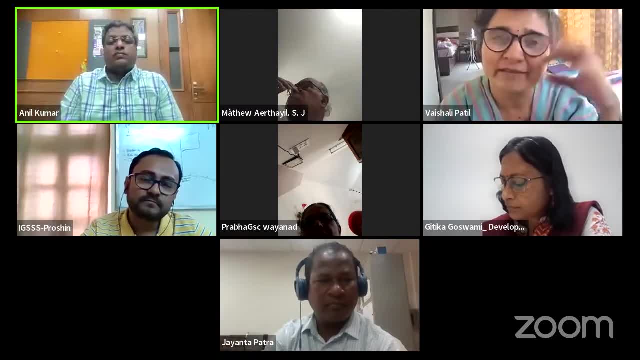 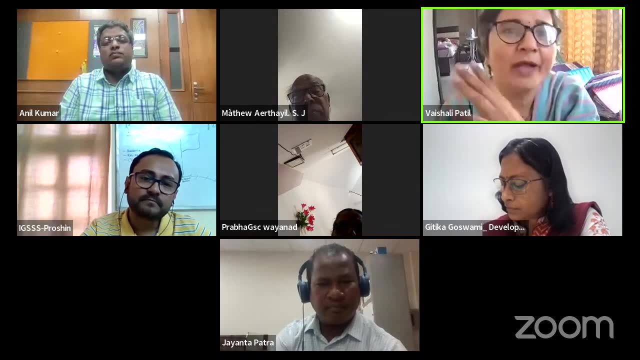 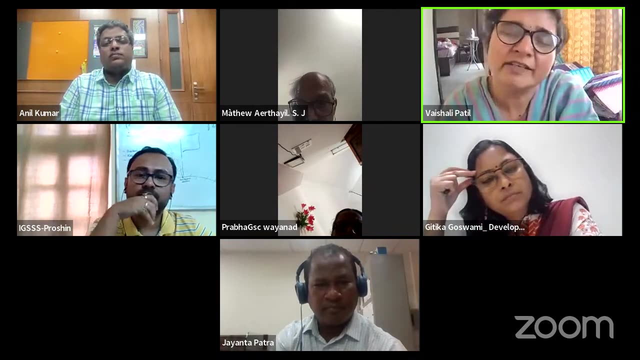 the forest land. so in spite of they being a forest right claimant now and filing the claim also, what we see a trained in them is giving up the upland and giving up the upland cultivation. and now we see that in the families with the children's diet, especially women and children's diet, there are no millets, there are. 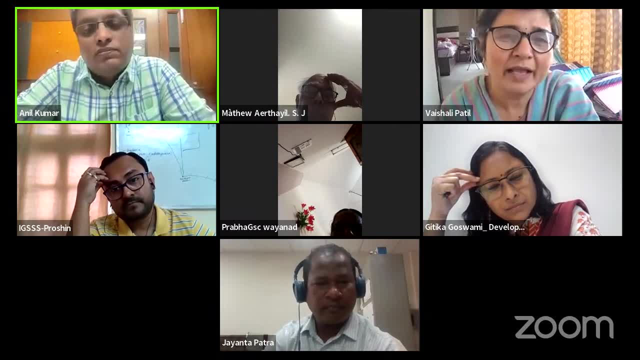 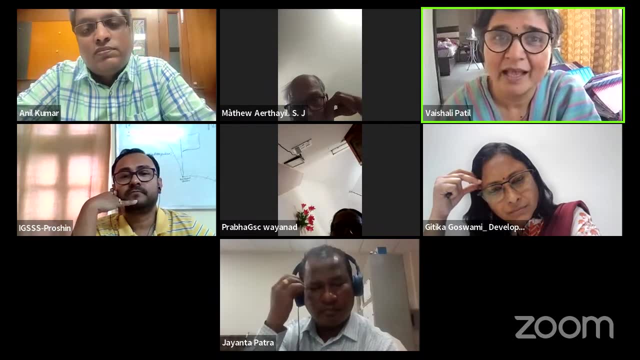 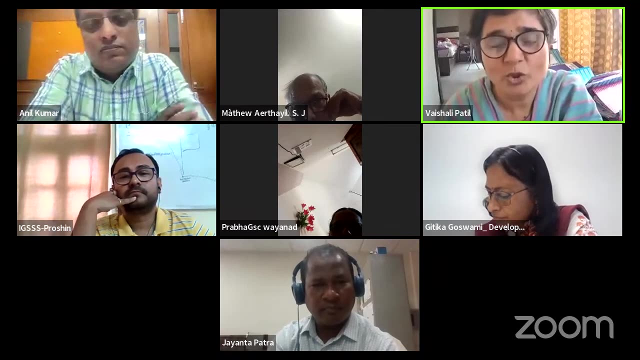 no tubers. so, uh, i mean this. uh, the reason why it is so is very clear: that now it is becoming extremely difficult to do the upland cultivation. a lot of labor is required. secondly, uh, the kettle grazing is also not controlled, and that's also one of the problem. and then land landslides, and 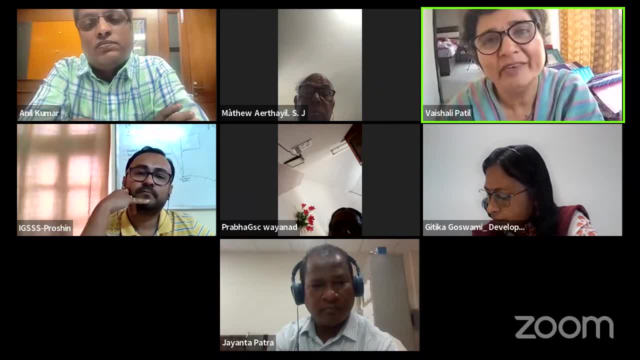 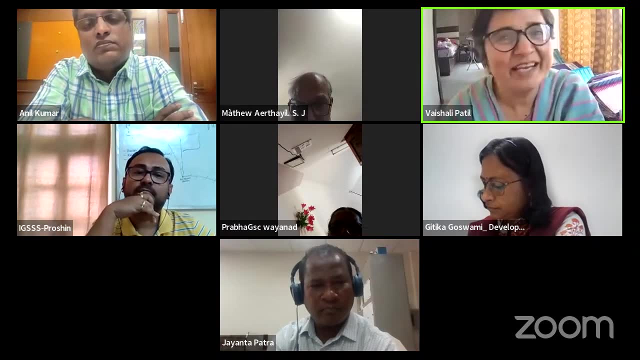 erosion makes it a little difficult, and on top of it we have a period in which the pvt just gets 35 kg of the ration, so like it is two rupees, three rupees. now it is free. 25 kg of grains are available there. so 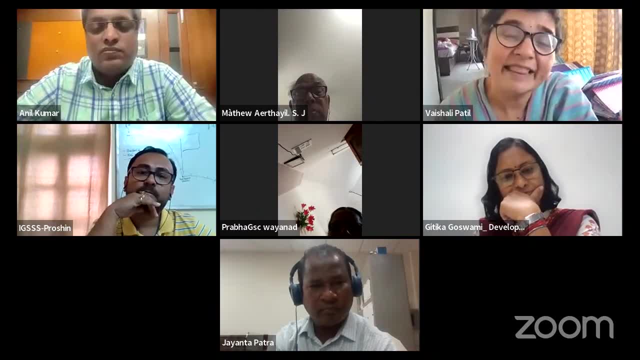 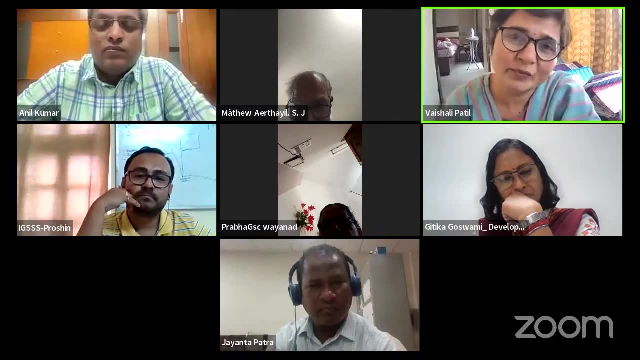 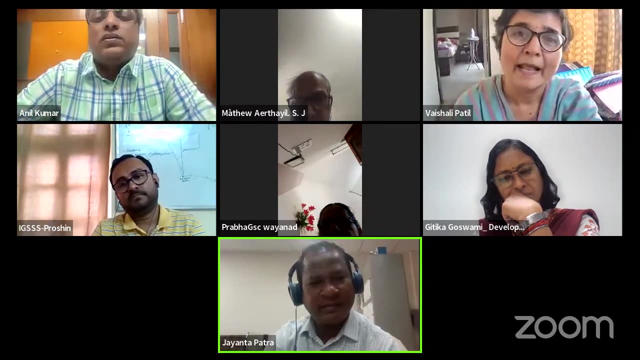 so there is no urge of having, and then it directly has an impact on the health of the women, children and the whole community. so we are finding it little difficult to really motivate, inspire them to do come to the upland cultivation. so what's the question then? uh, the question is: how do we? 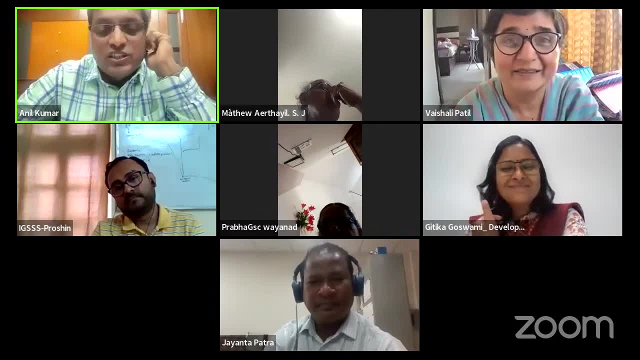 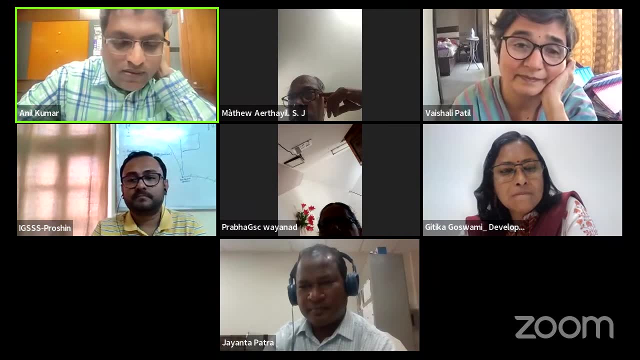 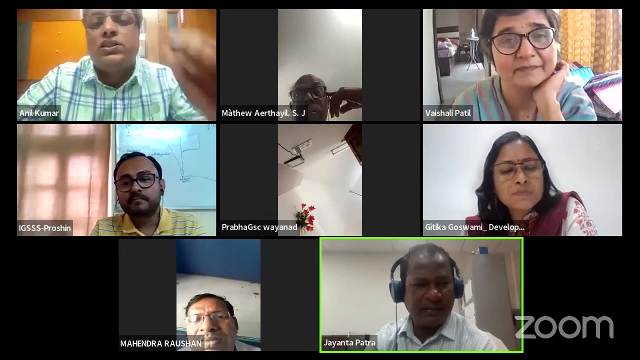 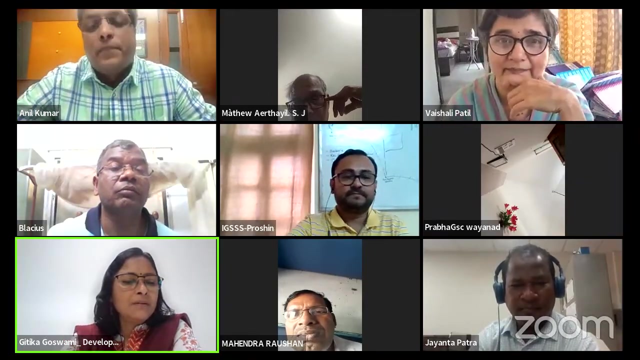 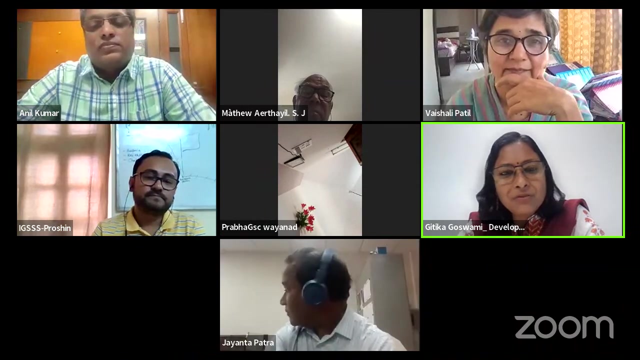 tackle this challenge? oh yeah, yeah, is dr anjali around? dr anjali, now i think this, uh, she's not here. githiga and proshen, you want to comment? uh, yeah, so uh, i think, uh, this is some of these issues uh, we are facing everywhere. 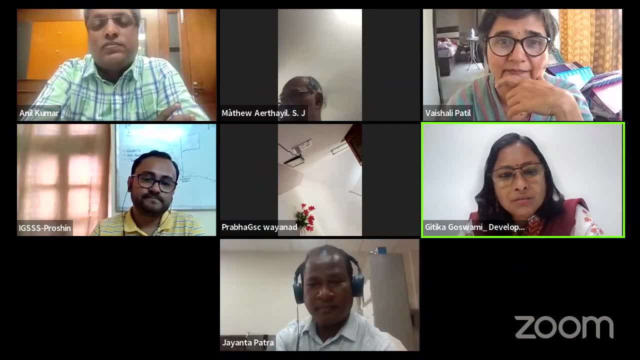 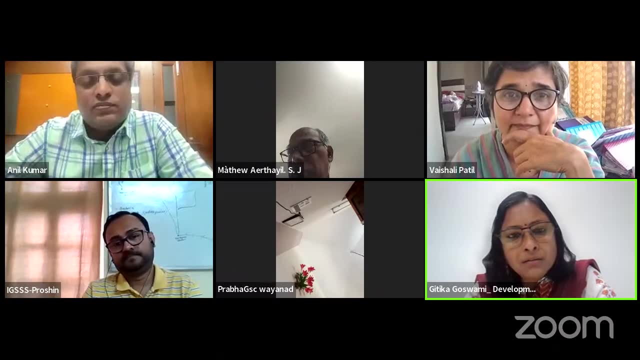 this uh, as you mentioned about, uh, the upland cultivation and the millets and the tubers and all uh, and i think this is a very important issue. and i think this is a very important issue and i think this now become an issue where the political leaders are also kind of aware of. and, as you know, there's 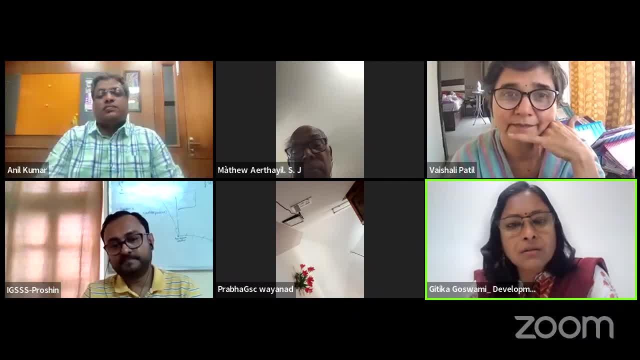 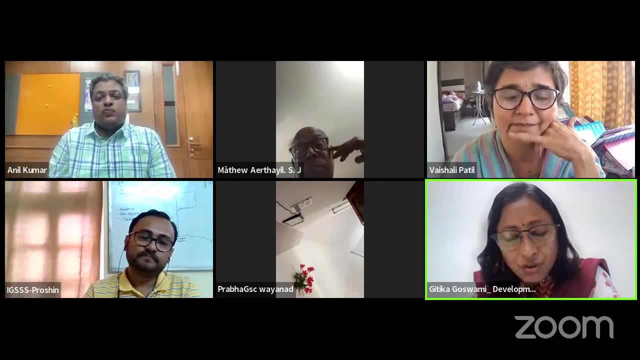 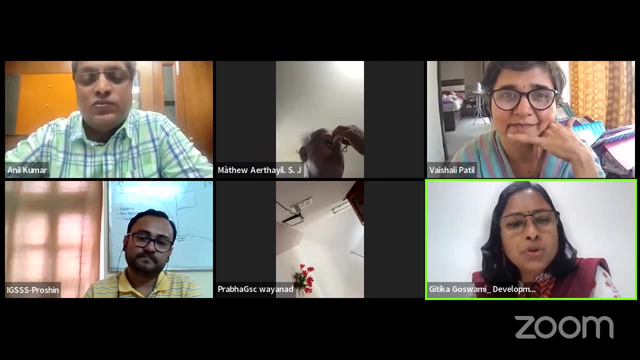 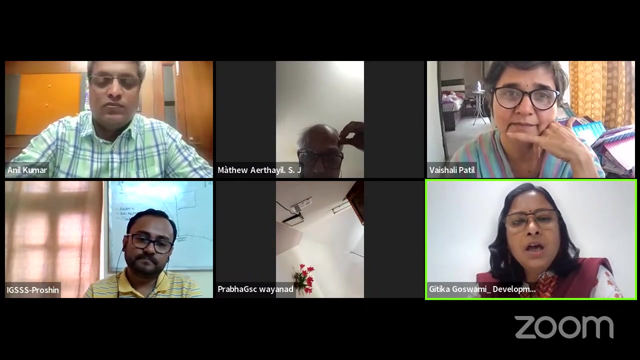 this year government has already started a mission, or millet mission, and it's the name is something very ser Guillermo López Oc Kopf, Above alive, something that嘩, that would really push from the top end to, uh, uh, motivate people to come for this millet cultivation and the zoom cultivation. i really 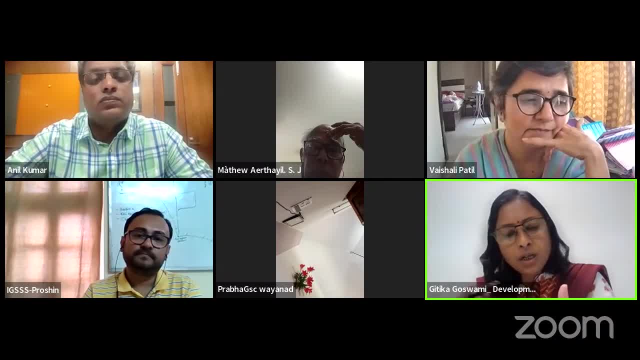 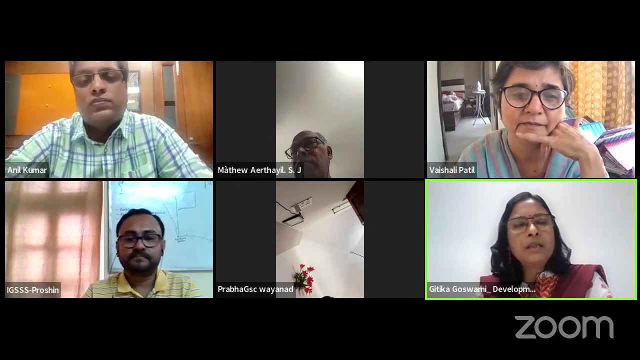 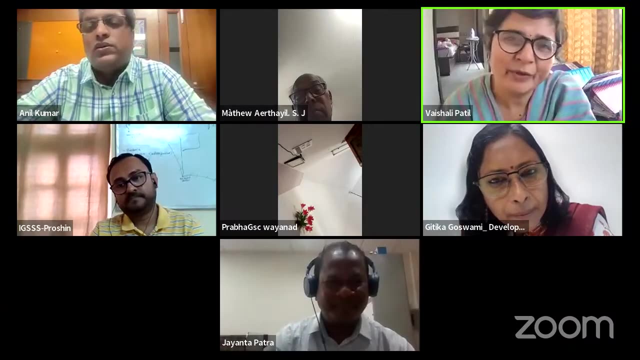 didn't understand that what you are saying. the zoom is continuing. that that's a problem and many a cases you know it is continuing but in a very um less intensity, right, or what is there in raika? i didn't find that connection. traditionally they had been doing a zoom cultivation and then 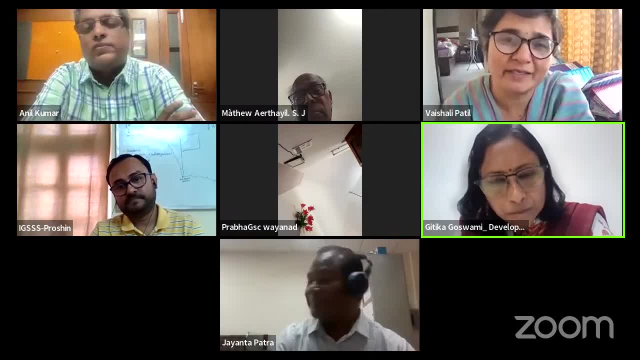 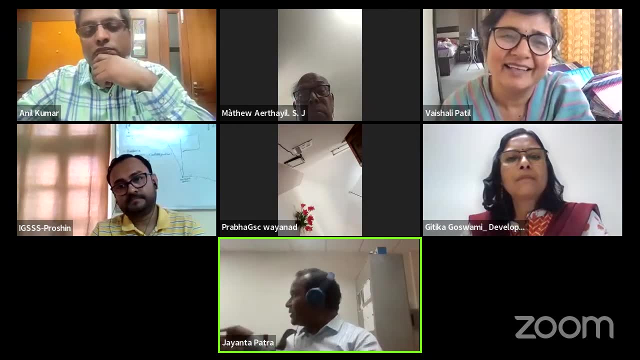 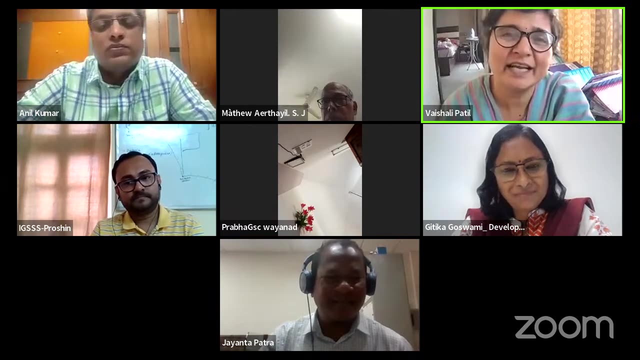 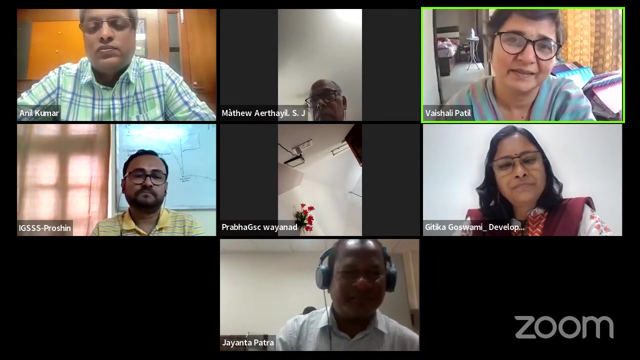 it was for the millets, for the mullet. so the larger percentage of the pvtgs are giving up cultivation, whether it is zoom upland, whatever it is, but they are giving up plant cultivation and they're going out for another, uh, migrate, or they're doing. 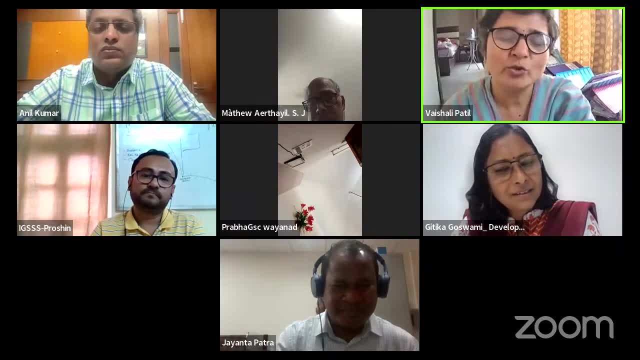 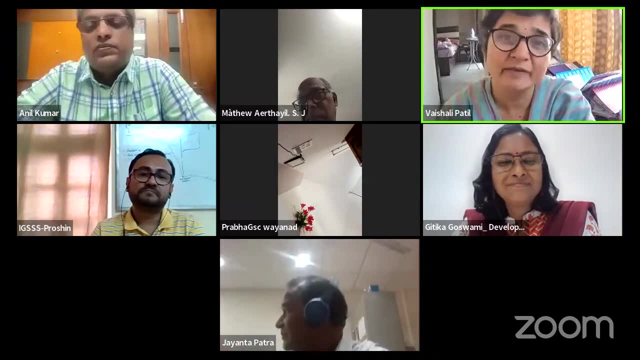 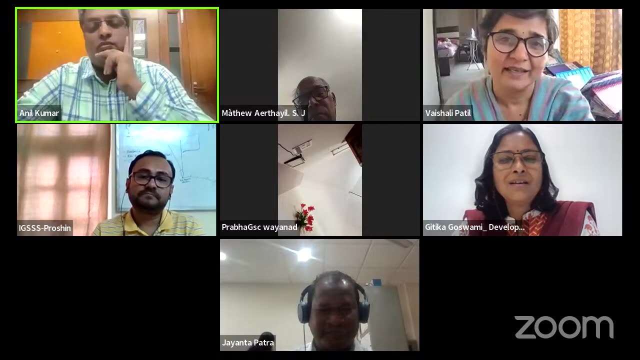 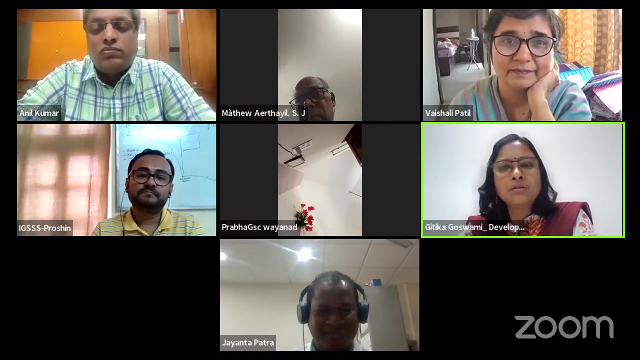 you know, yeah, because it's very easy to get a regular and assured wages on the construction. so they are happy to work with the contractors, they are happy to work with the builders, they are happy to migrate but get something very assured cash in the hand. yeah, i think it's a, i don't know. i mean this. uh, this phenomena is all across. you know, entire. 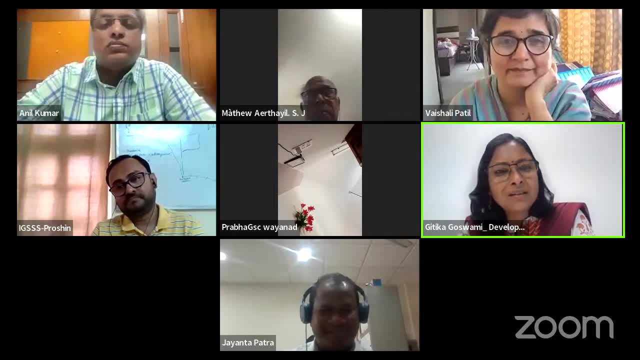 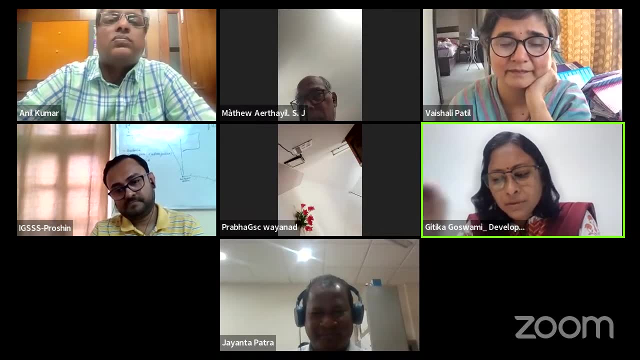 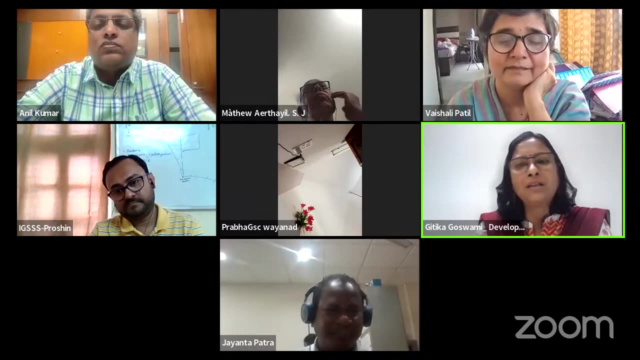 country and the kind of urbanization which is happening and you need to make this particular, Susan. it is also people can uh actually, uh saw that you know People can actually work in a construction sector. that which is much better than if you are working in the agriculture. so it is very much automatically. the new generation is just 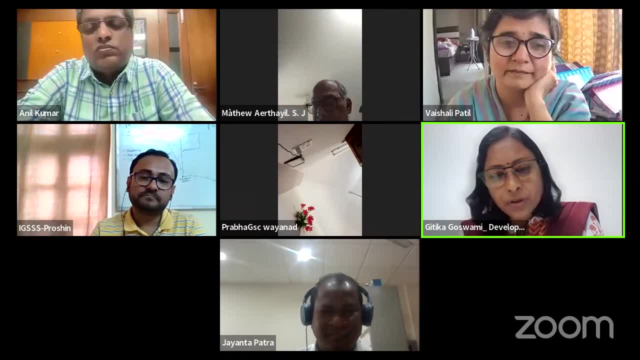 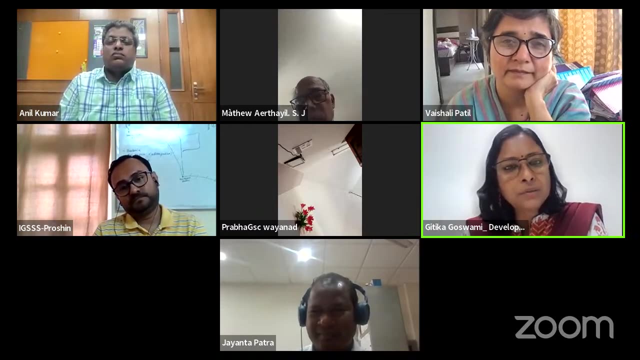 just going out and migrating, i think, one way which i feel is very important. in basbengal we have seen the result that the, the main, are all going out from the villages. uh, for you know, working in the in cities for the labor, but the women are still there and the aged people 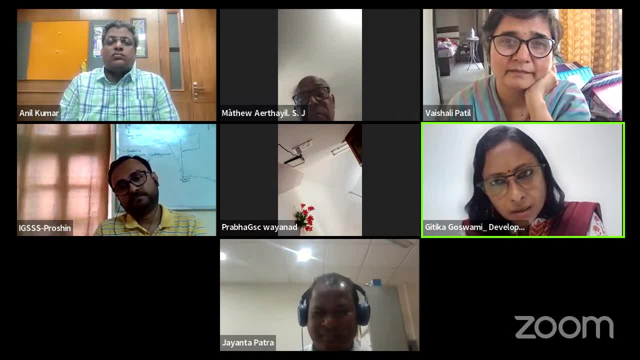 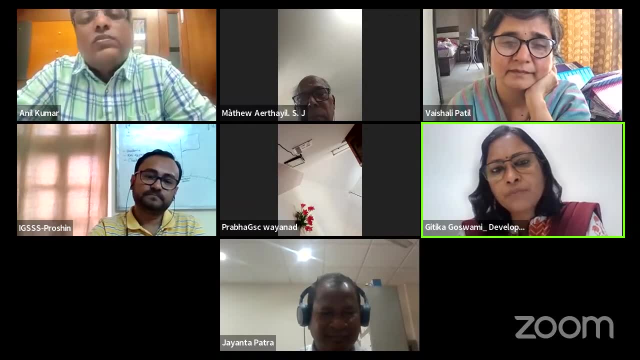 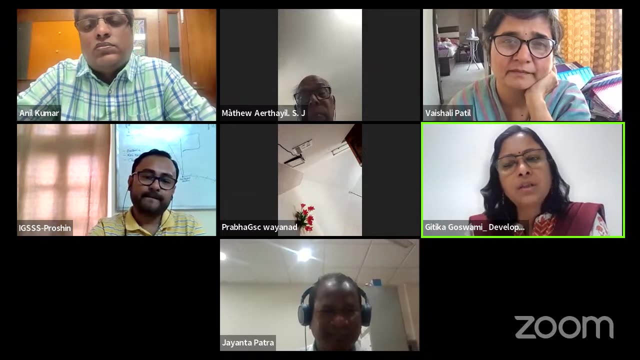 are still there in the village. so if we kind of start this, let me work on this: millet and other agriculture, crops and alternative livelihood. some other thing maybe goatry, some you know, poultry and those with only the women member of the families. i think probably you are already doing that. 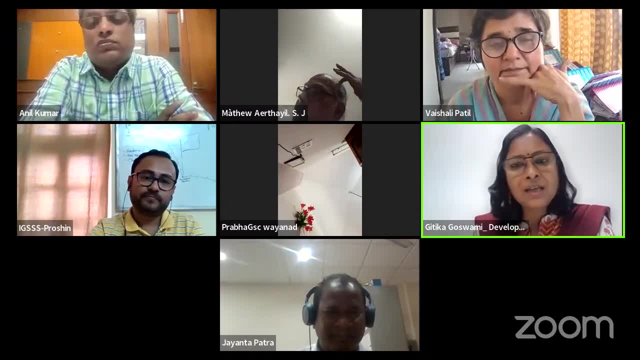 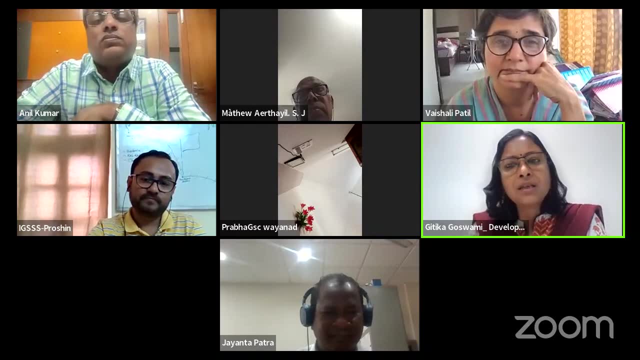 and which, if this main member can see that, yes, this is profitable and the women member are getting really cash, hard cash, in their hands and they are managing that, can only, you know, pull them again to the village. and in case of west bengal, in bapura, purulia district, there are examples where 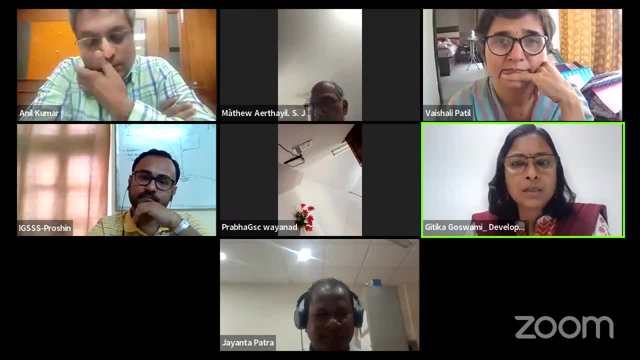 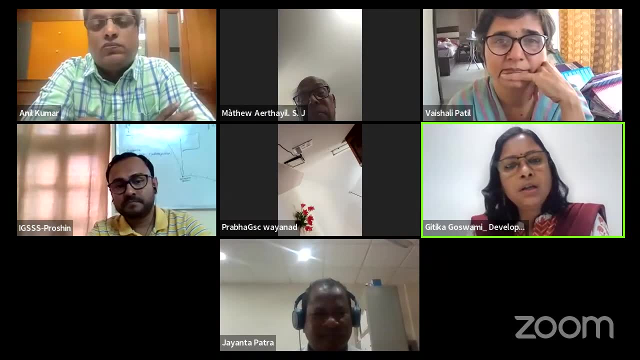 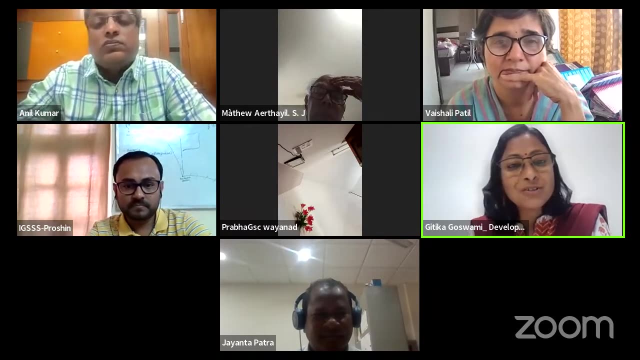 the husband then stayed back with his wife and started doing this trip, three, four types of livelihoods. earlier they used to have one crop, now they are getting with the goat and the poultry, and those they are not only. the women is not only empowered and not only getting. 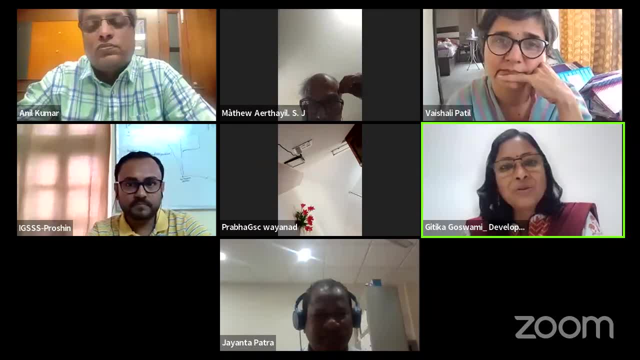 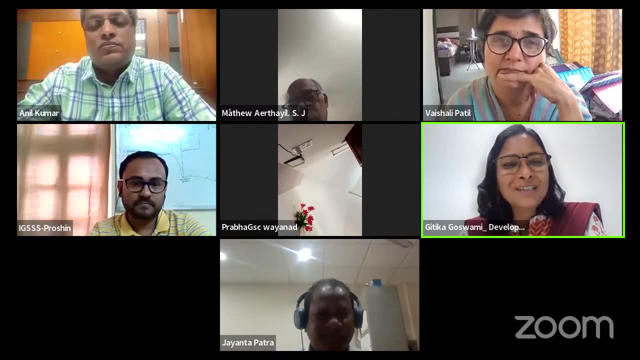 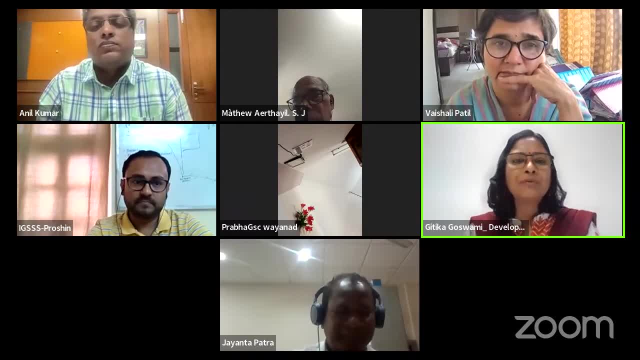 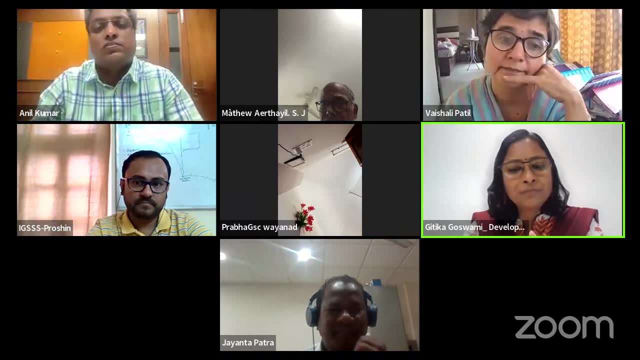 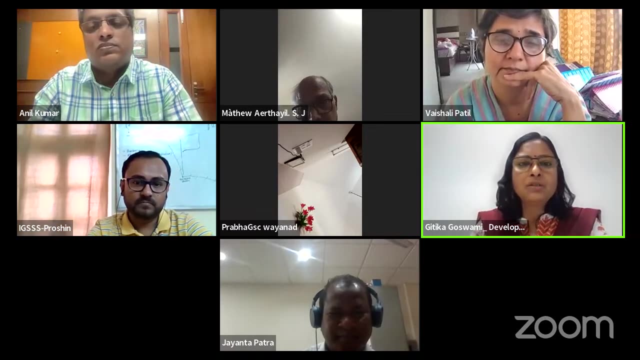 benefit of the family. so i think these are some of the examples we have to as, uh, you know, i also said- and, um, the sister also agreed- that we have to do some, you know, different, uh, different strategies have to be taken and also make partnership and network. that's, i think, the motto of today's life. 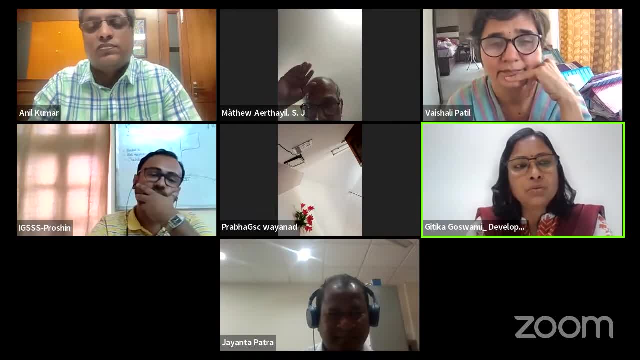 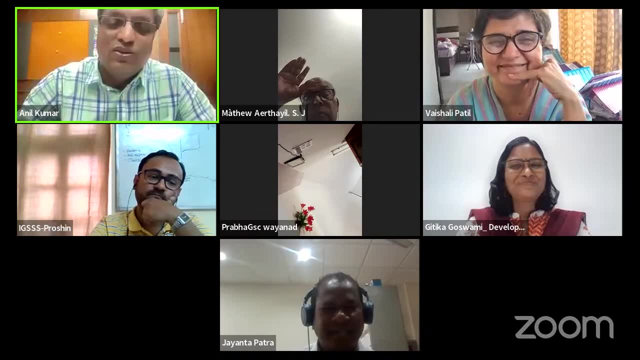 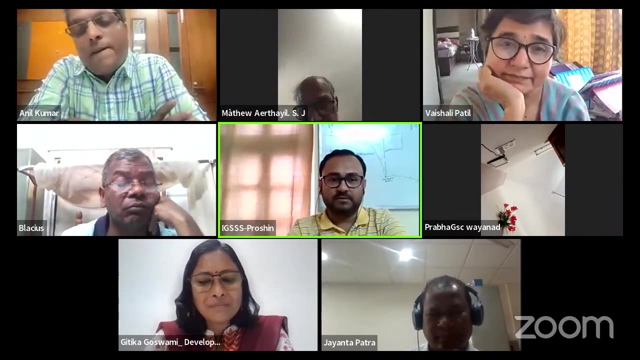 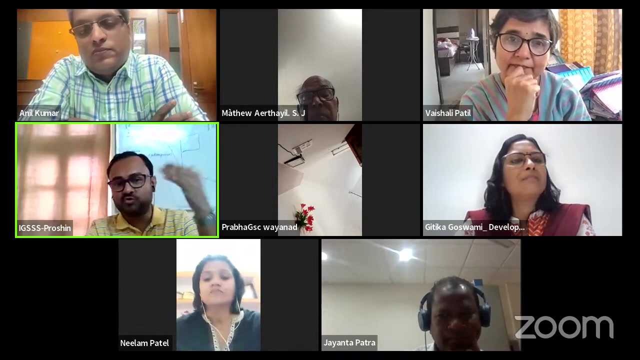 you know we have to work together and then only we'll be able to really do and sustain in this world. with the current scenario. yeah, thank you, thank you. i just want to add with the: basically, you know that we need a climate resilient, like, okay, so uh, today it is planet resilient, but it's 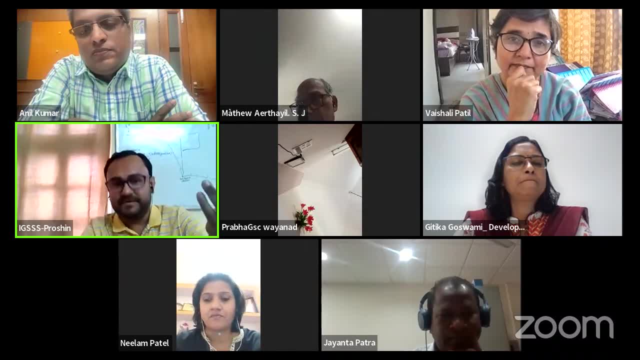 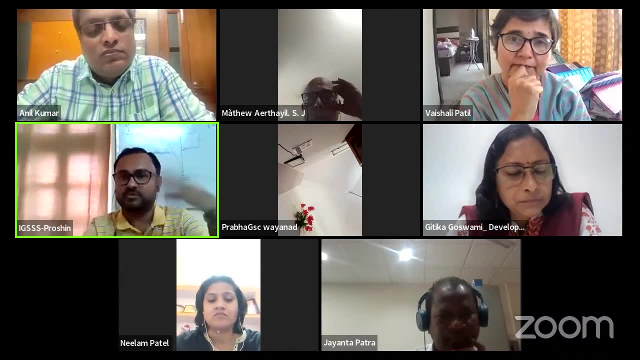 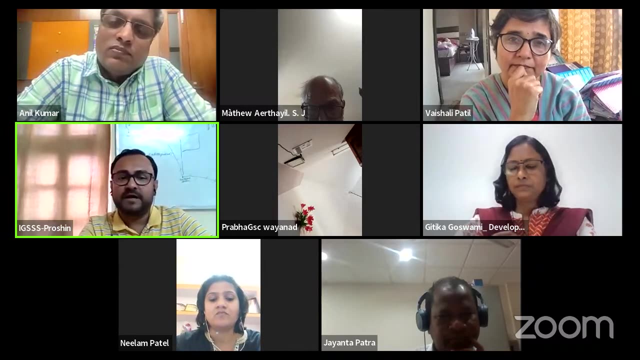 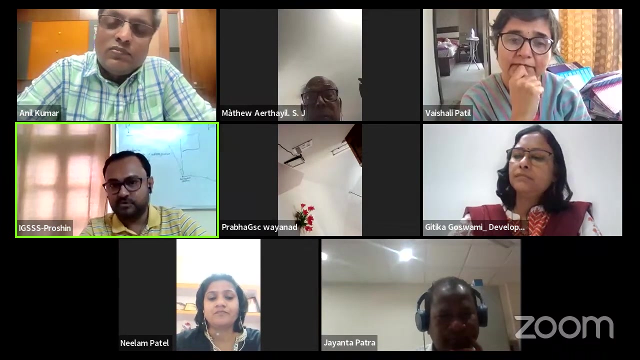 not mean that after, uh, some years, it will be climate resilient, climate resilient, but climate is very much up and down, so changing. So your situation, I have understood your situation and I want to send you something, if you give me the email id, because we worked with this PMTG group earlier. IGSS and IGSS. 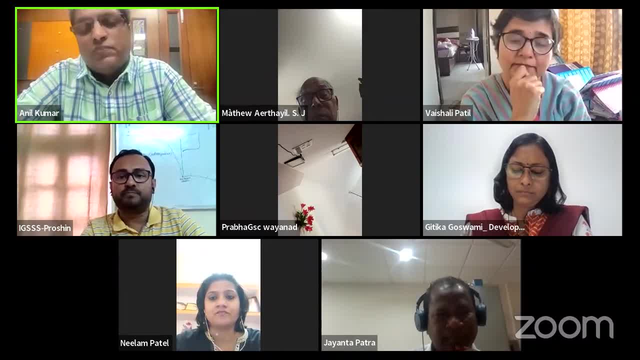 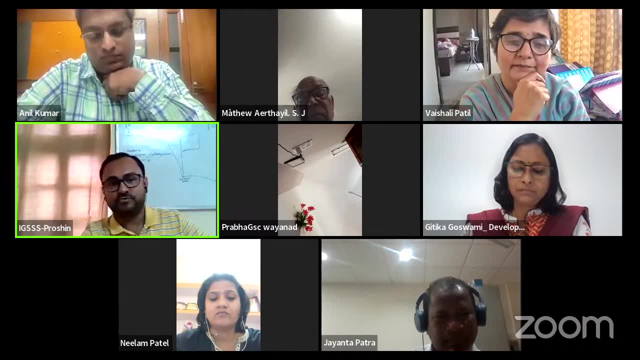 had a good experience in this and we have a good knowledge for that, so probably it will help you. So if you give your contact, or maybe I can send Anil and Anil will send to you. okay, Thank you very much. 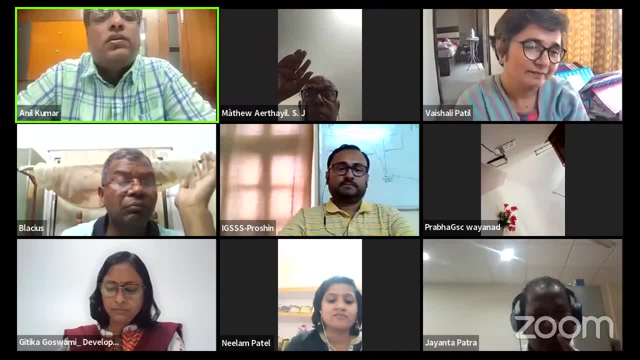 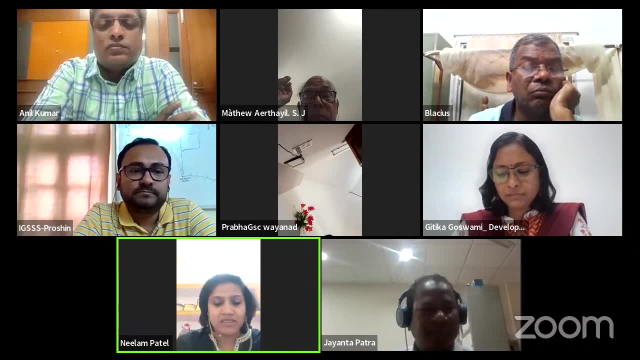 Neelam, you have any questions? Yes, Anil ji, Hello everyone, My name is Neelam Patel and I am from Pratipat Foundation, from Banaras, UP, And UP is said to be a big province for the production of vegetables. 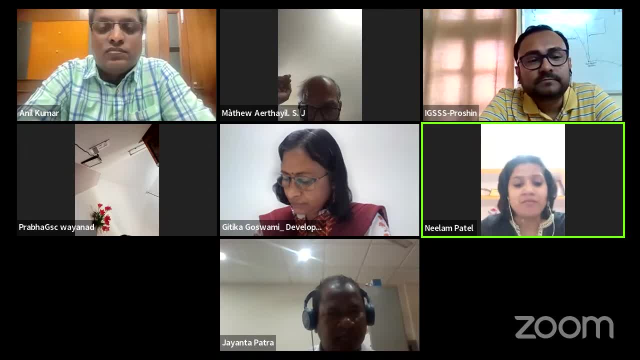 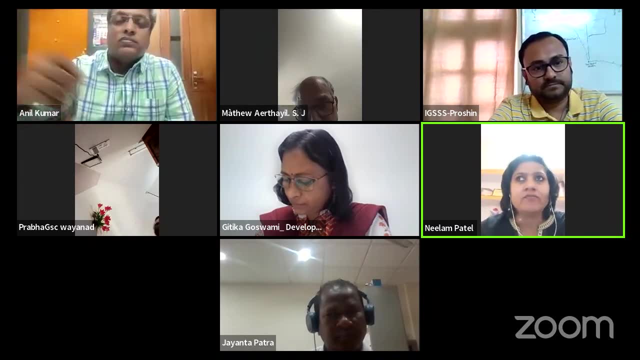 But my experience in Banaras is that slowly, the production of vegetables is getting finished, So I am very happy, But the problem is that people are migrating. It might be because of the lack of soil in the soil And because of which vegetables are not getting produced and people are gradually migrating. 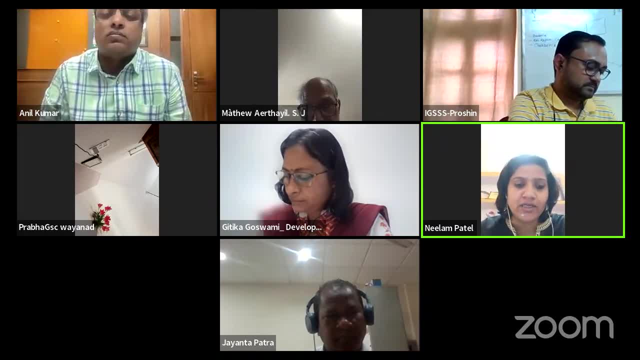 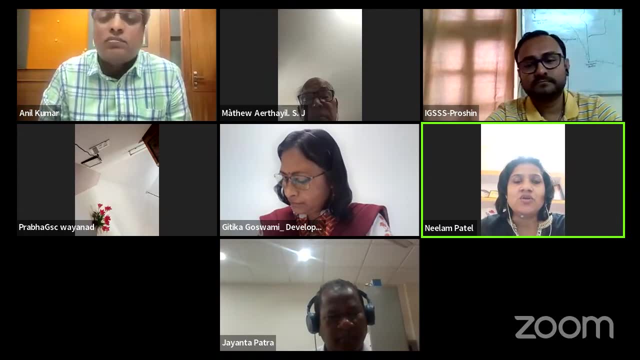 to different states, different places or different jobs, Because of which most of the farmers here were farmers and they are selling their lands without being farmers. So my question was that, because of the climate change, do you think that the economy is going? 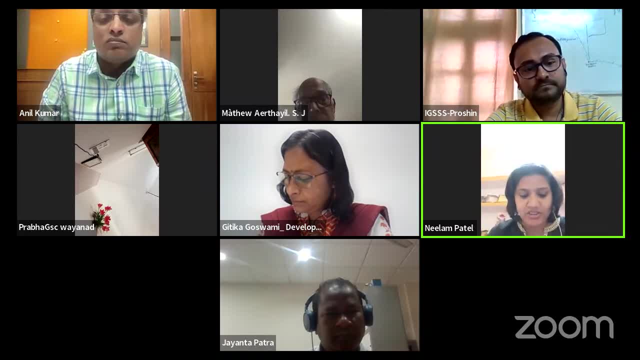 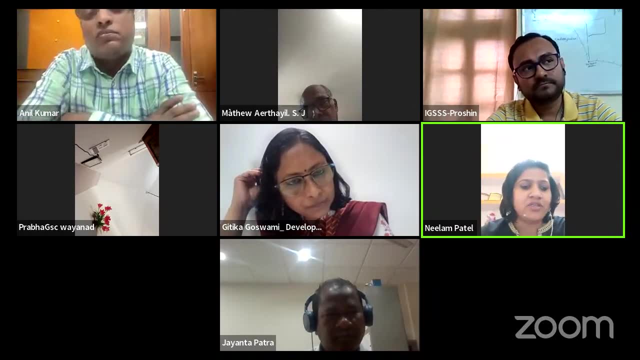 to be better. Yes, absolutely Yes. Because of climate change, the effect of vegetables on the fields is increasing. More than half of the vegetables in the fields are getting spoiled or it is not happening as per the time. So what can we do? What is the solution? 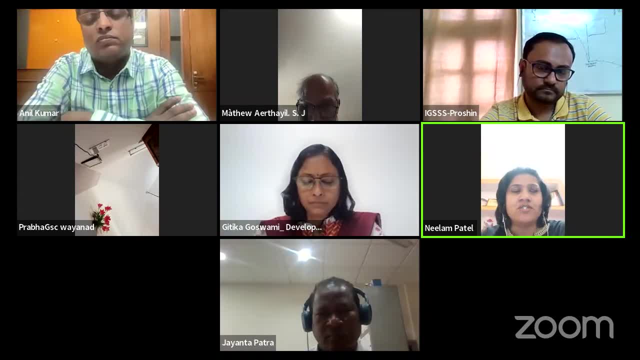 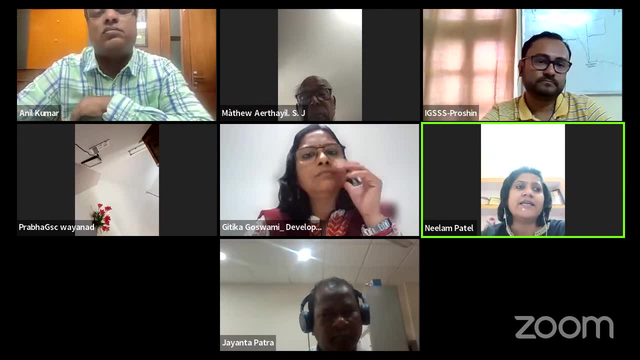 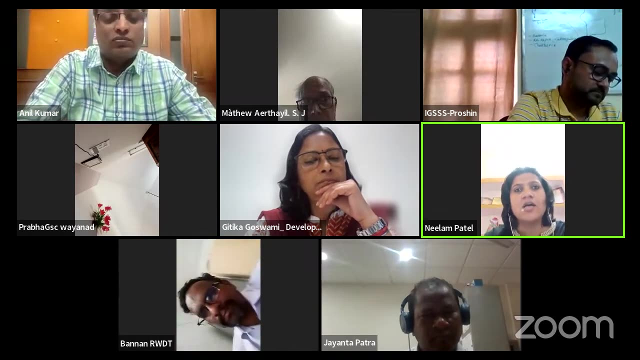 The farmer who is farming and his whole family is dependent on the vegetables. On the one hand, he has a whole life, So how can we give him a solution so that his vegetables are better and the effect of climate on his vegetables can be eliminated? 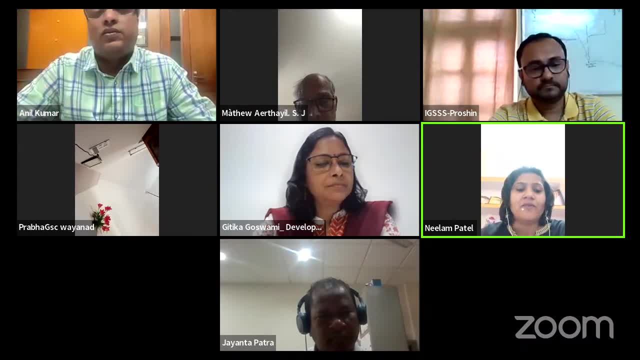 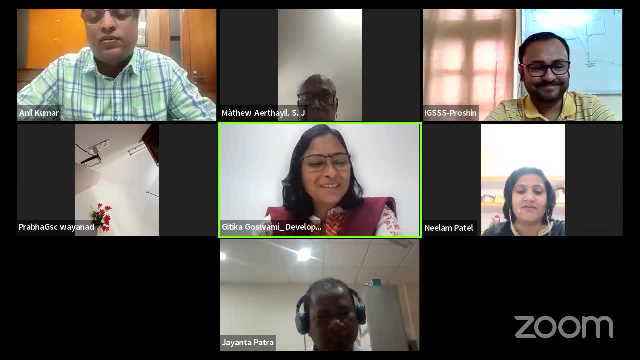 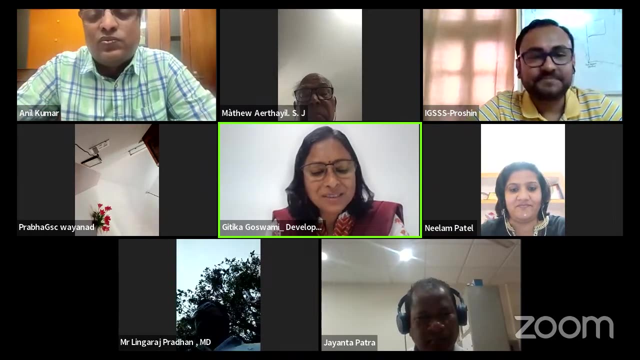 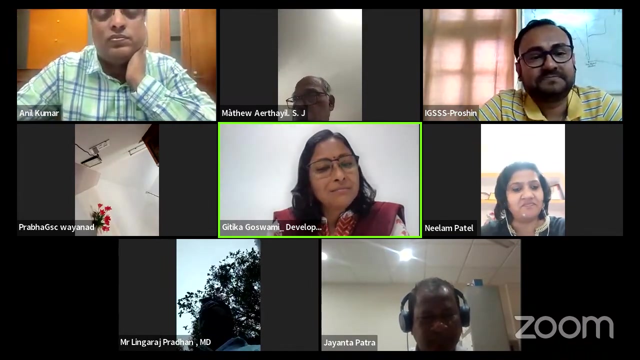 So this was my question. Ms Nitika, would you like to start? I think, yeah, we can, I can. I think all of these questions are very, very much, very much similar. Migration is an issue and people are going to cities for earning hard cash. 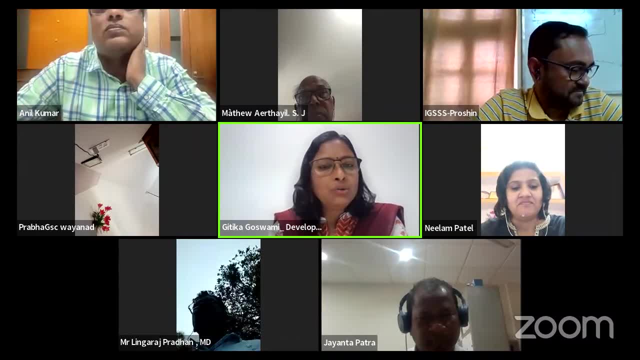 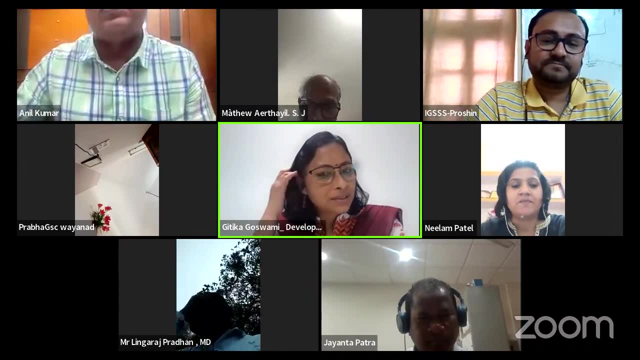 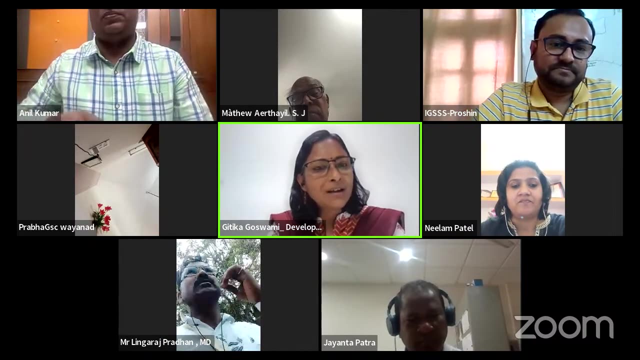 Overall, if you look at it, people are having more cash availability when they are migrating to the nearby cities And in many cases it's kind of a ripple effect. If one person is going to one family and he earns more, then the surrounding families are also starting to do the same. 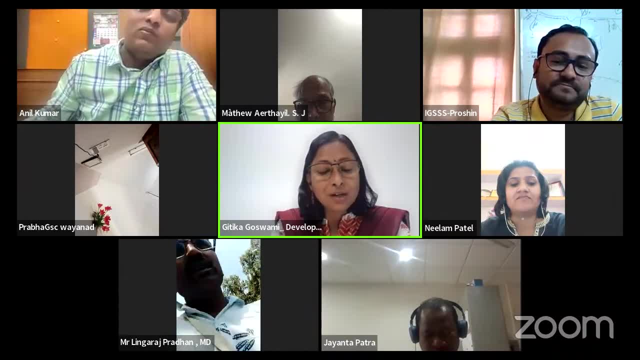 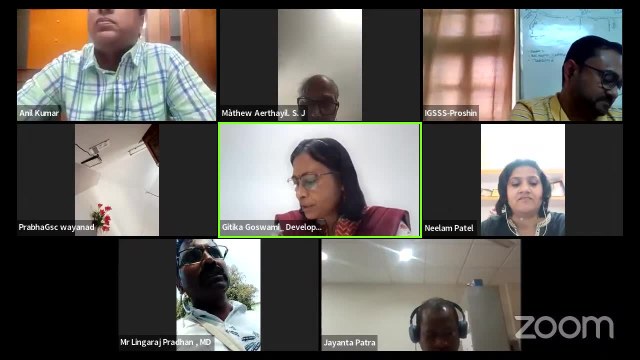 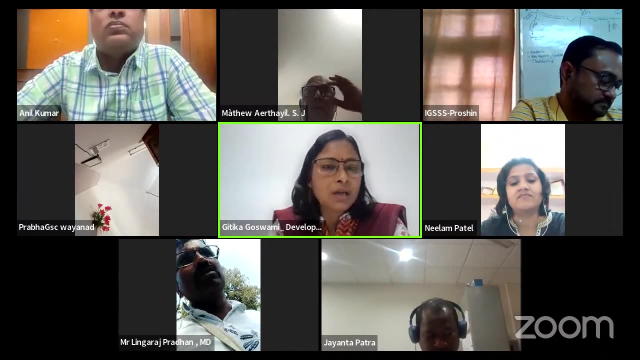 They also say: let me also go and I will also work. That's the issue And I think what I have already said to my earlier response. I feel that we should work especially with women, And you are talking about vegetable cultivation And vegetable cultivation. if we can really do the different kind of cultivation. you know, too much production and using too much chemical fertilizer. That was last 10,, 15 years, 20 years. I think that became the trend And due to that we are really 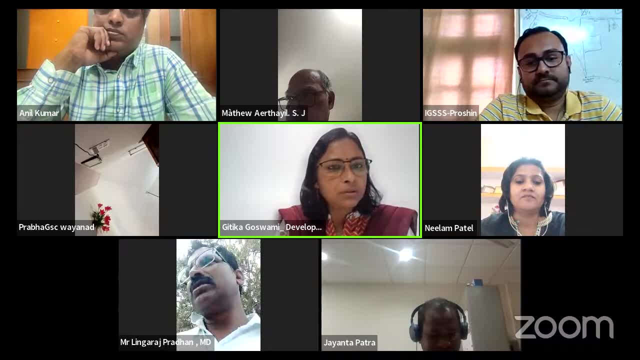 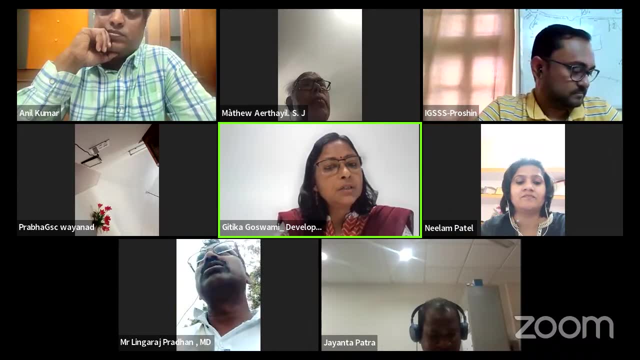 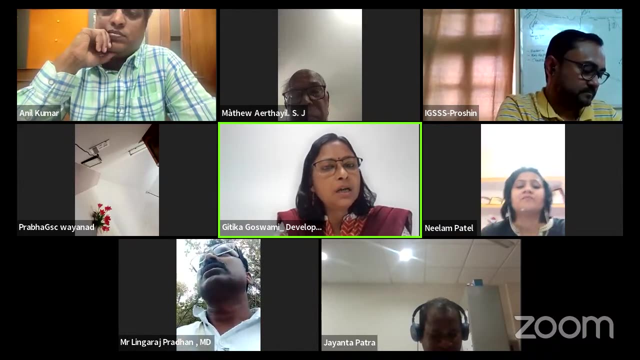 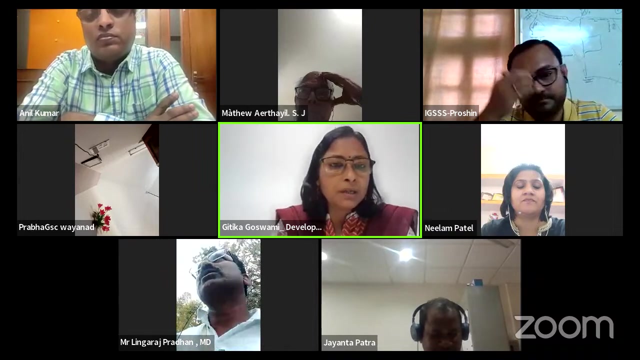 that soil quality is increasing. And once you use chemical fertilizer then its input cost keeps increasing Because the actual quality of the soil, the quality of the quality of the soil it gets completely ruined. So if farmers know this, even in many places 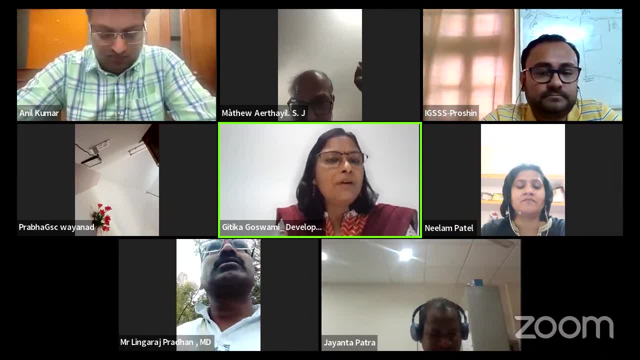 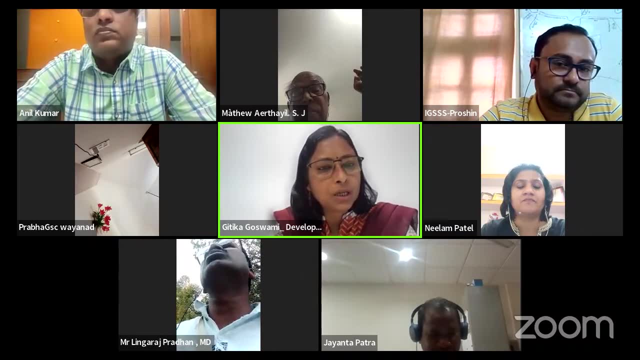 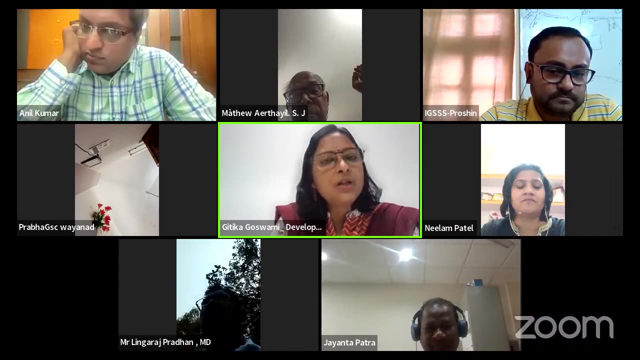 Farmers do not use chemical fertilizers for their own family. They use it for commercial purposes. So it is possible that if we start the practice of natural farming with some people in the new areas, then the production will be less for one or two years. 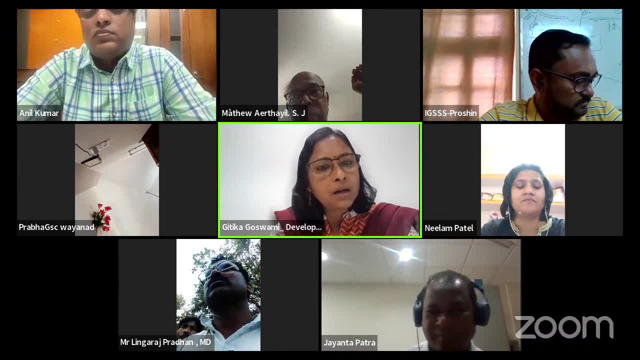 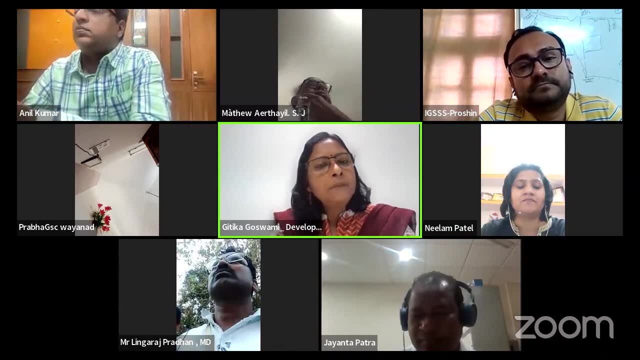 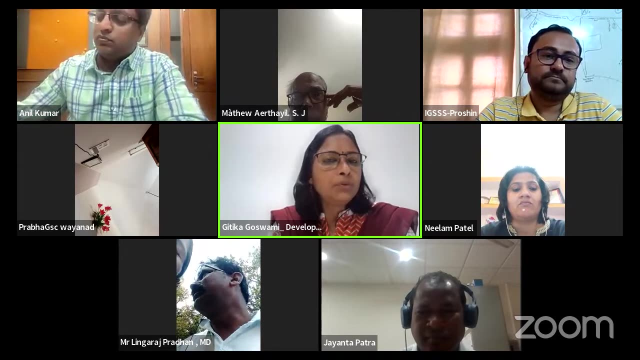 But it will be good in terms of quality And if we slowly convert it into totally organic agriculture, people's health issues will also get better, And in the first one or two years there will be some losses because the production will be less. But ultimately it will be good for the climate because it is a natural farming And now I think the government has asked a lot for this. In terms of JB farming, it will be good. Sprinkler irrigation means you have to give less water. 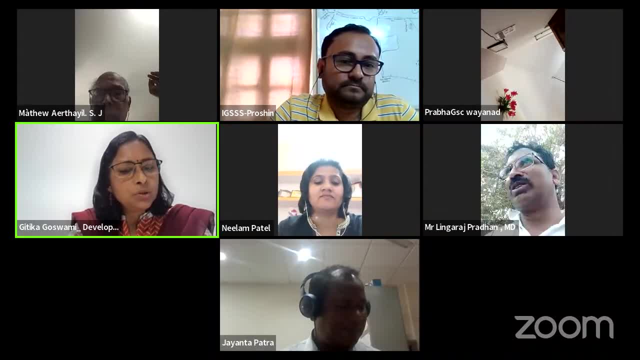 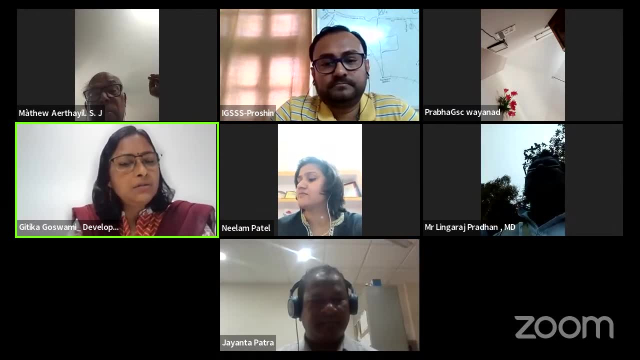 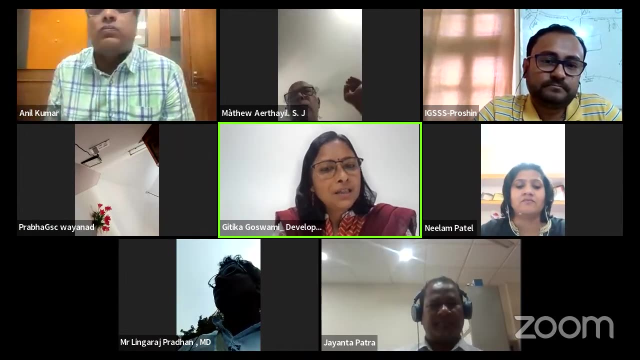 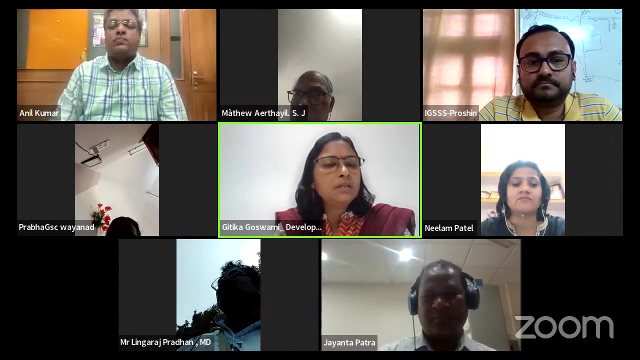 Solar irrigation. These schemes are very important. Under these schemes, maybe you start with only the women members of this in a small village, like maybe 10 villages, 15 villages, Start it a little. I think It will not happen in one year. 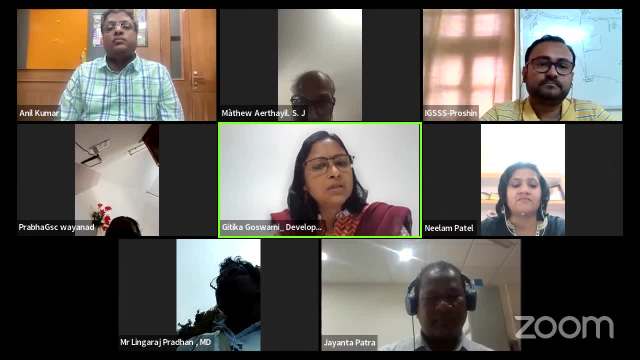 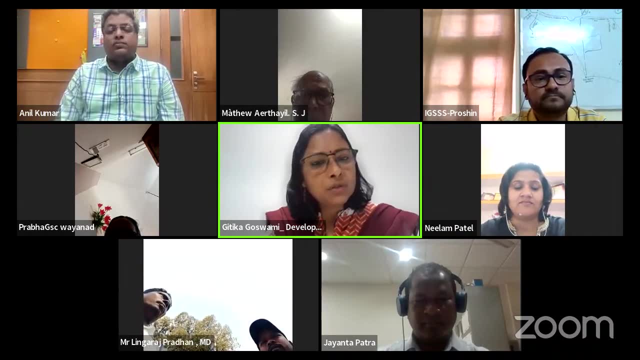 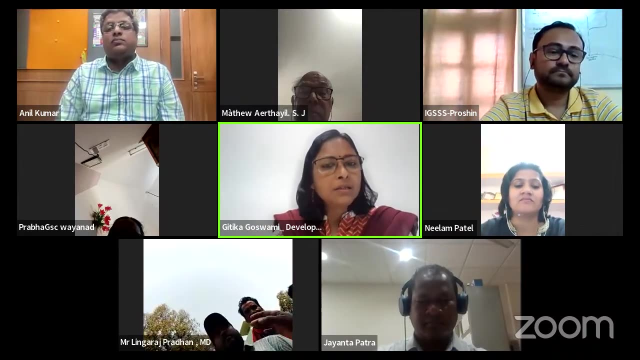 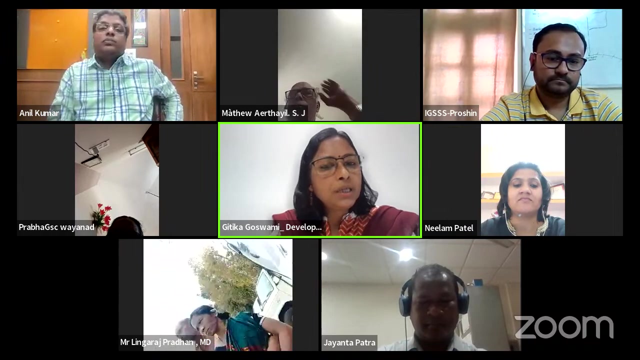 But in two or three years it will start looking good Because in the first three years, as I told, it will have the reduction in production, But ultimately the quality of the material would be good And nowadays people in Amazon and other cities want organic agriculture. 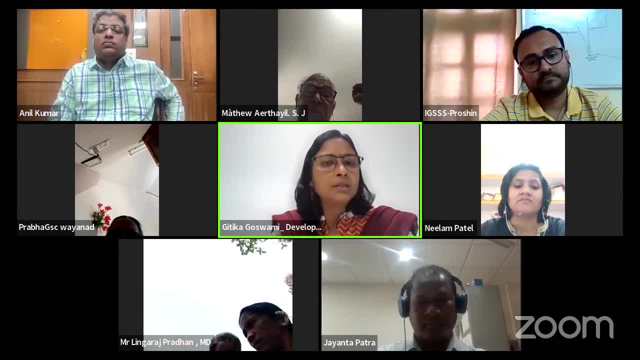 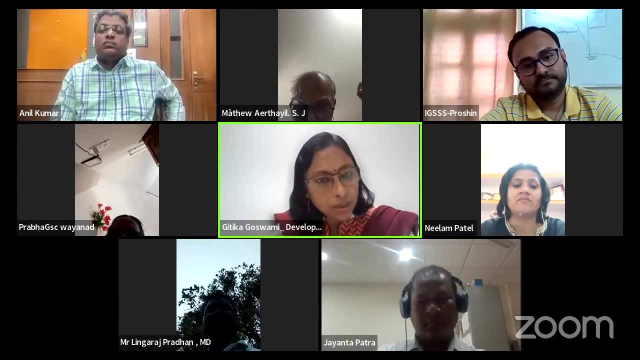 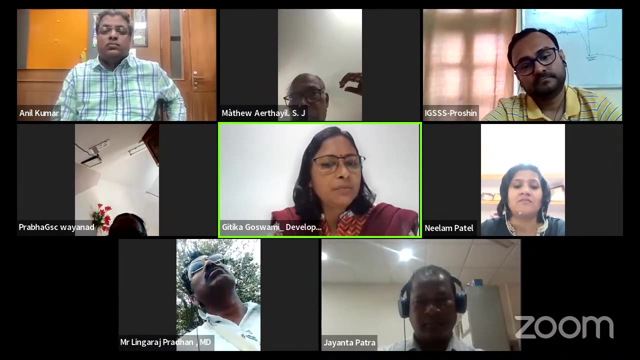 So how far do people order from? And there are a lot of such enterprises that are being built now By doing this farming, by making a niche market, by supplying people online, really making a profitable business. Maybe we can kind of think that way. 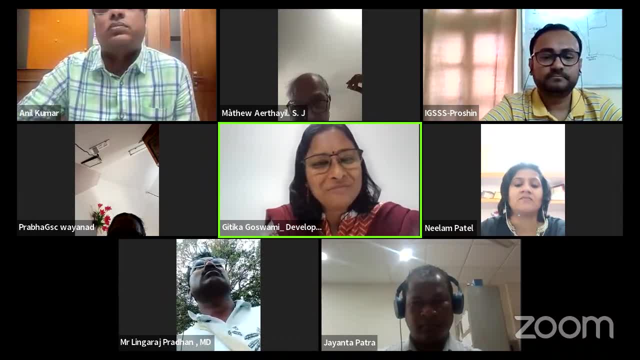 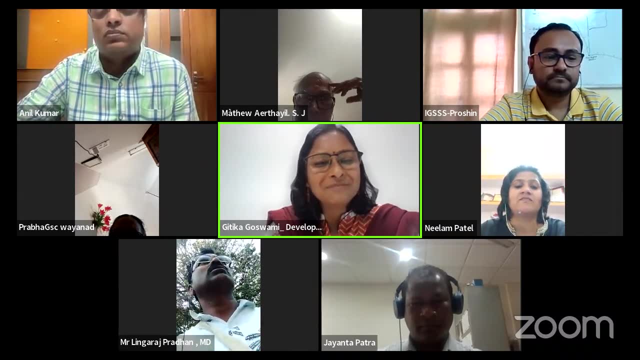 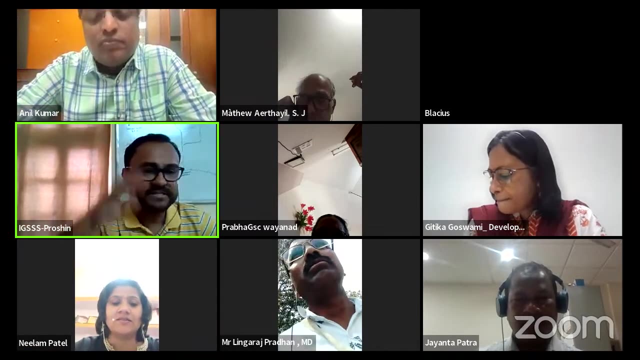 This is what I can only say. Yeah, But we can be having discussions, We can continue to have this discussion. Thank you, Just adding to Geetika. Thank you, Yeah, Just adding to Geetika. Basically, something that came in my understanding is that weather forecasting is very, very important. 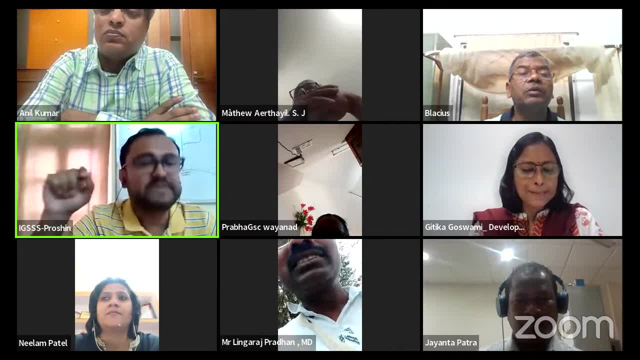 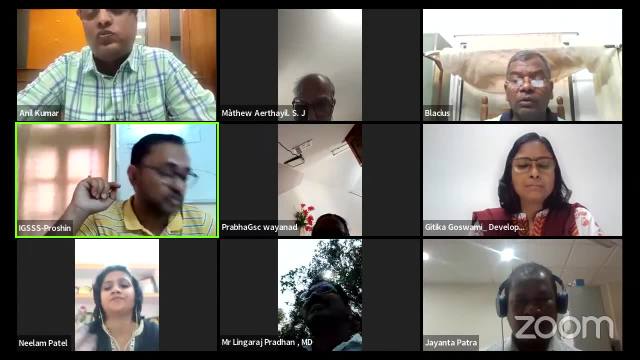 Because now there is a link of the government, there are government numbers from where you will get advice, from the weather advisory that is the Ministry of Agriculture. Okay, So weather advisory, Follow it. This year, in Maharashtra, when it rained, it didn't rain. 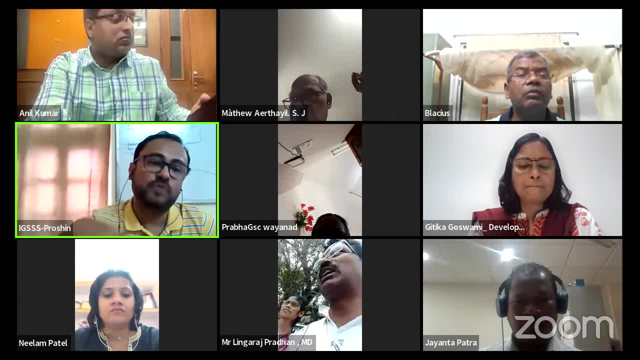 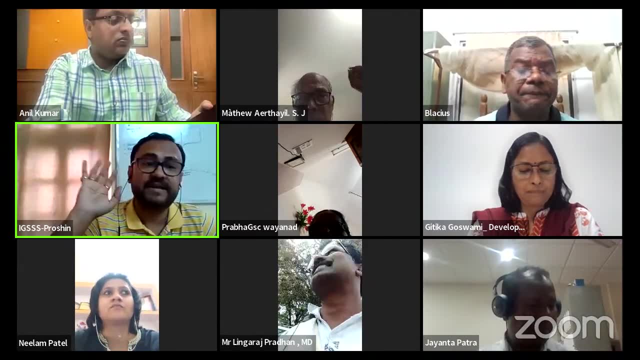 It went back. It went back for two or three months. That's why a lot of crops were destroyed. So please follow the weather advisory. The weather warning will also come from here. Okay, And don't just follow it. I mean, in the village people, I mean farmers, have to be intimidated. 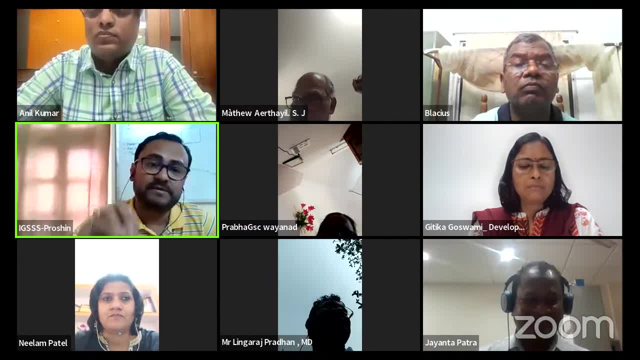 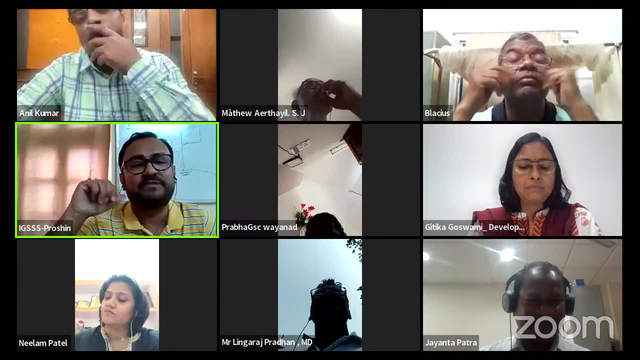 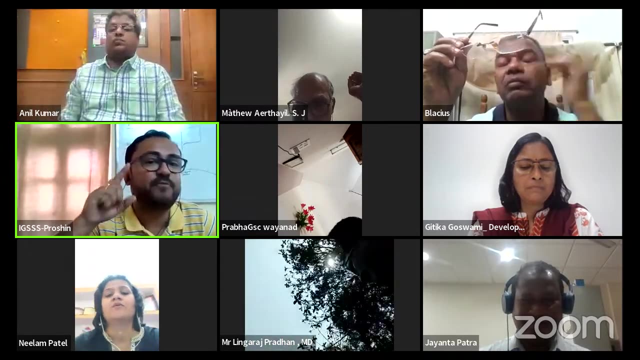 This is the process and this is the thing. You can get the information from this so that they can update and give these things Number one. So you have to do some multi-cropping. When you do do not do it in one crop, it is very important to do four or five crops in. 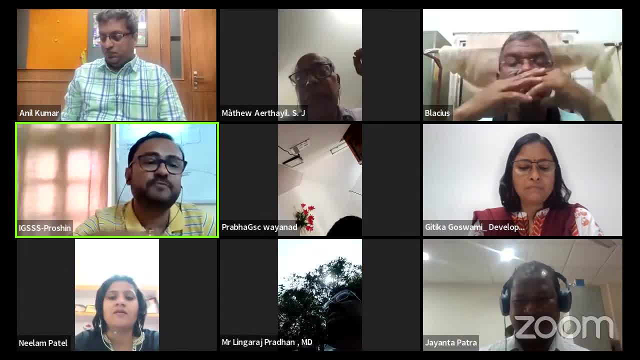 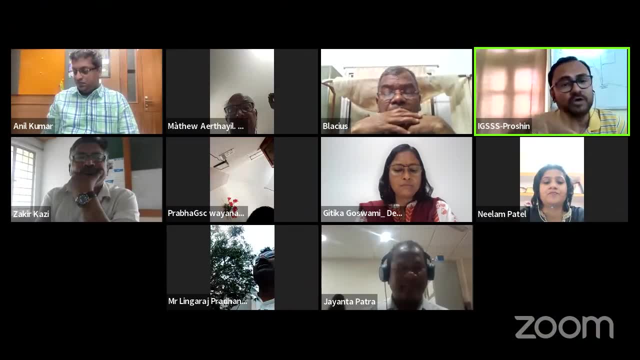 one field, because what will happen if it depends on one? One is over and gone, So you have to multiple options And the another is one is very important. that agroforestry model is very important because there are a lot of things together: there is horticultural things, there is a vegetable. 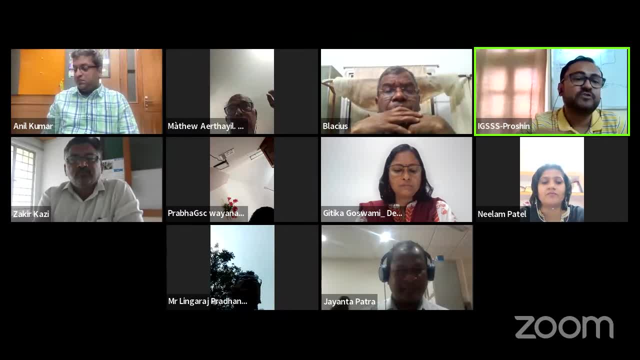 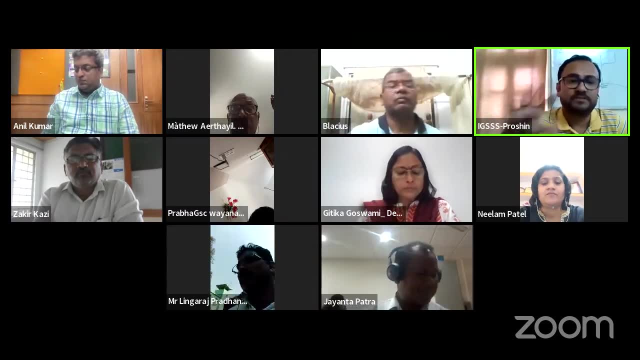 thing. there are a lot of things together. So what will happen in this? What will happen in this is that you will get an alternative way. One is over, one is ruined, then the other one will work. So these are the things, some strategies which you can follow. 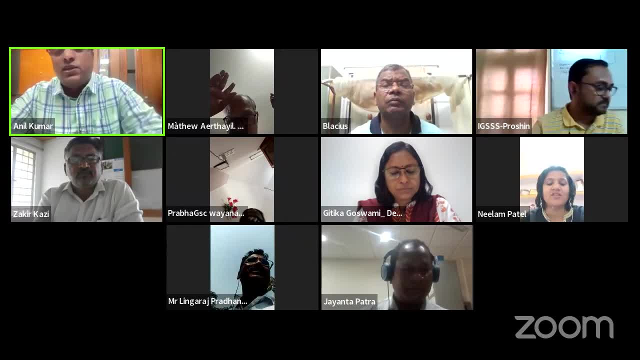 Yeah, Thank you. Thanks, Divya. the question No. Father Matthew, Father Matthew, please, Yeah, Matthew, working among the tribals in Atrapadi Palga district, Kerala. First of all, I congratulate you. 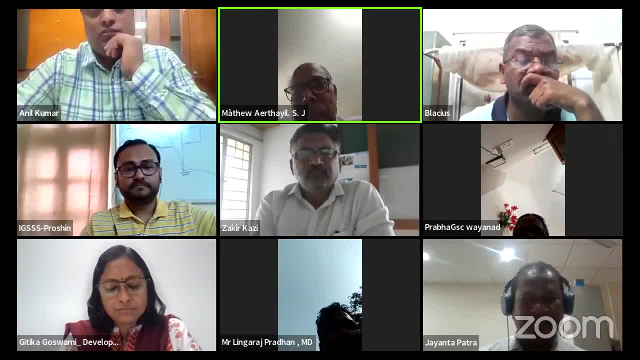 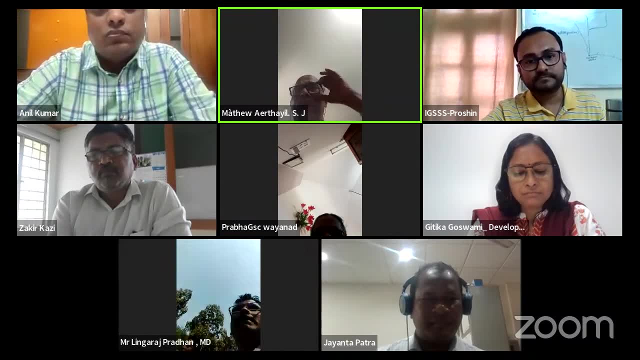 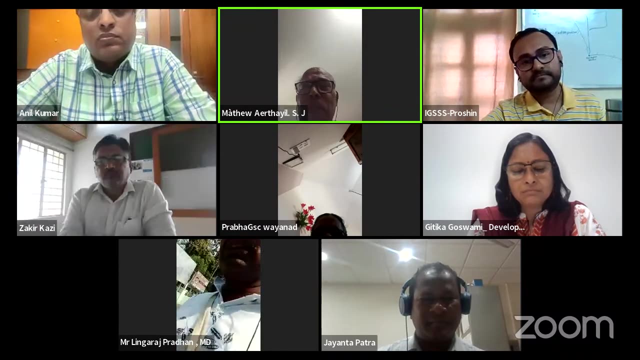 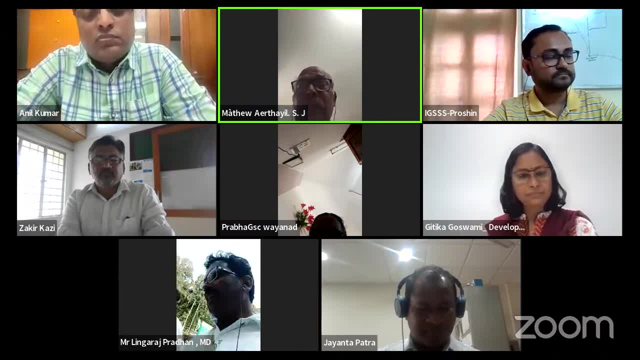 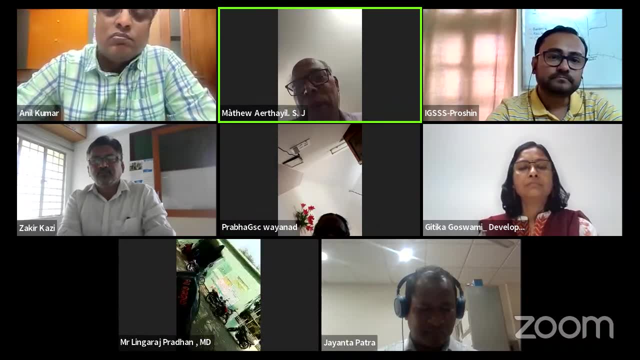 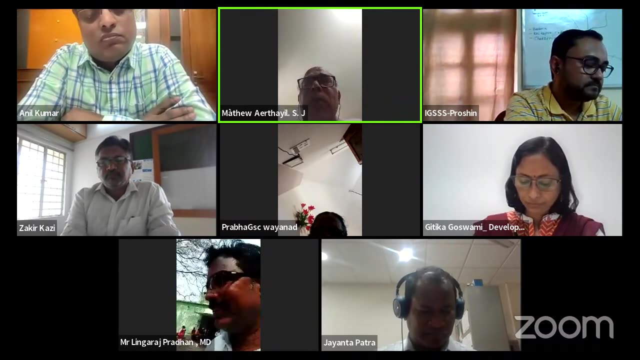 And I know moderating the whole thing very well. We have in Kerala three units. What units? Unit of Lough Bench, working among the coastal people, fishermen That is called about, which Sister Mercy mentioned. Actually it is a sea erosion. 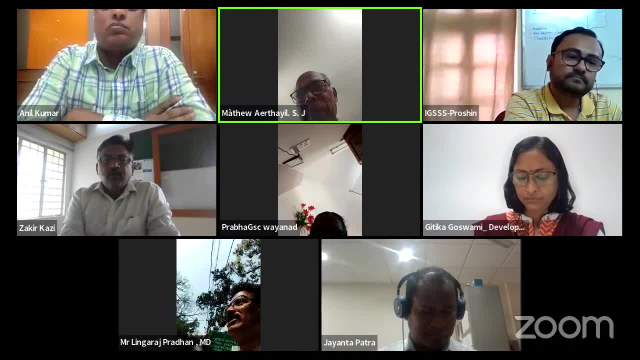 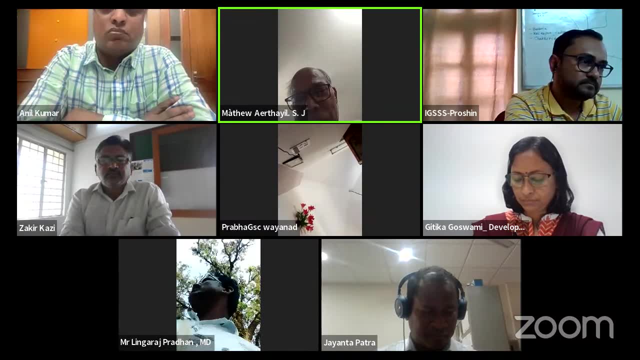 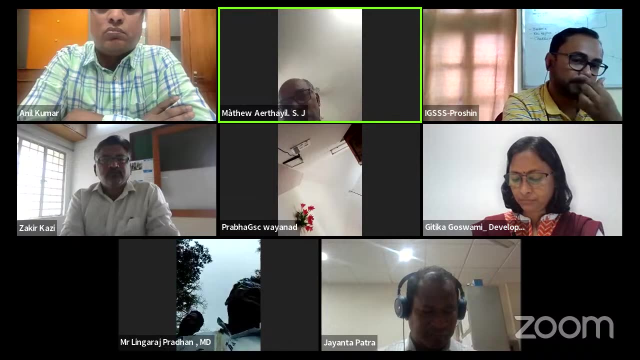 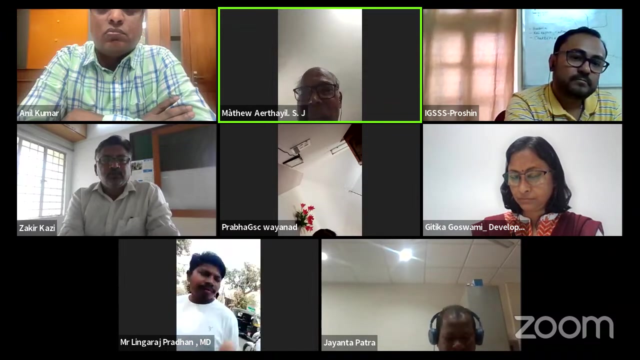 also added by the construction of the international port, which is called Virinyam Port, against which the fishermen in the south had a very long agitation, about two months agitation, including the church, and it was all suppressed. It is Hathani groups. 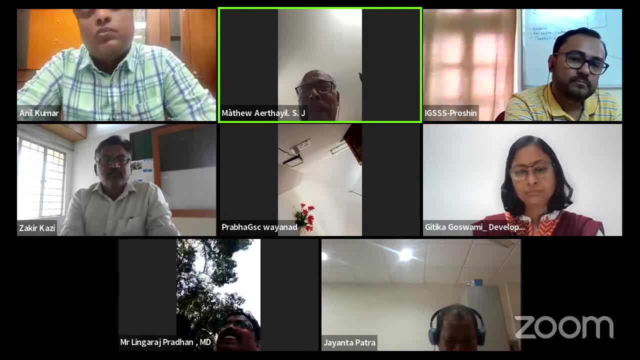 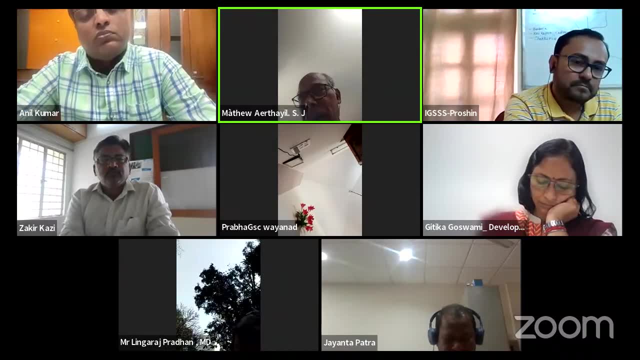 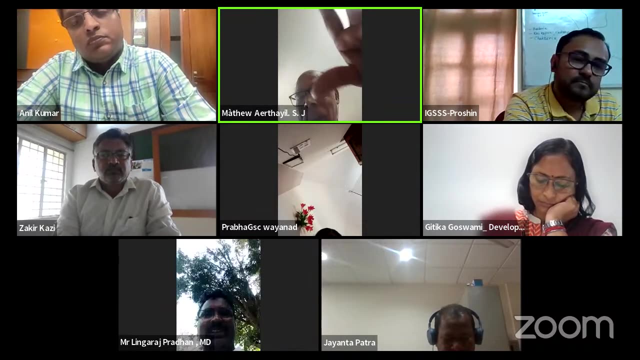 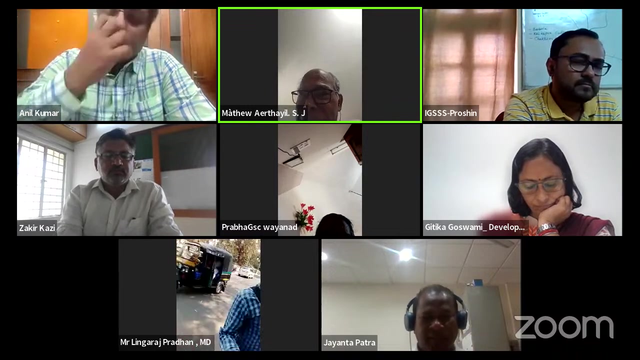 which constructs the international port. Now the other two groups are working among the tribals, One unit here in Palakkad, the other one Wayanad. So now I am speaking about the tribals They had actually many of them do not have land. 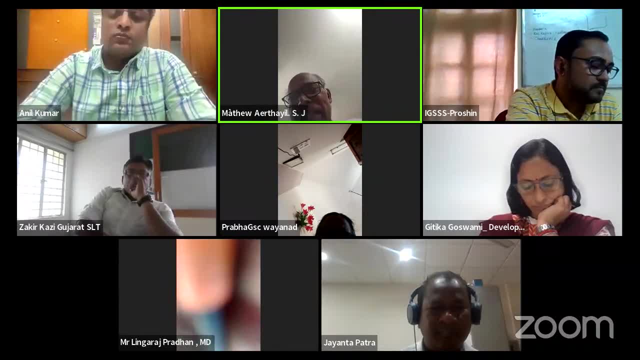 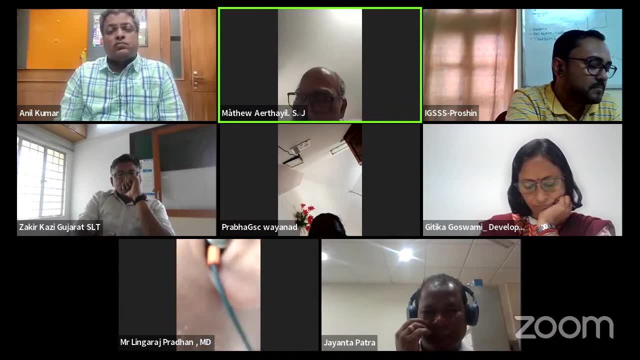 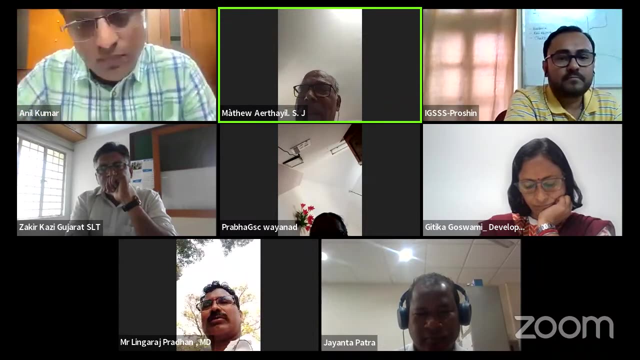 Those who have land. they are not of good quality And therefore their traditional cultivation, especially millage, ragi and other things, are not much now popular. Therefore they are in dire need. So also in Wayanad. 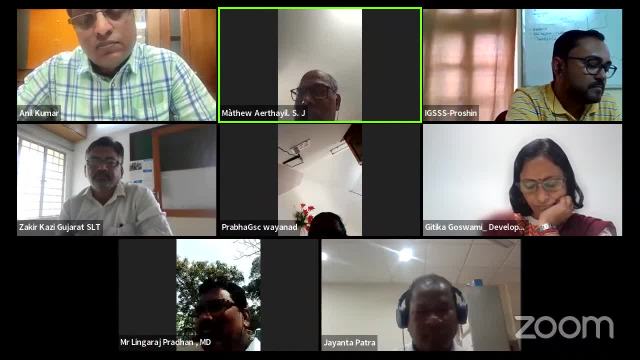 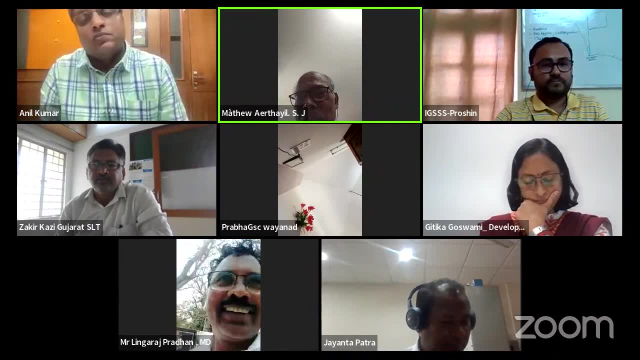 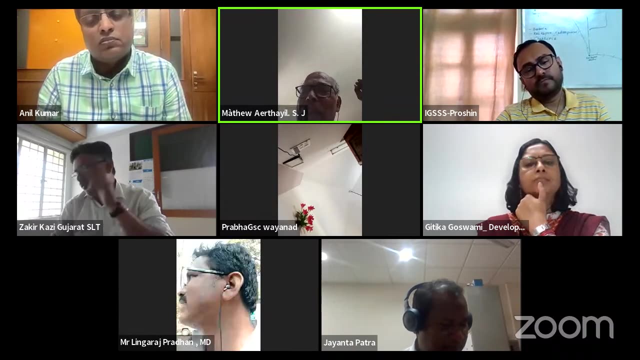 they are not able to live on the cultivation, traditional cultivation they had. The Kerala government started the millage millage, encouraging the millage cultivation, But it remained at the experimental level, especially in Palakkad, in Kattapadi. 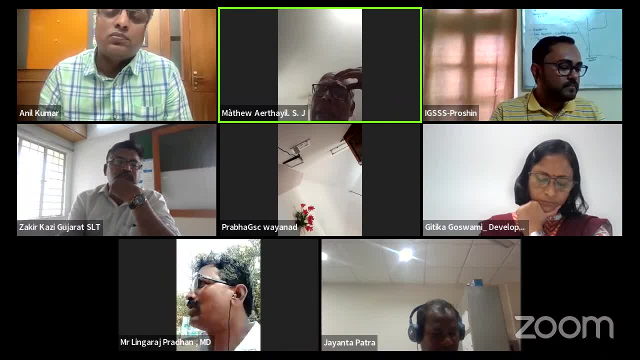 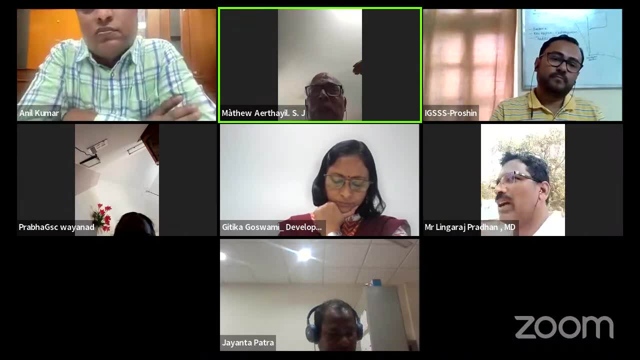 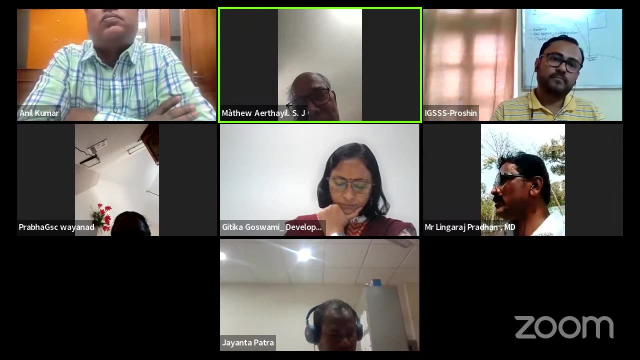 In Wayanad also, it was not there. Now, therefore, the tribals. what we are facing is tribals are not able to understand their problem of cultivation and so on, in the light of the climate change. Recently, we had a talk with the collector of the place. 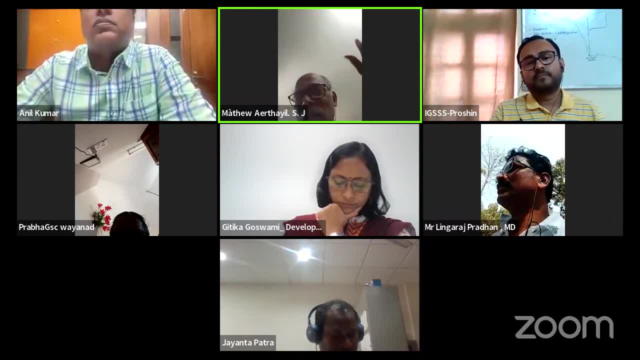 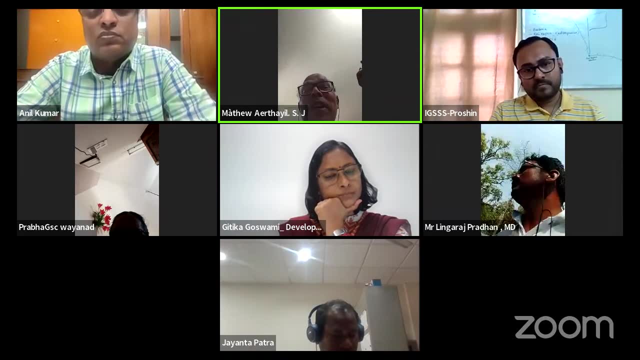 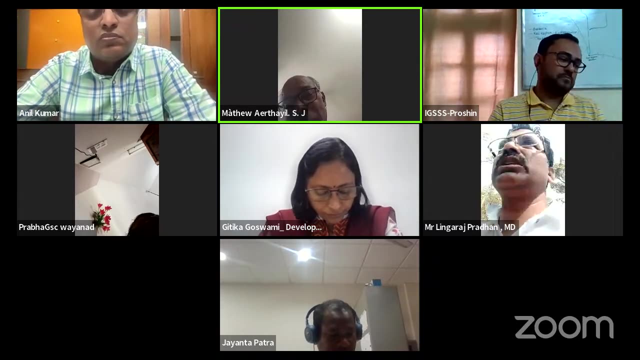 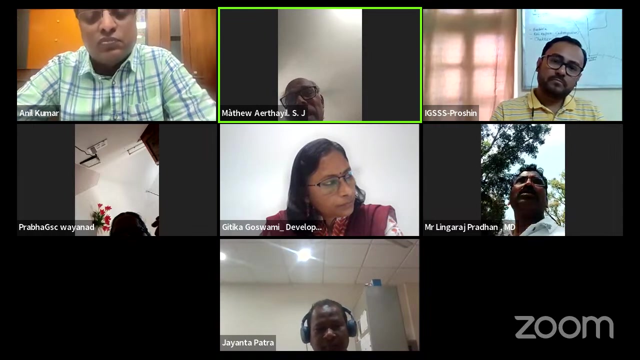 She was totally unaware of this one. They should not understand how the climate change could be part of the problems of the tribal people And therefore make the tribal people understand the connection between the climate change and their livelihood, especially the agriculture is a problem we are facing. 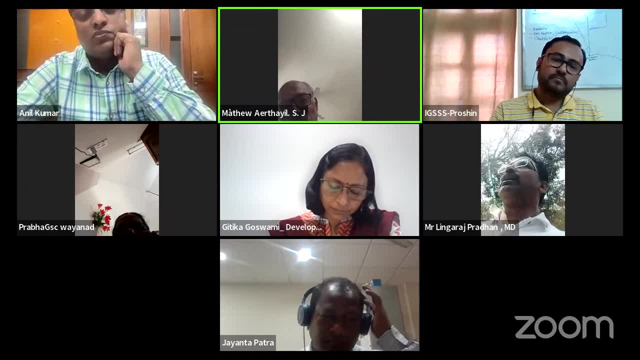 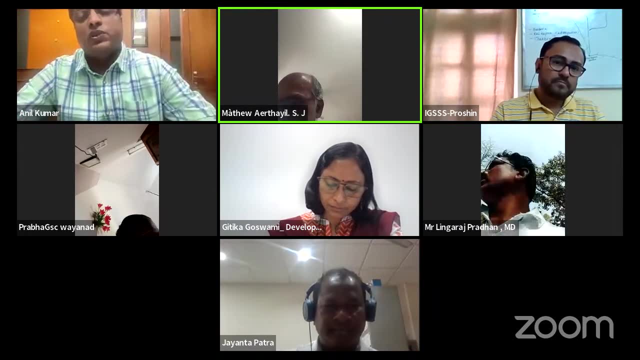 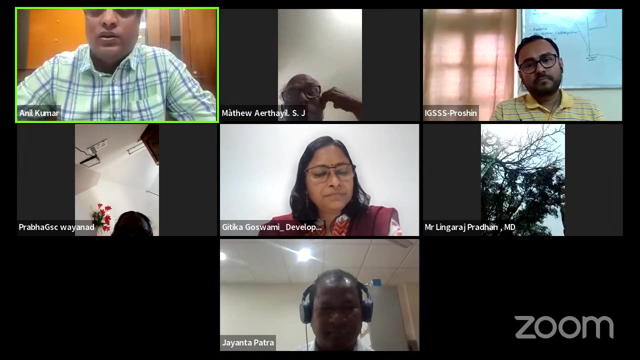 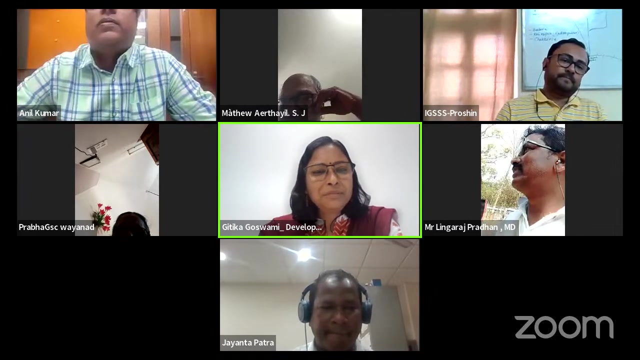 And I am just posing that. I am not seeking a solution as such, but then the problem, posing the problem. Okay, Thank you, Fr. Madhya, And any response from our experts Githiga and Prashanth. I think he already mentioned that. 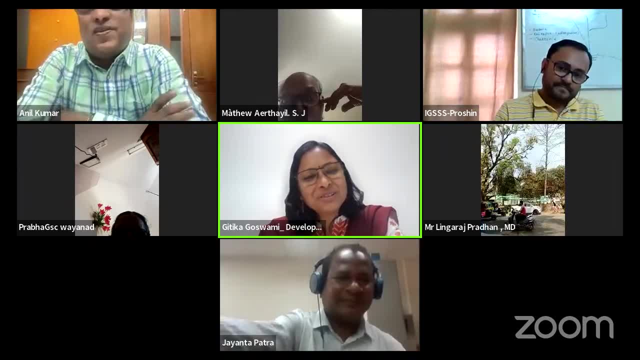 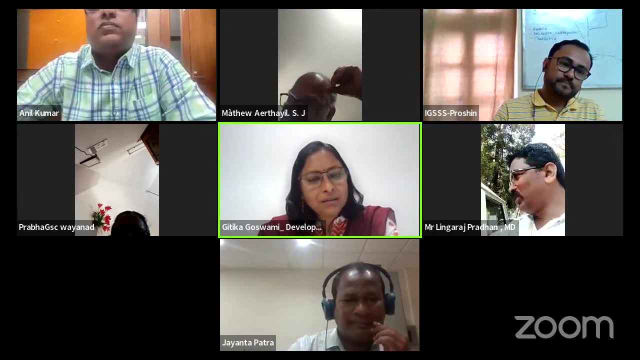 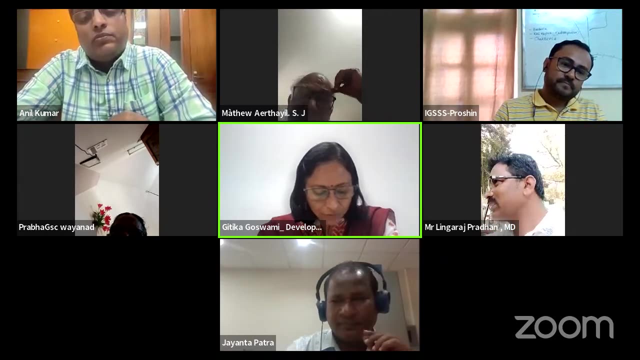 he doesn't need a solution because he is well aware of this. I think one thing we have to do for this: understanding tribals are not able to understand the issues of the climate change and how it is related to the livelihood problem. I think one thing that is very important. 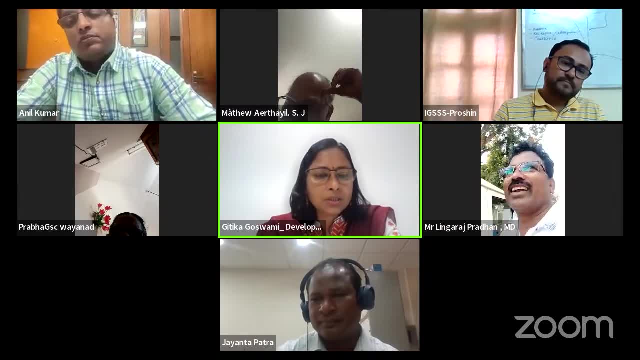 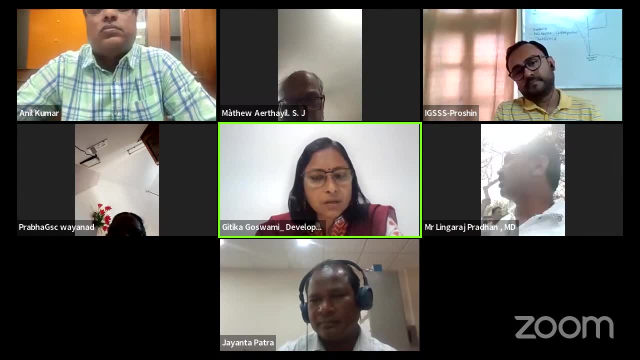 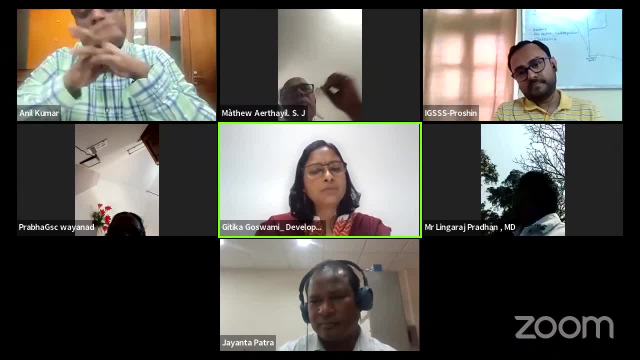 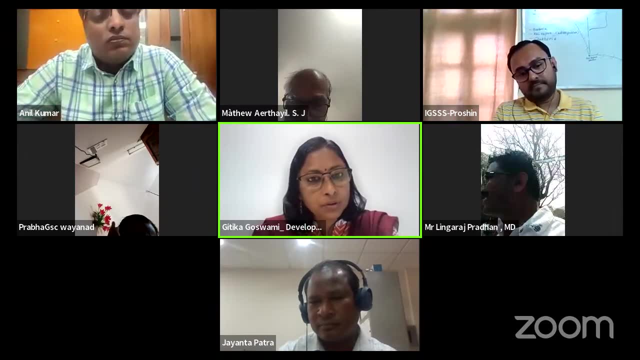 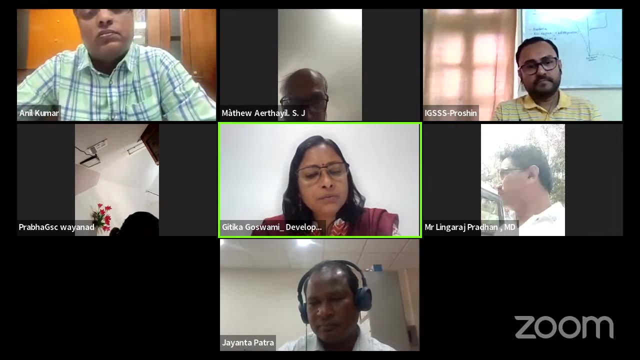 This is important, even if the government has all those schemes on the millet mission, and all those schemes and those millets are part of their livelihood, the tribal community's livelihood, like two decades back or maybe three decades back. I think we have to somehow. 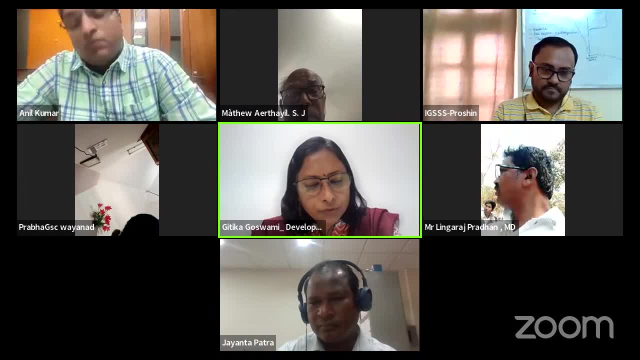 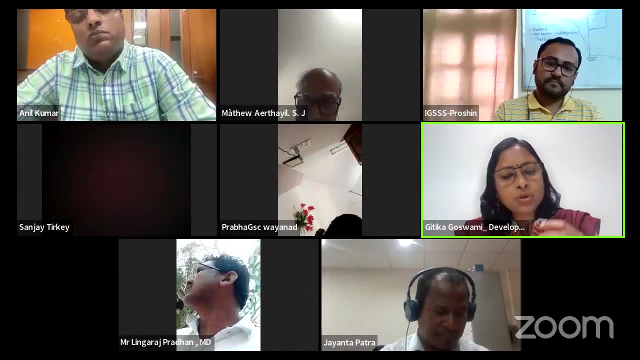 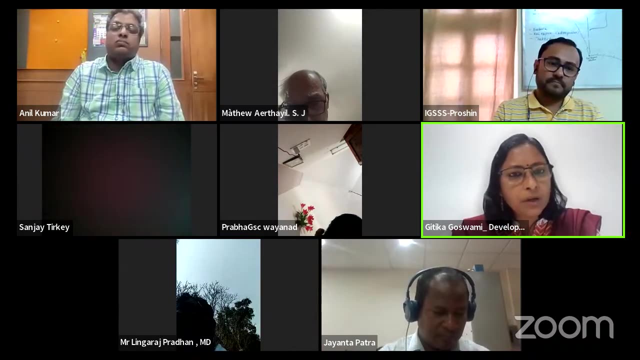 instill the confidence into the farmers with continuous interaction with them, give them. maybe it is also good if we take them and give them an exposure. visit, maybe nearby, wherever it is doing, wherever farmers are coping up or the fishermen are coping up. 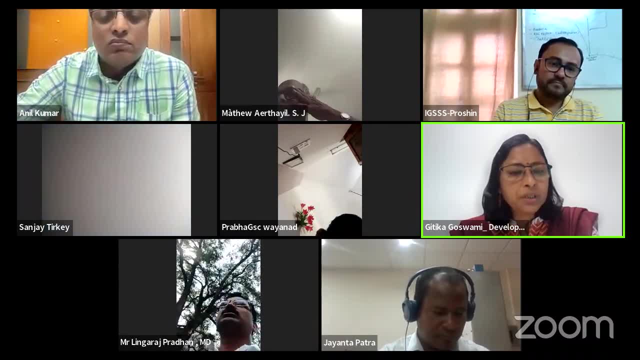 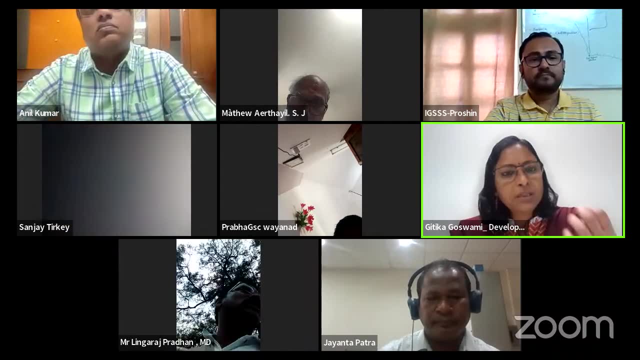 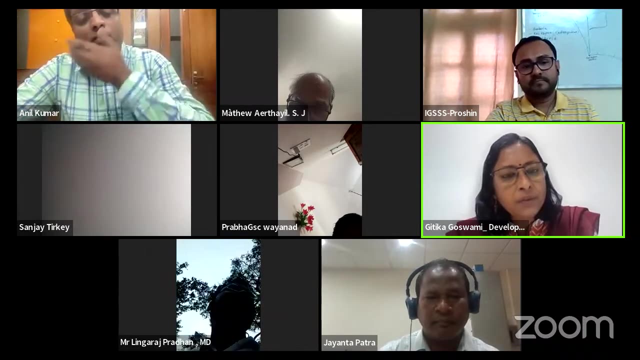 in those problems. I think, if they can, peer-to-peer learning is much more important rather than a top-down approach. So maybe these are five, six strategies that we can take up to make people understand the climate issues and how to cope up with that. 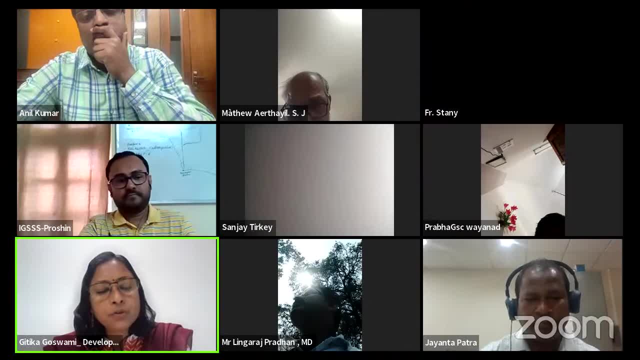 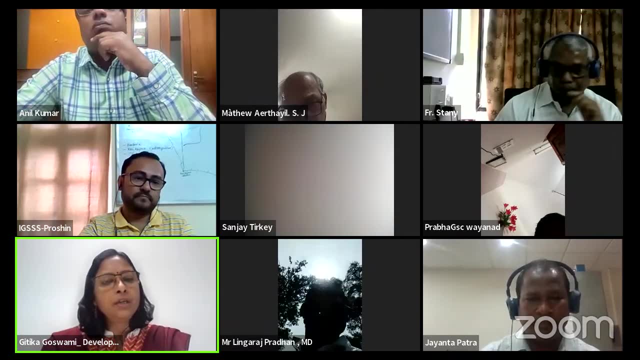 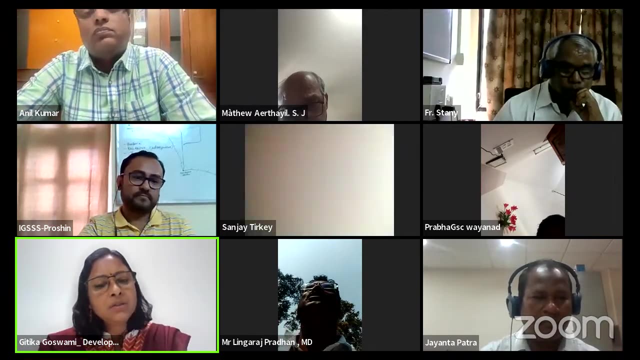 And I think these farmers and the fish and pork they are, they know their area much more than what we know And if they just get the exposure I think their capacities will be built and they very easily will understand. Just we need little bit of time. 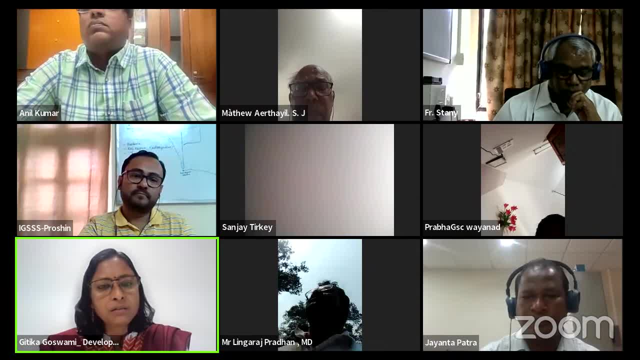 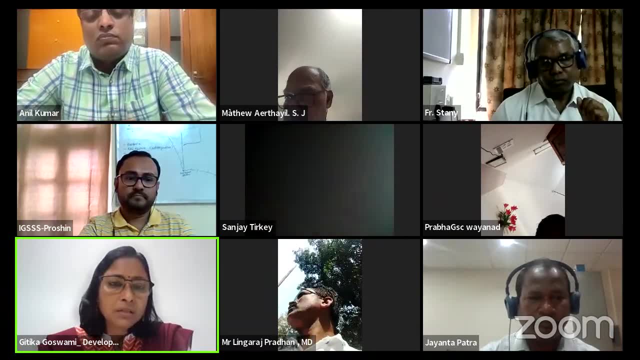 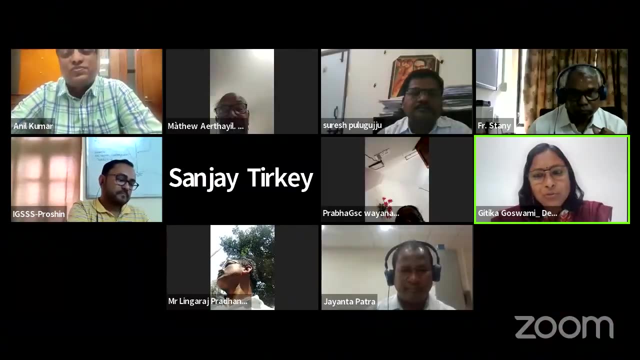 to continuous engagement with them and do kind of campaign, awareness generation, capacity development, exposure, visit, training and so on. I think we will be able to manage a bit. but I know you are on the ground and you know much better than me. 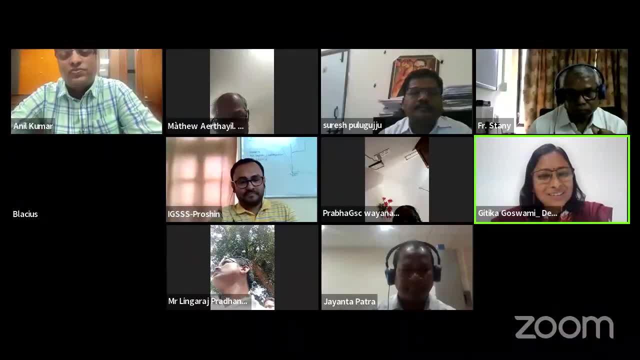 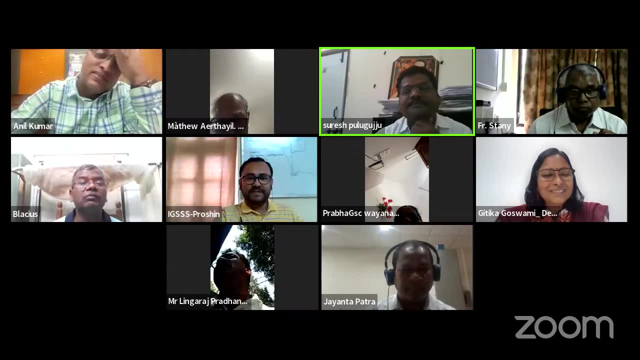 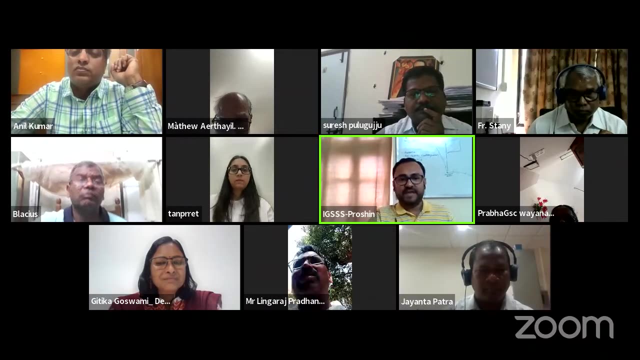 So it's just what my experience in different areas. that's what I am sharing. I have a question Just very quickly with Mitika. I think we can prioritize the national knowledge. I understand that they have a lot of traditional knowledge, so what was? 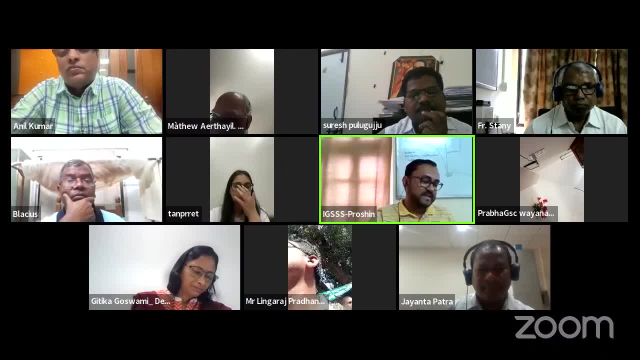 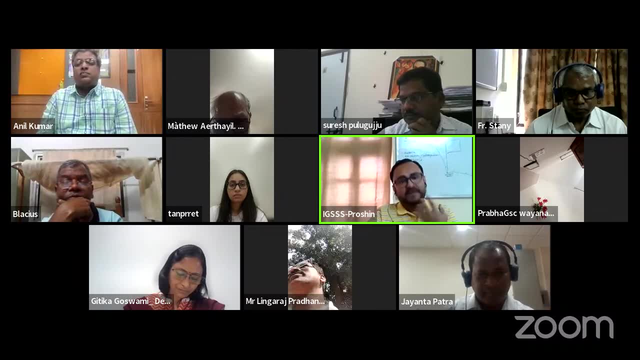 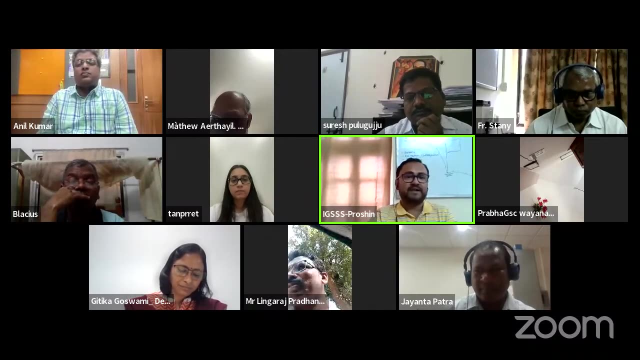 before 50 years, when there was no climate change. So then, this is the thing, And the second is, I think that climate change science, we have to demystify the climate change science to them, The language in which they understand what climate change is. 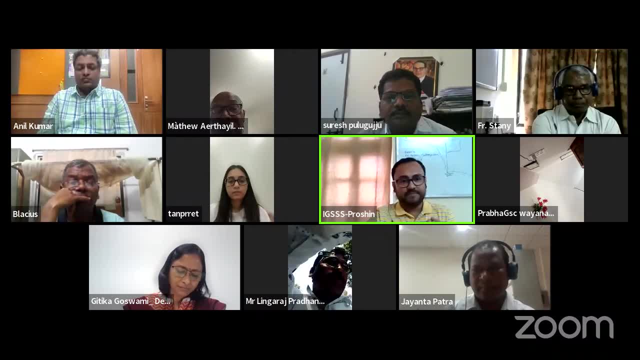 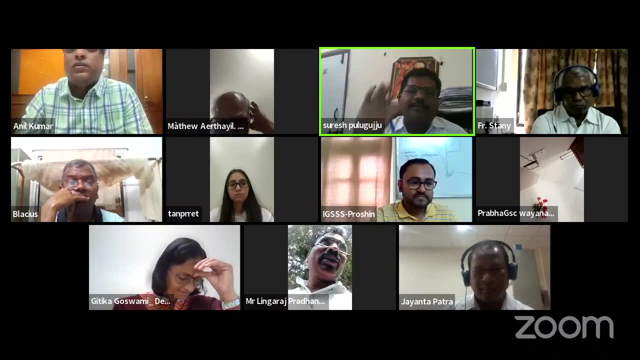 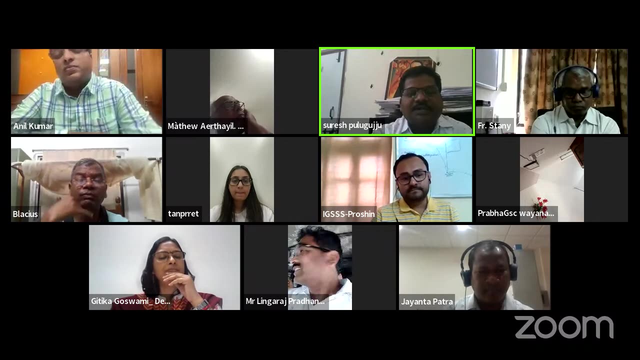 for them. it's hot, it's very cold. this is the thing. Nothing is difficult. everything is simple for us. I have a question. Please introduce yourself, Suresh. I am Suresh from Andhra Pradesh and Telangana states. 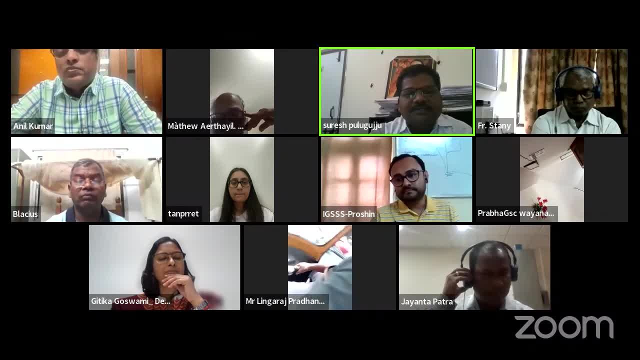 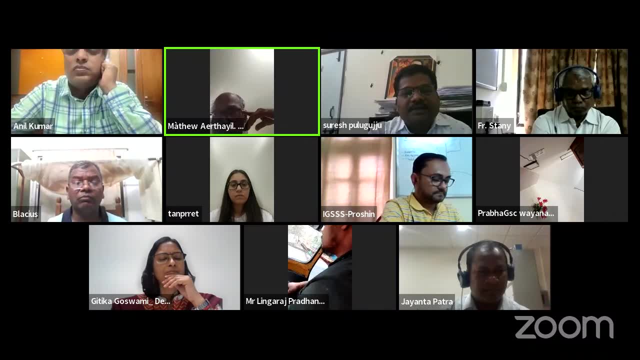 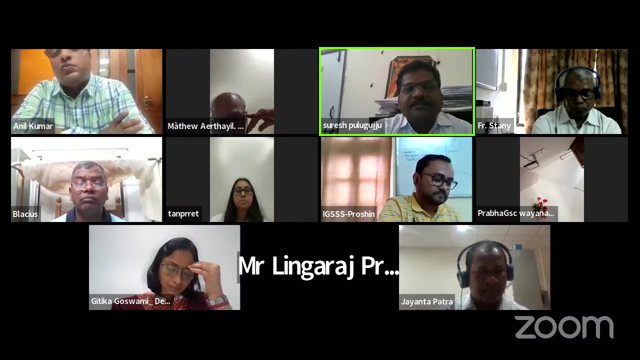 We are working with the Adivasis. They are from Chhattisgarh. They have migrated to Andhra Pradesh and Telangana. They are living in deep reserve forests. Almost 45 villages are there. Government is recognizing them. they are the. 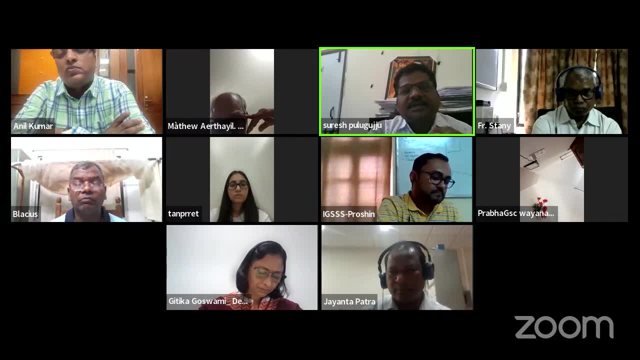 citizens of Andhra Pradesh one thing. Secondly, they don't have any land rights. They are cultivating for the food only, but they don't have any land rights, And government is not allowing them to construct even the toilets They don't have. 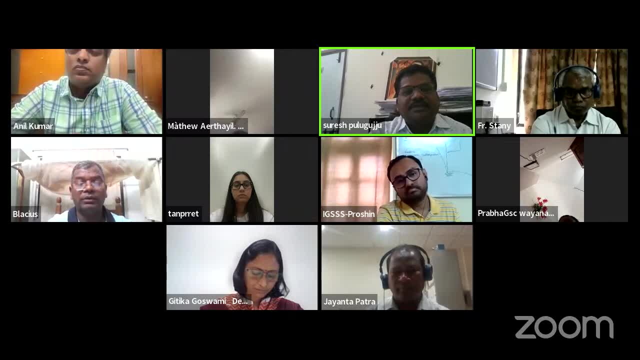 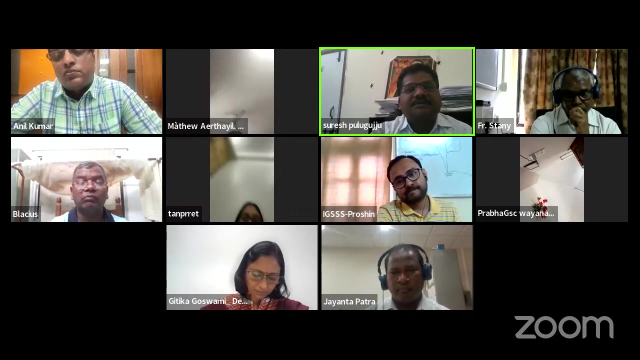 road facilities, transportation, everything In the recent days, government is harassing them to to. This is the situation of thousands of Adivasis in Andhra Pradesh. So how to tackle this issue? Is there any networks? or, with the climate change, how can? 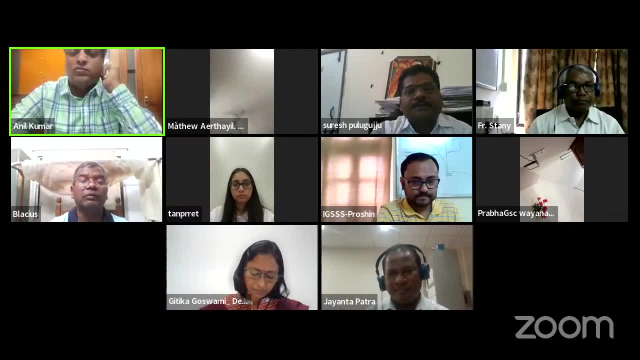 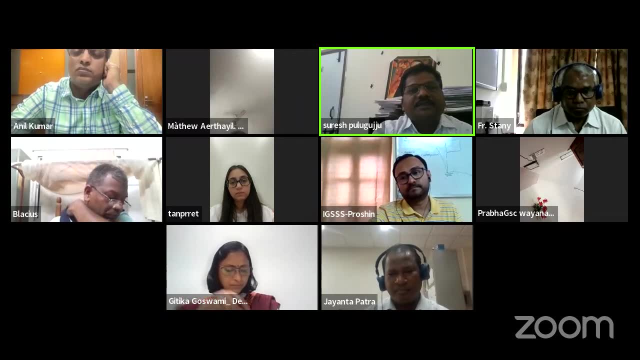 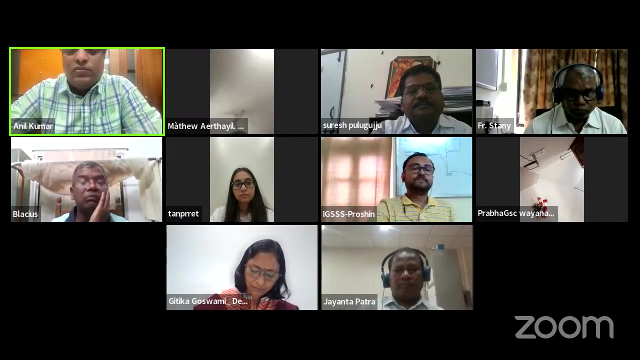 we work with this. Even the government is not issuing the caste certificate for them, So they are not able to go for higher studies, even intermediate. also, That is a very big challenge for the Adivasis, Mr Suryash. 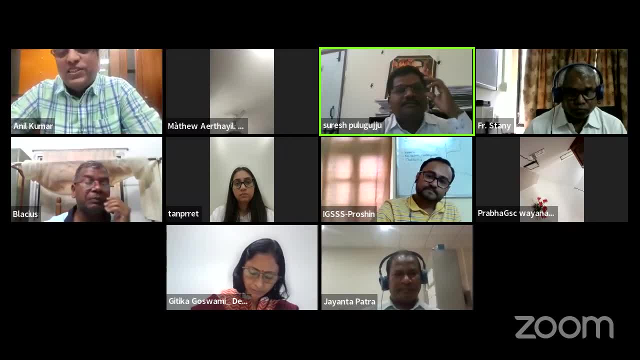 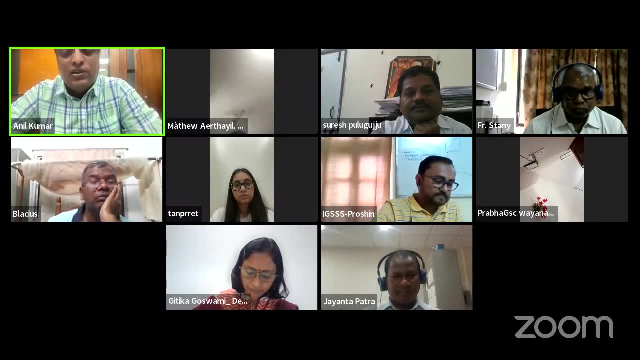 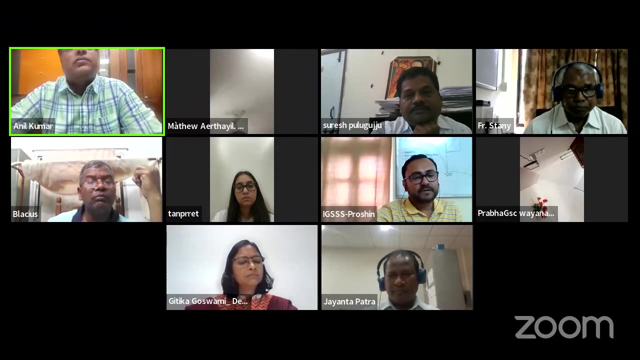 this question is not directly related to climate change. Yeah, This is part of the very much larger campaigns which we are already connected with and engaged in: Githiga and Prashanth. do you want to comment something? Actually, almost the same. 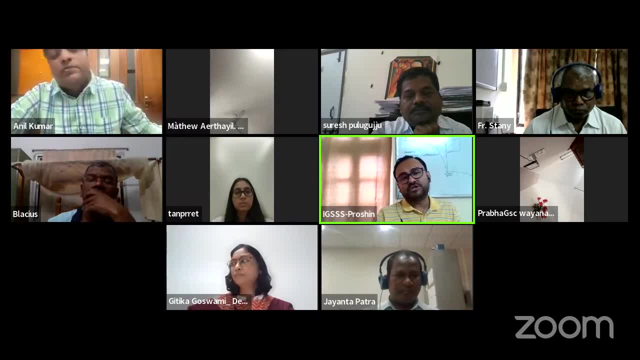 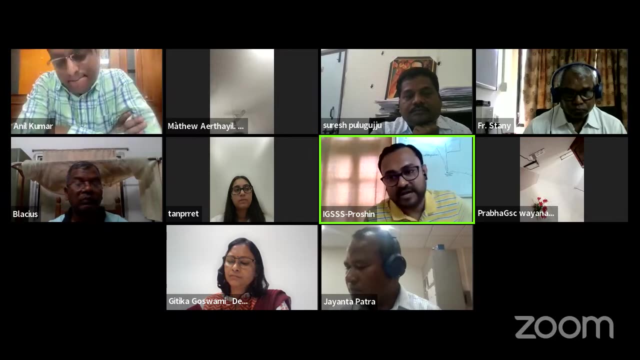 thing is going in slums. If the slum is not authorized slum, then addiction problem is always there And government will not listen. They will never listen or are listening. There is no such case where the government has listened. So basically, 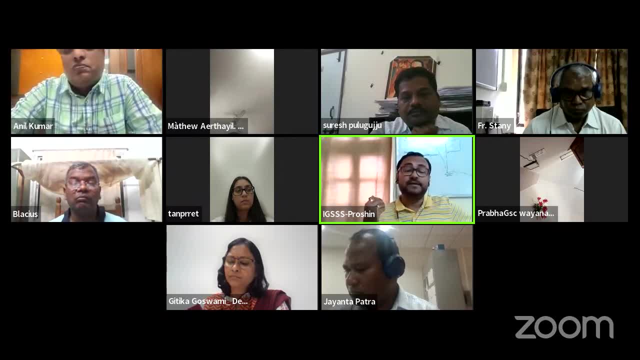 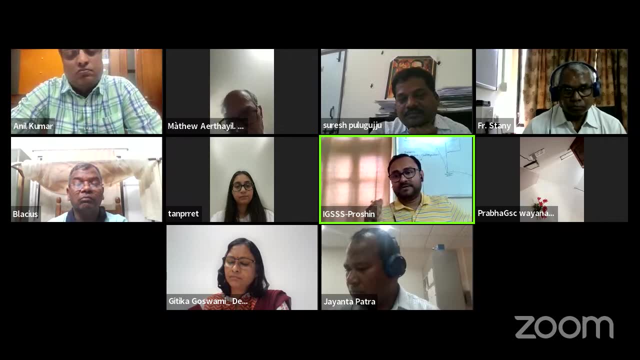 we have to- I am not sure whether it is right to say this in this month or not- We have to make a strong face-to-face effort, Otherwise we have to build a good, strong, network, strong platform in this for a good campaign. 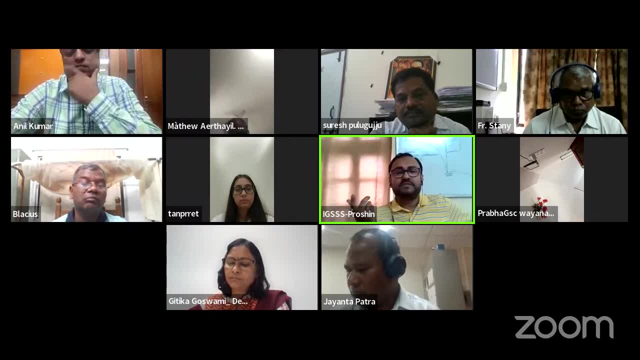 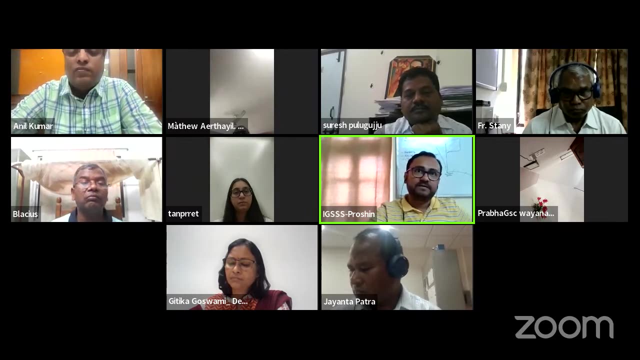 That's the thing. Because there is no such solution, There is no such way that we can go. if we go this way, They will get a land part-time, They will get everything. There is no such solution. So this is the thing from my point of view. 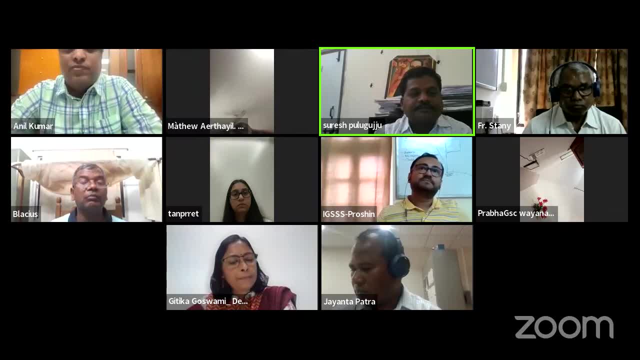 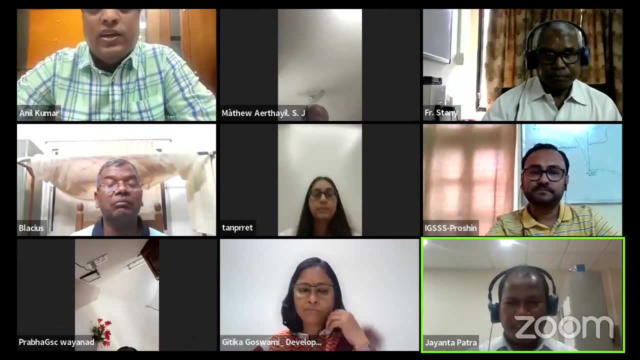 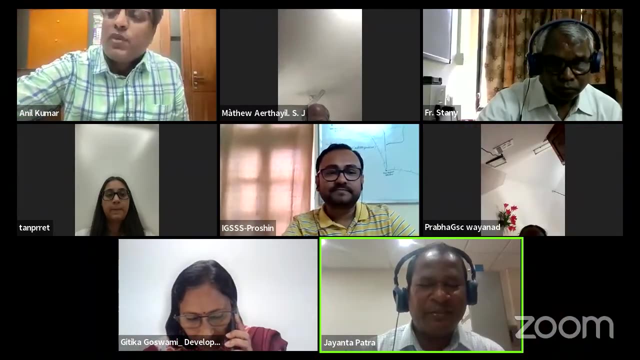 Okay, sir, Thank you, Thanks. I think we can wind up now. Many thanks for the speakers joining us today. Over to Jayantoo. Okay, Thank you so much, Anil. Before proposing for the vote of thanks, I have two, three. 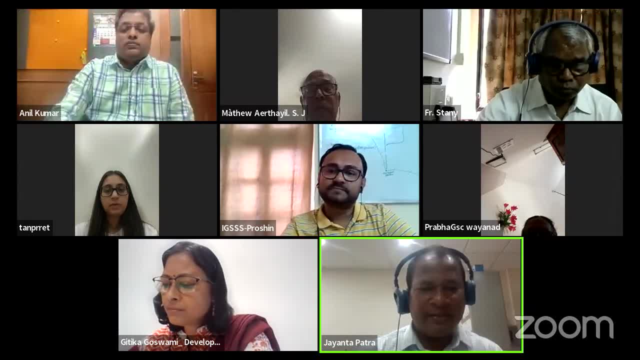 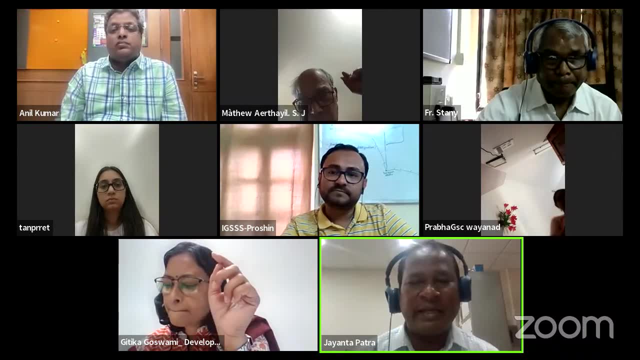 very specific questions which will help us, our partner, to understand this climate change and also, how can we collaborate? and all The first question is: what are the government initiatives, particularly to mitigate this climate change or to adopt climate change in the particularly vulnerable groups? What are the 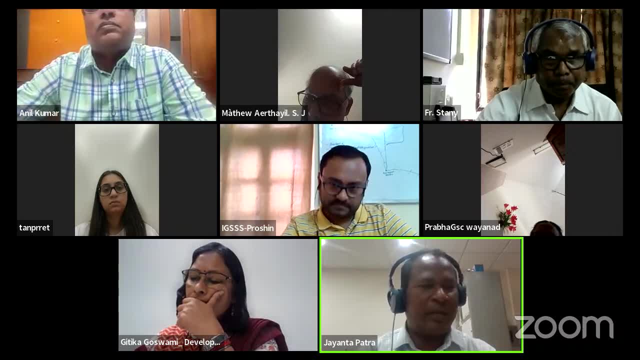 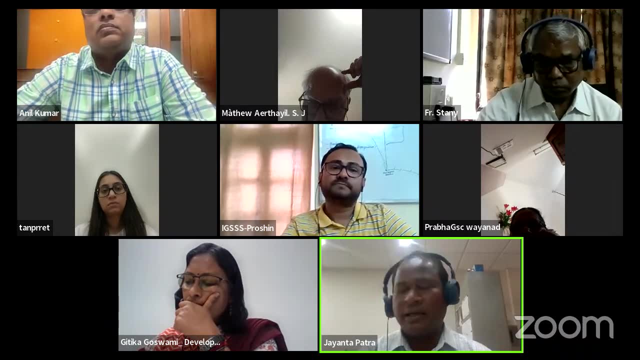 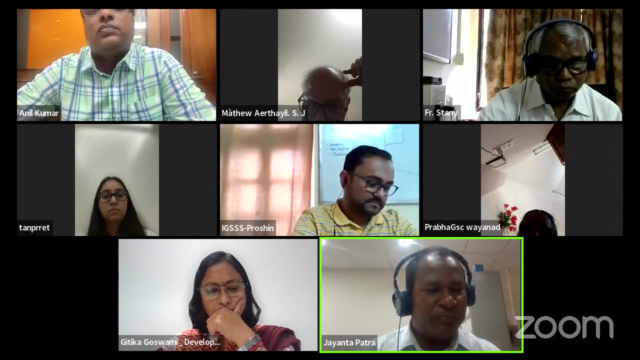 government say, for an example, plantation is one, So what are other schemes and also the policies are there. This is one. The second question is: can you also help us to design some kind of tools, how to go for this like a PRA? 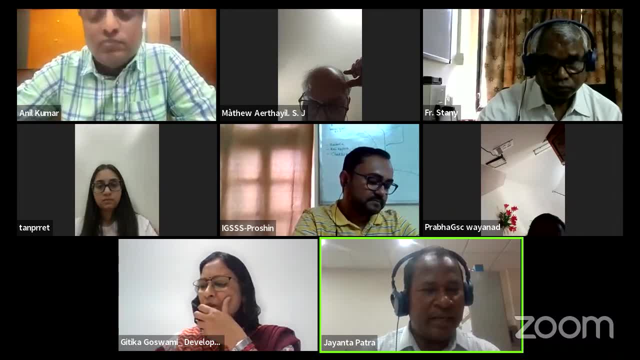 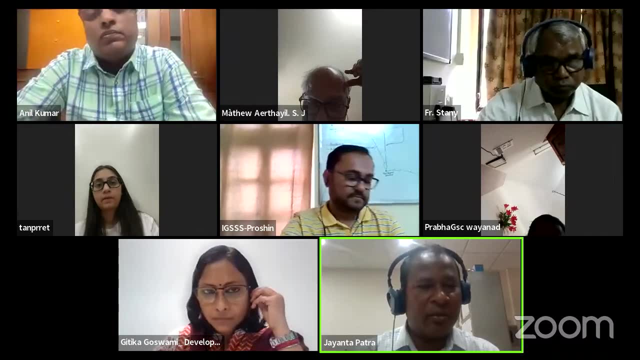 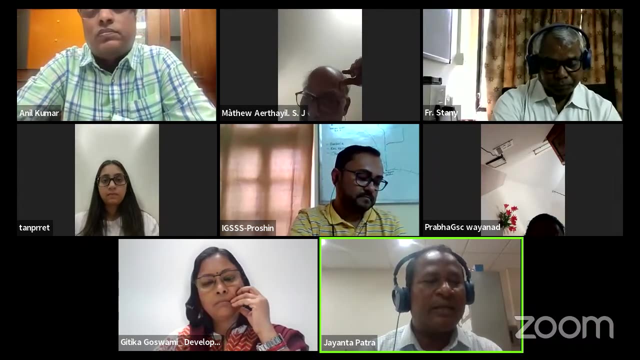 or maybe some kind of mapping tools. So if you can help us in that also, that would be fantastic for us. Then third question is, also like government, do you have any partner or who are the stakeholders that you are working so that our state partners can? 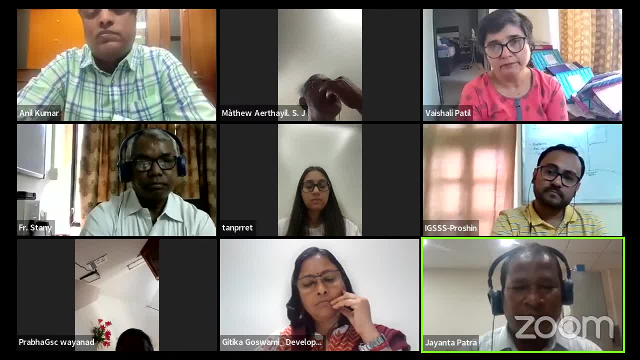 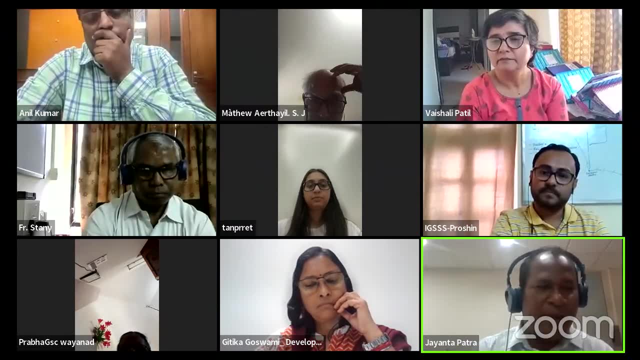 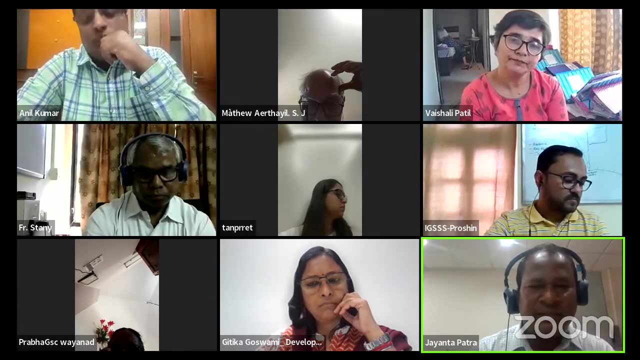 collaborate with them or can learn each other? as Githika said, peer learning is the- I mean the raw experience. the best teacher of peer learning is very much required. So these are some of the three questions. If you can just respond, that would be great. 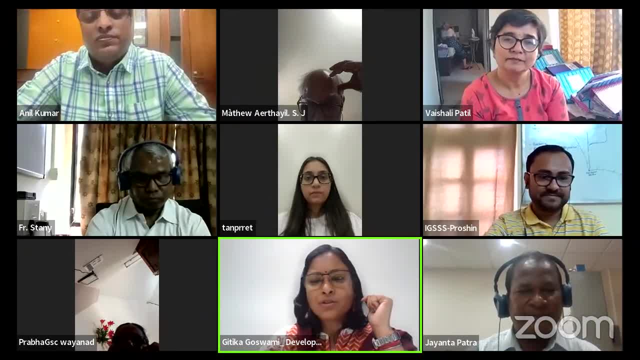 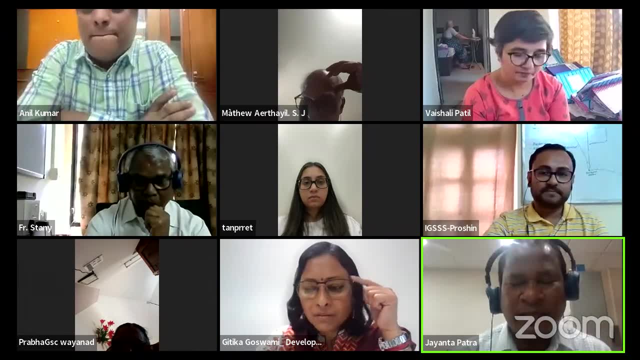 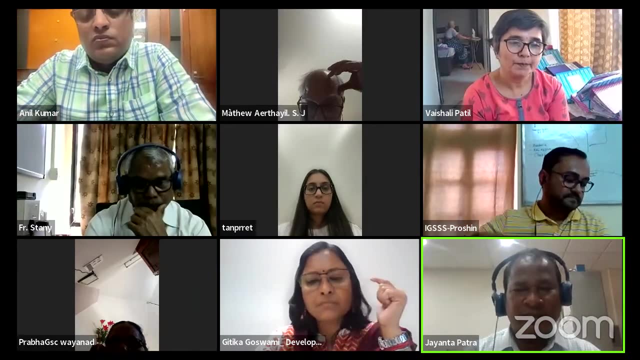 Githika ji, aap sundi ji. Sorry, I got a call and I just missed the questions. Okay, So first question is: what are the government initiatives to adopt or mitigate this kind of climate vulnerability in the rural area? This is the first question. 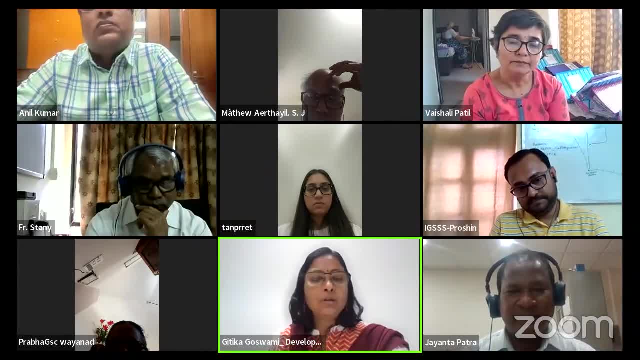 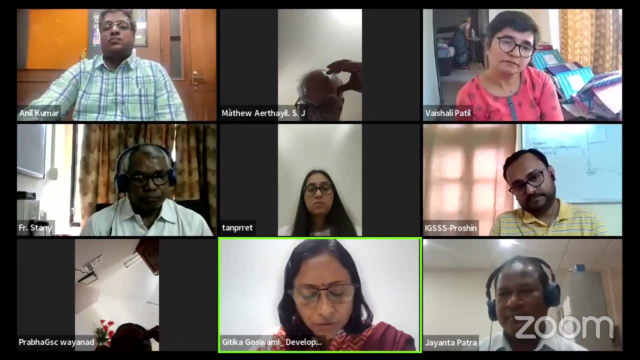 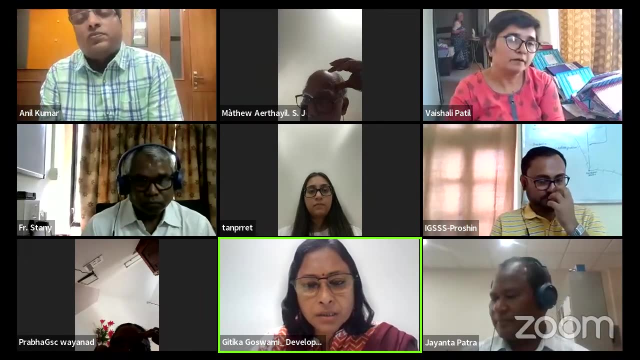 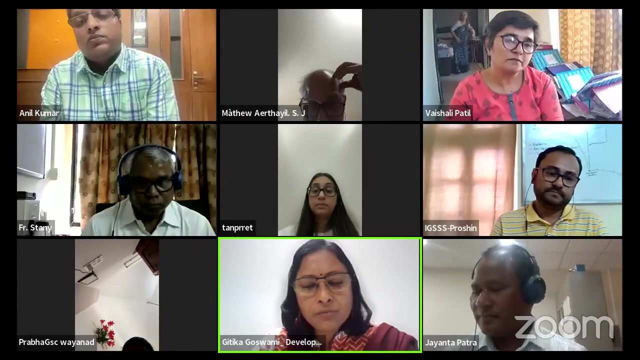 Okay, So I think there are also in the different responding to different questions I mentioned. there are several initiatives that government has. I mean schemes at least government has come up with. but I think that not only announcing a scheme will solve any problem. 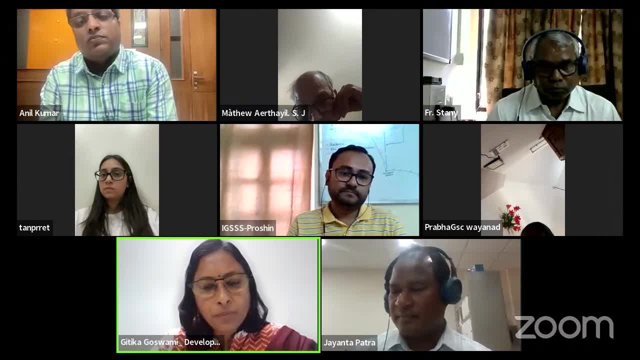 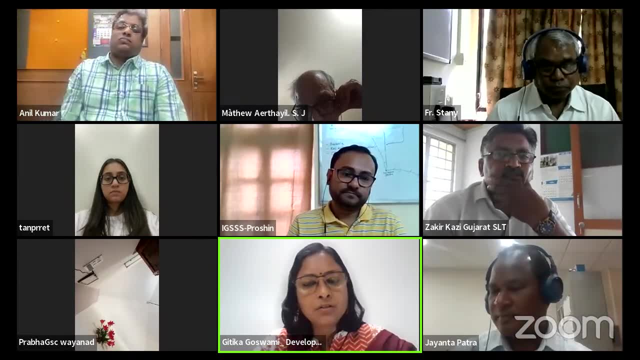 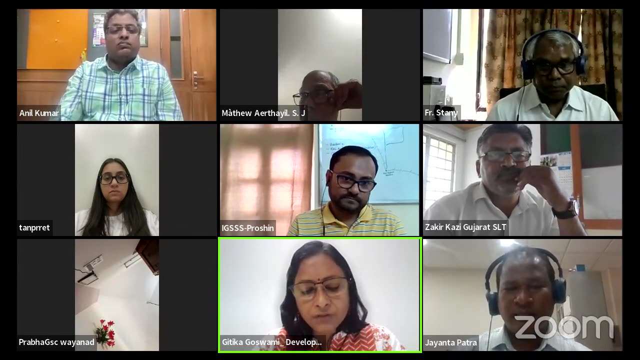 So one thing is the schemes has to be implemented in a proper manner, and many cases it happens the schemes are only being implemented through the panchayats, and if the panchayats are not really adept enough to implement those schemes, it's really difficult. 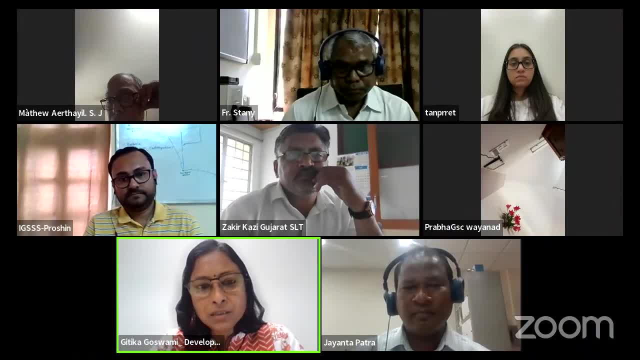 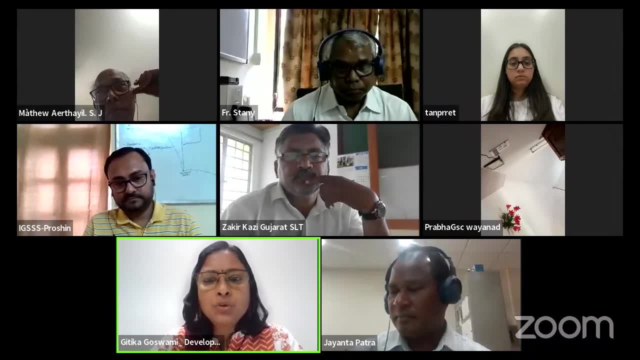 So the role that we have, the CSOs have, is to work with the panchayat and the local government very closely to see that all those schemes really being implemented on ground. they should be reaching to the beneficiaries, I mean, who are 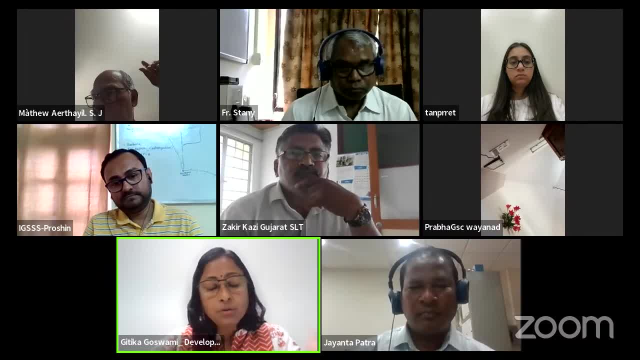 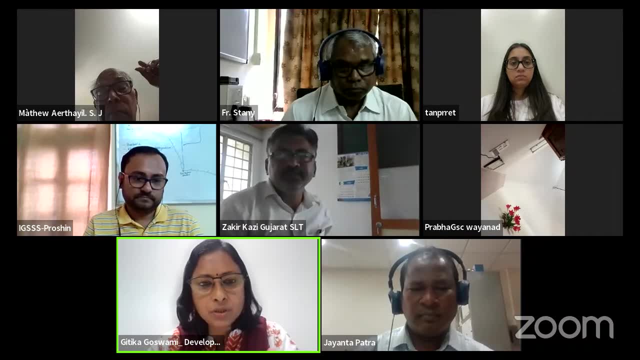 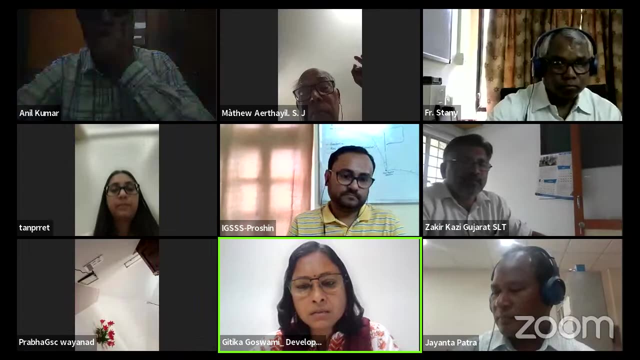 the vulnerable communities. So, as I mentioned, I don't know what the name of the all initiatives, but these are very important at this Milet initiative which has come up, which is very, very important with the current scenario of water scarcity problem and 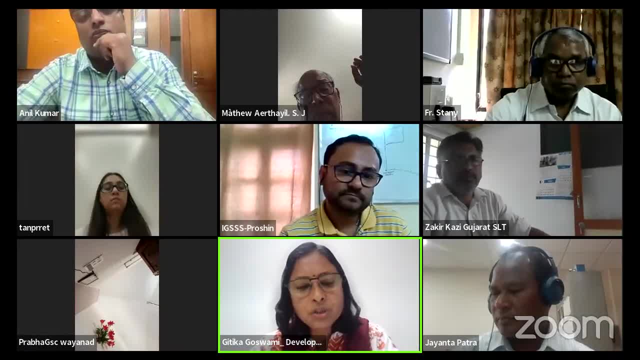 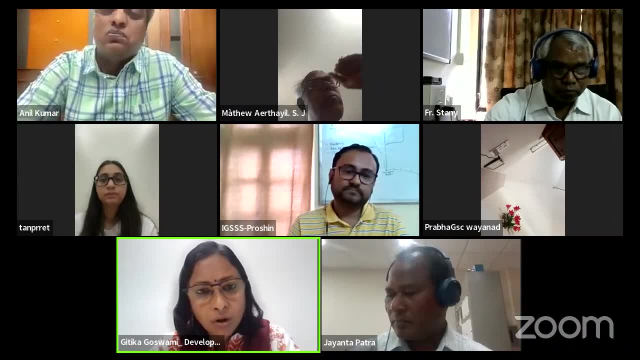 the reduction of the rainfall and all. I think that Milet Mission, Kushum, that's the solar irrigation system which is now being implemented. I think South India a lot, they have already started. Then JB Kheti, that's the organization. 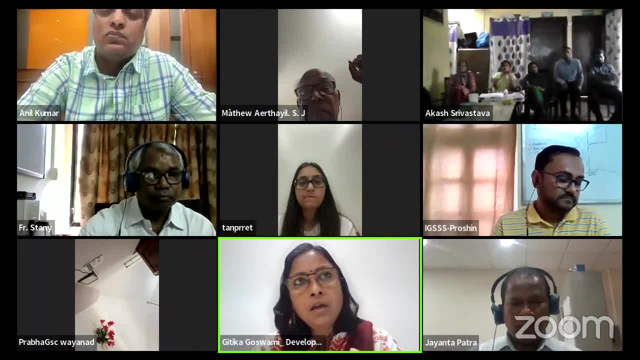 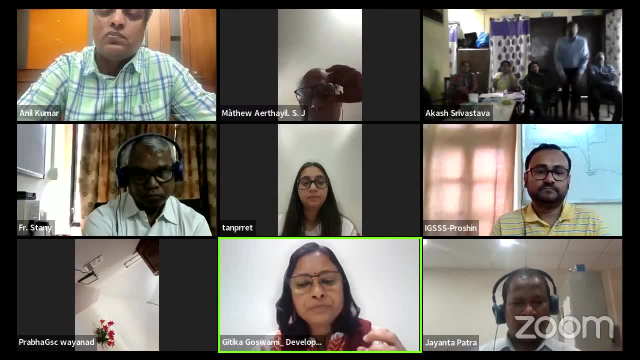 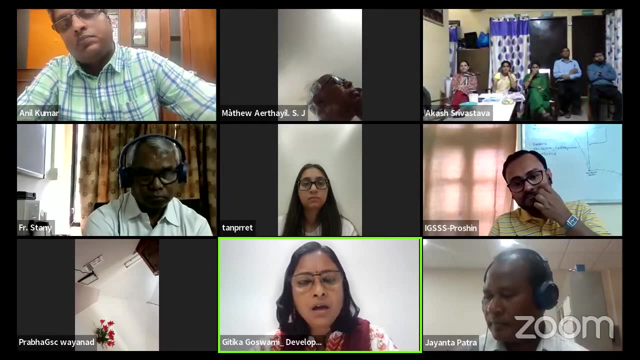 which is running fertilizer and which are really very, very good scheme from the point of view of climate change adaptation, as well as development, and there are lots of skill development and green skill development that's being happening and those are. that green skill development scheme is basically across the sector. 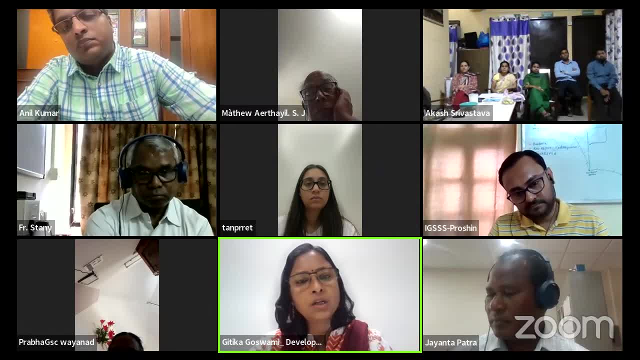 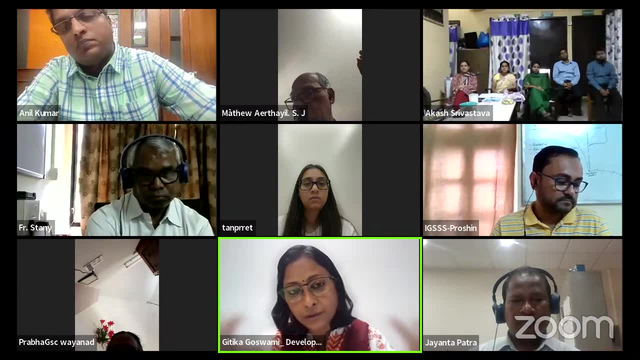 you know, and across the society. So it's from Farmer, it's for the farmers, local government, district officials, So there are several, there are under green skill, there are these kind of trainings been happening and also there are trainings happening. 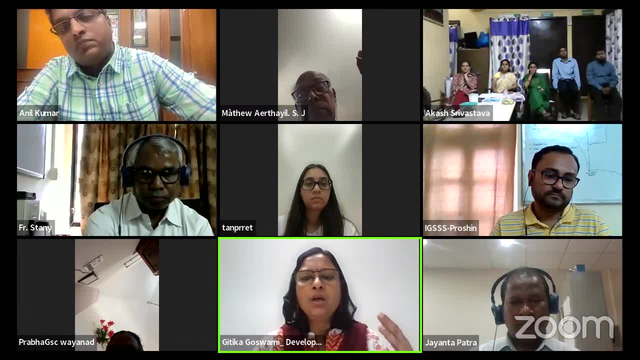 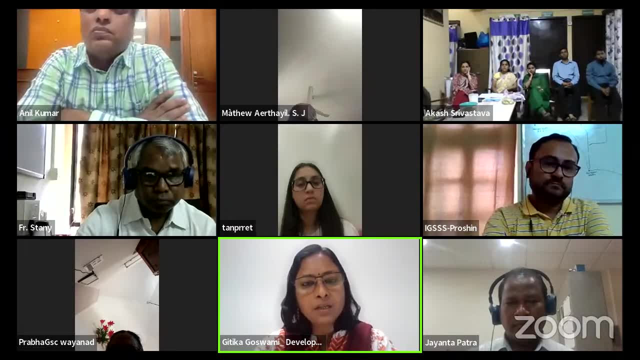 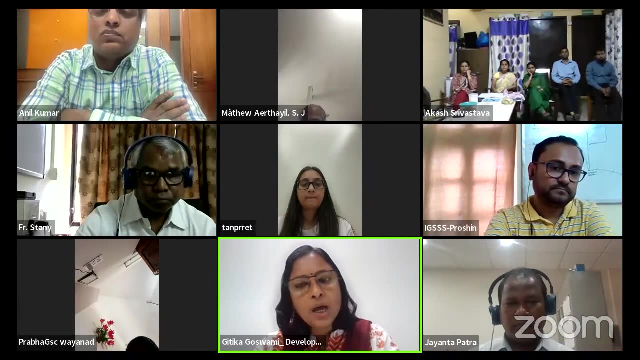 not only from the government end, but also from the NGOs, academic institutions, agriculture, universities- those are also like lot of capacity building training is happening. So I think the main thing is now to disseminate as much as knowledge to among the communities you know across the society. 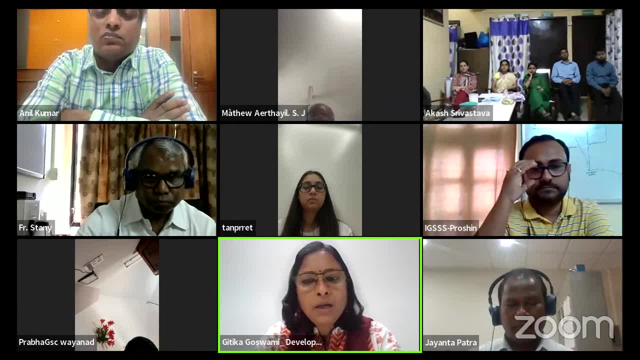 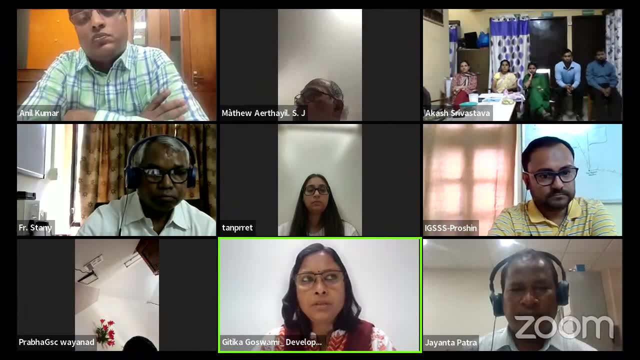 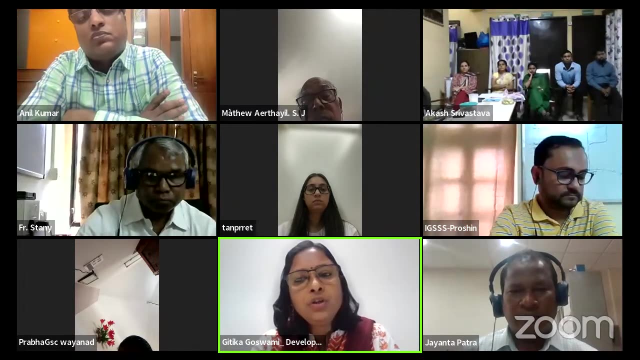 sector which I think is the need of the hour. One is that, once the knowledge being disseminated properly and if we are knowledgeable, I think half of our problem can be solved that way, If we know where to go, how to do. 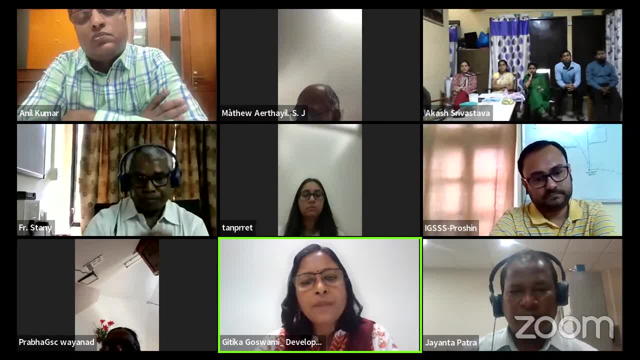 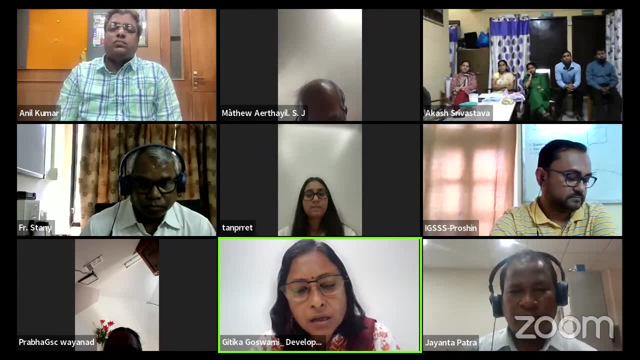 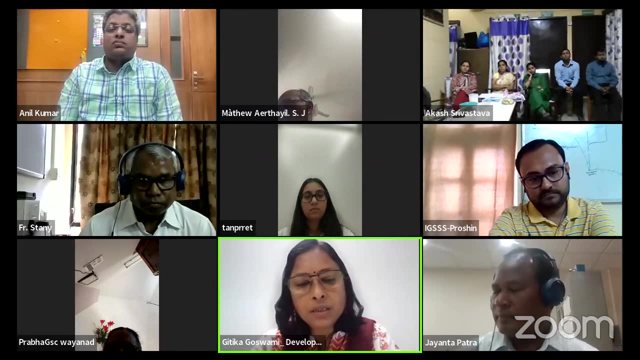 where I get support, where I get training program- which are the new, you know schemes that has come- where I can get this organic thing. you know, kaad is one thing. you know the JB we call JB kheti, but 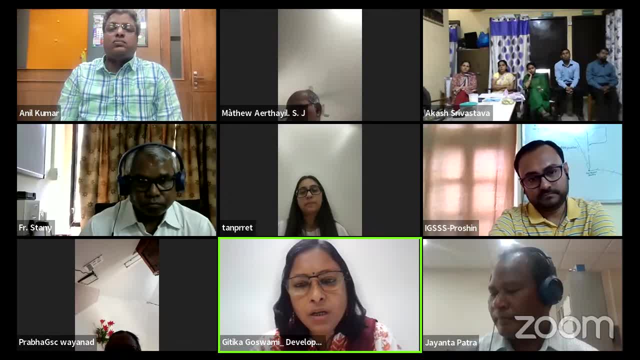 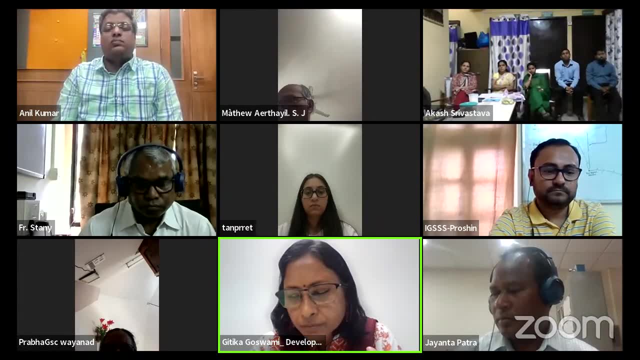 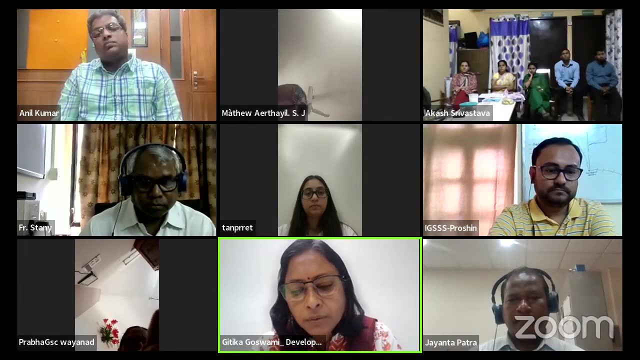 this mean in traditionally, we are using the kauda, we are using the entire, you know the waste, the household waste, the kitchen waste, into the, into composting or the that. I think those are some of this thing we have to really. 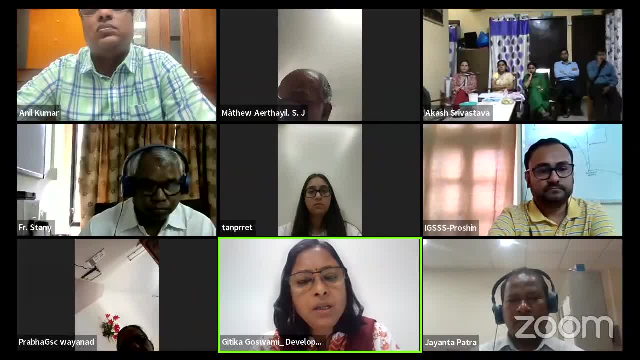 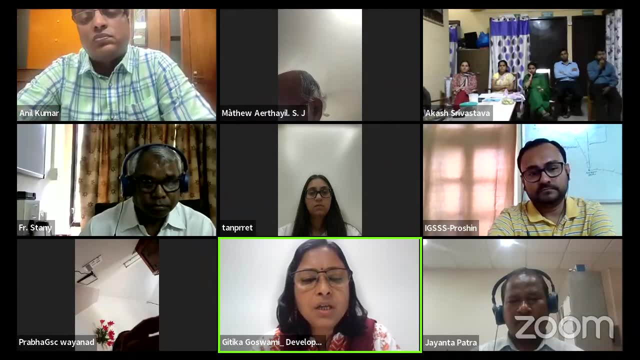 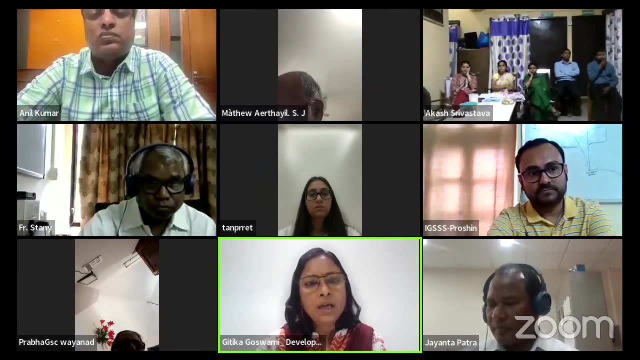 focus on now. There are ample things available just to touch them, just to take them into this. And the first and foremost, I would say, initiative is required from any communities If I think that Sarkar will do everything, but even if Sarkar is doing, if I don't, 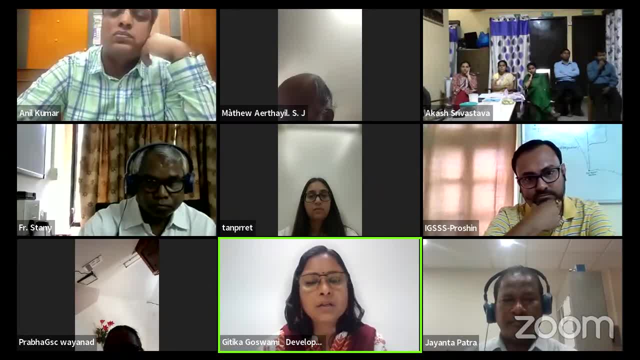 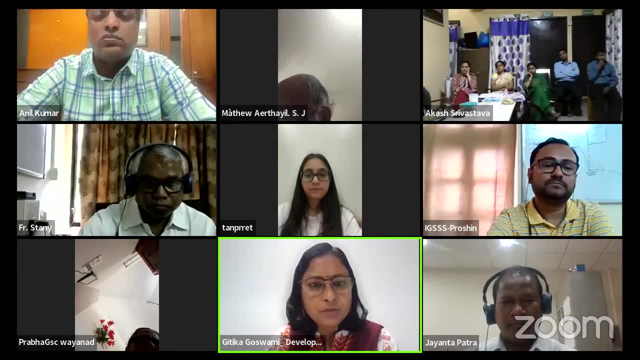 go and know what is Sarkar is giving. I won't be able to cope up with, you know, and that is why I mean the direct benefit transfer. I mean, I don't know. it is not connecting to the today's discussion, but where we 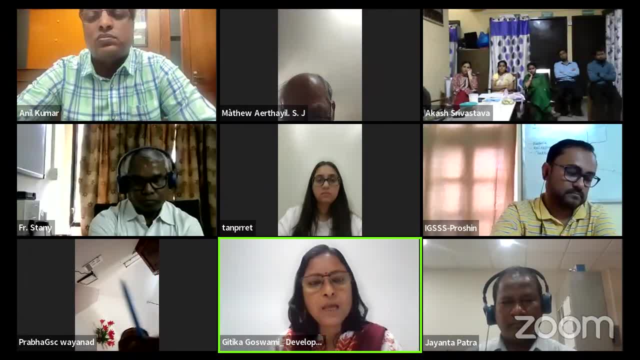 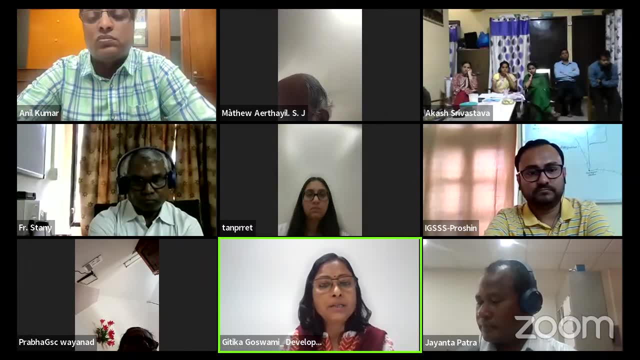 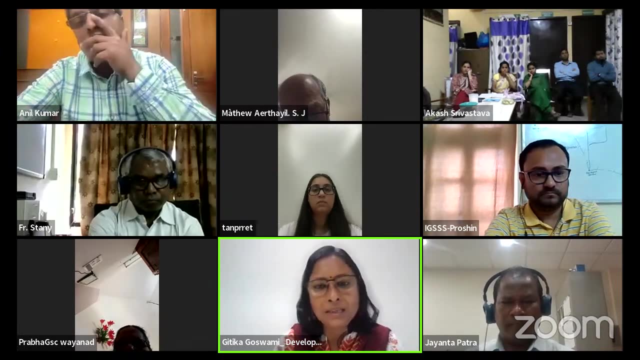 are seeing. the direct benefit transfer is absolutely the great scheme that the beneficiary is getting the money at their bank account. Now the point is, you know, if we get some money without doing anything, you know we became really lazy- If we are really 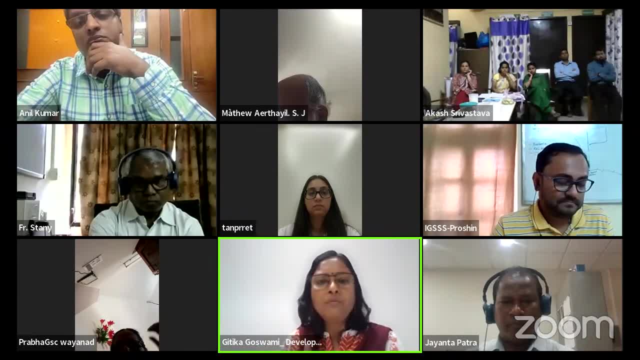 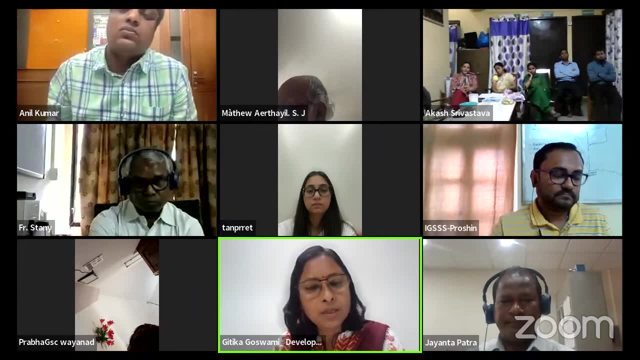 very. you know. use that money to do the work which is the intent of the government, then it will be, you know, very much successful. But we really don't know what the money is being used. you know If it is for 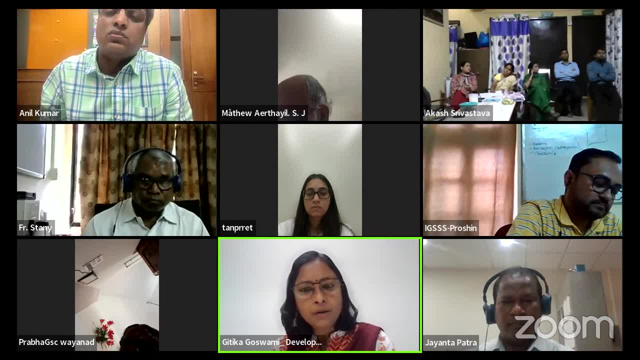 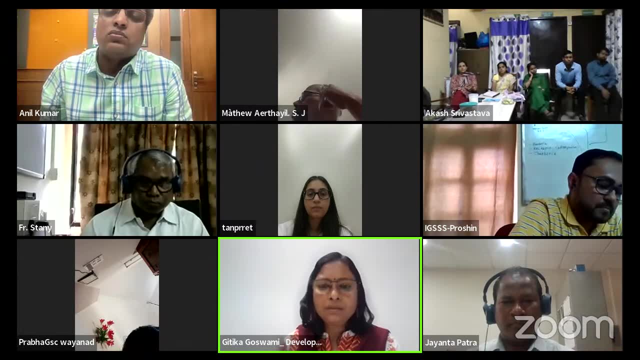 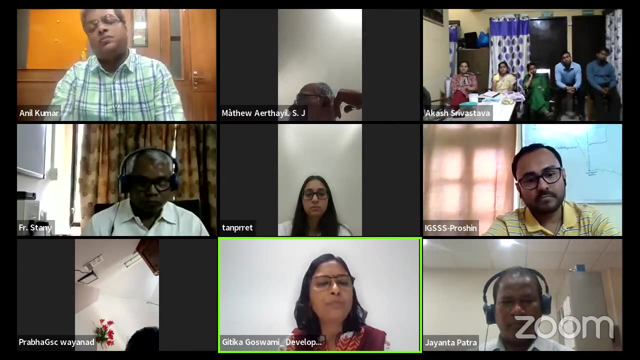 purchasing seed or purchasing fertilizer or doing some solar irrigation system, then absolutely it's the best thing, But that has to be implemented And that is why monitoring and evaluation is one of the components that is very much required, And I think that monitoring and evaluation 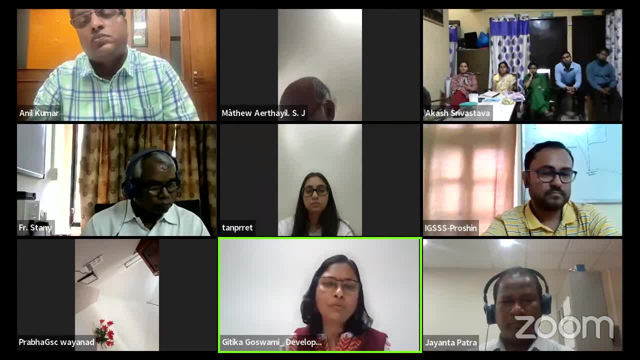 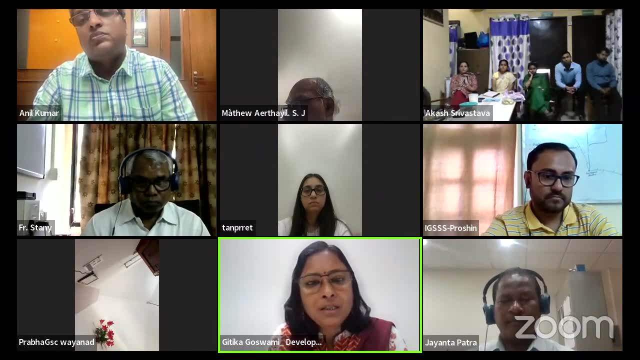 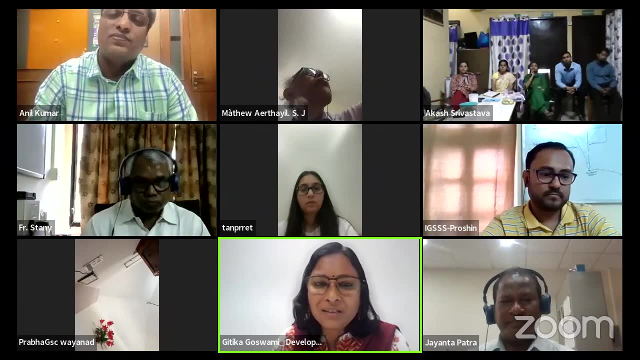 should be done or can be done from the bottom end itself. You know, if the peer is really aware of then, people cannot sit idle and say that government did this. that's why I am so much poor. That's my feeling, But it's completely my opinion. 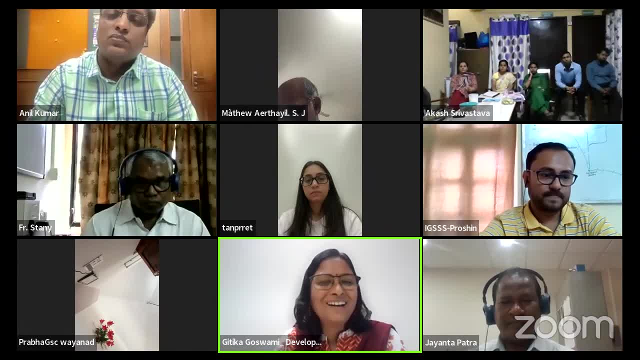 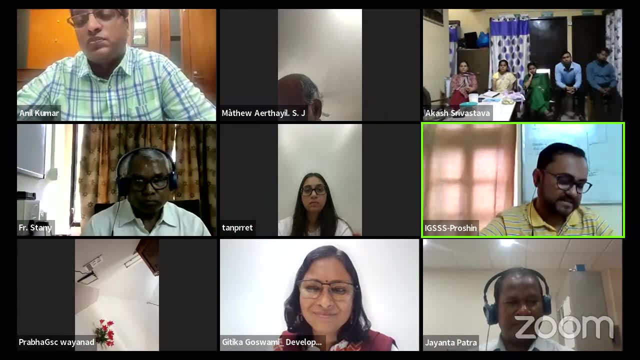 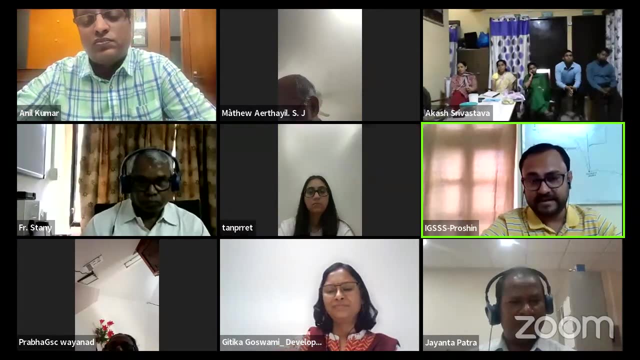 There must be, you know, a broader opinion as well. Yeah, thank you. Yeah, adding to Geetika ji. basically, I want to add three more things which are very important. Firstly, whether advisory there is a line. phone line is there. 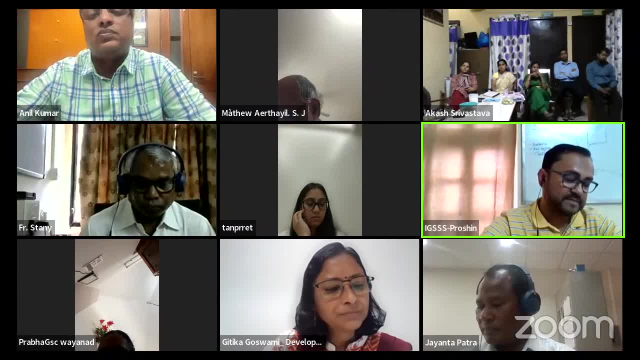 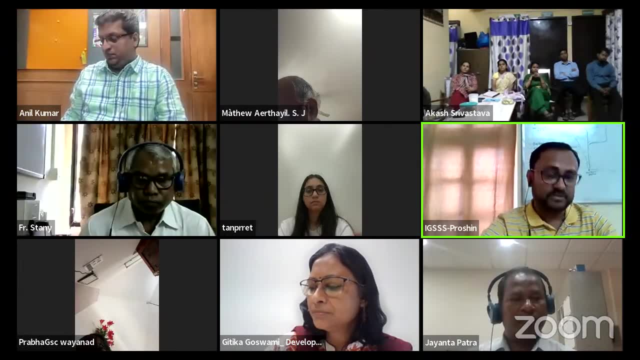 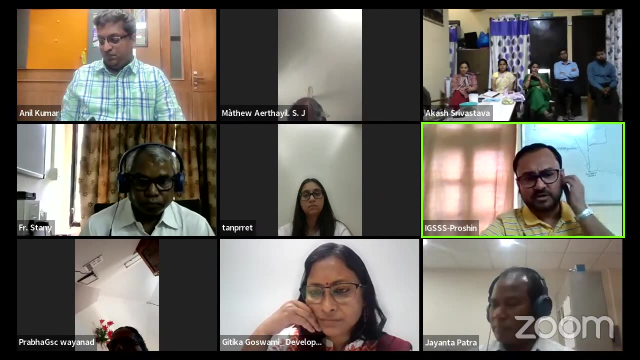 So helpline is there, So the community, that farmers must be in touch with this contact and this because it's very important that it's a very innovative thing. Secondly, already Geetika ji has said that a lot of emissions have been used by the government. 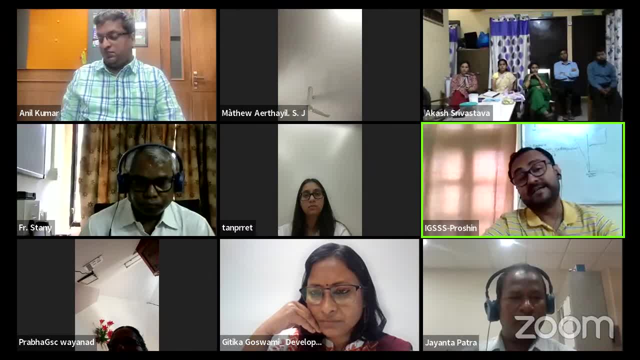 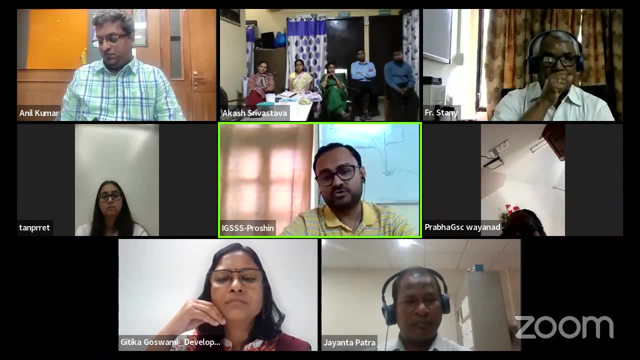 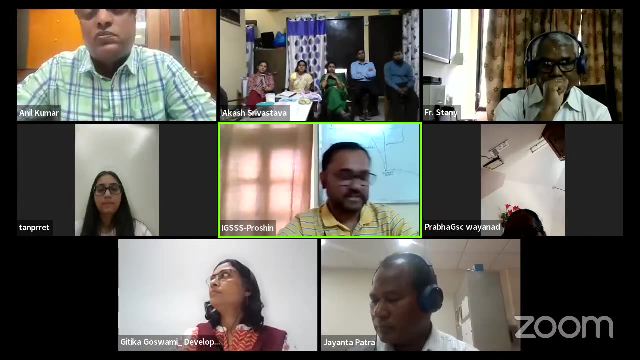 And thirdly, I think it's very, very important- is that crop insurance, Because a lot of societal cases, lot of things are going on. So crop insurance is something which we can minimize the impact. So crop insurance is very, very important. 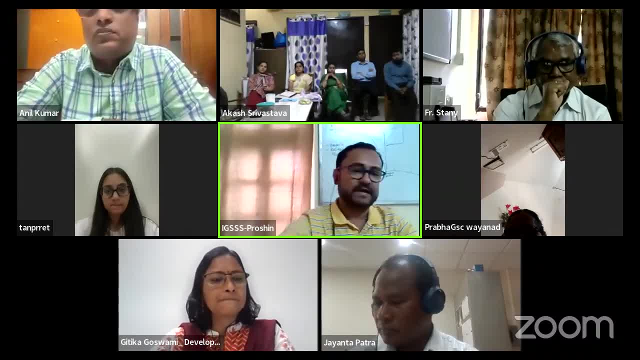 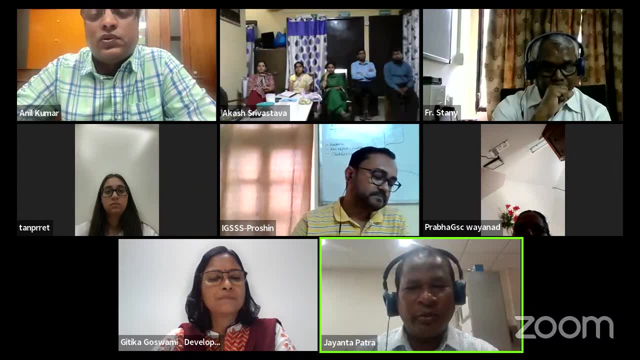 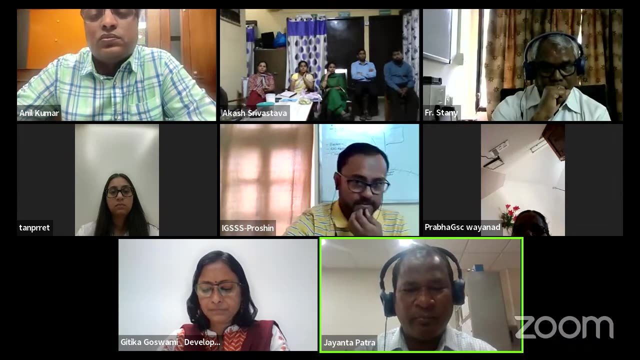 So this is very couple of things from my head, Thank you, Thank you. The second question was: do you have any network or do you have any stakeholders you are working with so that our Lokman's team can collaborate in your intervention area? 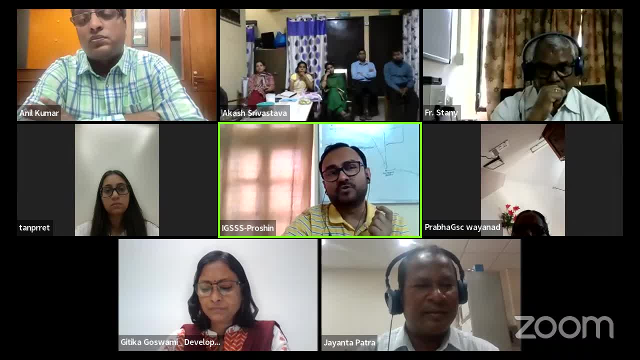 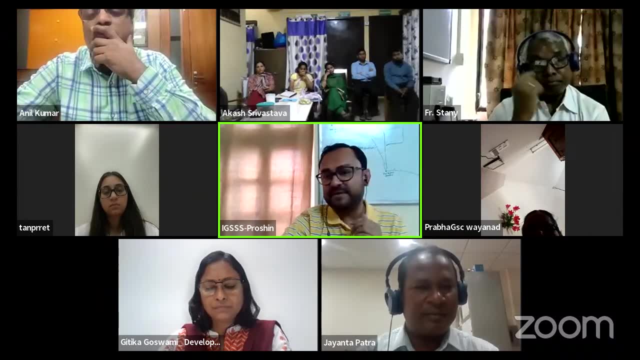 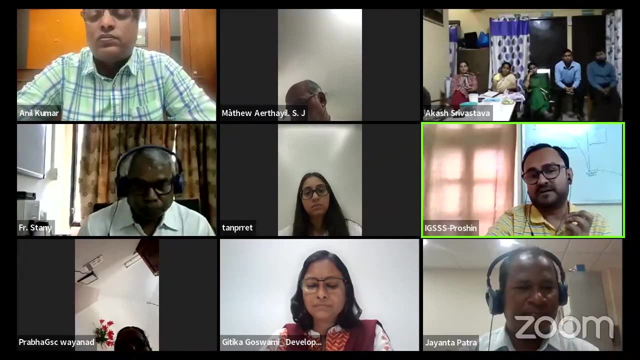 Jayanta ji. RGACC is working almost 15 states. So recently, due to the re-eventment of HCRA, I just implemented everything. There is no such partner of HCRA right now, So in the 15 states we are. 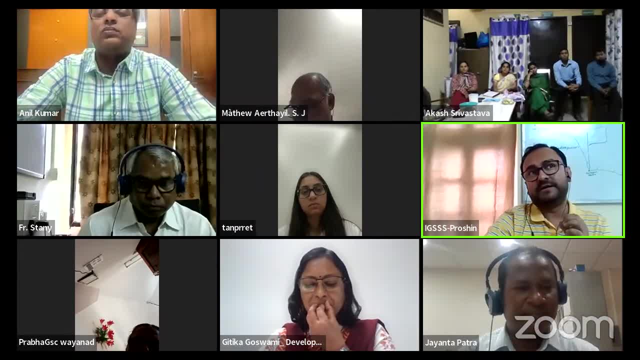 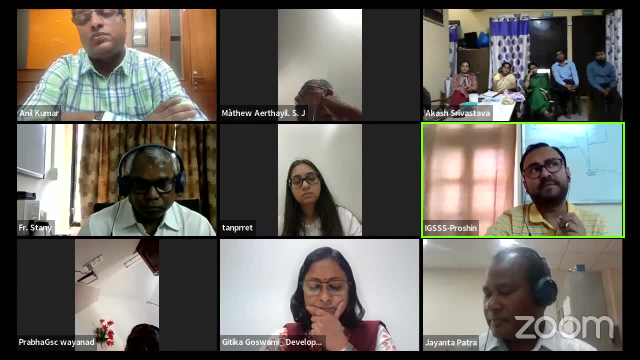 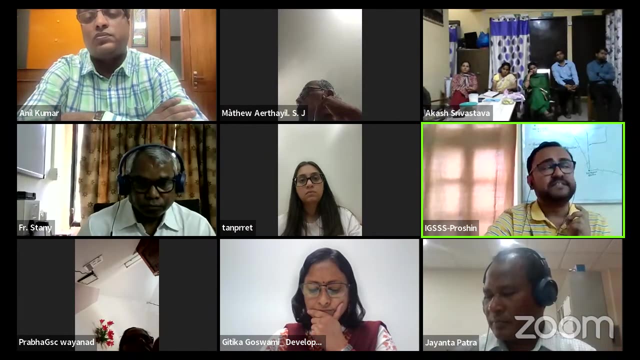 very actively visible And we in 6 states we have already done climate consortium. So there are lot of CSOs. maybe 20-25 active CSOs are in the same platform of this climate consortium. There is a Jharkham, there is Orissa. 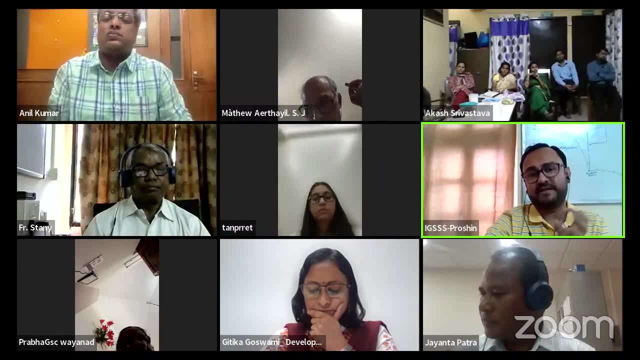 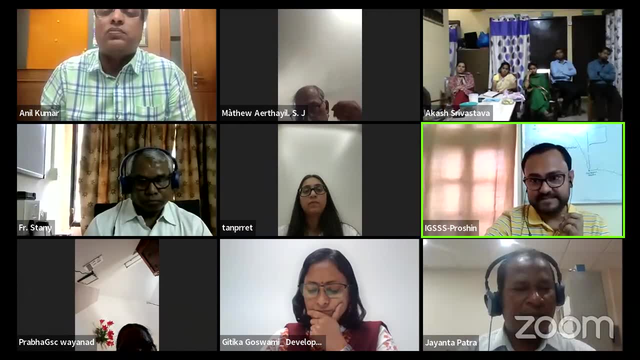 there is NP, there is UP, So these are the states where very active climate consortium is just constructed in last year. So we have lot of plans to do in this year in the upcoming days. So, of course, our partners, everyone. 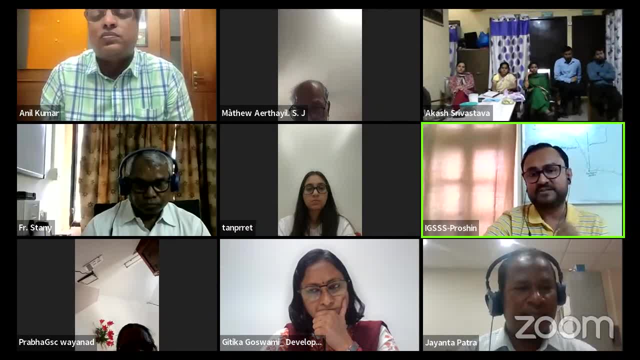 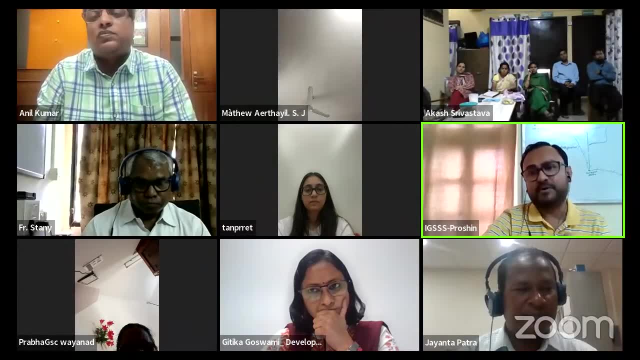 who are presenting climate change, what we want in this climate change thing, So we can come in this platform and everything we can share. There is a cross-sharing possibilities. There is advocacy possibilities, networking possibilities, some learning, cross-learning possibilities. So these are the things. 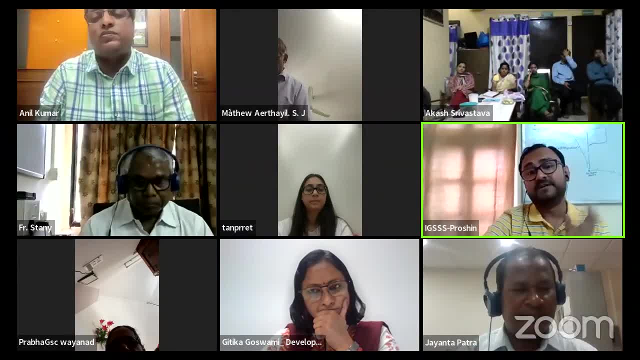 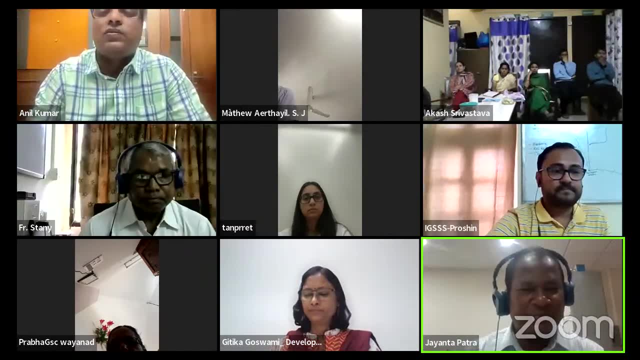 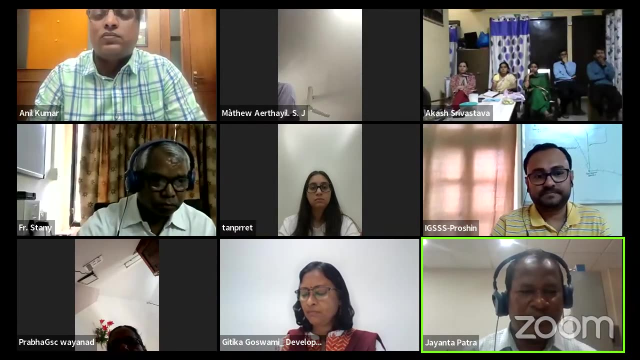 I think we can explore these things together So it will be a better result and better impact in the next year Over. Thank you so much. Thank you so much. So, before we move on to propose the vote, of thanks, Father Stani, do you have? 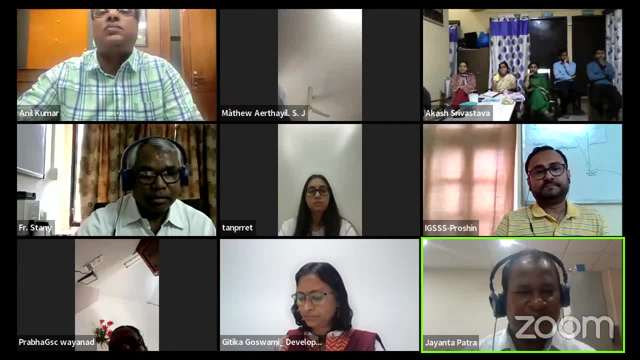 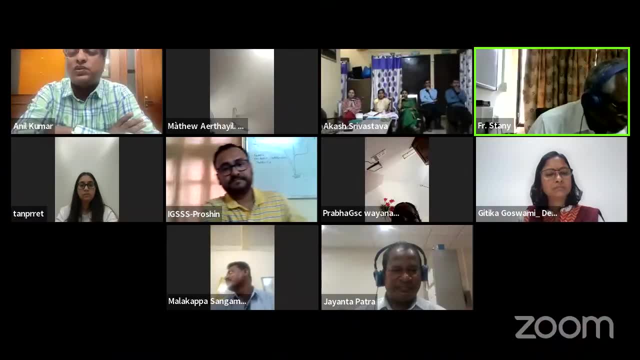 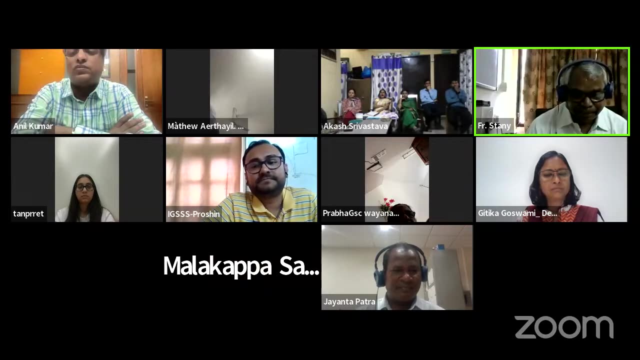 the last comment or anything. Well, I must thank our resource persons, Geetika, Prashin and Anjali, for being with us, for enlightening us to understand deeper, both from different perspective- technically also- and the practical. 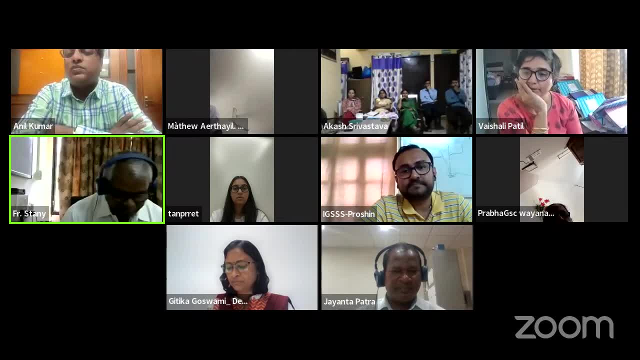 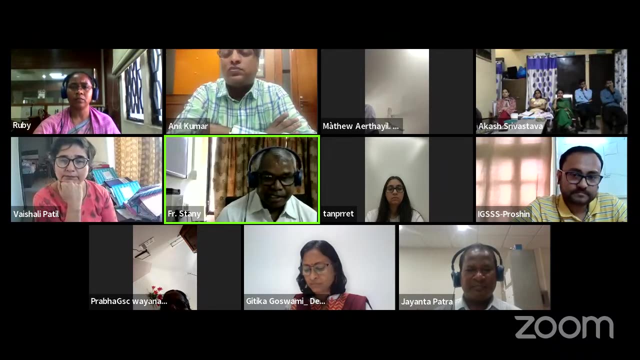 approach to some cases that you presented. I think we are grateful to you. I am also thankful to Anil for moderating One thing which is coming. climate change has also socio-cultural and political implications, For example, identity, existence of indigenous and tribal. 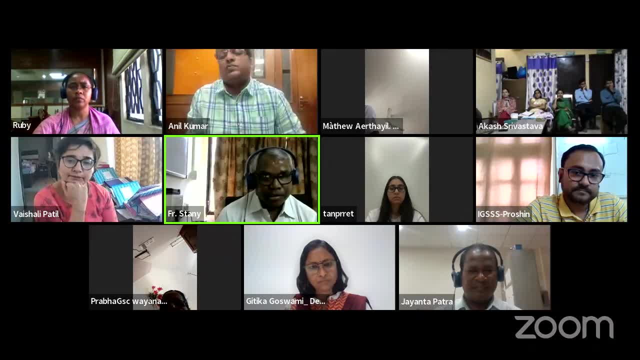 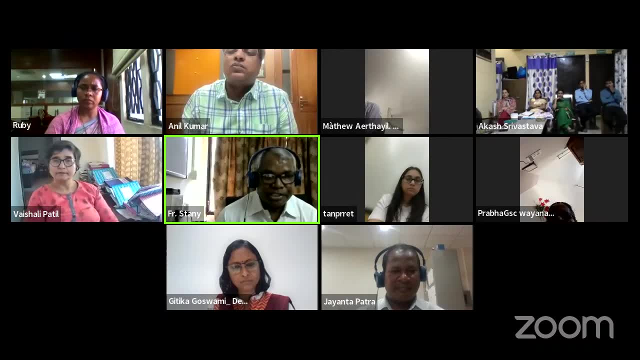 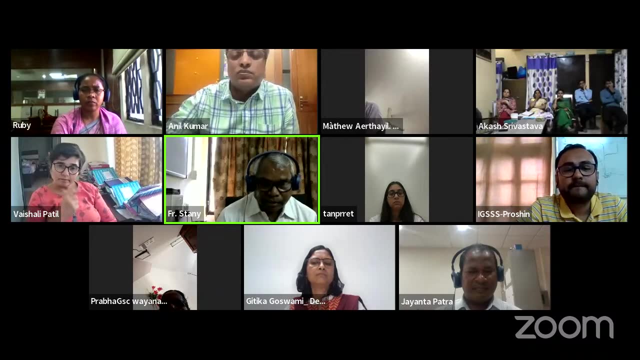 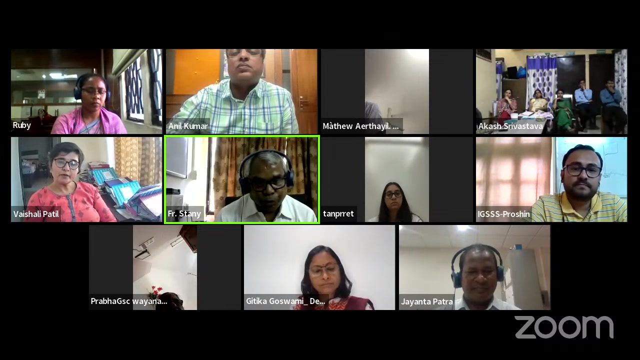 people, cultural aspect is being affected. So from that perspective, I feel the indigenous knowledge and wisdom research could be taken, because indigenous knowledge and wisdom has sustained nature, The alternative model of sustaining soil conservation, nature conservation. all this research could also help us. 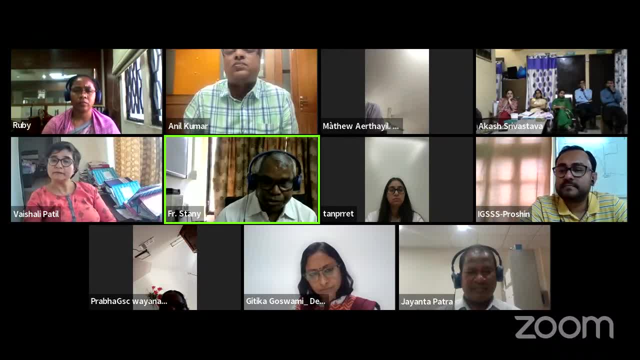 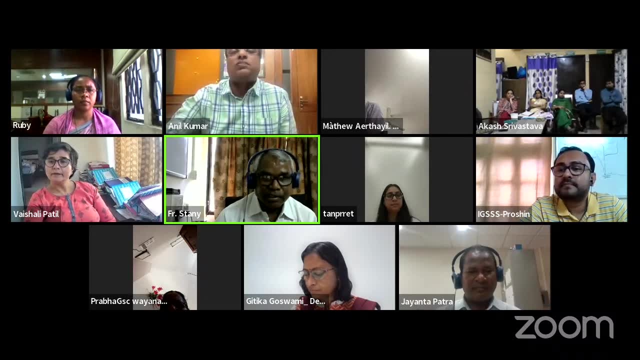 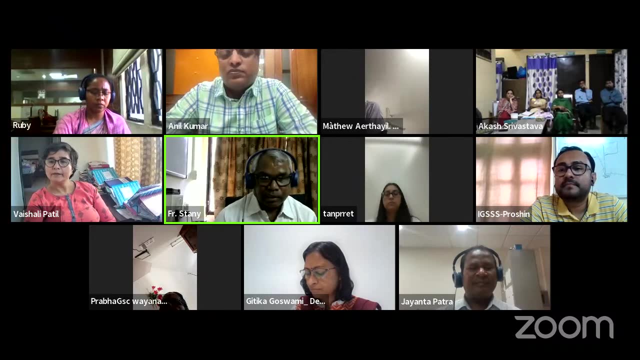 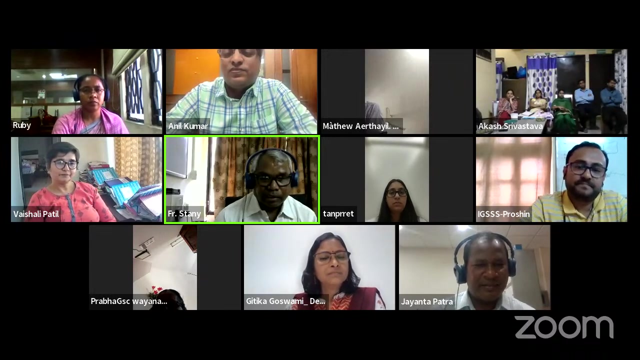 in terms of empowering and also better knowledge sharing of indigenous people from their own wisdom and knowledge. That area is also, I feel, need of the hour. So that's my observation. Thank you, Geetika, Prashin and Anjali for being with us. 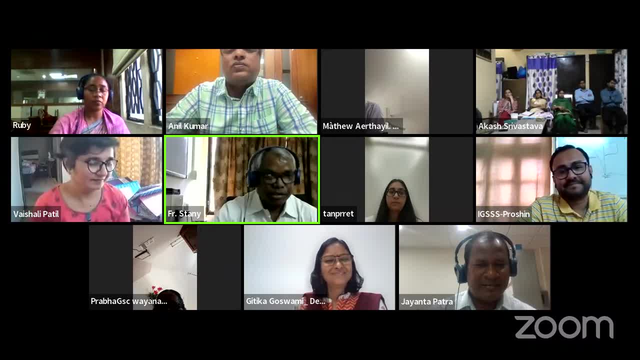 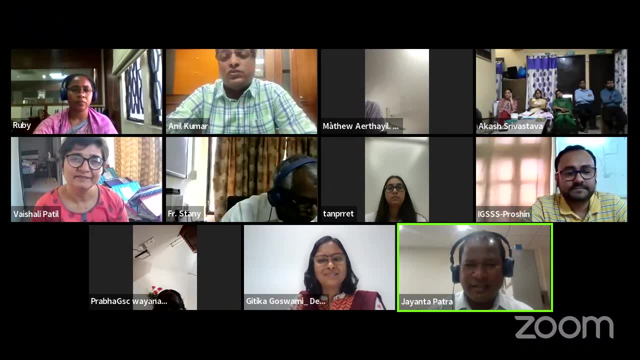 The session is already quite late, So that was my comment. So, thank you, Thank you very much for being with us. Thank you, Thank you so much, Father. Now I would like to request Tanpreet, our colleague, networking. 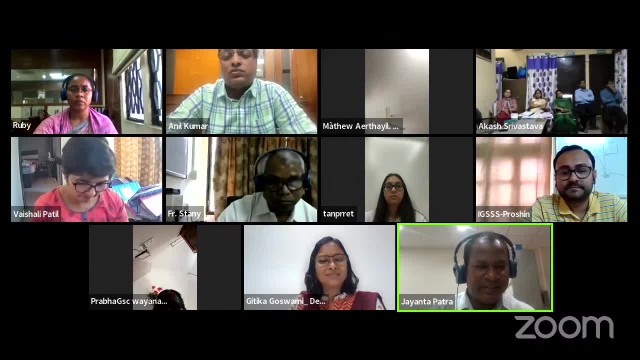 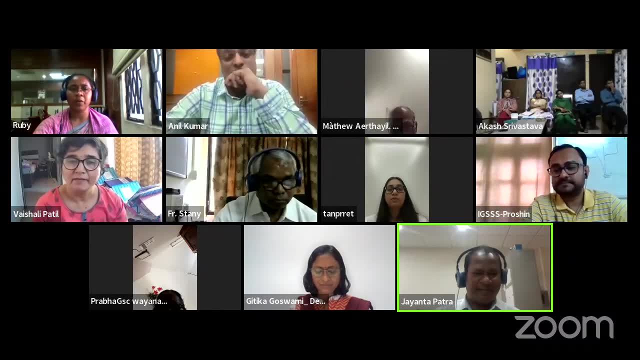 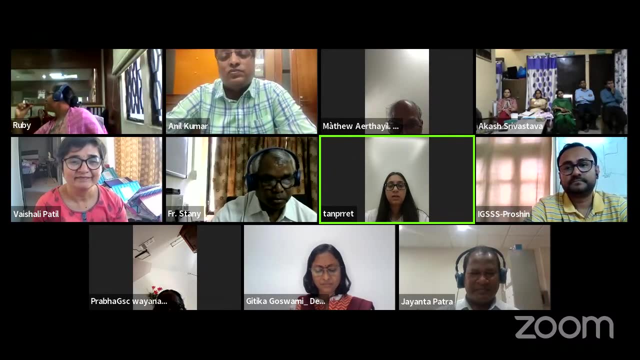 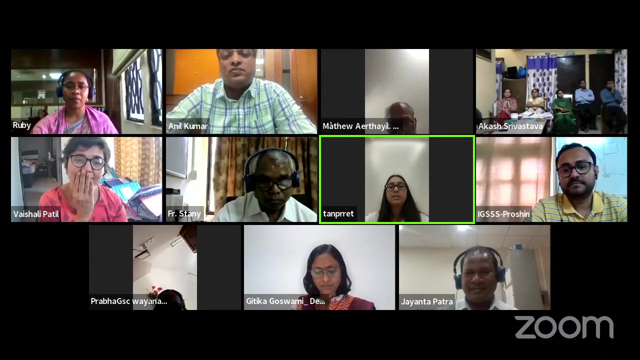 and campaign officer and Sister Ruby for the vote of. thanks, Tanpreet and Sister Ruby. Should I go first? Am I audible? Yes, It was a pleasure to have organized this Climate Change Mitigation and Adaptation Strategy Workshop. Special thanks to our thematic. 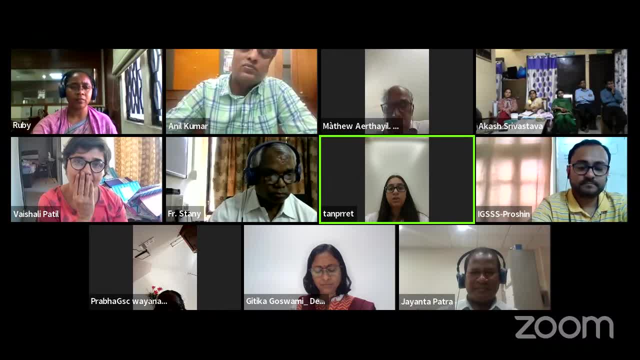 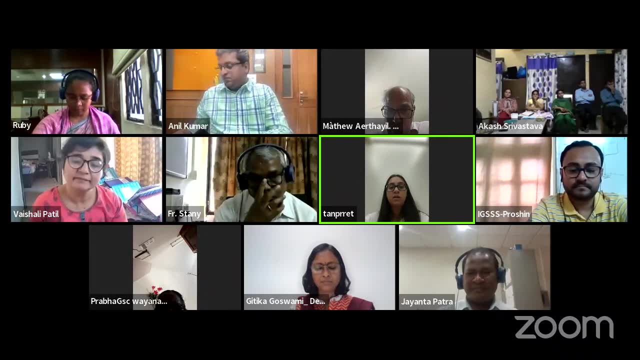 experts Dr Anjali, Ms Geetika and Mr Prashin, for sharing the knowledge and expertise with us. I would also like to thank Mr Anil, Father Stani, Jainth, Sir and Sister Ruby for all the support and management. 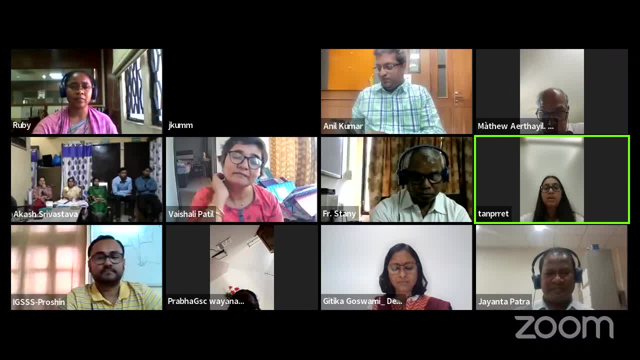 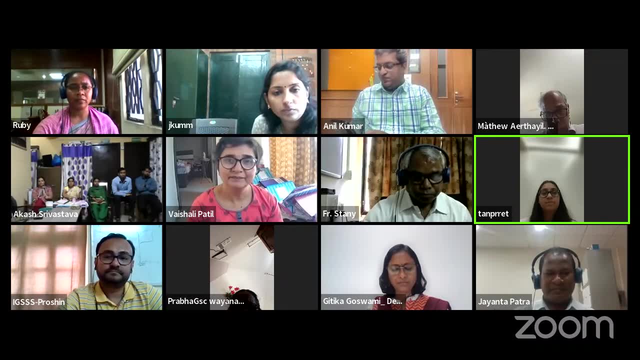 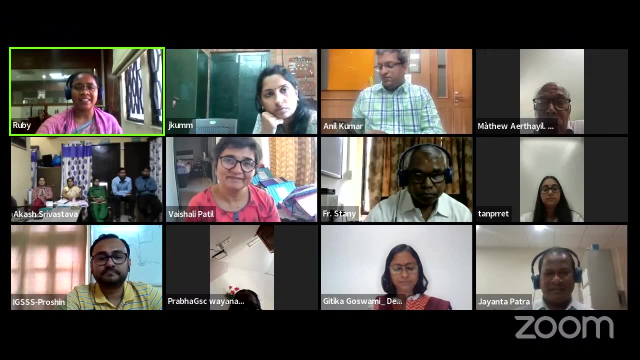 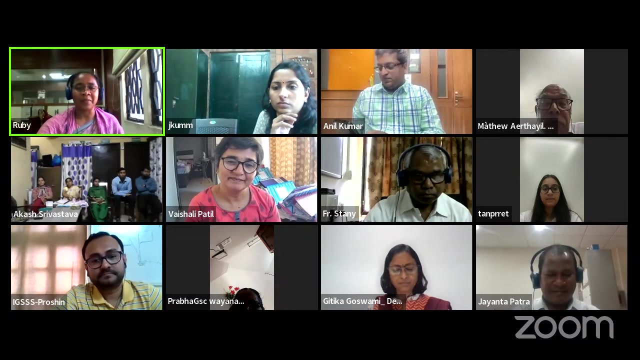 And last but not the least, thank you to all the participants for taking out time and being a part of this informative workshop. Yeah, thanks to everyone. Just I would like to tell our resource person that hundreds of our participants joined through Zoom and. 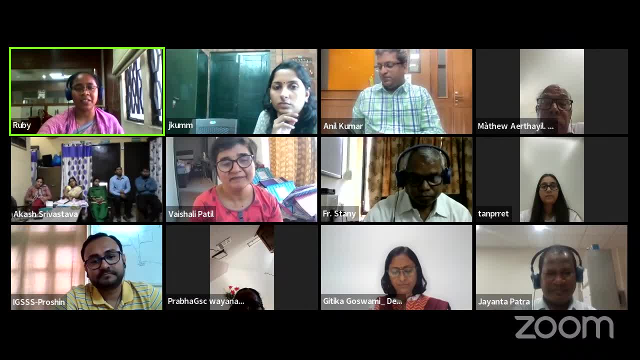 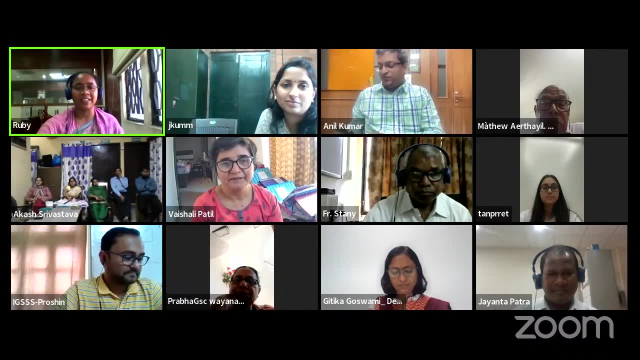 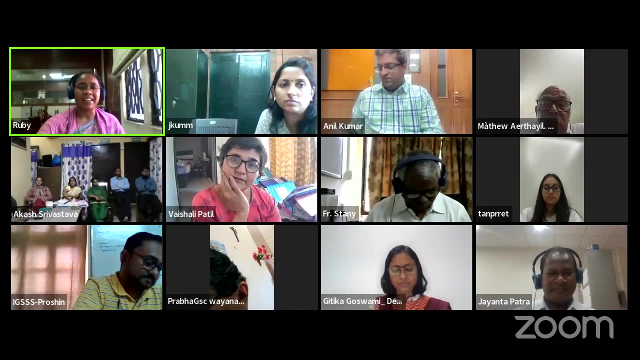 our staff, our field workers, have joined through YouTube. They could not come in, they could not keep their ideas, views, but they are watching the live streaming through YouTube. So many of us are getting the benefits from these input sessions. So thanks to